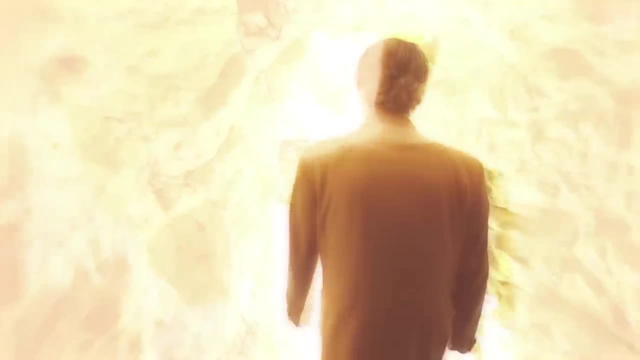 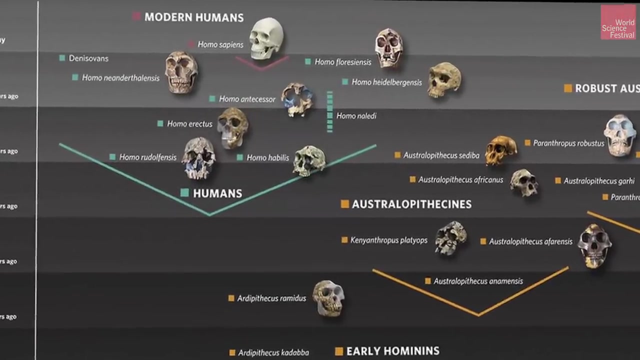 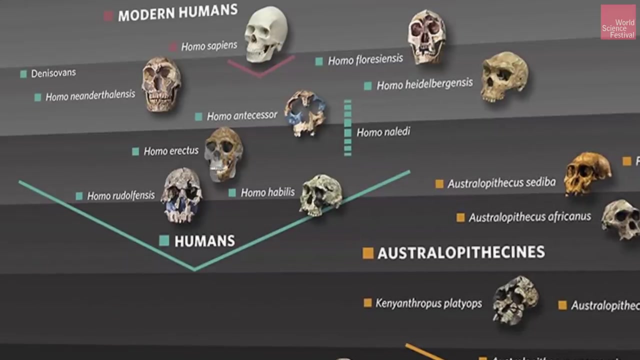 Perhaps our ability to think abstractly made the difference. We create art for pleasure, we use materials to communicate information and ideas, we develop rituals that create cohesion and identity within a community, And that level of abstract reasoning is a profound part of what defines us. That's what makes us human, But new research is challenging this perspective. 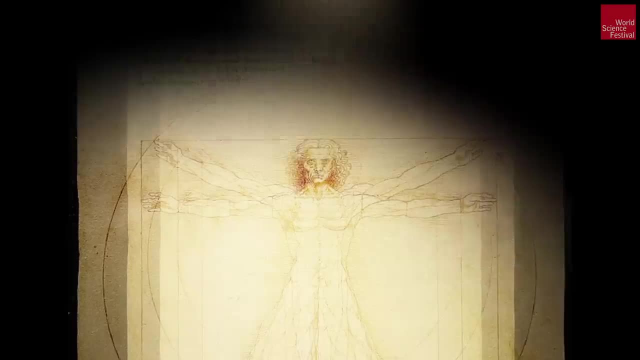 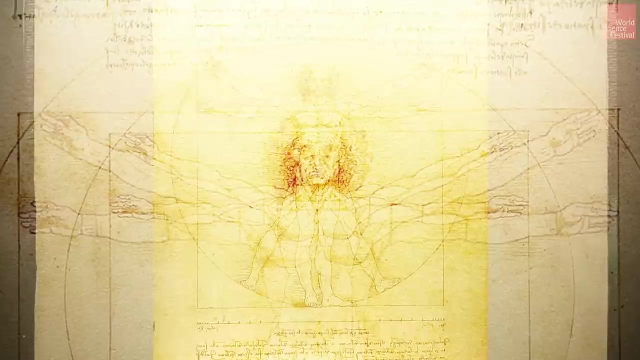 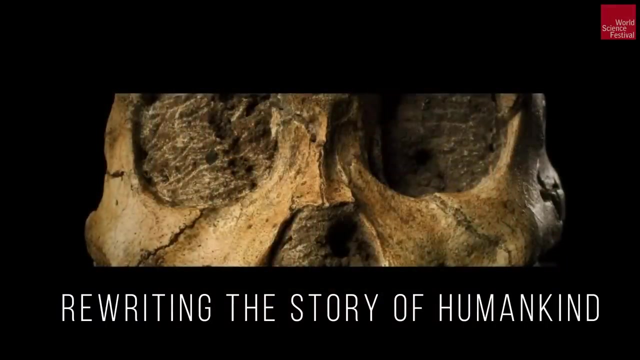 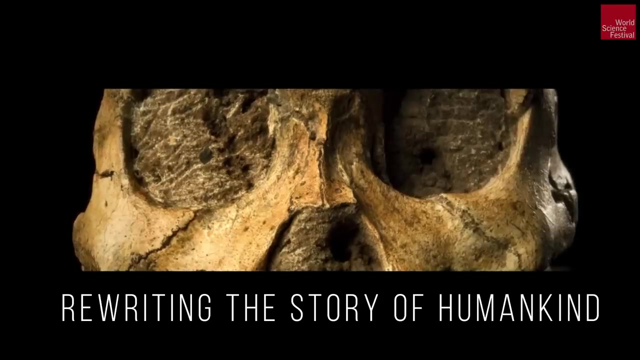 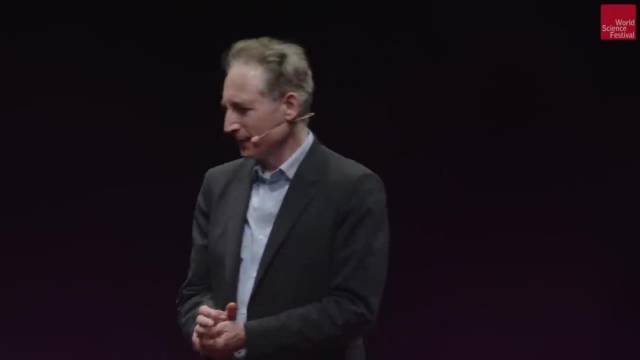 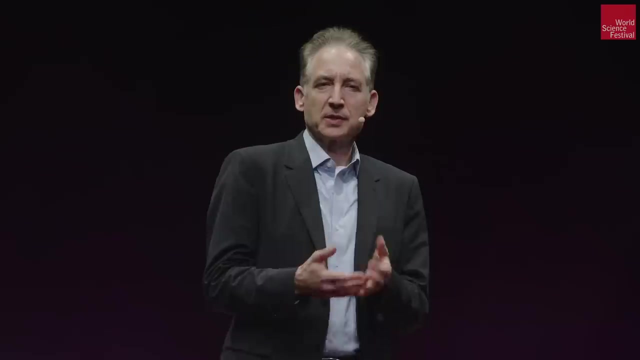 by raising the tantalizing possibility that we may not be as different as we once thought, Because some of the other early human species may have also had creative and abstract identities, findings that may well be rewriting the story of humankind. Thank you, You know, when we try to answer some of those questions, questions that really speak to. 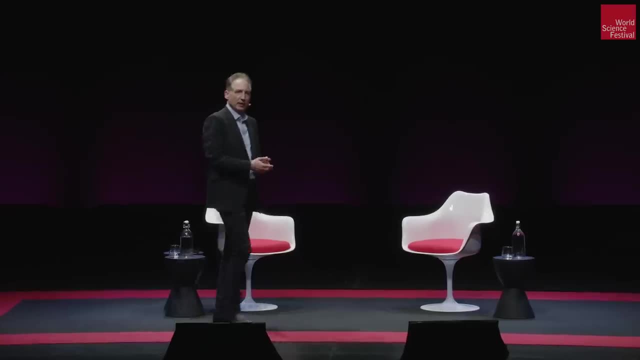 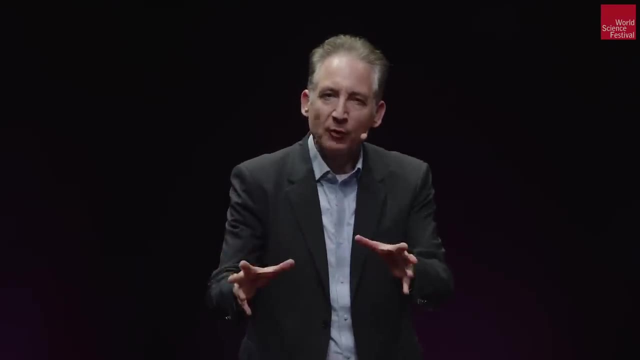 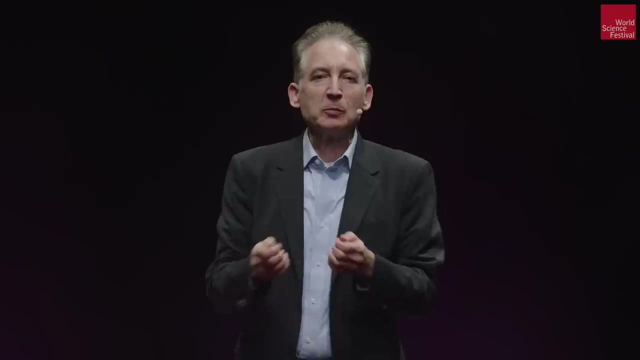 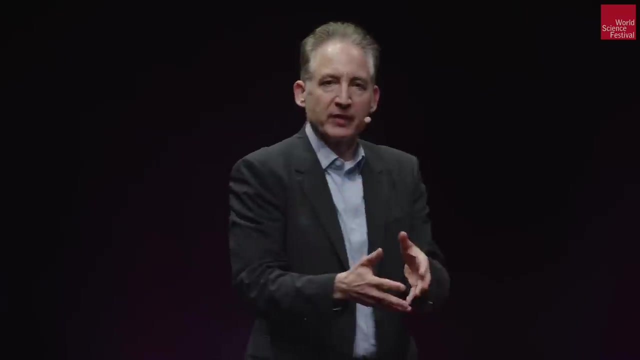 who we are, how we fit in to a grand story, a grand narrative. Issues of origin prove to be these powerful anchors of our understanding, at least in part. That's why many of us are consumed with trying to understand the Big Bang, the origin of the universe, the origin of it all We are driven to understand. 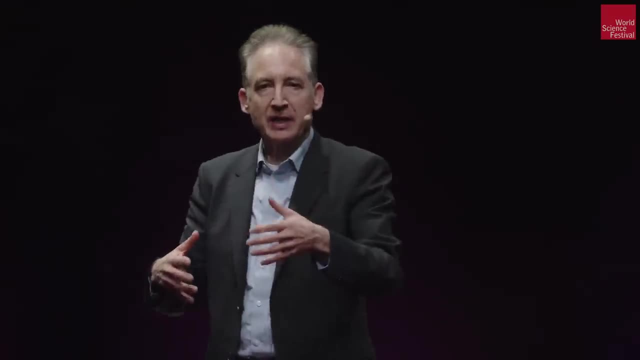 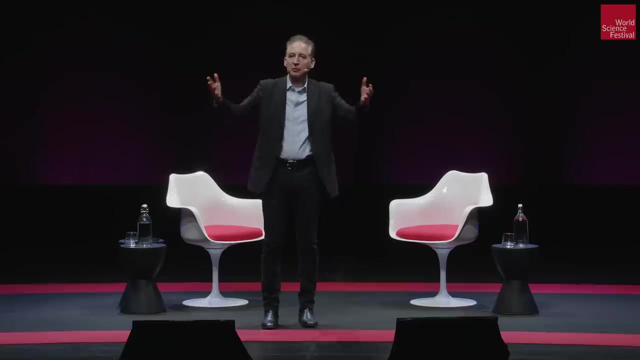 the origin of galaxies and stars and planets. We want to know the origin of life. We want to know where intelligence comes from And, as we pass through the lineages, we want to know where our genus came from, where our species has come from. And this is a journey. 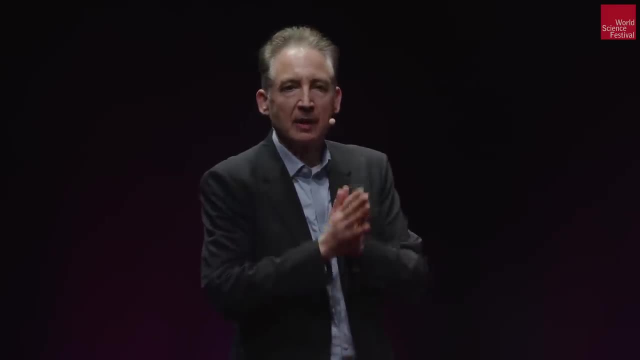 as briefly noted in that piece, that we have vigorously pursued for some time, And our guest here today is a person who has been a member of the Big Bang for a long time. He's been a member of the Big Bang for a long time. He's been a member of the Big Bang for a long time. 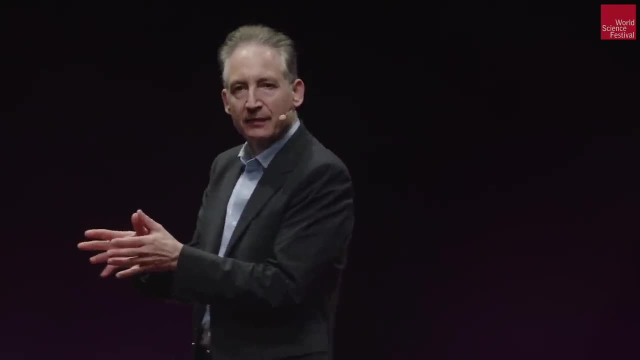 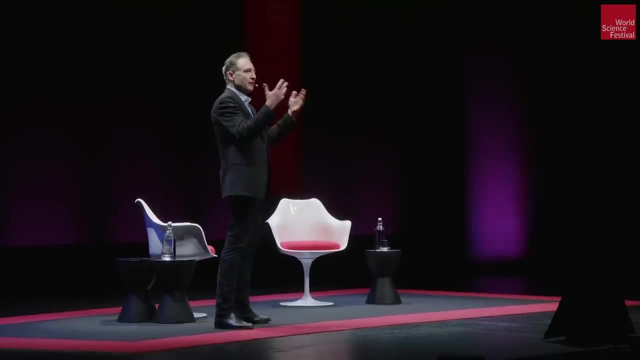 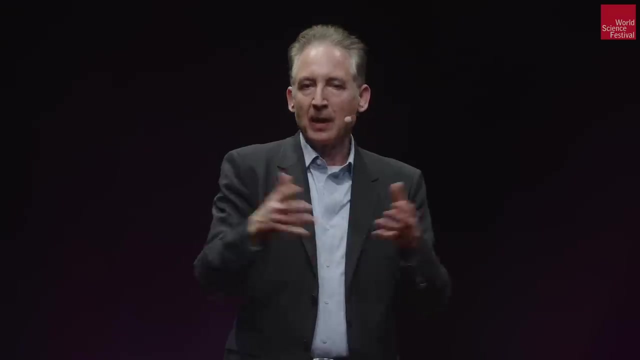 And our guest here today is one of the leading lights of the field. Our guest is Lee Berger, a name who many of you are deeply familiar with, who has made some of the real great discoveries in trying to further our understanding of those deep questions. He is the chair of the Paleoanthropology. 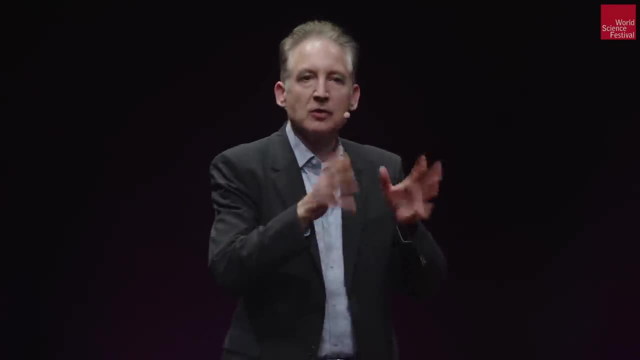 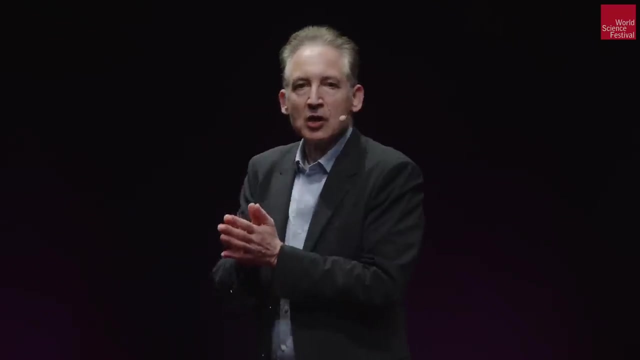 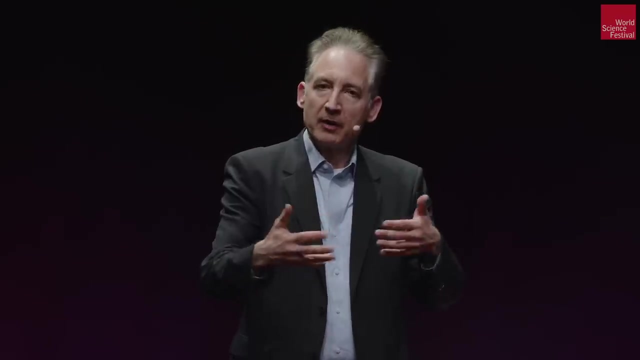 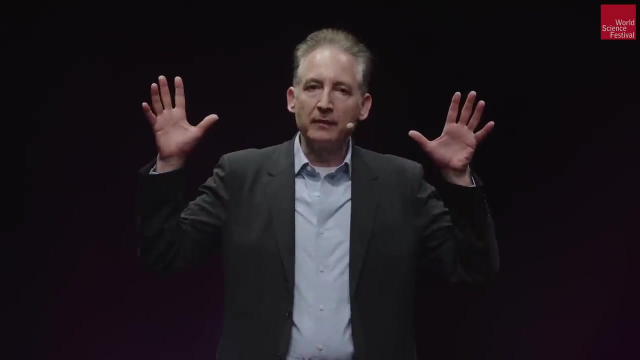 Department at the University of Witwatersrand in Johannesburg, South Africa. He has had wonderful series on National Geographic, NOVA and he is here today to give us a sense of where we are in this grand quest. And the wonderful thing about Lee is not only is he one of the prime movers in our 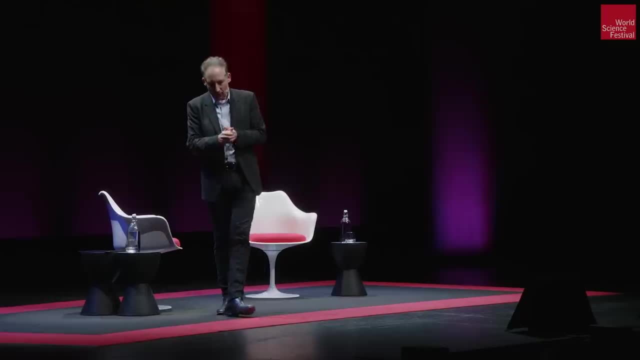 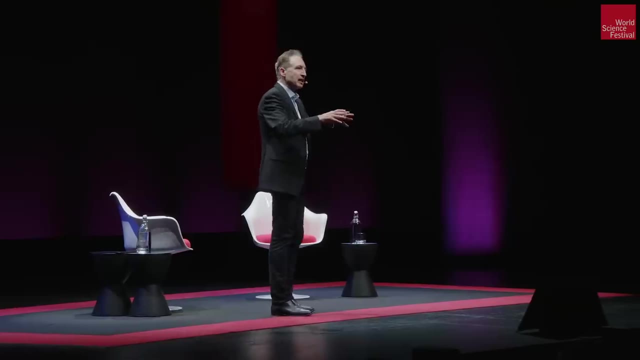 evolving understanding of our own evolution. he is also one of the great narrators of science, one of the great storytellers that speaks to the world. And he is also one of the great narrators of science, one of the great storytellers that speaks to this journey that we humans have. 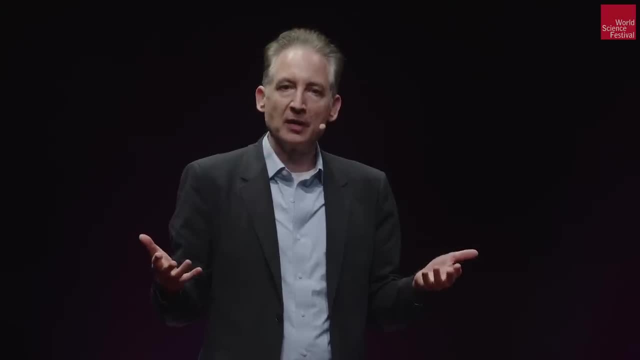 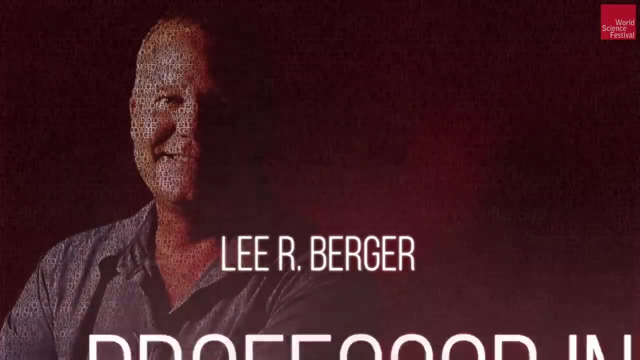 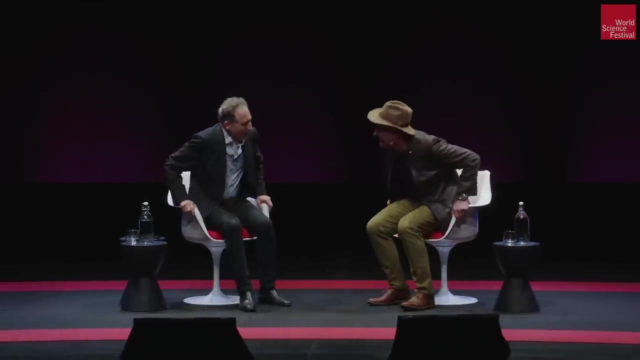 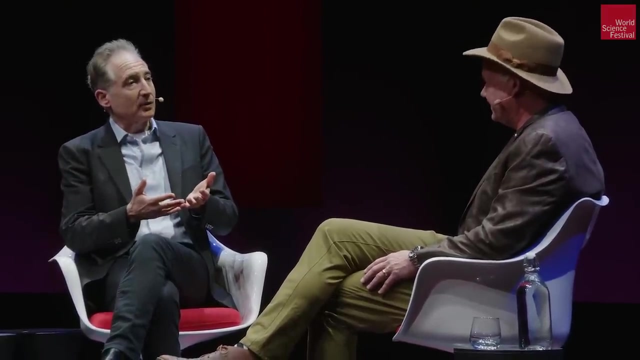 been on to try to understand ourselves, And so it really does give me great pleasure to welcome to the stage Lee Berger. Thank you, Thank you everyone. Thank you, Brian, Thank you All right, So in our discussion today, it would be great to get caught up on the rapidly moving field of 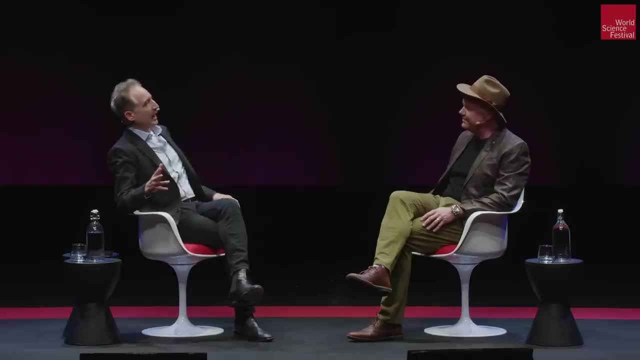 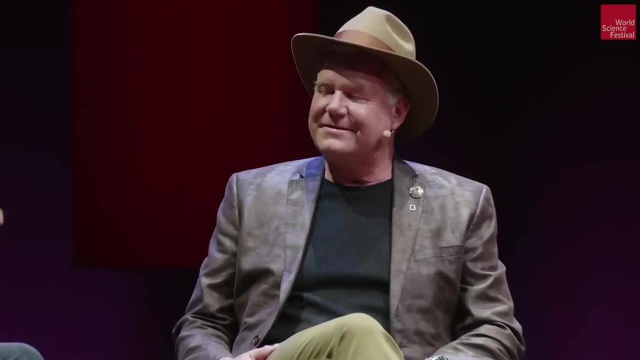 understanding human origins. But before we get to that particular story which speaks to all of us, if you don't mind, I'd like to spend a little bit of time on your individual story because, look, I mean part of the. 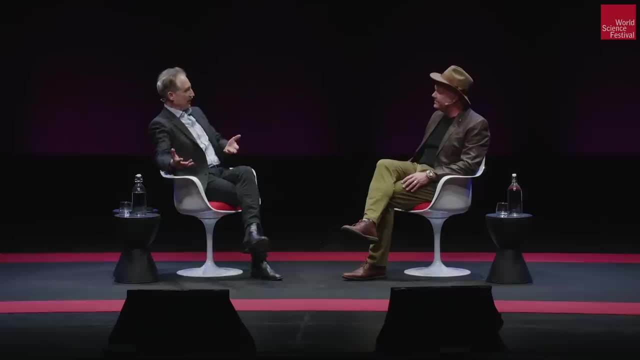 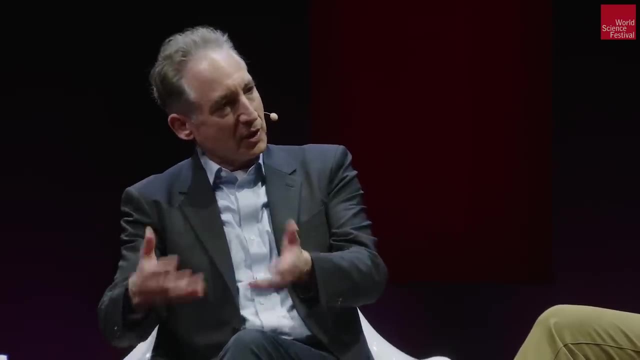 reason we have these conversations is you know you want to inspire the next generation so that they can get a sense of you know what it takes to be somebody who really changes our understanding in the way that you and your colleagues have. So 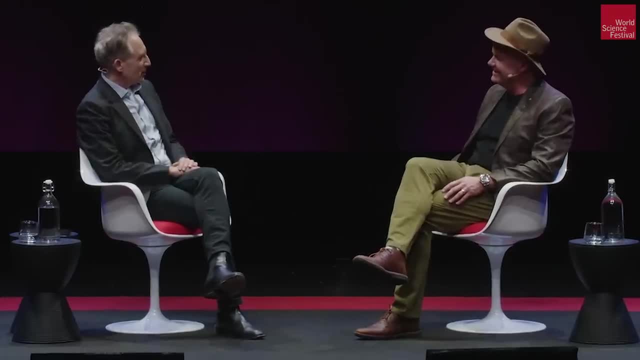 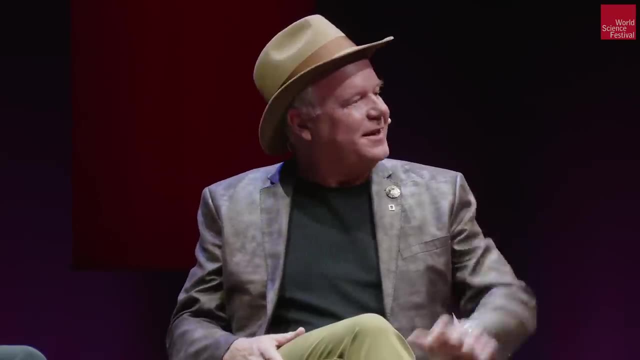 very beginning, you were born in Georgia. is that correct? I was born. I wasn't born in Georgia, I was born in Kansas, Kansas. I grew up in Georgia. Georgia is sort of the rural south in Hello Brisbane. It's great to be here. 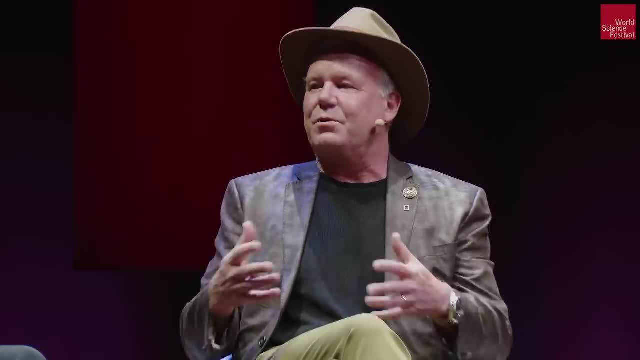 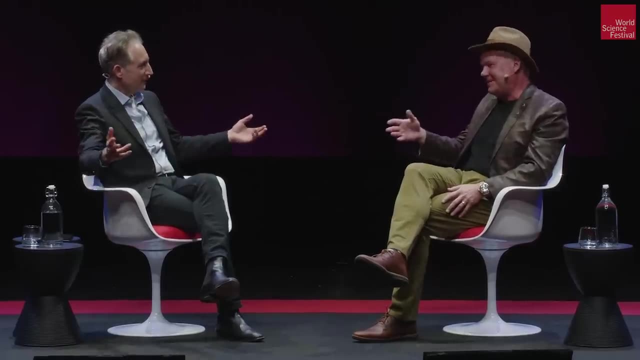 I was a kid that grew up in sort of this idyllic rural area. You know I would spend my summers fishing and running through the woods and, Like Dorothy, Like without the dress- Yeah, Mostly Yeah, And I would. I was fascinated. 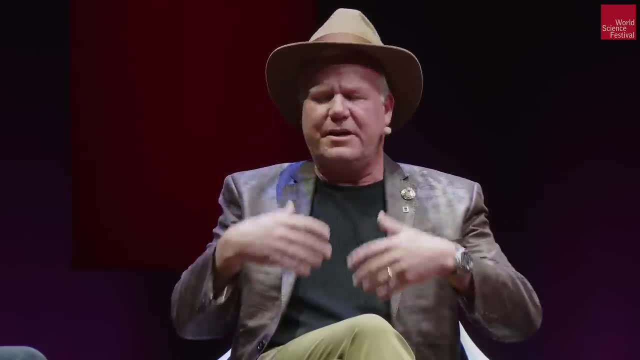 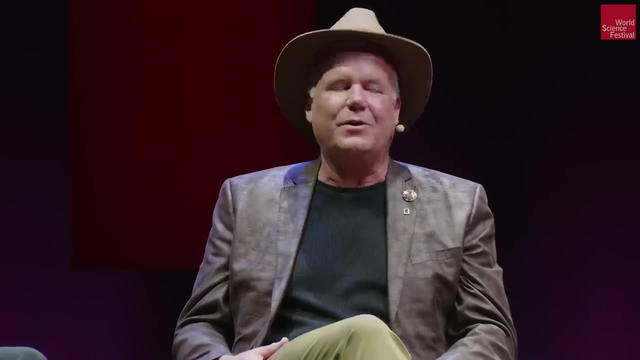 Even as a child with you know, Native American artifacts which appear from plowed fields and geology. My, my grandfather, was a frustrated oil wildcatter. you know one of those guys missing fingers from the chains and you know, had pet chimpanzees and drove a Cadillac. 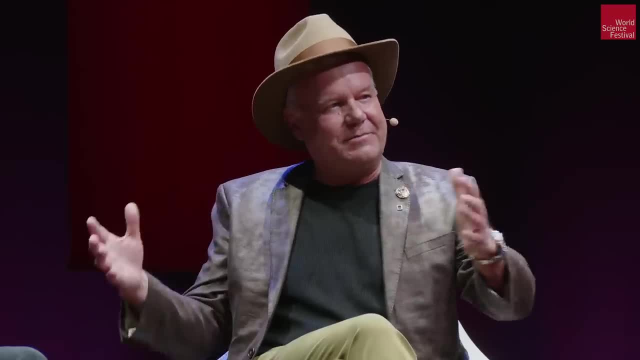 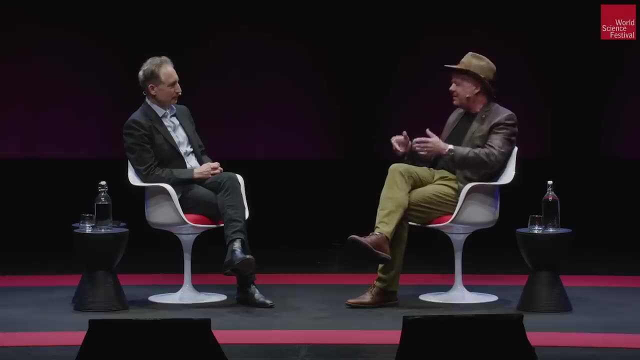 And my father grew up in the back of a slipstream trailer in the Texas and Oklahoma regions, And so there was this deep fascination. but that wasn't the pathway they ended up. They were middle class family, My mother was, I was a math teacher. 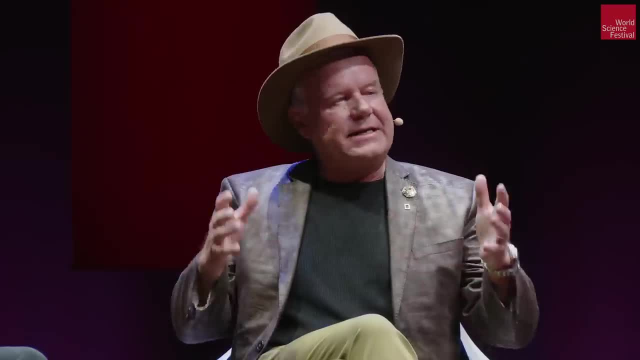 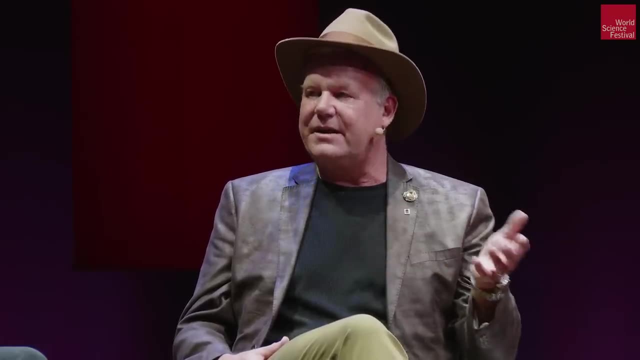 My father sold real estate and insurance and I was a bright kid in a rural community And in that time there was kind of only a few places that a bright kid could go like that And in I think it's probably a lot like rural areas everywhere in the world. 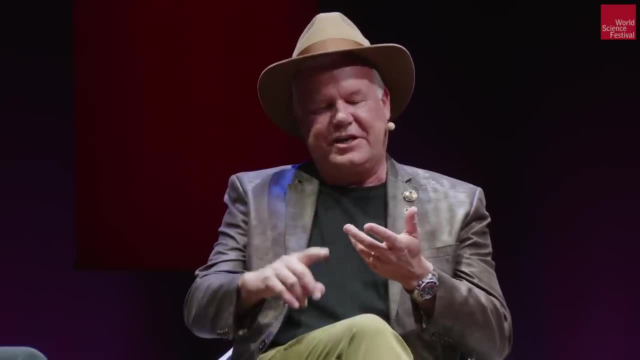 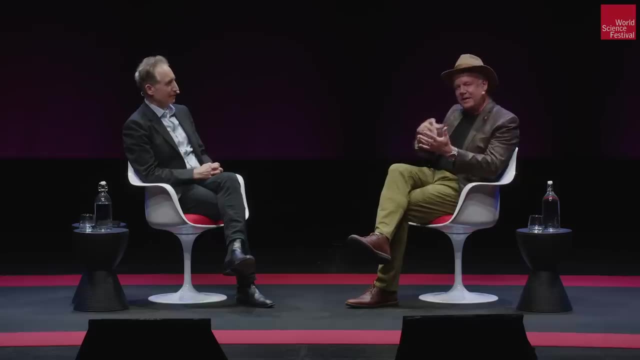 You were going to be a doctor, a lawyer, an engineer, an accountant and maybe- particular to the south of America- a preacher, And one of those would become a politician sometime or something like that. So I went. you know I had to get a scholarship. 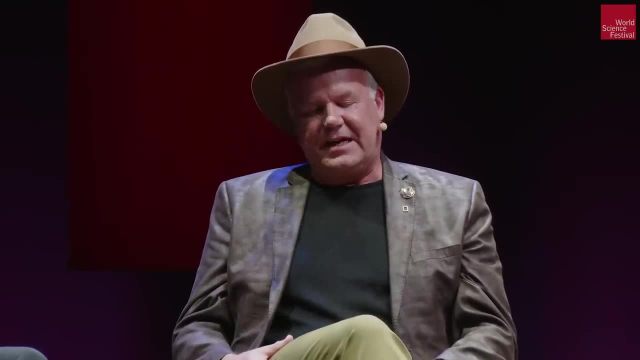 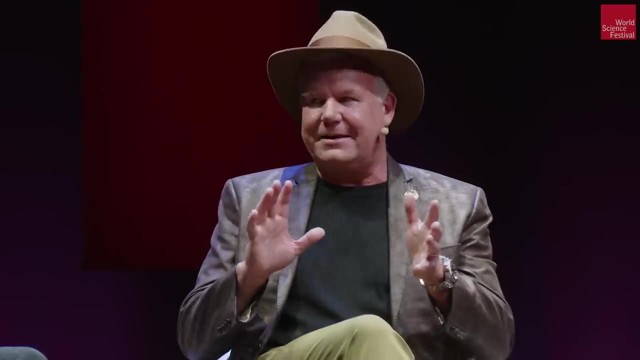 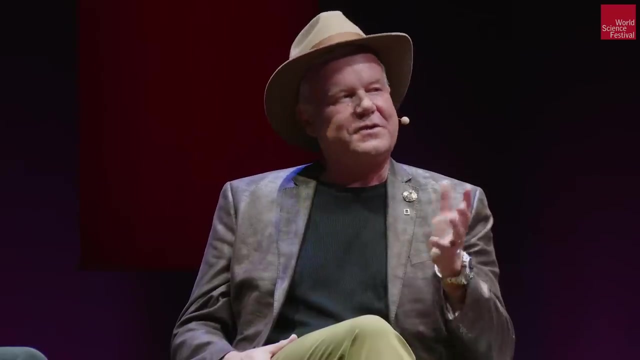 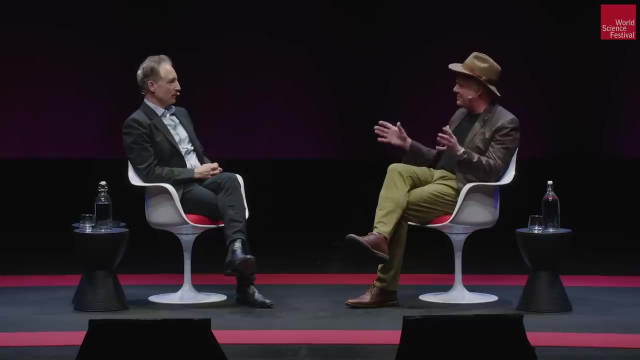 I got naval scholarship, went to university at pre-law and hated every moment, Really, Except I got to take electives. I got to take electives in geology and archaeology And for the first time in my life- which I really didn't even envision those as a career- you know, they weren't in front of me as a way to a pathway- 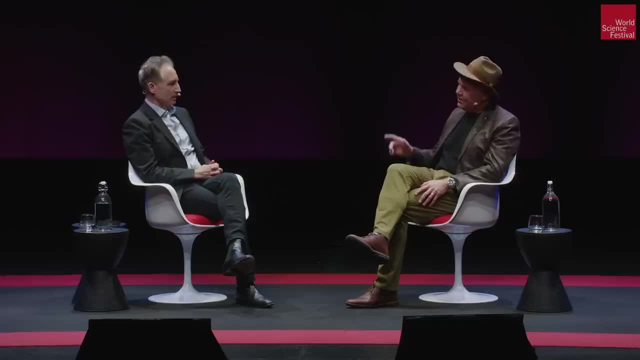 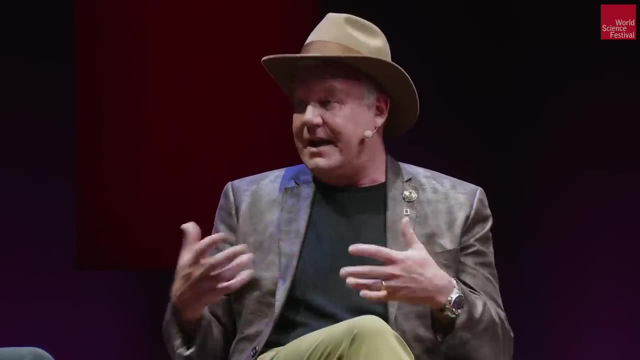 I saw people who absolutely adored what they did, And I also found out that all that time spent exploring as a kid was valuable in finding fossils. I had a knack for it: I could go with a field trip and see the fossils they were looking for and find them. And I became one of these funny things of failing all my main courses, literally F's and D's, you know on that. Is that really true? That's true, And making straight A's in all my electives, Hmm. 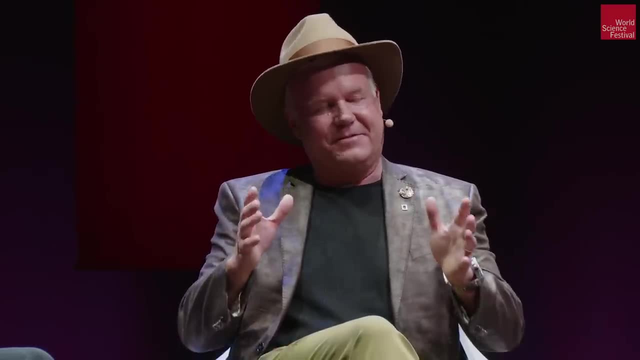 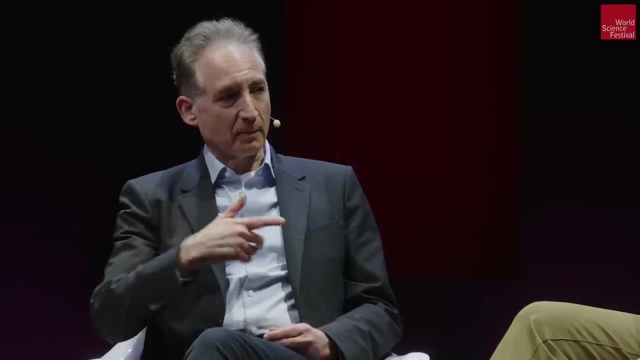 And I ended up in front of this naval officer. You know he was my academic officer And one of the horrible things was at that time, if you'd accepted one of these officer scholarships, You'd have to pay it back. Is that really true? 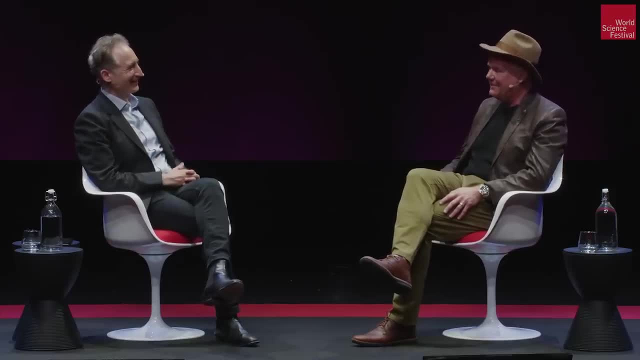 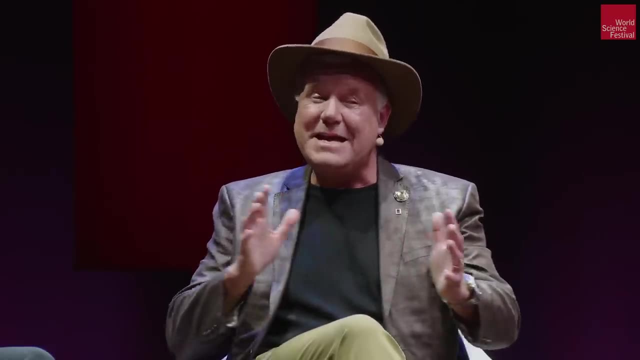 You'd have to pay it back if you fail out And you go enlisted to do that. And Vanderbilt, where I was, was a very expensive school. It had been many, many years in the Navy, And so I'm standing there at attention. 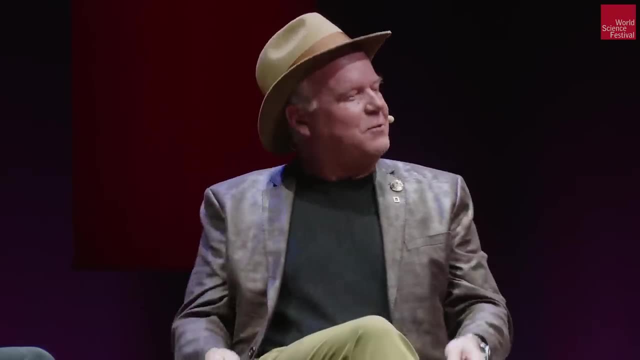 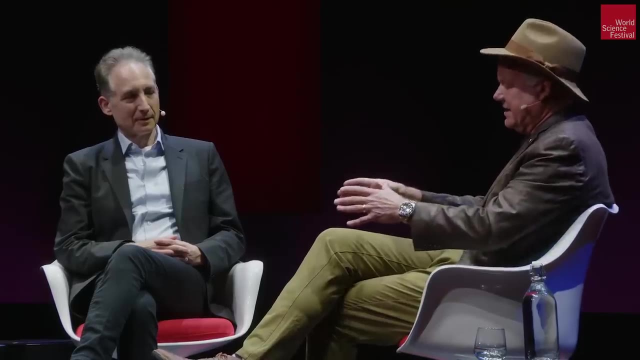 You got to imagine this. You know, I'm in my, you know these sort of top gun whites standing there, Attention, in front of this officer, That's my life in his hands, My attention. And he's got this paper on his desk, which is my transcript, which is embarrassing because there's lots of F's and D's on it, you know. 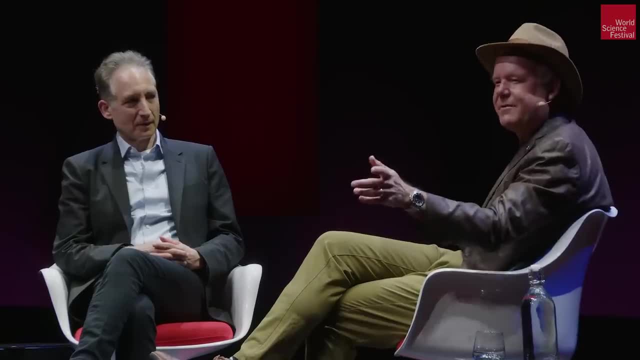 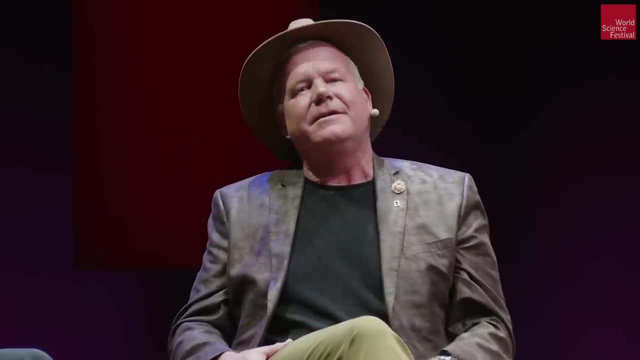 And he says Berger- Lieutenant Ron Stites, by the way, naval aviator- And he said Berger. he says what do you see here? And he pushes it across with one finger And I remember going something like: you know failure, sir. you know something dramatic like that. 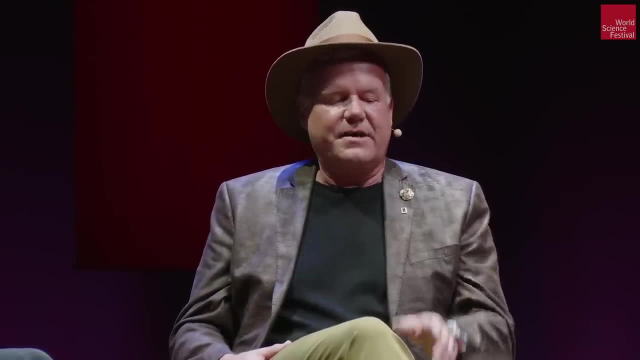 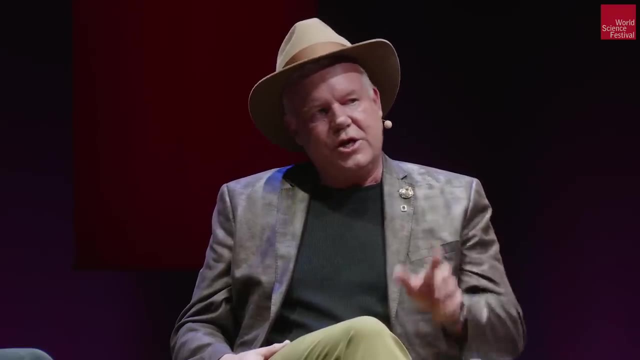 He said: I don't see that. He says I see a young man who hasn't found what he loves. He said: if you promise me this, you will Quit the university right now. Go find what you love and then come back. 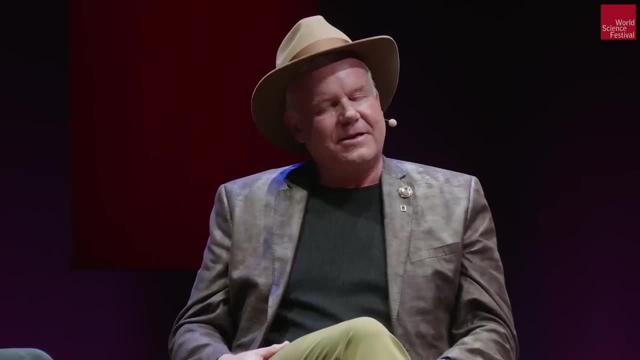 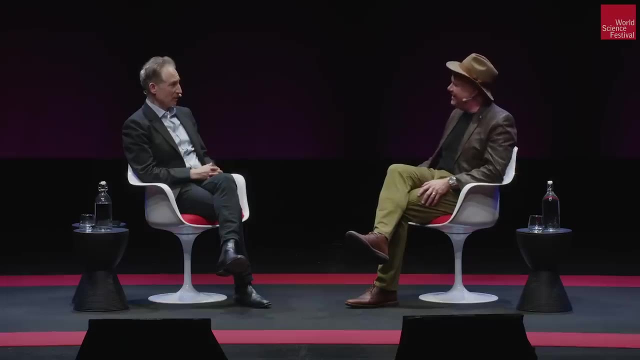 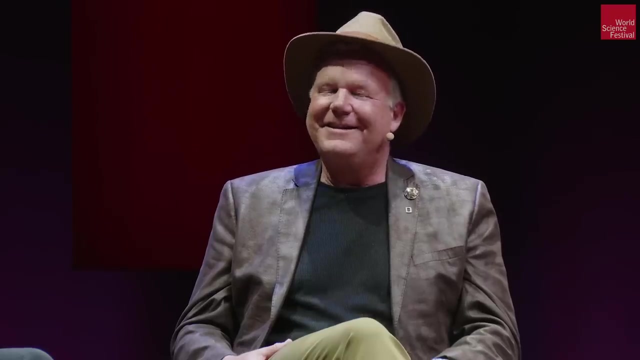 And he pointed to the geology and archeology. I'll let you out, I'll sign your release papers with no. That's hugely unusual, Boy. you know it was. he had it particularly for a naval officer. Yeah, And I said yes. 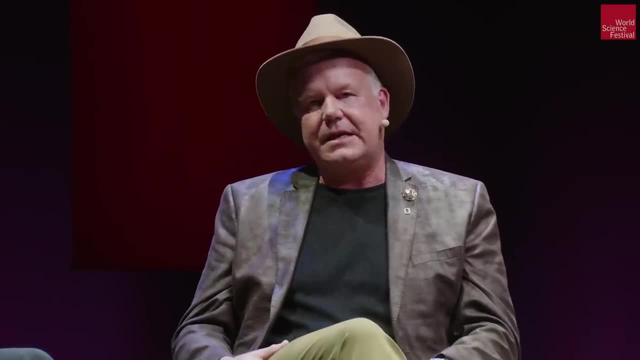 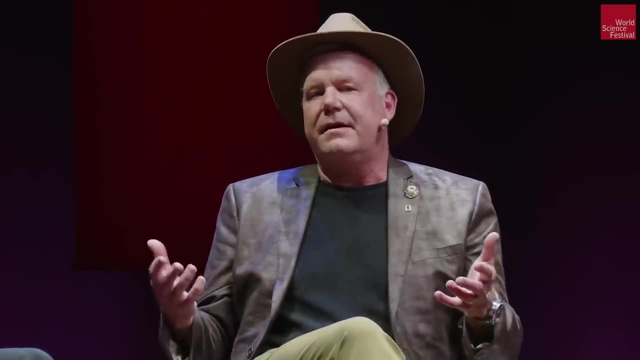 And went and found Myself and eventually came back to university And it was never work for a second after that. You know I'd found this place And that took me on this journey that I was going to. you know I came back. 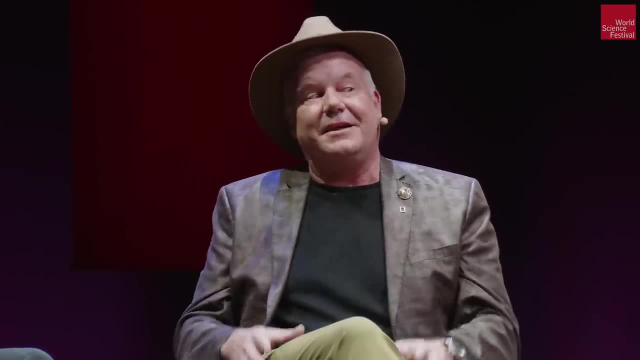 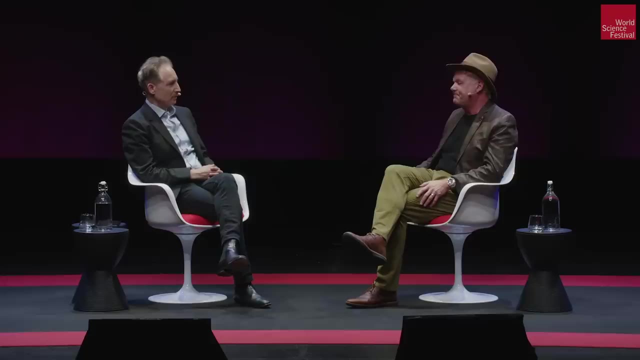 And, of course, I found paleontology like one does, And I found dinosaur paleontology like every young person does, And I was going to be a dinosaur paleontologist And I read a book called Lucy Sure, Don Johnson. I'm sure many people have read that. 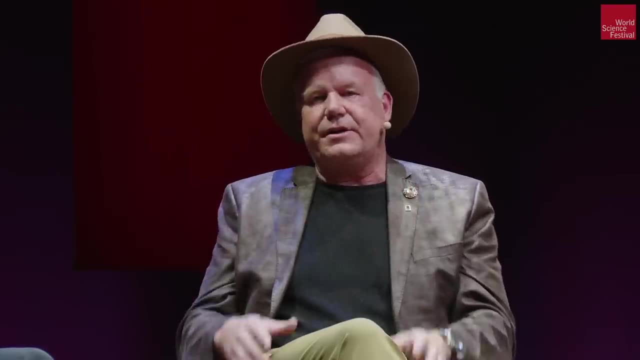 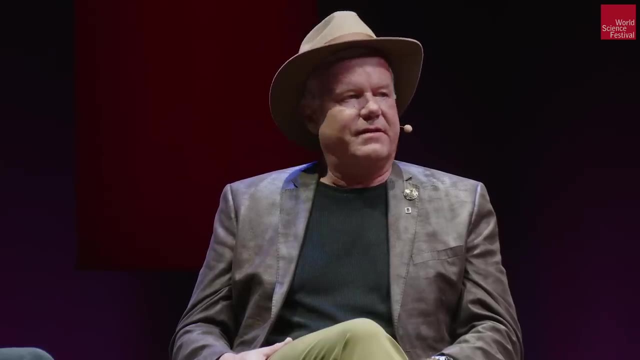 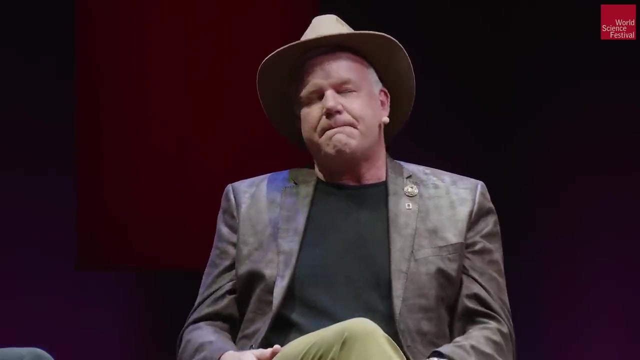 And in that and in the discussions that were occurring around that, Don had said that there's something like a one in 10 million chance of discovering an ancient human relative fossil, even if you are in an area where they are known to be, And it was in Africa. 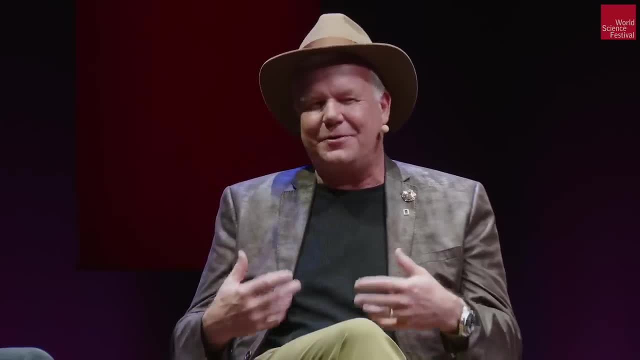 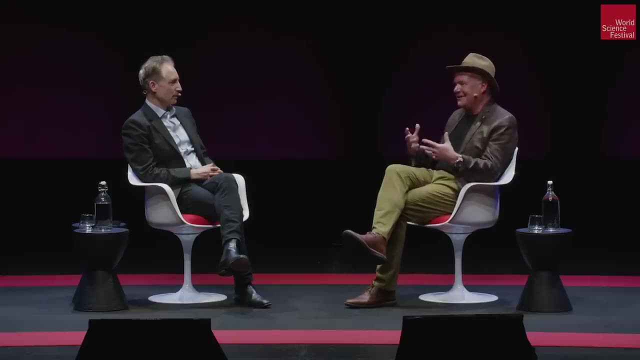 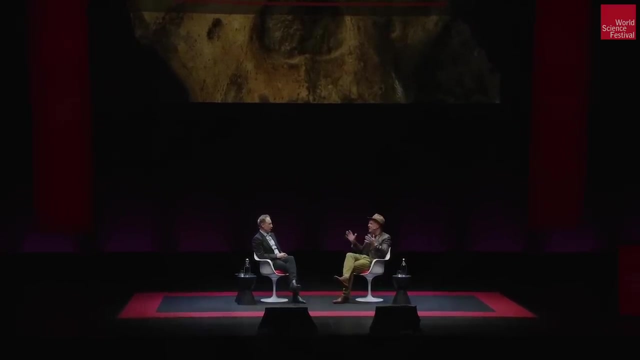 And for some reason that had incredible attractiveness and resonance me, And maybe I shouldn't be proud of that And maybe I shouldn't even reflect that, But it had. You know, I was thinking. here's a field that, even if you make a tiny discovery, you can change. 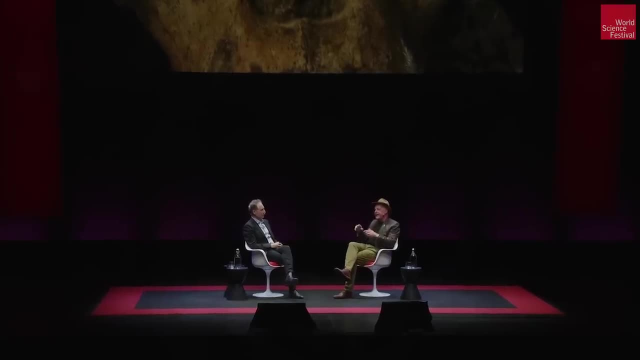 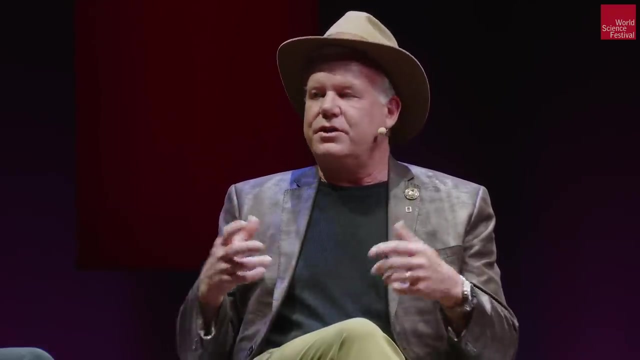 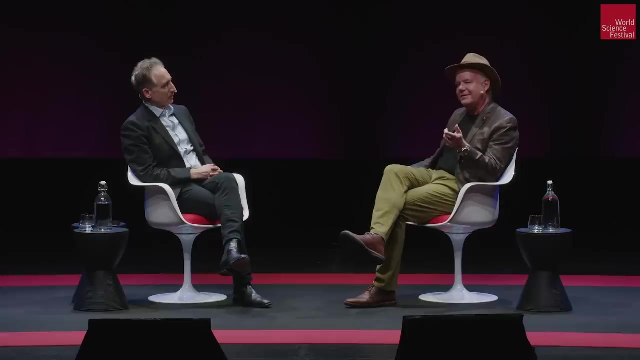 I mean at that time. it's hard for people, I think, to imagine. At that time in history there were almost certainly more people who studied human origins and evolution than there were physical objects they studied. Imagine that. Imagine a field of science that has more practitioners than it does data. 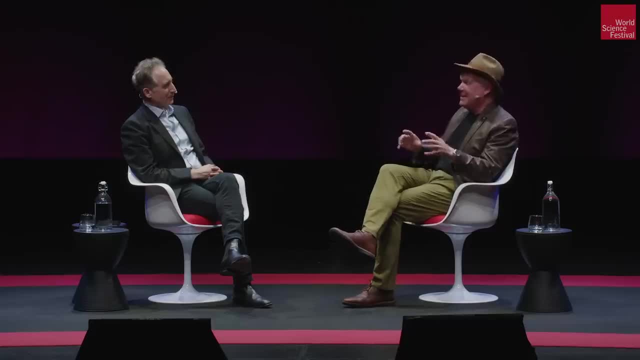 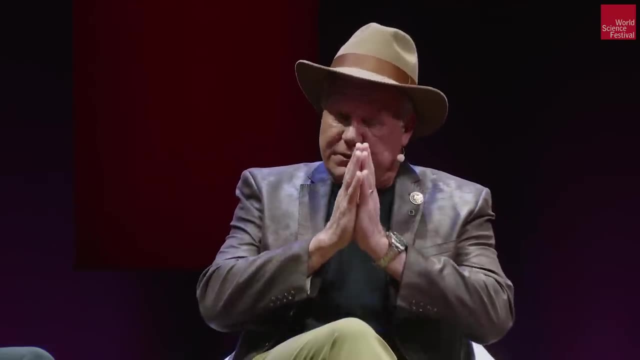 It does not make for a pretty field of science. It does not make for a pretty field of science. It does not make for a pretty field of science, I assure you. It makes for a very violent, possessive, scarce science, And paleoanthropology was every bit of that in the late 80s and early 90s. 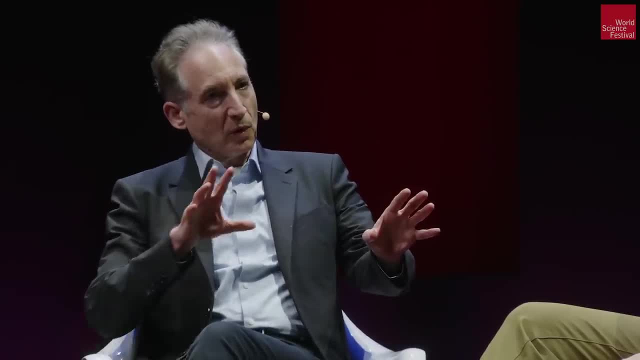 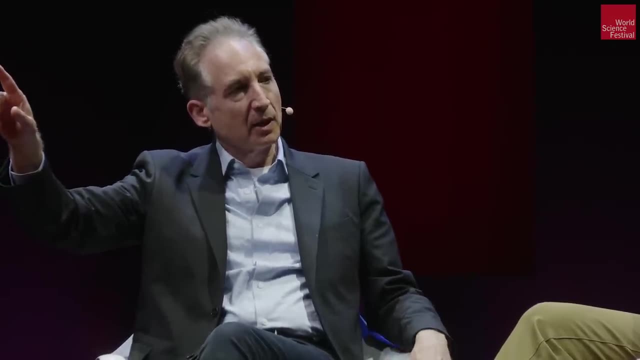 But there's something really interesting there. So you were driven more by the challenge than necessarily the specific content. I mean, if it was one in 10 million to find you know a bone of you know a giraffe or some ancient sort. 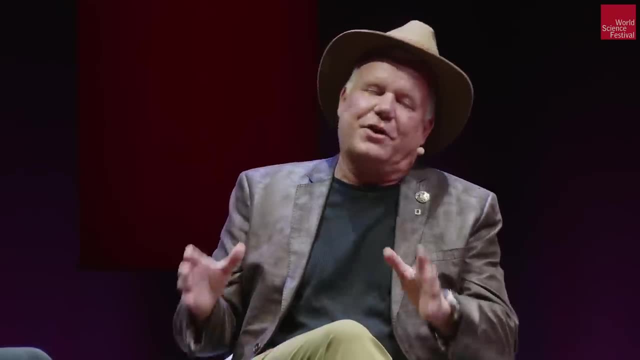 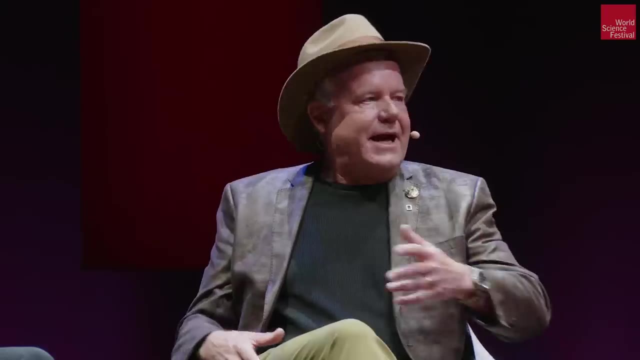 that might have been the direction that you went, Absolutely To be honest. I mean, who isn't interested in human origins, right? Who isn't interested in where you come from? Same reason, I bet everyone in this audience has looked at their genealogy. 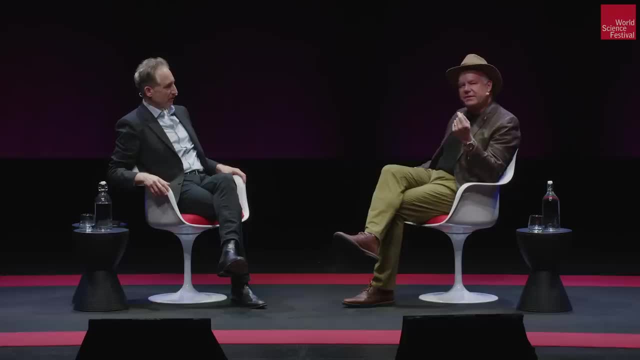 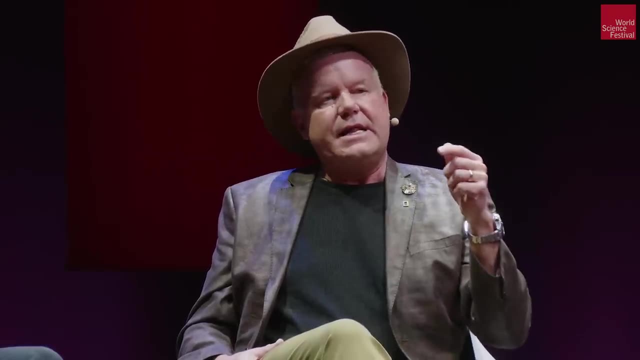 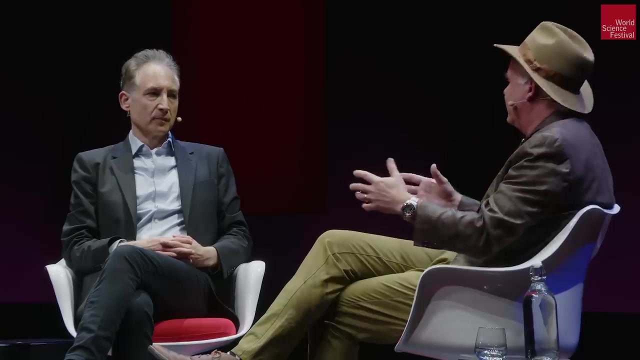 You ever wondered why you do that? You do that because you understand that in your grandparents, great grandparents, those distant lineages, there is meaning and the making of you. Yeah, I just do that. people like me just do that in the extreme. 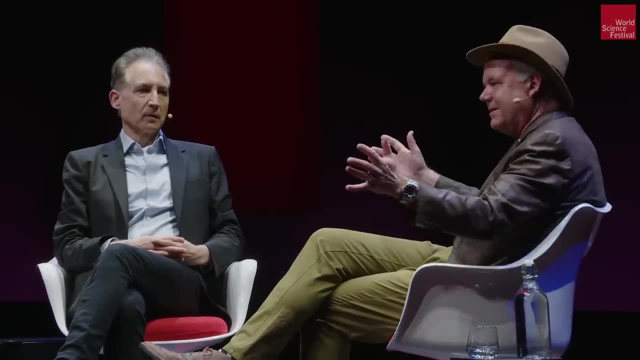 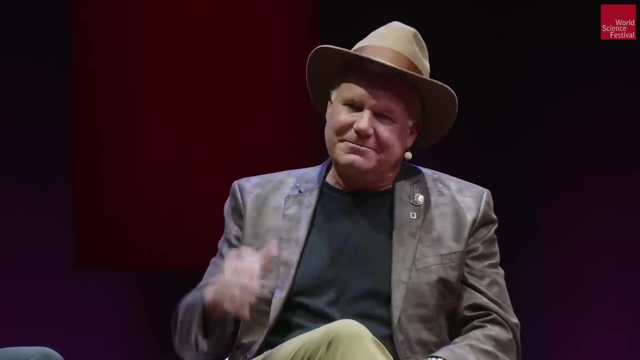 We're interested in the making of us, And so, of course, I'm attracted to that. It had meaning to me, But yeah, you know I was up for that challenge. I buy lottery tickets too, But is that the case? 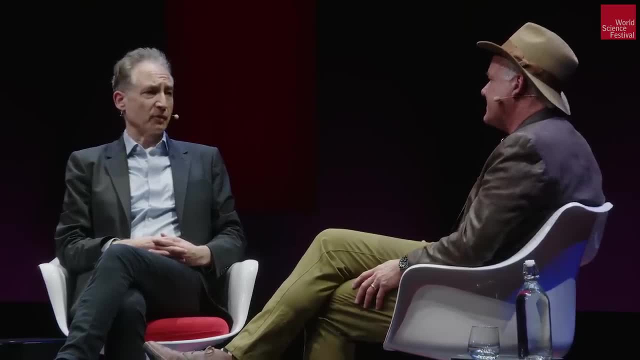 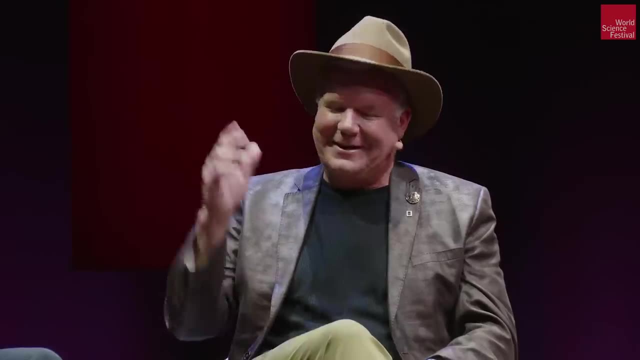 I mean, I was going to ask you, Are you? I mean, lottery ticket is not much of a risk because there's not much to lose there, But are you a risk taker? I am, I am, And I think you'll hear a little bit about that as we go on. 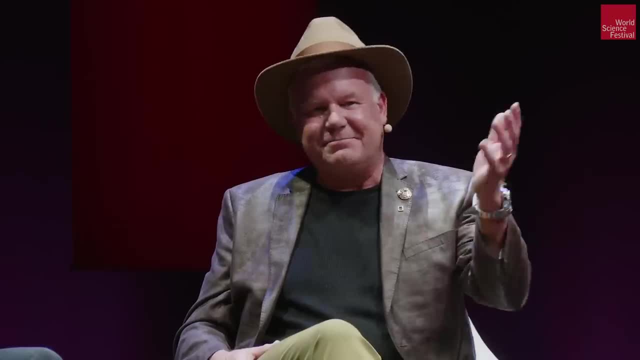 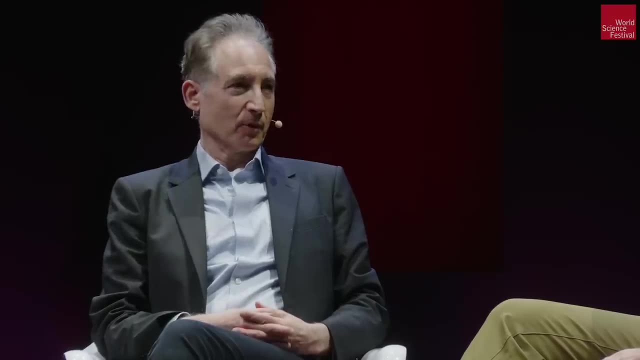 But I'm not a gambler, by the way, But I do buy a lottery ticket just because the story of my life has been sort of lottery level discoveries. But you know, you're guaranteed, if you play the lottery enough, that you will lose all your money. 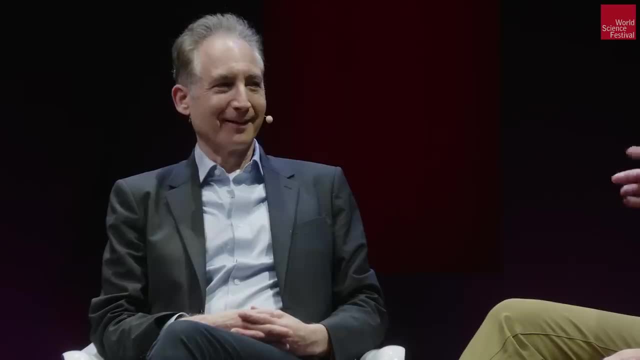 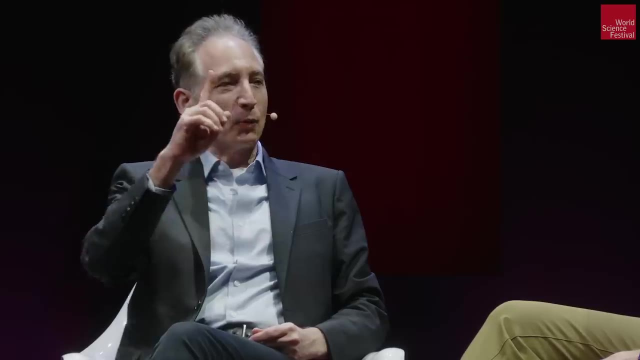 It's virtually guaranteed. I just don't find it that interesting. You're also guaranteed that if you don't buy a lottery ticket- True too- You will never win. That's true too. But that suggests you should buy one ticket, because you go from zero odds to infinitely more. 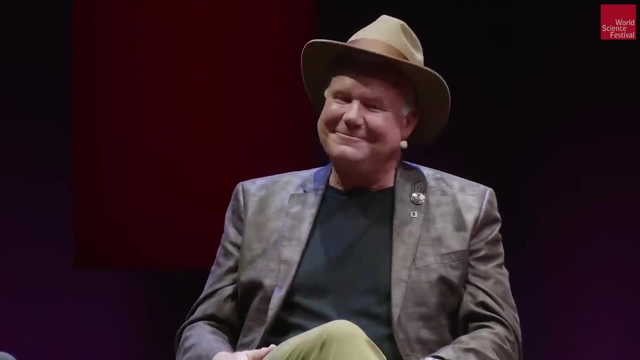 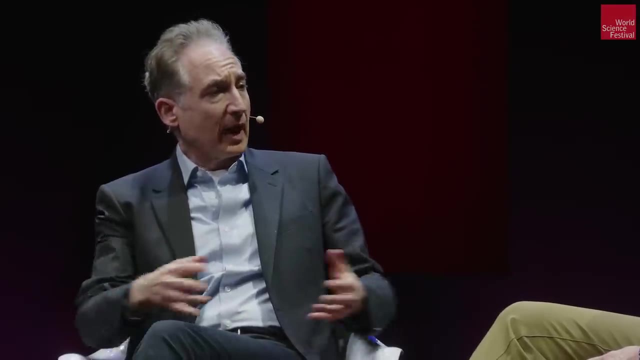 That's all I do. That's still a tiny number. That's all I do. Yeah, Okay, Anyway, so we won't fixate on the lottery. We can talk about this all night. Yeah, And so you decide to go in that direction. 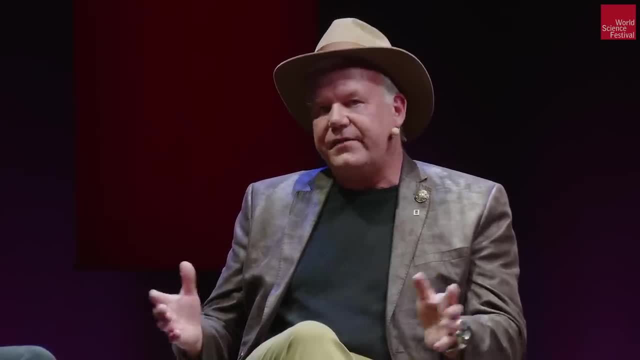 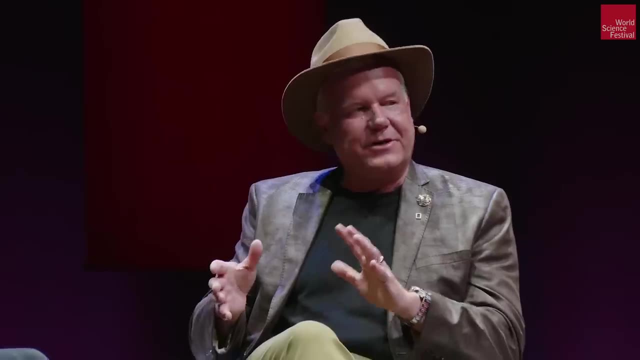 What's your next move To get to Africa? You know this is a closed field, And so I ended up making a phone call Back in the days when you had to look up phone numbers in a phone book or call an operator. 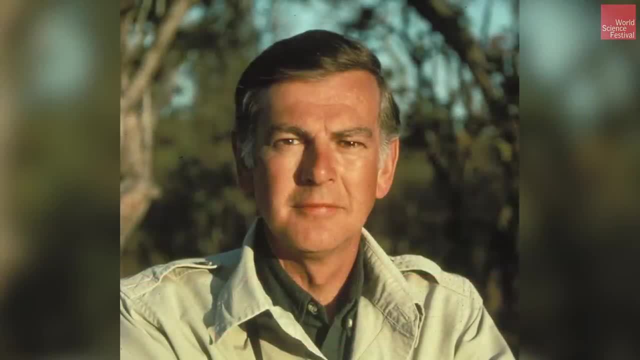 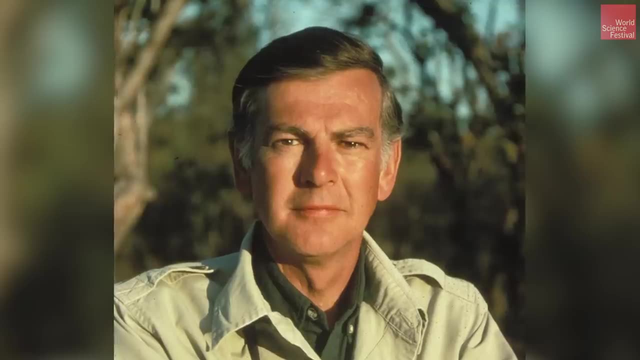 I found Don Johanson's number in California And I heard he was coming to talk to the Georgia Science Teachers Association. I called him up. I called his bulldog of a secretary. I mispronounced his name. You know, Dr Johanson in. 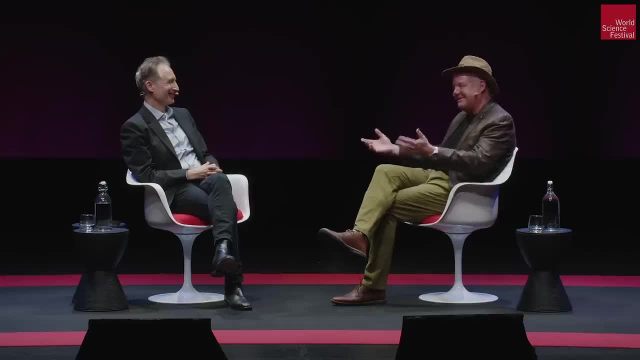 He said: Johanson, You know I was almost in And then got through to him. amazingly, He took my call And I said: you know, I live in Georgia. I'd like to meet you. And we did. 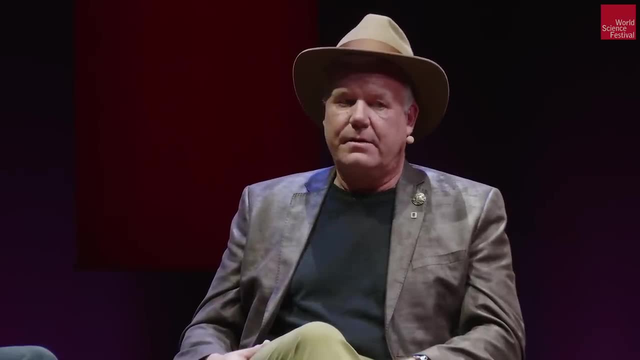 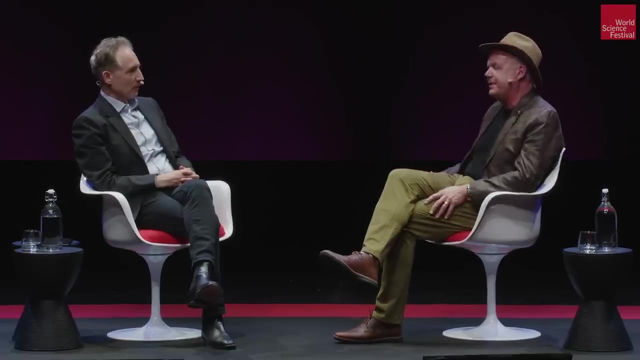 And he took a liking to me And he heard my story And I had had, by then, a degree- I was in geology and a degree in archaeology and anthropology- And he said: you know what I need: an assistant going to Olduvai Gorge, where I'm going to work. 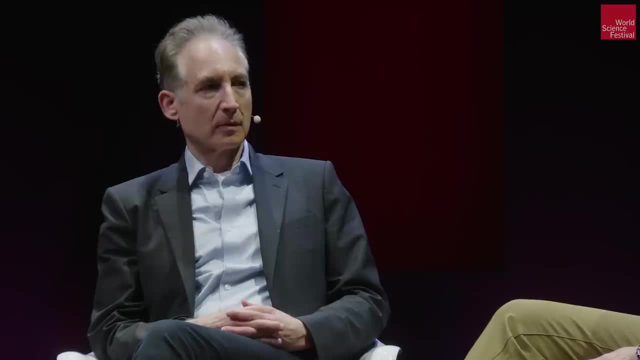 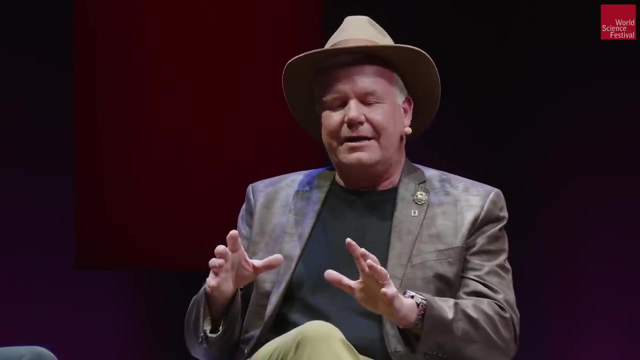 And you can be that assistant This summer. I'm made right, My life's about to happen. Go away, Scrabble together, Get money for a plane ticket. I'm on my way in that direction And I get three weeks before he's going. 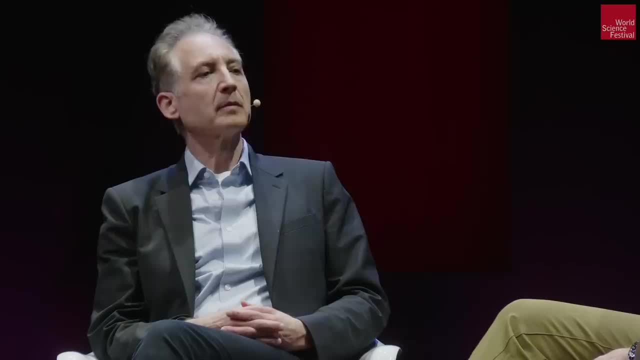 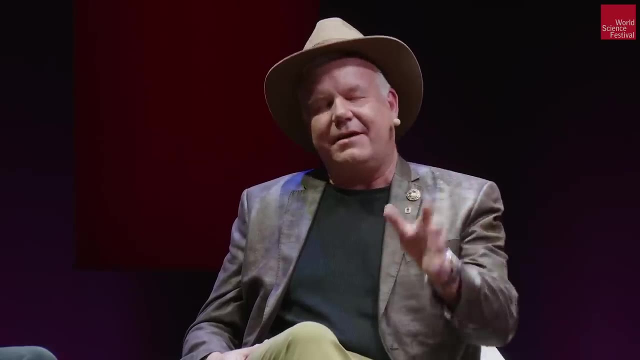 He calls up and says he lost his permit, He's not going And he did something really strange there which I've, you know. I've inquired but I never got a really truthful explanation to. He took the moment to call Richard Leakey, which some of you will hear from the great 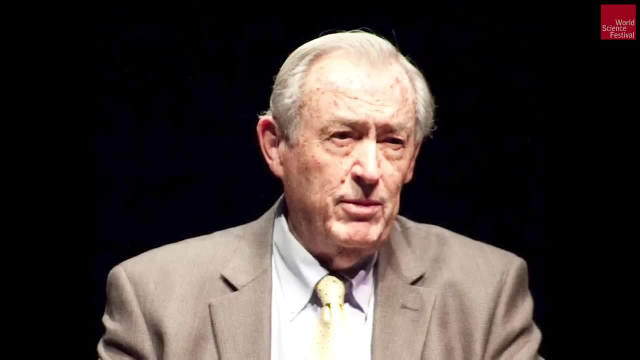 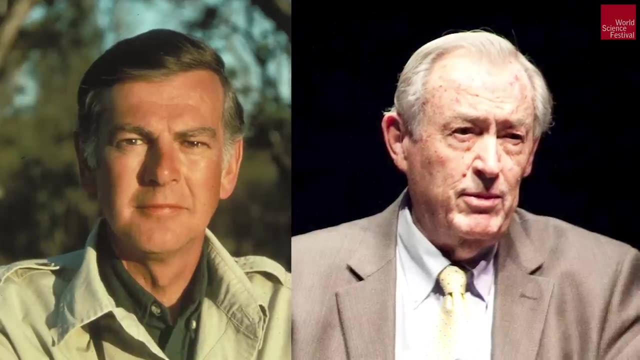 Leakey family of Kenya who he knew was holding the Harvard University Kubi 4 Field School at the same time And he said: there's this young guy and I've disappointed him. We're not going Now. a lot of people don't know this, but Don and Richard really didn't like each other. 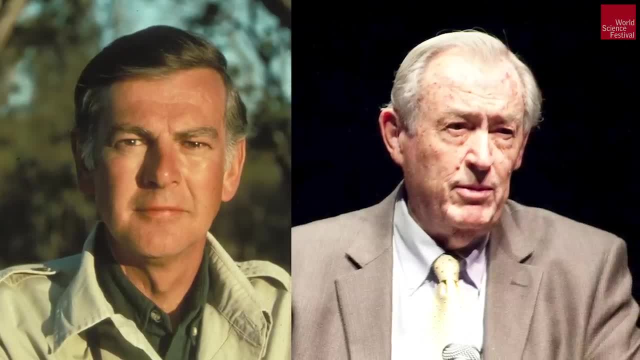 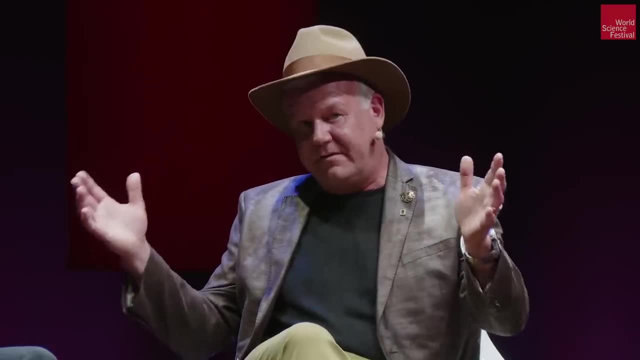 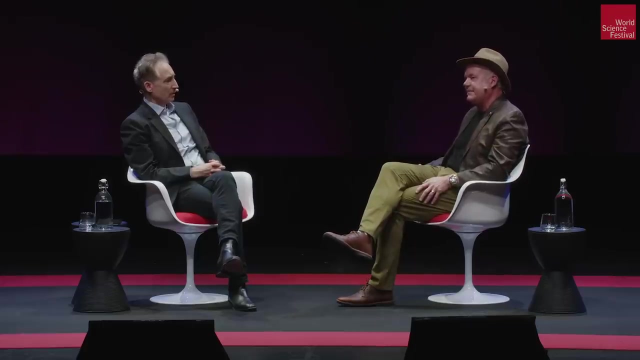 very much. They were at war with each other as two of the biggest fossil finders of that time. And for some reason, Richard said: sure you can come. And I went and I found myself in Africa. Where in Africa? Kubi 4, northern Kenya Lake, Turkana, Jade Sea. 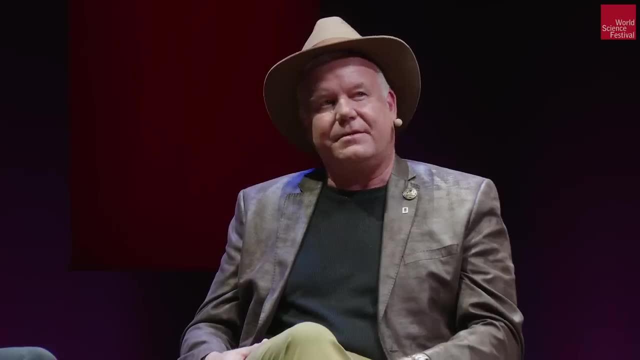 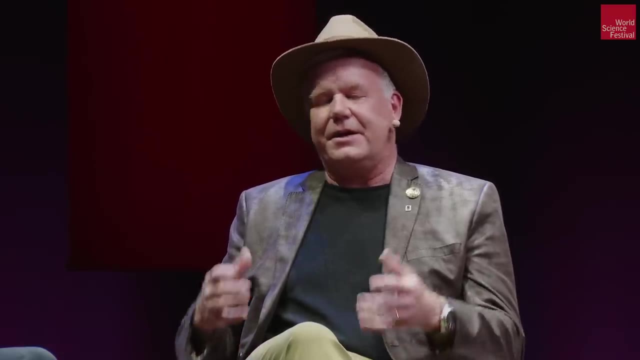 And on the first day there, we arrived the day before. after this just two day, you know lorry journey And we get there and I am so excited I cannot sleep. I get up at four in the morning, I'm the only one up. except there's a light at this, this tea tent that they have. 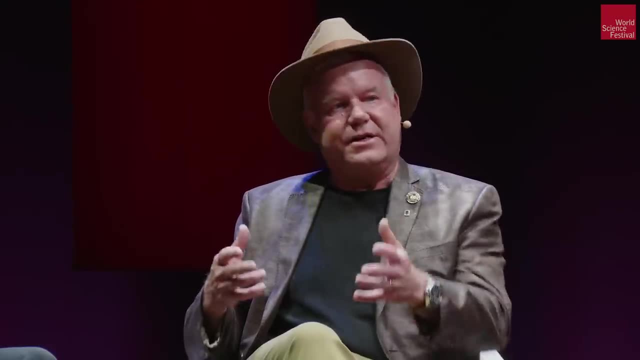 And I walked over there and there I met John Kimmigich who was preparing to go out for the day, One of Richard's great fossil finders. He loved it. He looks at me and you know he sees this enthusiastic kid awake at 430 in the morning. 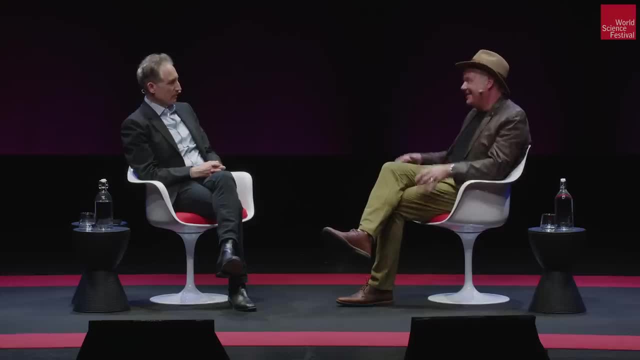 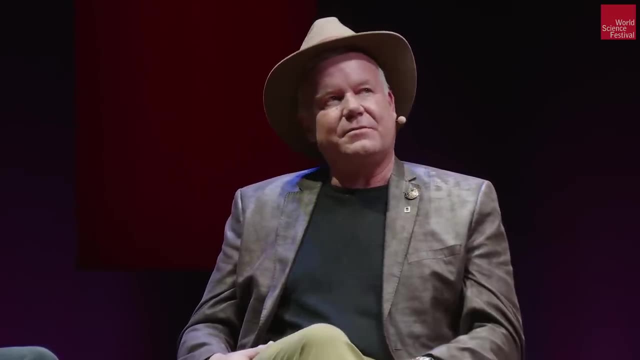 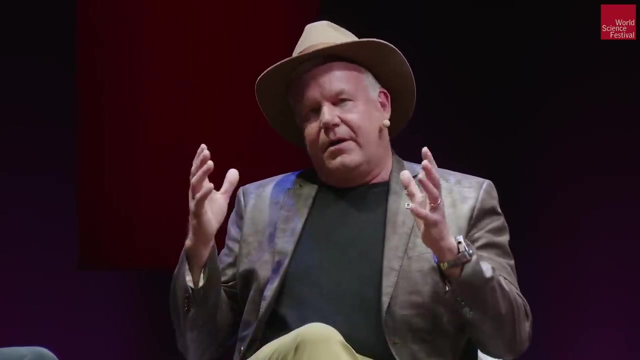 He said: you want to come with me. I'm like, yeah, I do Go out, And the next magical six or seven hours was just where he taught me to see this landscape and see the fossils and understand it, And I'm enthralled. 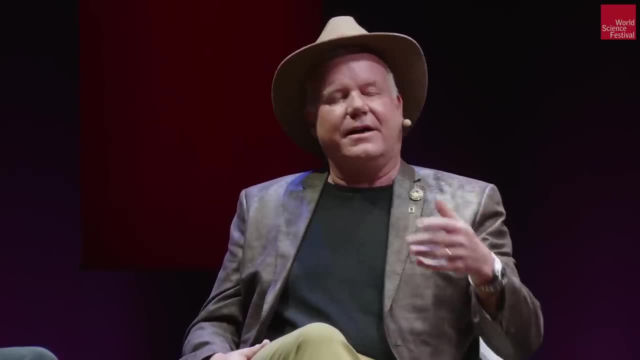 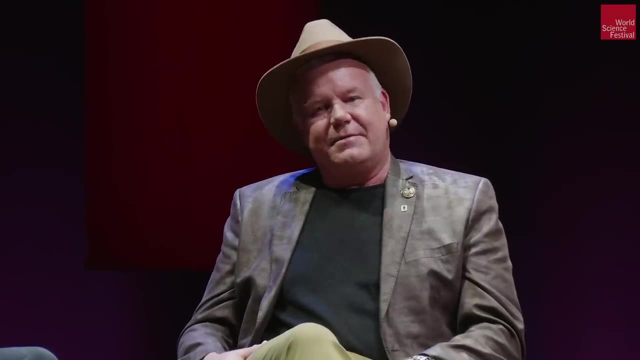 I have found this thing, And on the way back 11 o'clock, it gets hotter than here in Brisbane, by the way. So you know it's terrible, Terrible, And we're walking back 11 o'clock in the morning, 100 meters from the Land Rover. 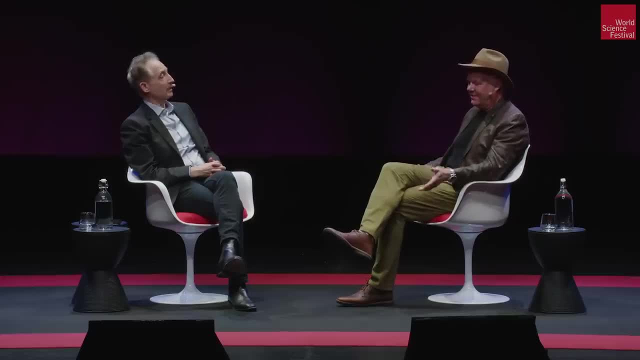 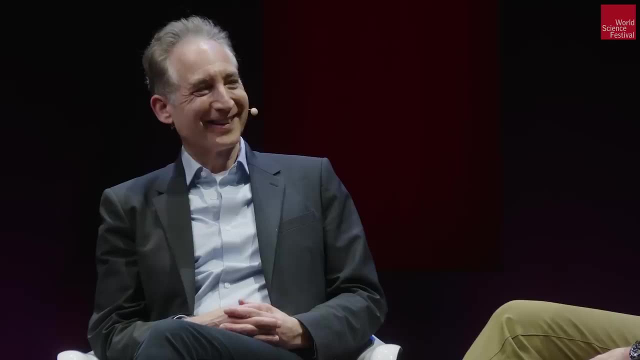 And I look down and there's a piece of a femur of a hominid on the ground. Pick it up. First day in Africa, First day on the fossil fields, Beat the odds. So that was one in 10 million, right. 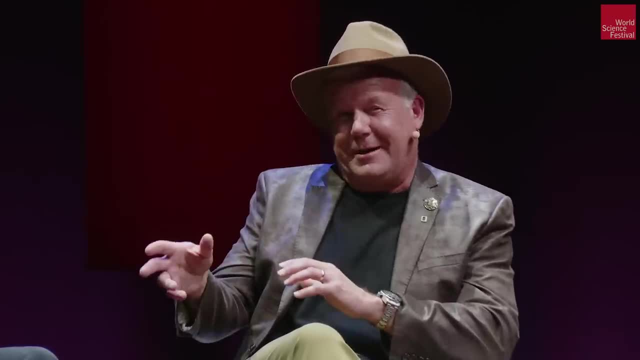 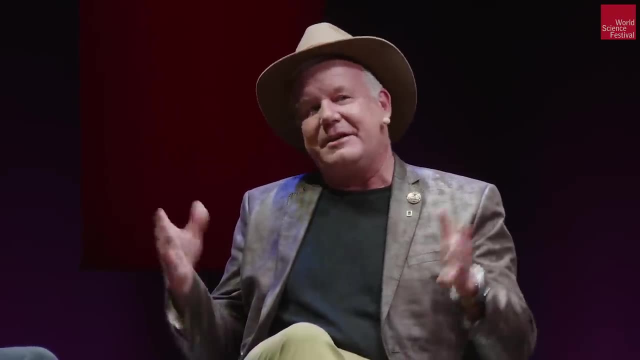 I don't know. I don't know if that number is true anymore. We'll talk about that later. Poetically, Poetically. it was one in 10 million Man. I was hooked. Yeah, You couldn't have dragged me out of Africa. 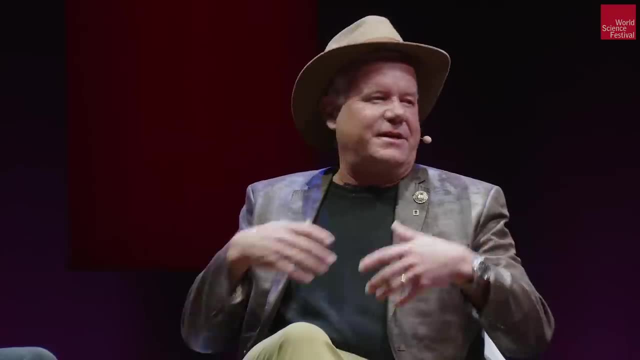 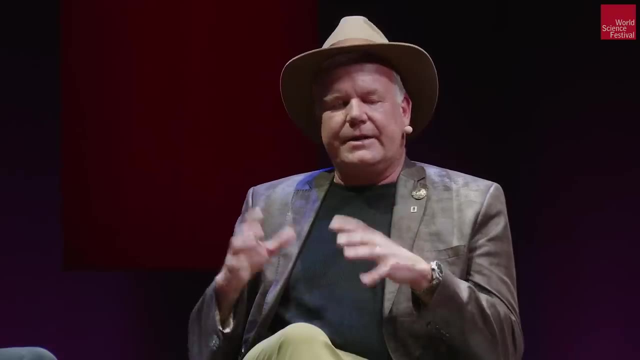 Ended up, I had applied to PhDs- That's the working degree in this field, as you know- And I, all over the world, got into most of the places that I was waiting on. I'd gone to Richard then and Don for advice because I said, you know, I want to be a fossil finder. 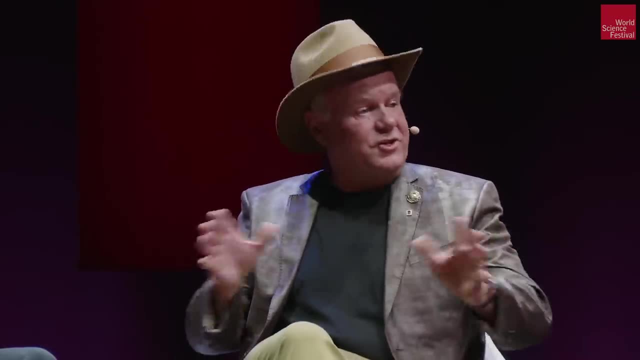 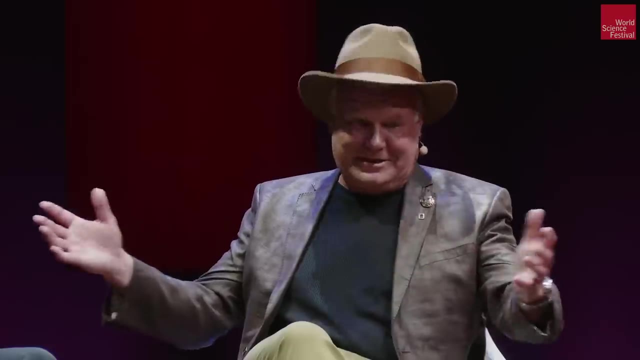 And they said: you're not working in East Africa. They said that to me just like that, Meaning No place for a young American guy in that landscape. They were too young, They were too violent, It was all you know, partitioned out. 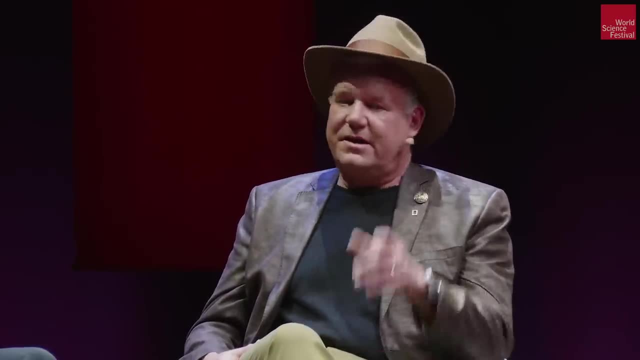 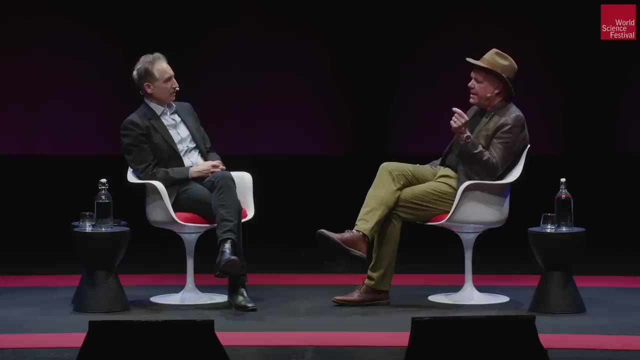 Partitioned out And both of them gave me the same advice. They said: go to South Africa. This was you got to remember the context of this. This is late 1989. They just announced that Mandela was going to be released in February of 1990.. 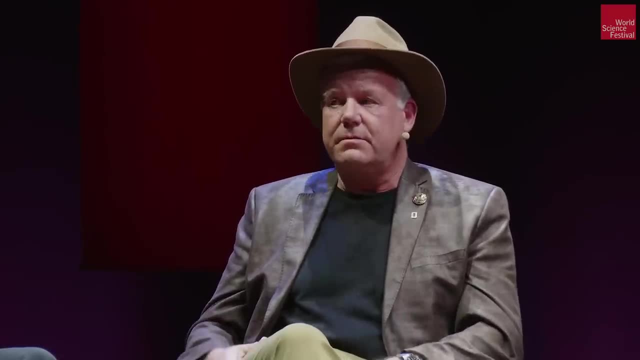 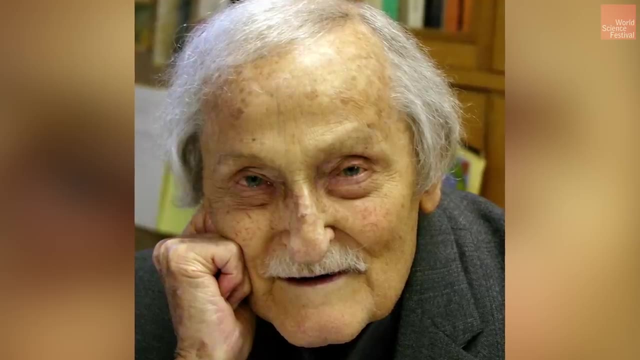 And they said: you know, the landscapes may be changing. They heard that a fellow named Philip Tobias, one of the great professors of this field, had a vault full of fossils that had been discovered over the last, you know, 30,, 40 years. 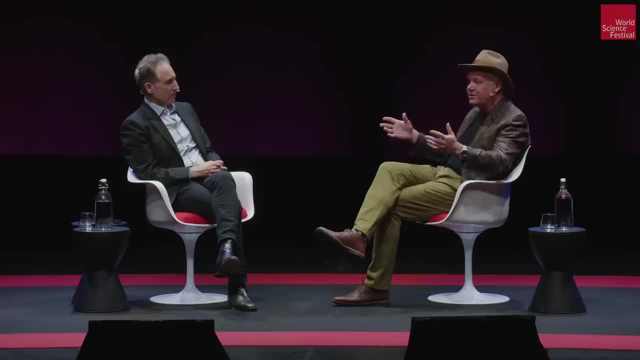 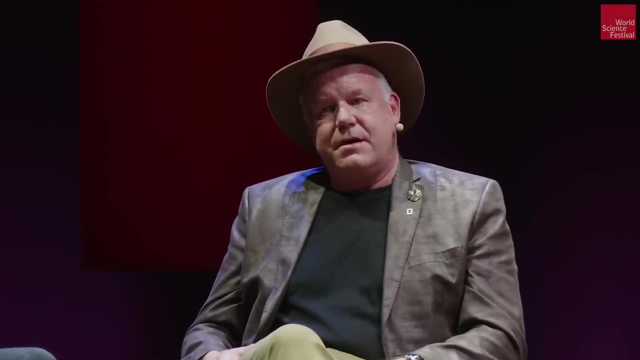 but hadn't been described, really because of the apartheid government's repression. So it's a vault in South Africa. In South Africa, The University of Witwatersrand, And I had applied there And so I called from a ticky but hadn't heard from them. 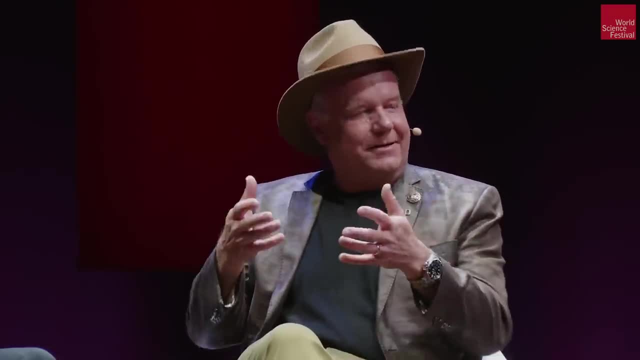 So I called from a ticky box. For those of you who don't know what that is, it's a. it was a pay phone. You put the little you know shillings in and you know he answers on the other side with. 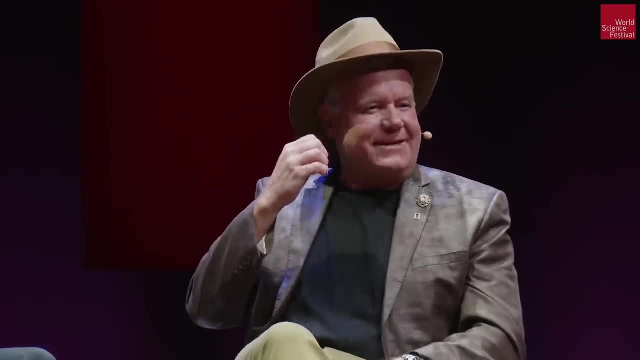 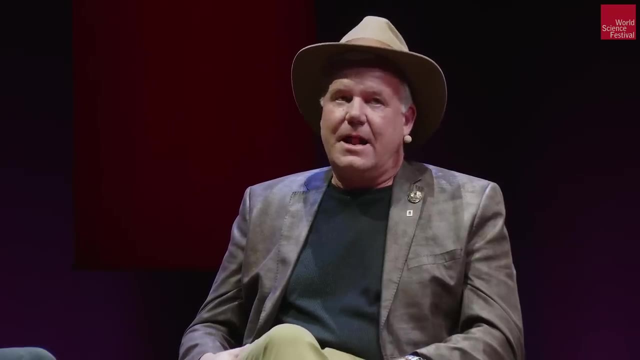 oh, dear boy, you know when are you arriving? That was my acceptance letter to the University of Witwatersrand, And so that's where I went, And it was a crazy time. You can imagine 1990 there, as Mandela was released and places blowing up. 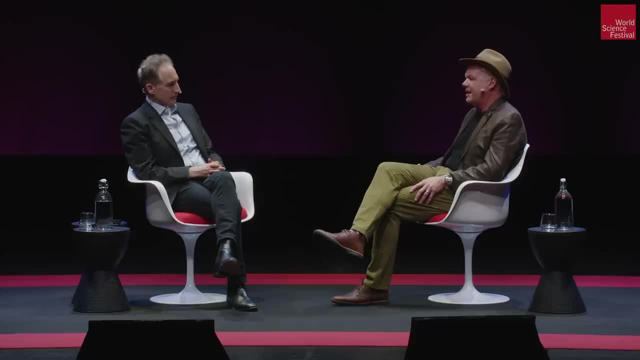 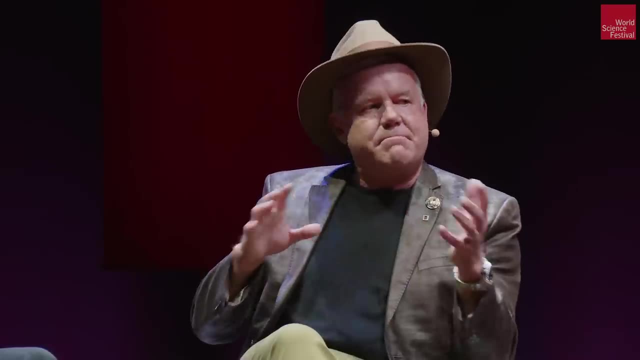 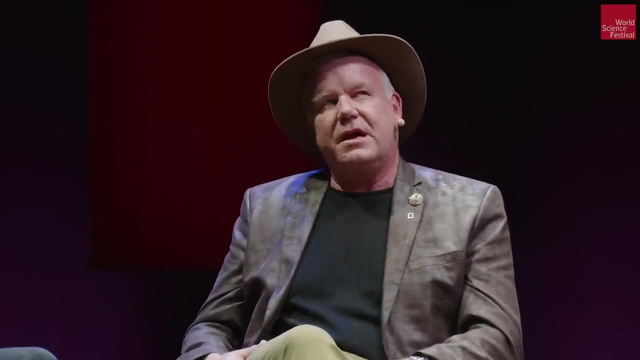 But I threw myself into walking the high felt of that area And as I was coming out of this East African mentality of one in 10 million, Yeah, There hadn't been a hominid discovery at a new site in sub-equatorial Africa since 1947, 48.. 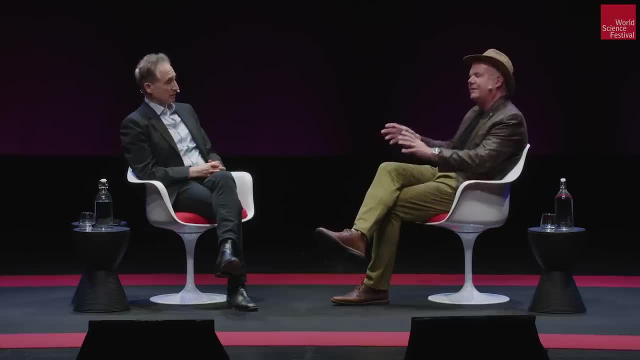 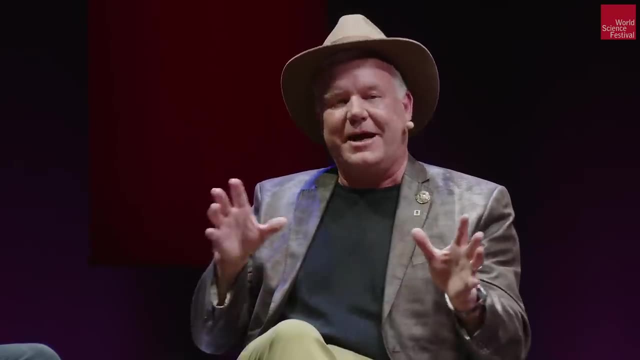 Nothing, Nothing, Nothing. on this side There's a lot, you know, apartheid government, Yeah Right, A little thing like that. Right It said. you know they didn't particularly like the idea of people searching for the idea of the commonality of all humankind. 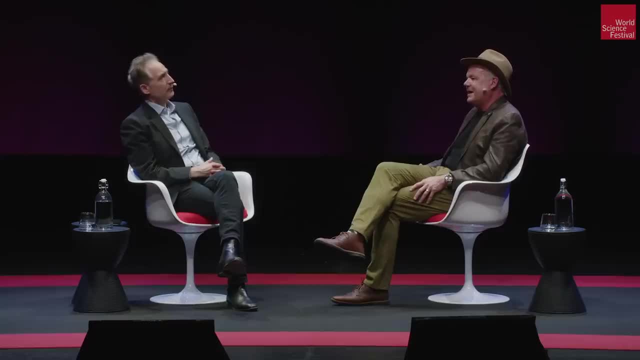 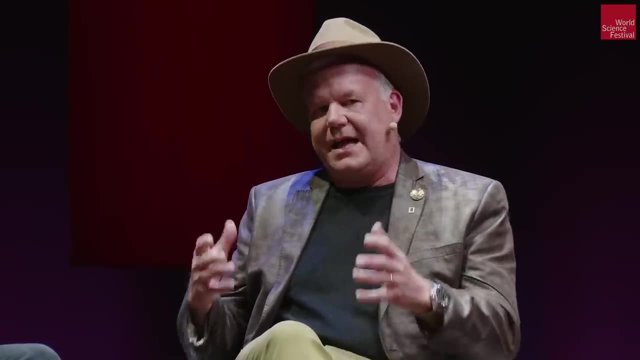 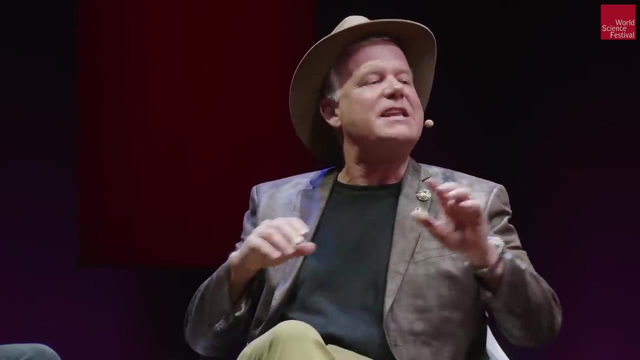 And those sort of. the subject wasn't particularly popular, But I was looking for a site that had a lot of bones and found one, A giant one called Gladys Vale. So I was given a job- by the way, way out of my league- as a table doctor teaching anatomy. 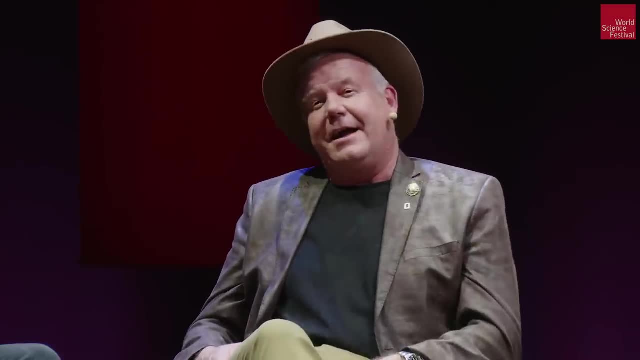 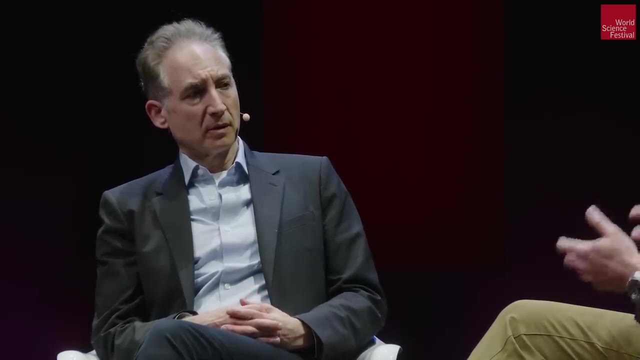 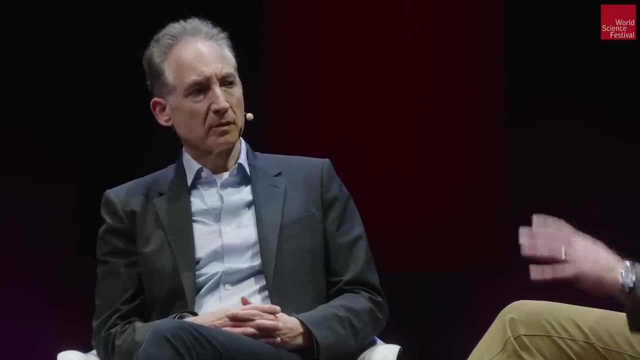 I never taught anatomy in my life- life, but i read well and you're still a doctoral student now. yeah, yeah, a doctoral student and the. and then i was teaching this bsc course in an honors course in science which i was teaching the human origins component of. you can all tell how highly qualified i was, for this is the first. 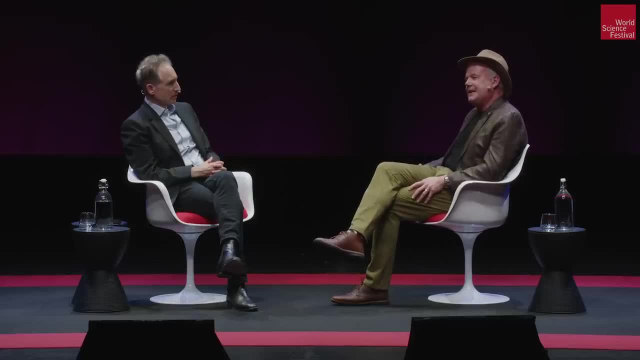 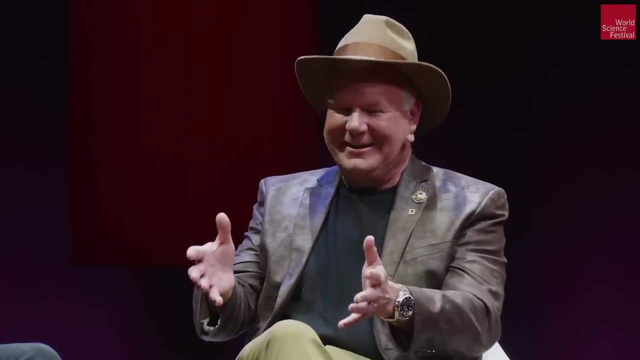 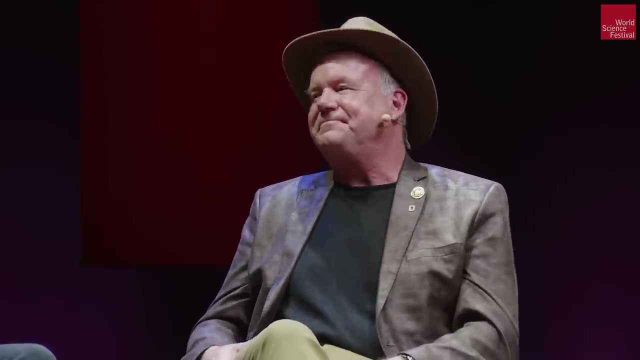 courses i'd ever taught in in that and um and i so i enlisted them, i drafted them as part of the course, to come out and work for me at gladys vale, um, under the argument that that's how you learn. you know, it's practical, it's a form of slave labor, i know, but don't tell anyone. and 16 days. 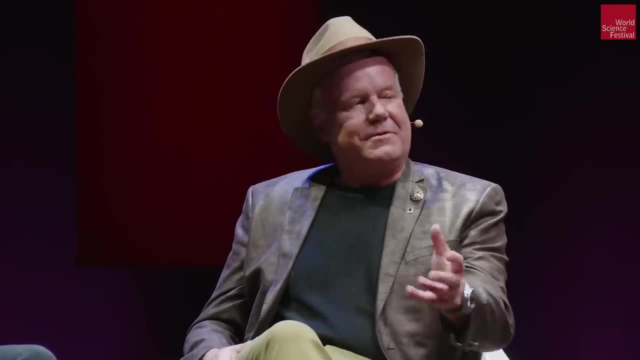 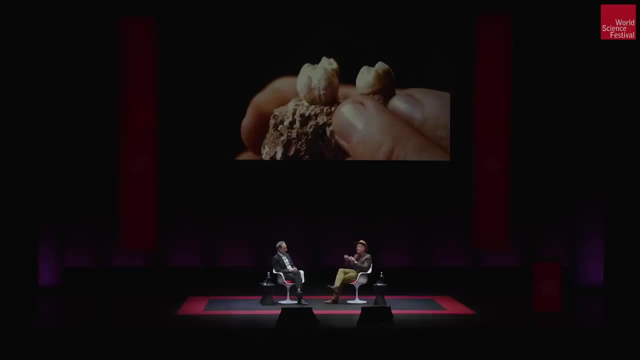 into this first expedition. michelle, erasmus, young woman on this course, picked up a rock and turned it over and handed me and said: is that a tooth? they're sticking out? this rock is a hominid. there, it is a hominid tooth. that's one on the. 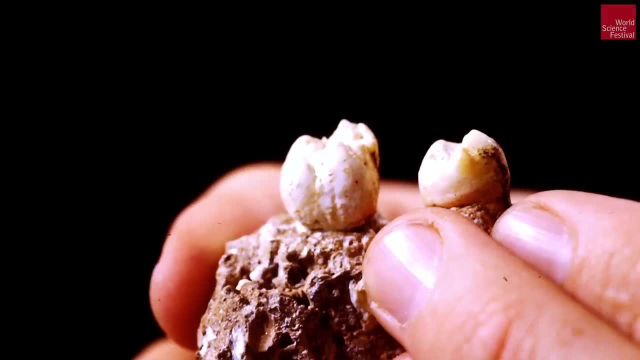 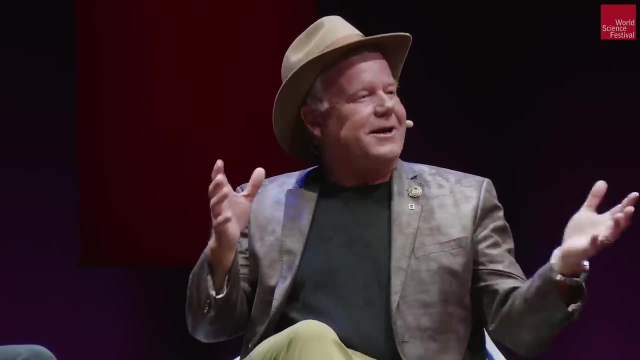 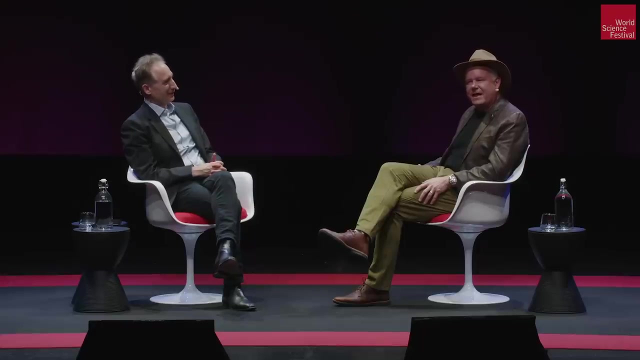 you left was the first one. the next morning the second one comes out. two teeth, you guys go really. you know, i can see the, you can hear the, you know the, the awe in the audience, right, two teeth. those two teeth got me a national geographic magazine. that is that, and you know. and then i threw myself into this site. 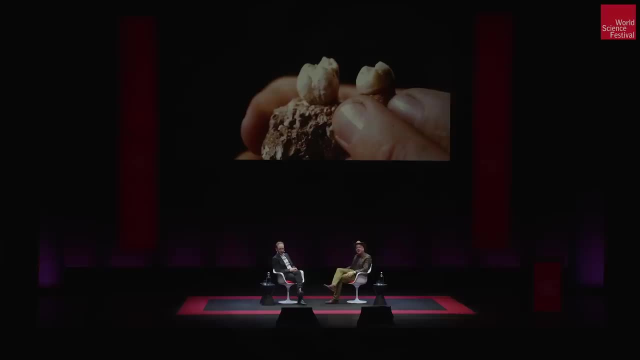 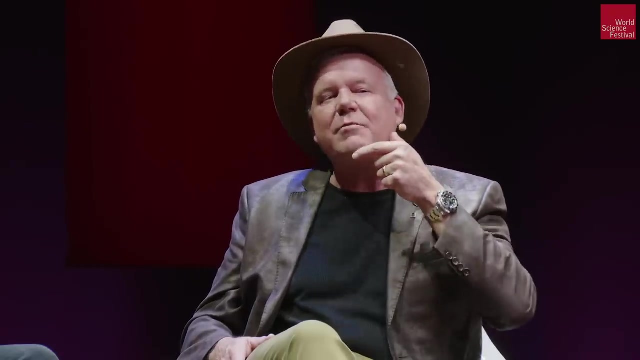 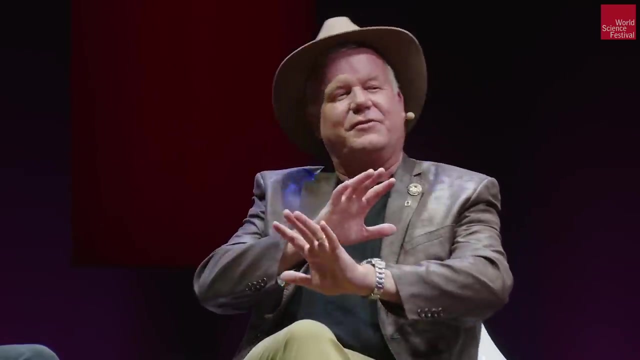 there i am throwing myself into this site. i knew that the next rock i would turn over would have that half of the mandible of a hominid in it, because i mean two teeth in 16 days, and i could dine on that at conferences for the rest of my life. 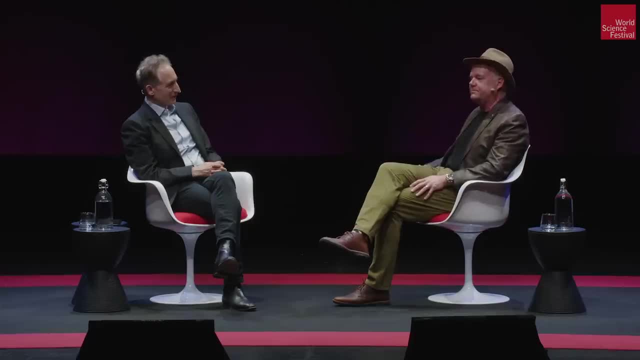 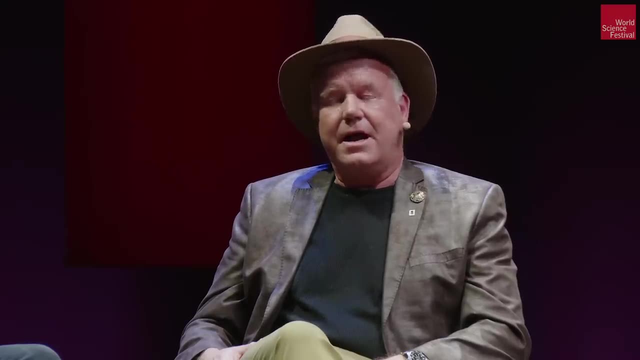 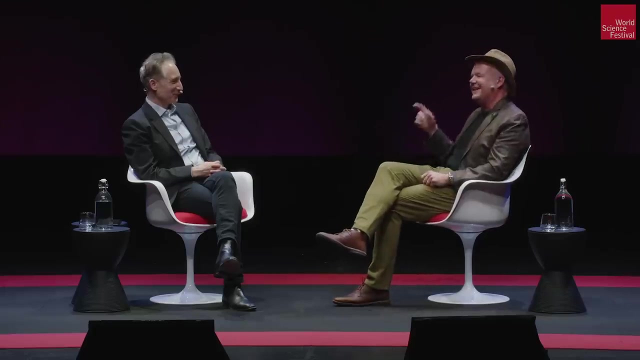 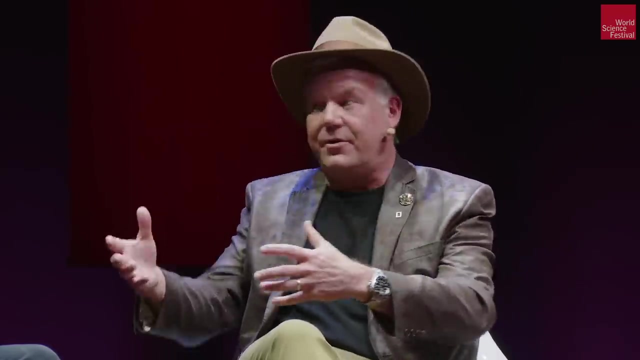 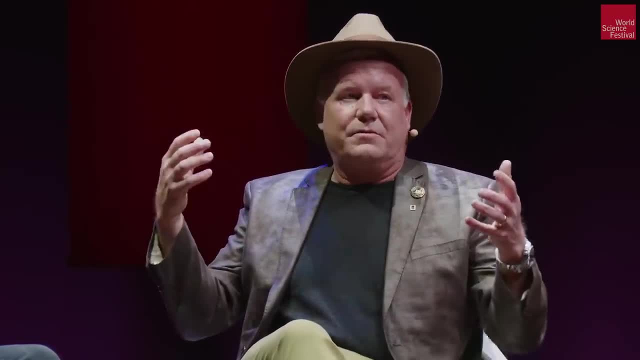 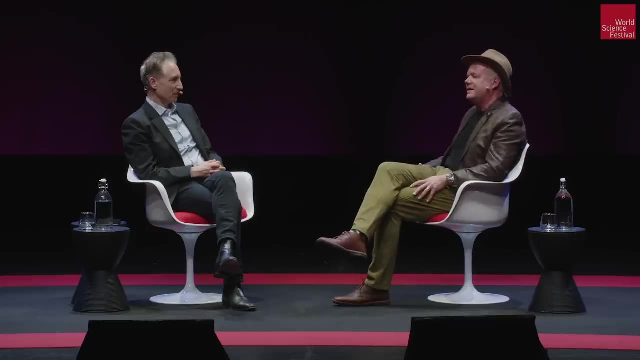 yeah, yeah, yeah, yeah, yeah, yeah. very proud of i was one of the first scientist- very controversial say- that early australopithecines, the most primitive of the eight men, so to speak, had long arms and short legs when we thought they were all human proportioned, which got me in a lot of trouble. 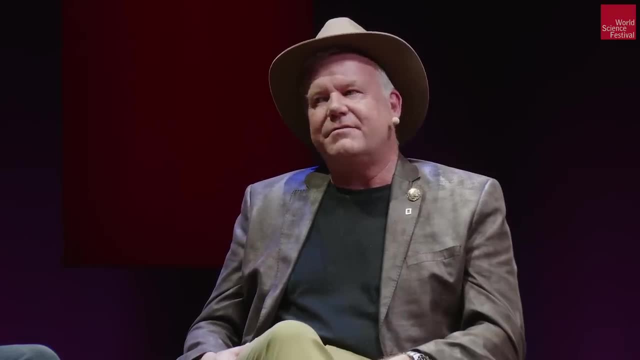 So, so, so, so, so so in the 1990s, but I didn't have that discovery. And by the end of the 1990s, just on the verge of the 21st century, I'd risen to this position. 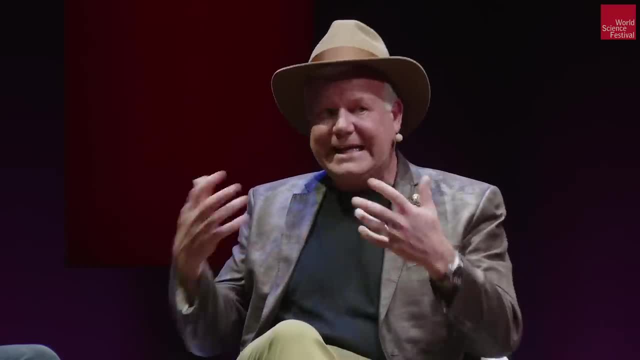 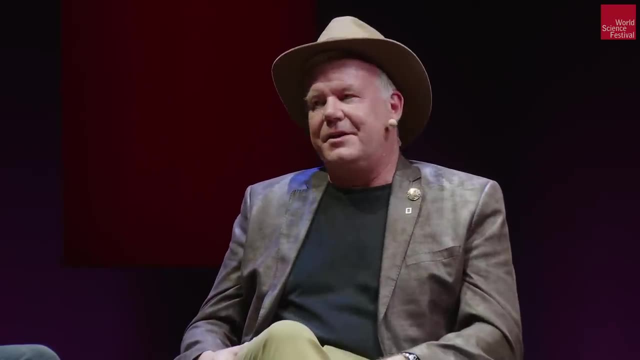 I took over Philip Tobias's chair. he'd retired. I was a kid, though, And you know I began to hear at these international conferences. here I am in charge of all of this now. you know I've never seen someone go so far on two teeth. 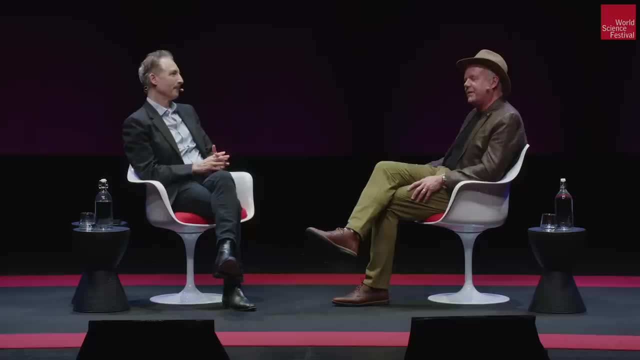 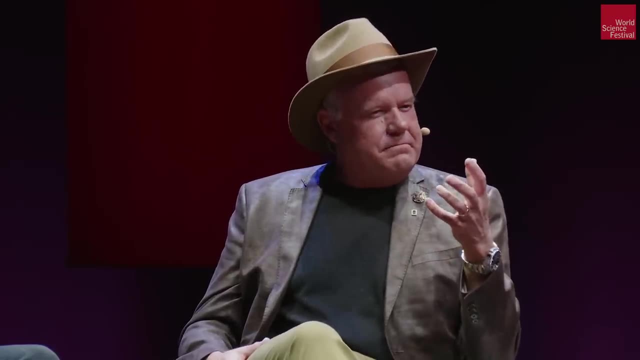 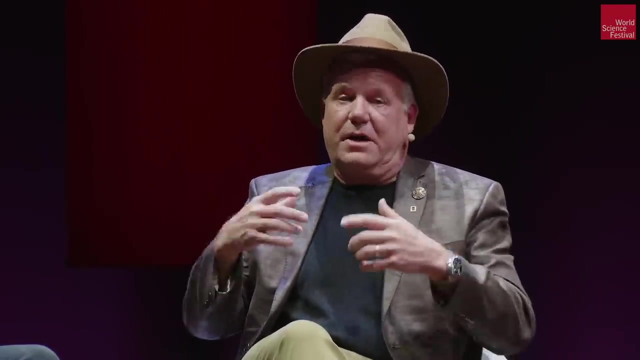 And you know, while I was naive, I wasn't naive enough to know that was not a compliment, That was a sort of you know, this field was possessive and it was about a mythology built around the discoverers. You almost had to be touched by God. 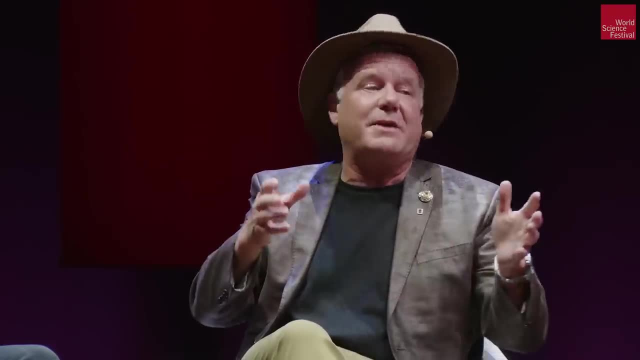 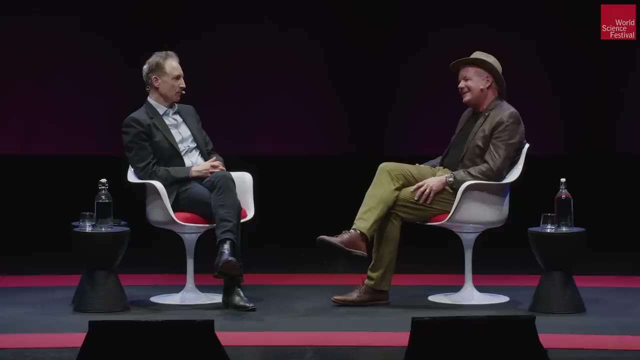 if that's not too much to discover these things. And then it began. you know, not just these things, but good ones. You know they started putting a level on it And I went through the worst years of my life in the early 21st century. 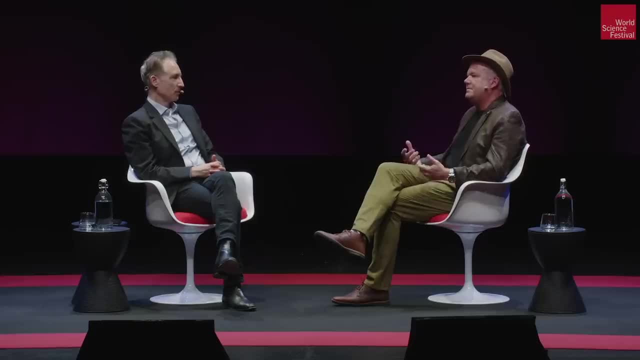 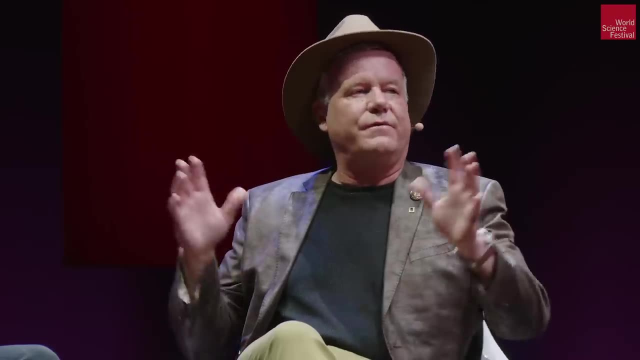 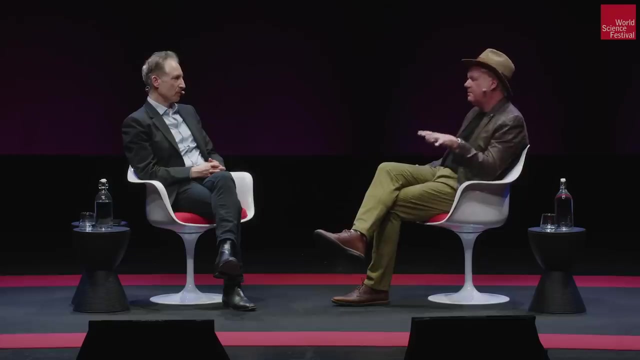 It was terrible Because I was becoming the poster child for the idea that the age of exploration was dead, That there were no new fossil fields to discover. There was even paper published in 2001 by the biggest fossil finder of that period. You know who I'm talking about. 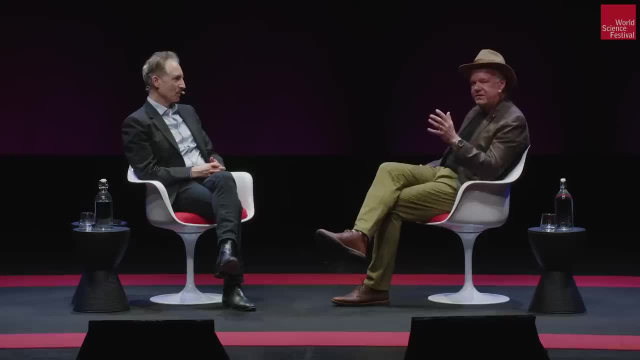 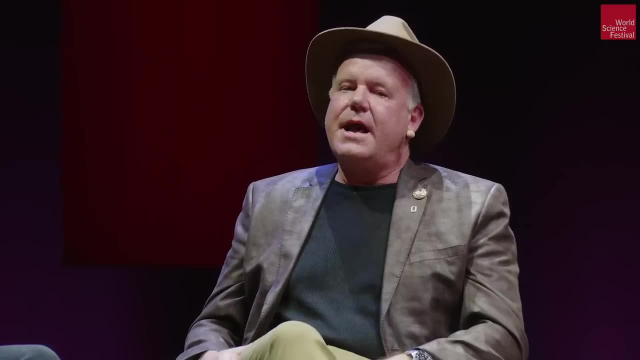 Who said there will not be any new discoveries that change the way we understand human evolution, That there will be no new fossil fields found And that we should stop training people to be young paleoanthropologists, because it is insanity to have a field. 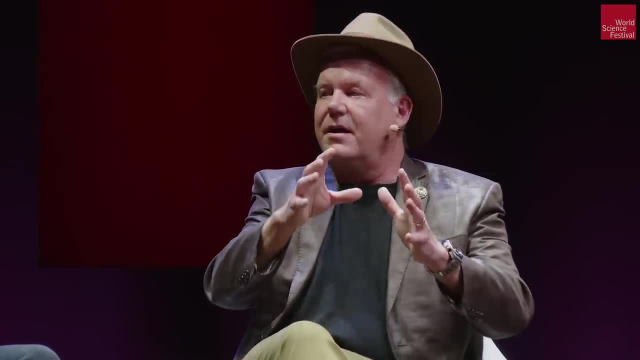 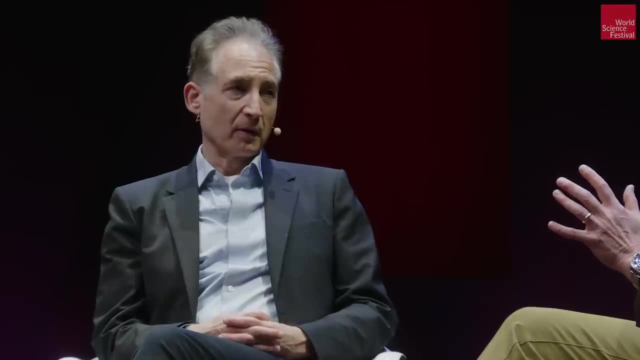 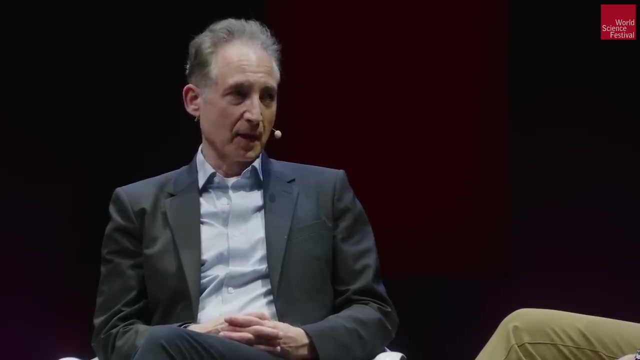 where there are more people studying this than there are objects that they study, That killed funding for exploration. I mean, killed it dead, And that's a fairly common kind of rhythm. right In the late 1890s there was a statement in physics: 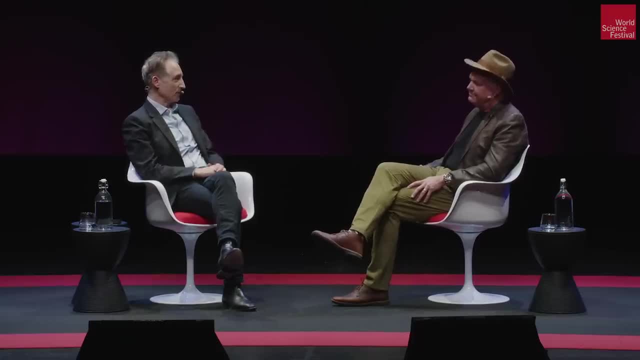 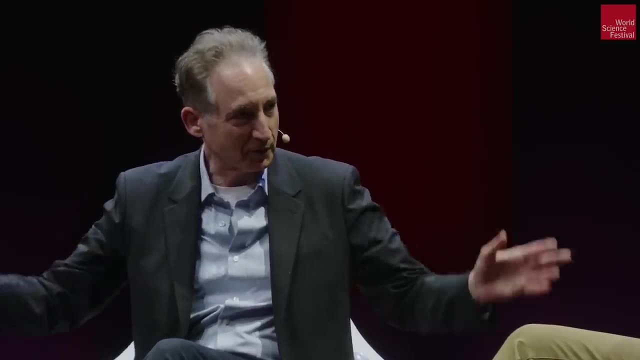 that all the fundamental laws had been discovered and all that remains is to determine this or that constant of nature to the sixth decimal place. And then we have special relativity, general relativity and quantum mechanics. So I suspect you did not take that as the final word. 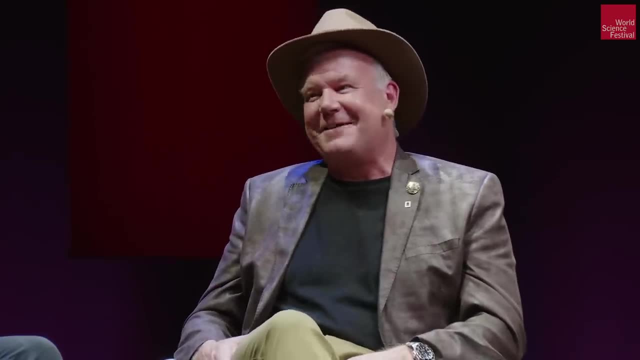 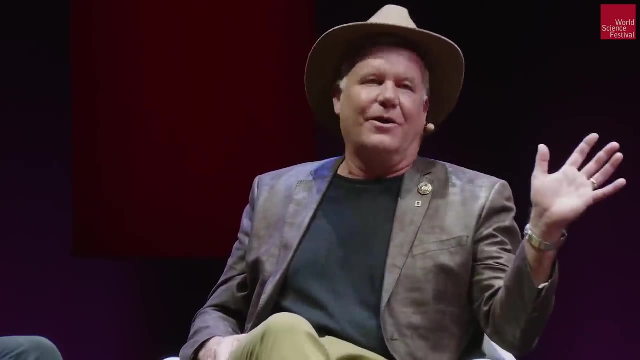 on this idea. It hurt. It hurt my wallet, It hurt my ability to do exploration. but you're right. I mean, I knew the history of dinosaur paleontology. Same thing, Early 19th century. we have it all. 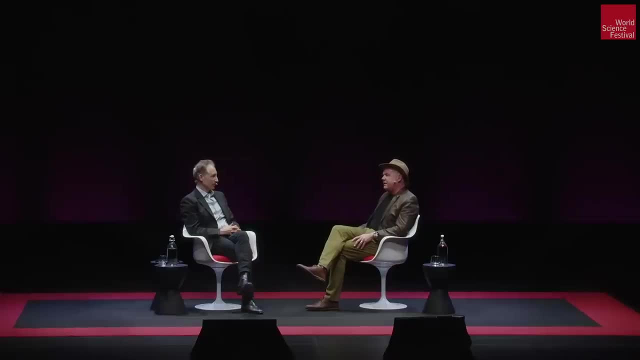 Of course we didn't, But it was tough. I'll tell you how tough it was that my university, convinced by the external forces of these big discoverers of fossils, said: you know what? We're going to close your exploration unit. 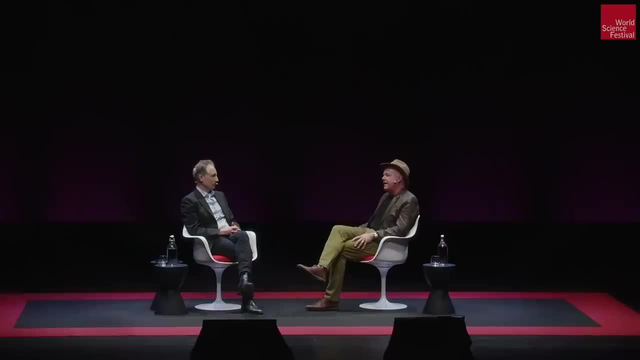 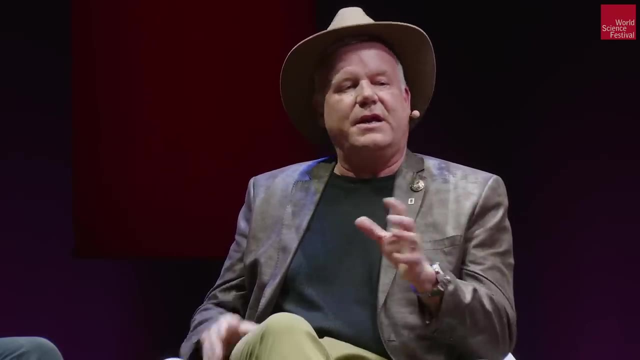 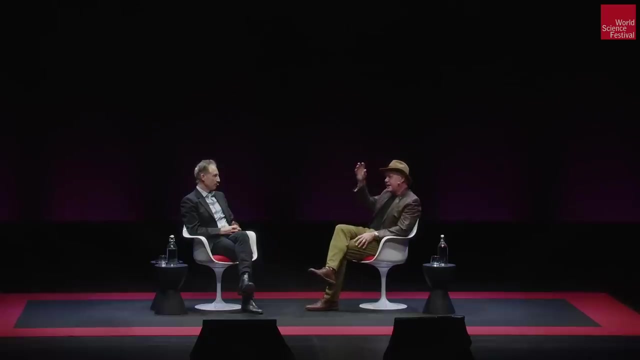 This is now 2006,, 2007.. And we're going to hire, under the convincing of these outside forces of the university, a young person to come in and revolutionize it, Because the idea was what was getting on the covers of nature and science were the sort of imaging. 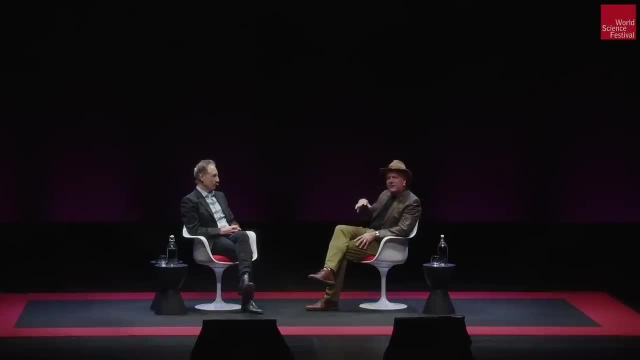 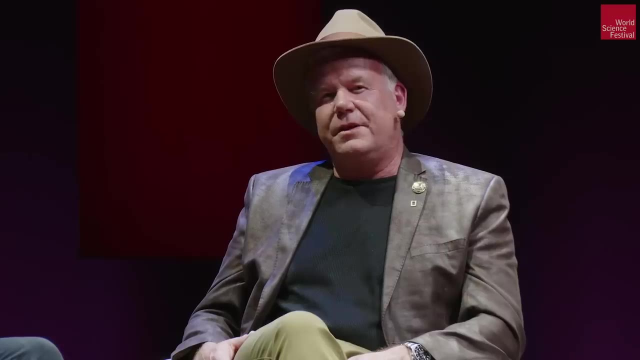 the sort of new technology, That's it, The technologies that were being applied to fossils, So the existing ones. just analyzing them, We were never going to find more. And I found myself in this really weird thing. I hope none of you ever do in your entire lives. 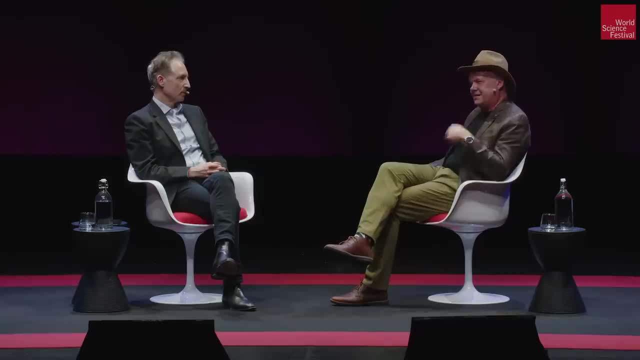 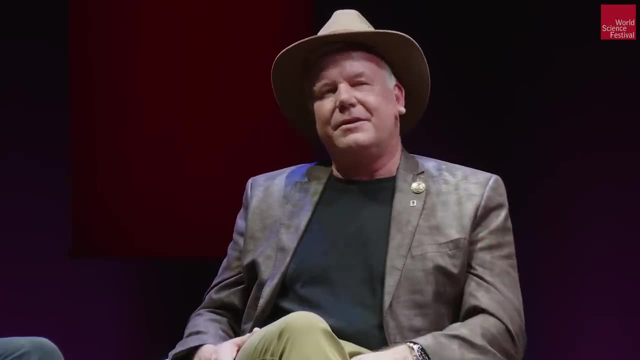 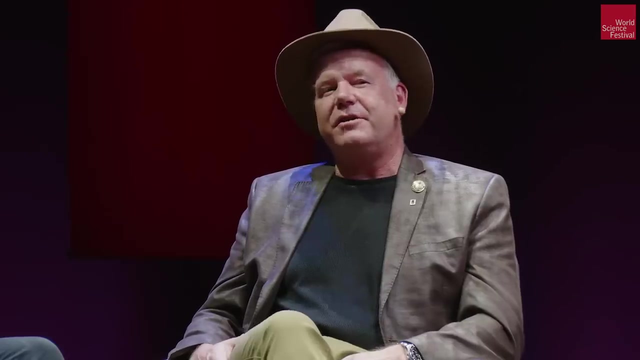 of actually sitting on a committee to replace myself. I was like 40 years old, You know 40, a little older than that. Were you resigned to this being the end of this career channel, Or I was soul searching? I was soul searching. 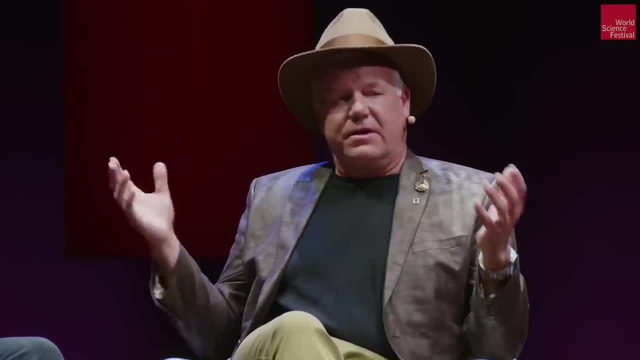 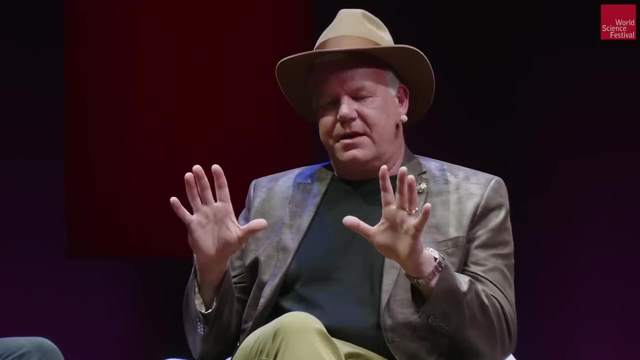 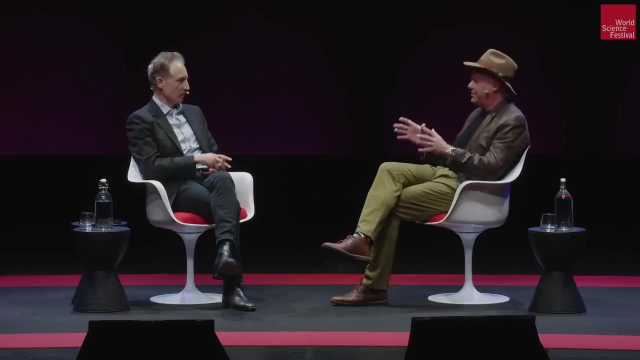 And I ended up. I remember the day this all happened, the next part of this story. I was sitting at home on my computer And I was doing what I guess all people of our generation do When you absolutely have no idea what your future direction is. 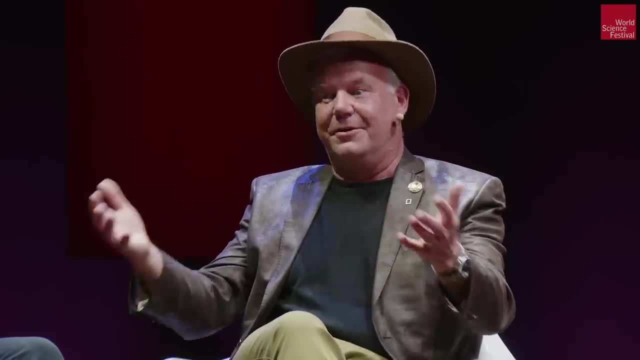 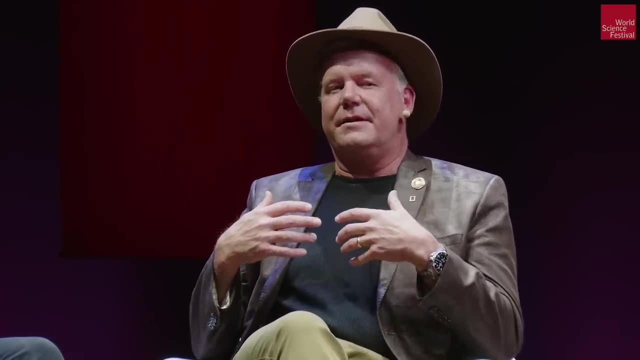 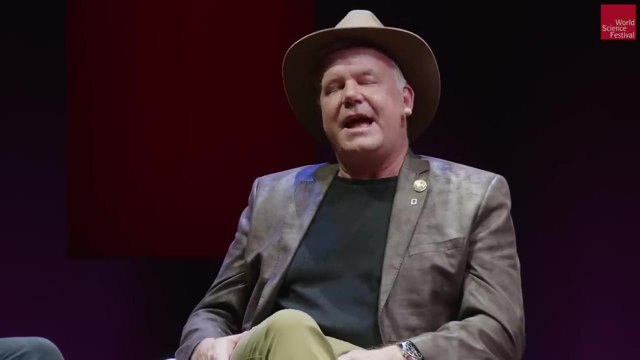 I was Googling my future, You know, just trolling the internet, saying what is a guy who's dedicated became the poster boy of, Of failure in exploration? What am I going to do next? And at that moment I became the singular, last human being. 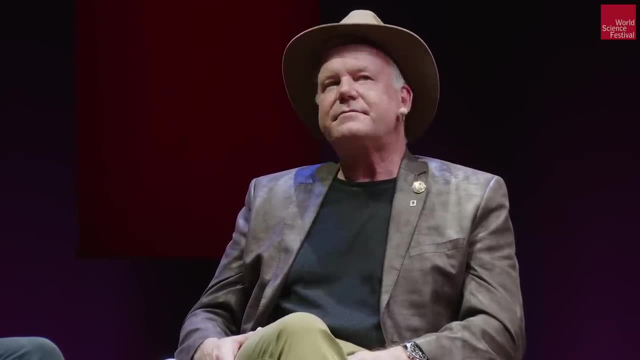 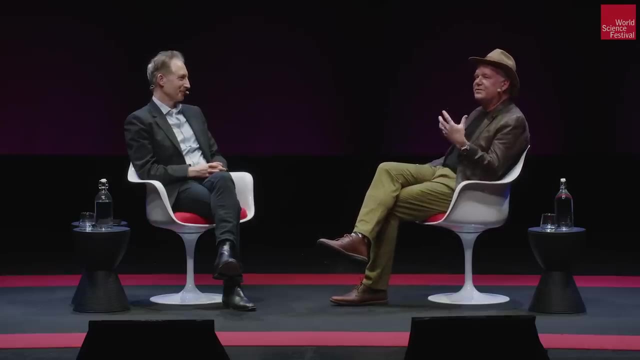 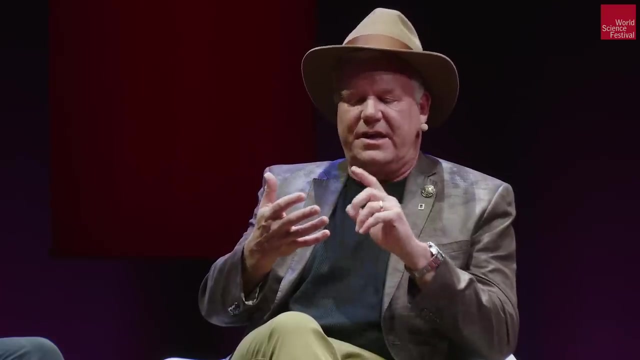 I am convinced on Earth to discover Google Earth And I. the reason it is so stupid is I've been a pioneer, as you know, Brian, in the 90s, On trying to take technology, handheld GPS satellite images. 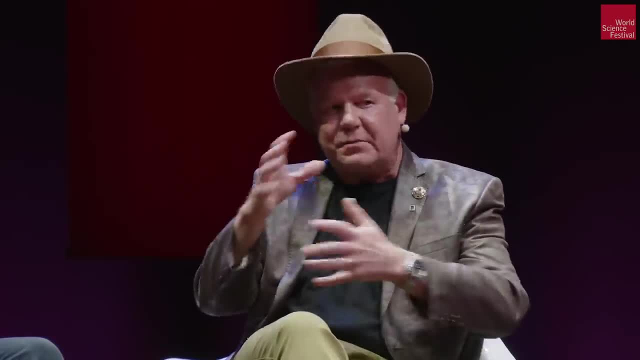 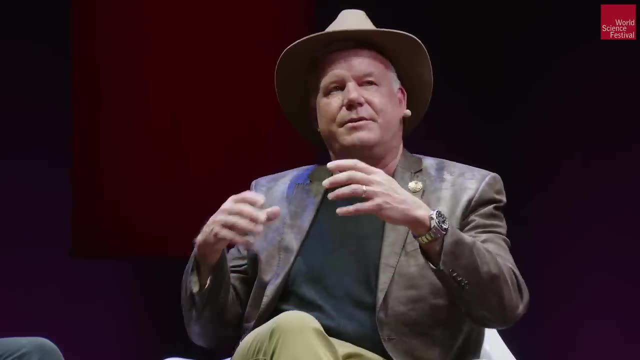 and combine them into a way To make Discoveries. I was convinced there was something there, But the satellite images cost $10,000 a sheet. The pixelation was terrible, The handheld GPS's were terrible And expensive And I had failed at that. 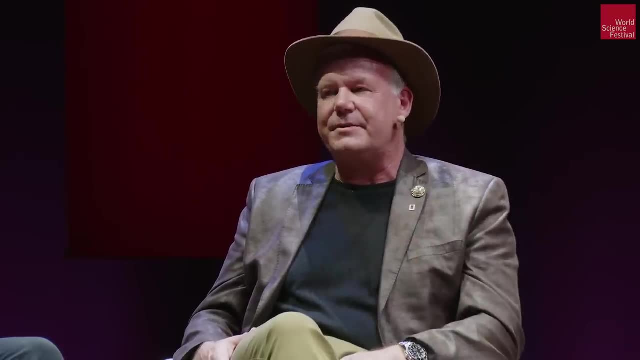 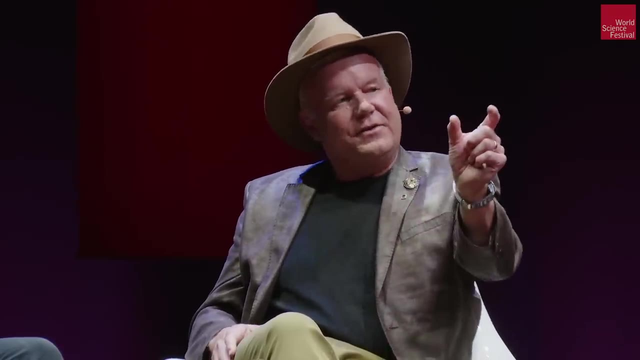 I had run a three year National Geographic funded expedition to do it And hadn't really done much at all. But then I'm sitting here looking at Google Earth. I notice that little white box up in the corner for GPS coordinates And I had, like some of the most expensive. 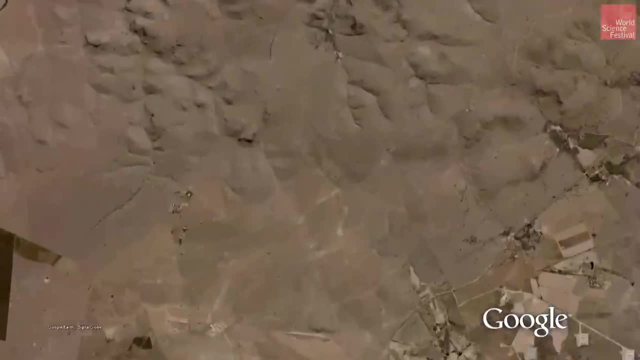 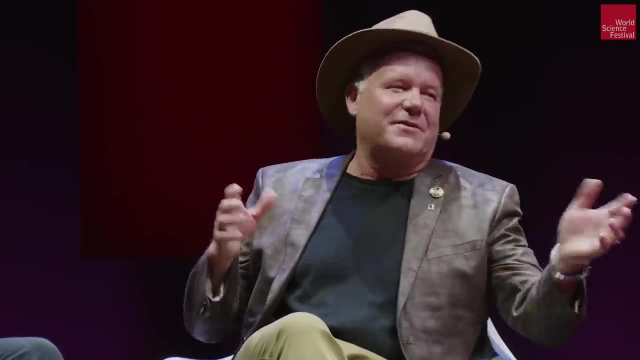 most easily obtained GPS coordinates ever And I put it in. and it does this right, It does a zoom into thing, And I started. I of course looked. if I was, you know, I looked at my house first. I'll admit that. 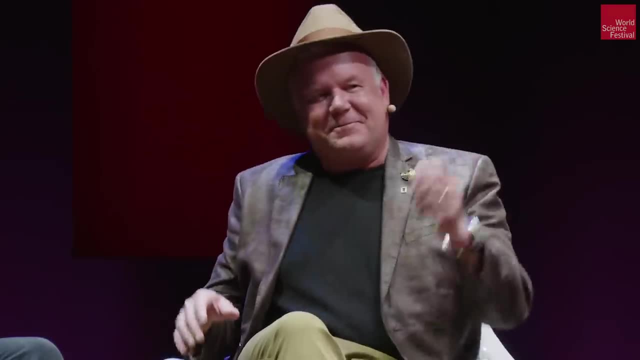 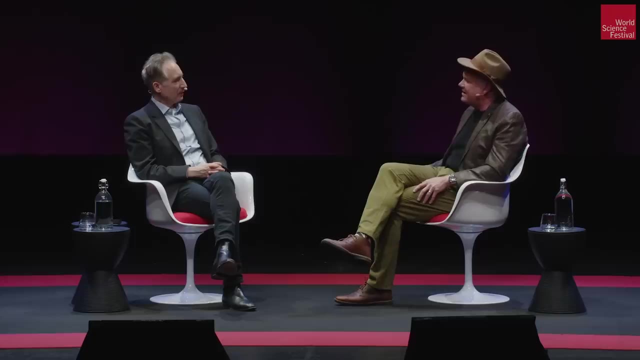 See if you're naked by the pool. you know that kind of thing And I wasn't. And then I applied it to these sites And it didn't land on the sites that I'd mapped in the 90s, And it didn't take me long to Google why it didn't. Because the US government had owned the satellites At that time And put deliberate error into them so they couldn't use for terrorism and that sort of thing, And so that, with the sort of error that was in the handheld GPS, has created a compounding error. 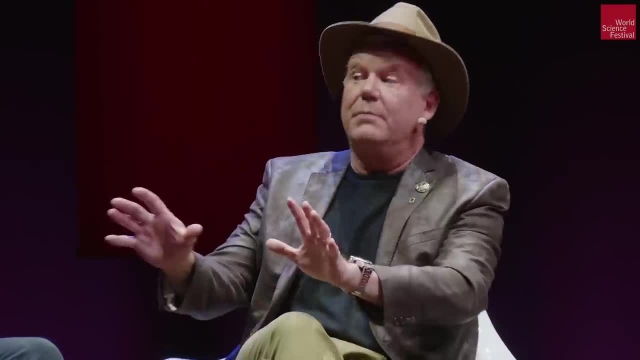 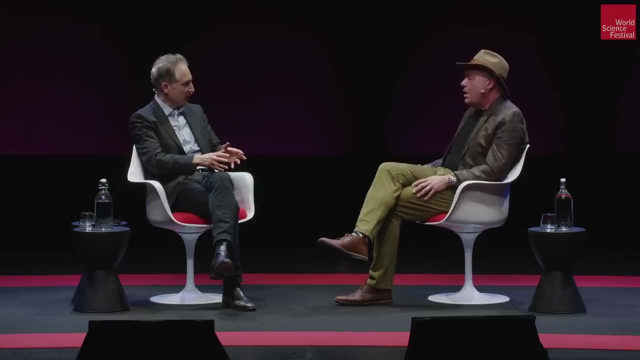 I was devastated. I mean, I'd spent, I'd wasted three years of my life, I'd published some of that data Wasted in the sense that you thought you were looking in one area when it was actually displaced from where it actually was. 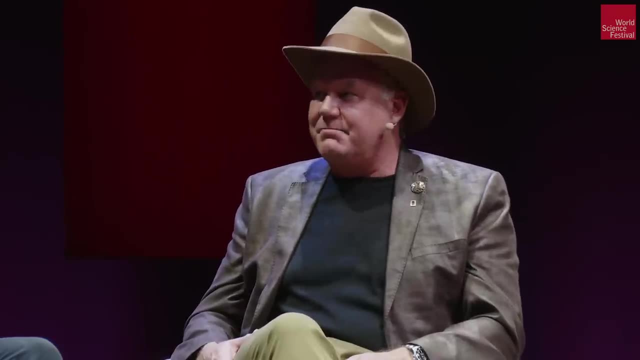 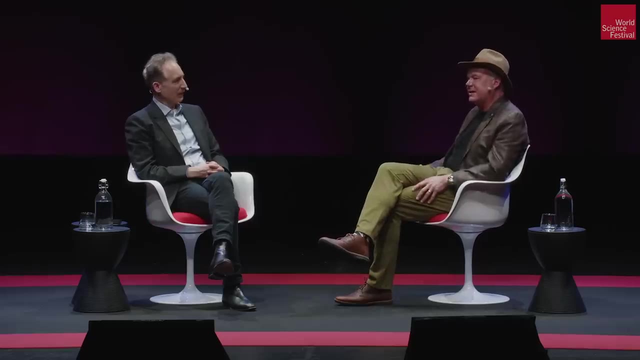 I thought I was mapping things. And I wasn't mapping things, I was mapping nonsense And that's not good. It's not great for your scientific reputation to be publishing that kind of nonsense. But I quickly learned that I could see the sites on Google. 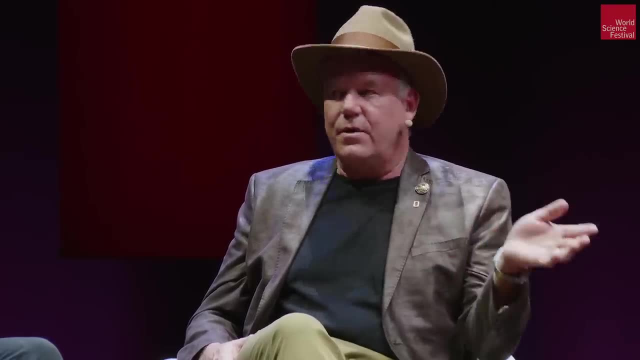 Earth that I intended to And I started moving those dots from the wrong place to the right place. You could see them through features in the landscape. Yeah, You'll see. like you'll see some right there, Like you see those trees. 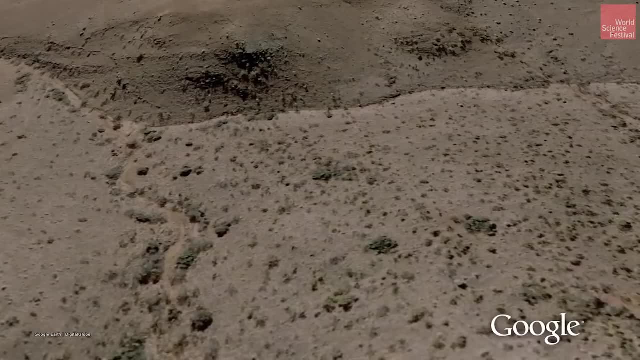 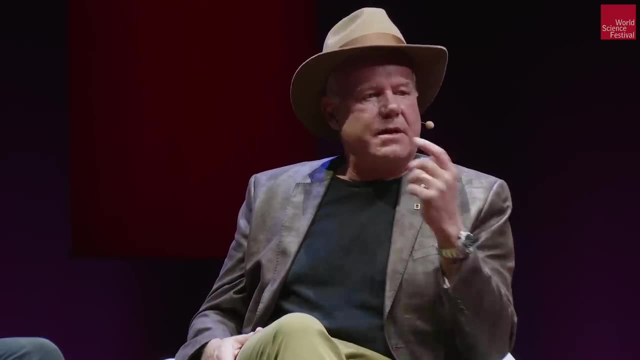 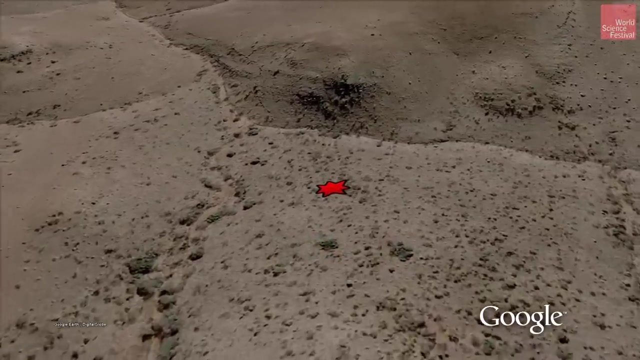 See those little clusters of trees. that's the green dots. Yeah, Those clusters of trees are marking cave sites and fossil sites. There were about 103 known at that point And I started looking and started saying, wow, If that's a cave site, then that looks like a cave site. 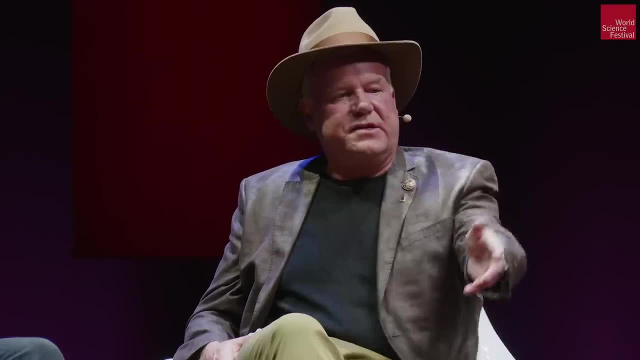 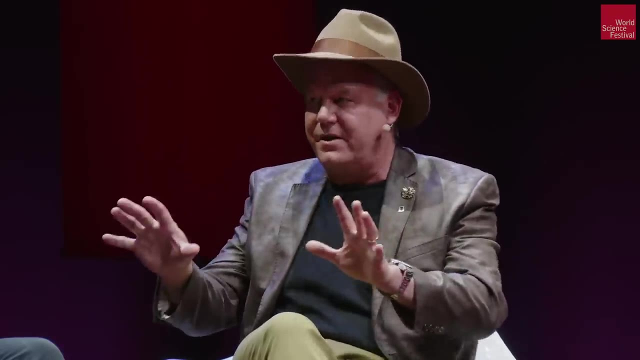 And so out. I went to ground, truth them Out, walking in this sort of environment, to see whether these were actually. I knew they couldn't. This was the most explored area on planet Earth for these things. There's no way they were. And as I started exploring on the very first day out, I created this target map, if you can imagine, Printed it out. It's far away from Glacier. It's as far away from Gladysville as I could get, Because I had 17 years of failure in that spot. I knew it better than anyone else. I went all the way, 30 kilometers away, to the edge of these dolomitic limestones- The greatest potential for these- And on the first day found over 20 new sites. Went from 103 to 123, one day. 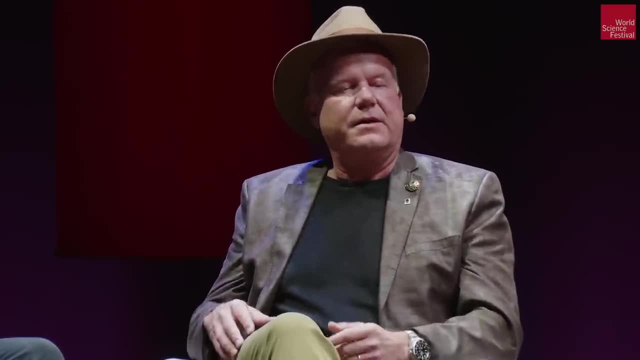 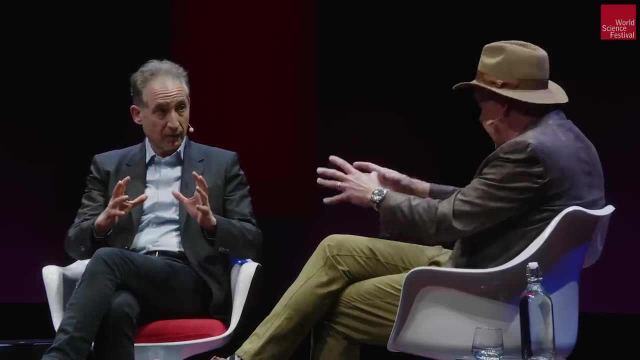 I was blown away. I mean, we'd missed it all right in front of us. And what they looked like were you know they were these clusters of trees By site. By site you mean new caves, Caves and some fossil sites. So there were only- let me put that in perspective- there were only 17 known fossil sites. I'd found four of them back in that 1990 expedition And then all of a sudden there are more of them And I started going out every day, over and over again. one after the other, one after the other, And suddenly, every day I was building this map: January, February, March, April, May, June, July. By then, I'd found over 750 new sites in the most explored area on planet Earth. 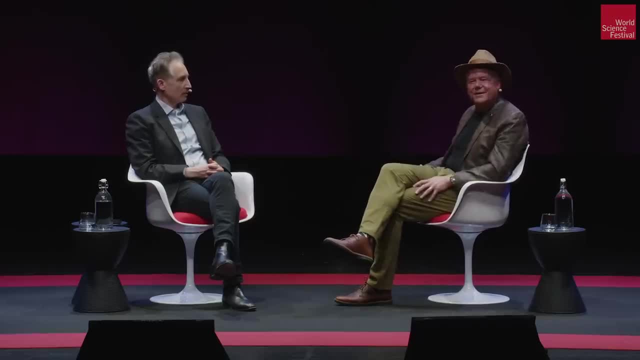 I was like, oh my God, this is my contribution, This is what I will leave the future, this almost unlimited potential of discovery. And was it mostly tree clumps as the operative way of finding them? Yeah, I'm sure we have an image of tree clumps. 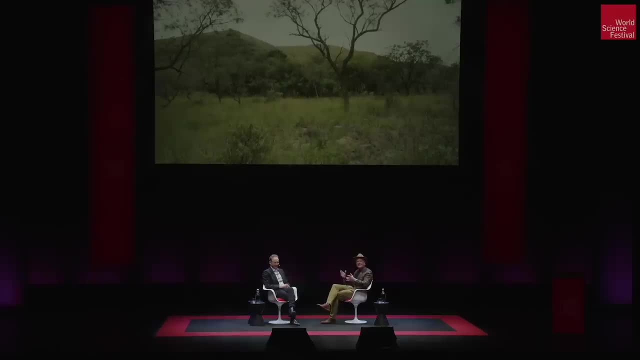 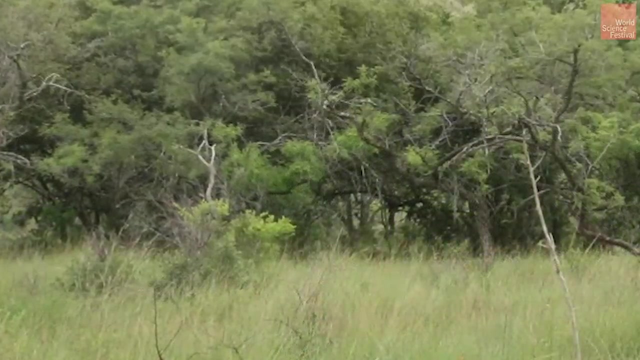 That's what they look like. Everyone's excited. I can hear the you know the awe in the audience. Look at it. But in that tree clump why? Wild olives, white stinkwoods clustered together. You could see them from space. 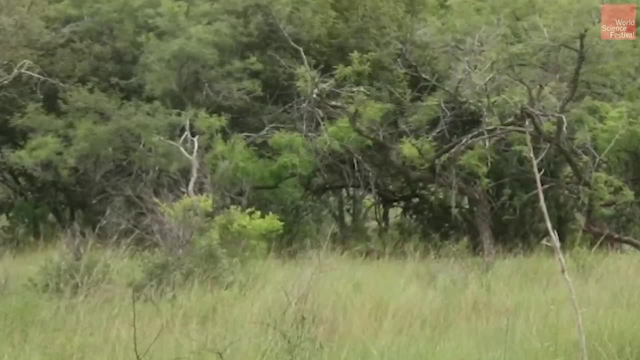 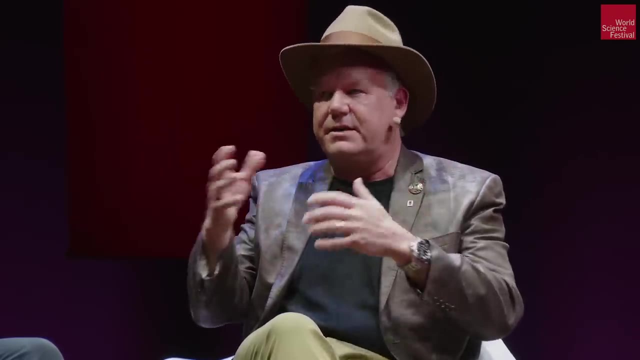 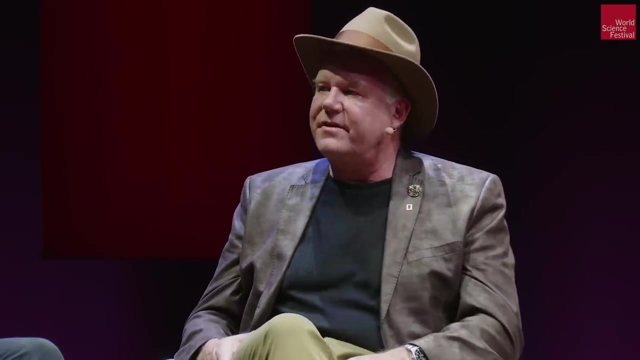 And in those are often depressions, holes in the ground, sometimes fossils that have been mined. often They were mining for lime in that area back in the, you know, late 1900s, early 20th century And eventually I'd moved right back into the area of Gladysville. 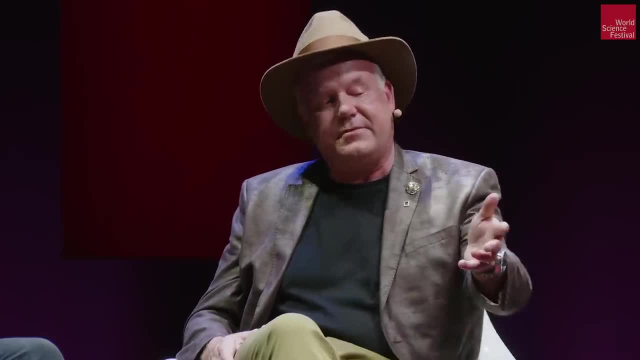 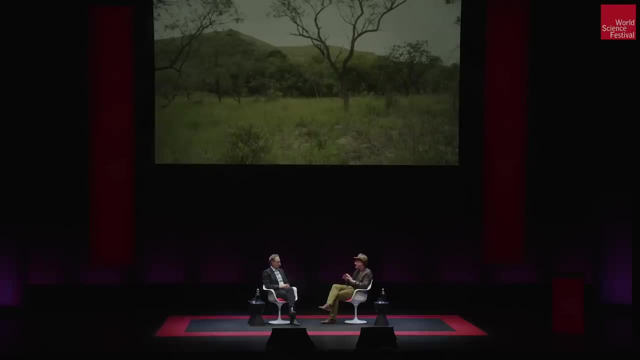 And I knew there was nothing there to find, But I'd gone. I'd gone to these tree clumps and walked up to actually this one And went to it first And the first rock I turned over had a fossil in it, which surprised me, because this thing 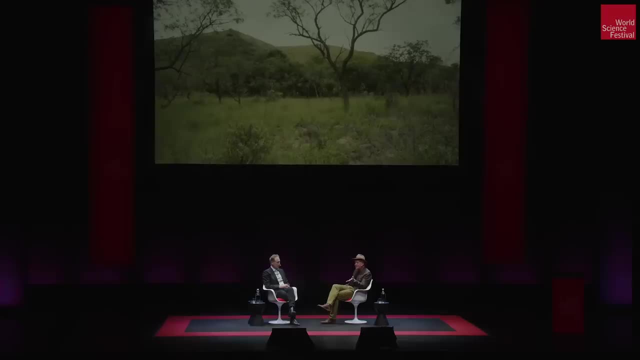 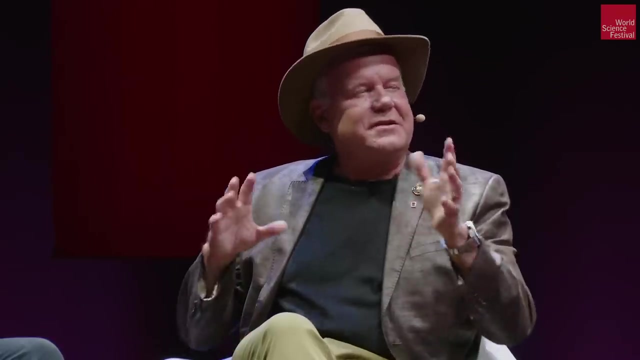 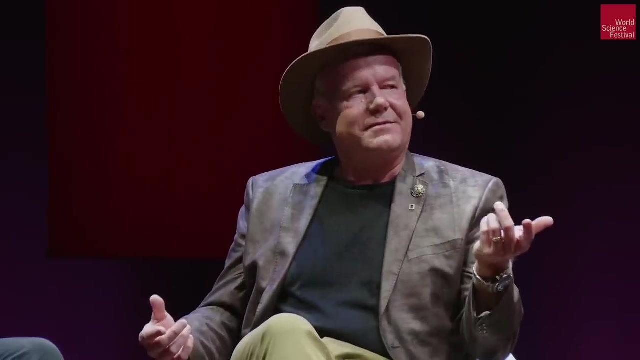 is like 800 meters from where I'd spent 17 years working And I'd missed these fossils. I felt like an idiot, But I was fossil hunting that day and cave hunting that day. So I just, you know, took the maps down and then went up in the thing and found 47 new. 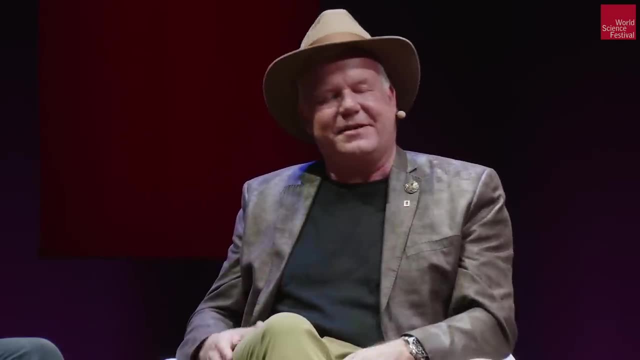 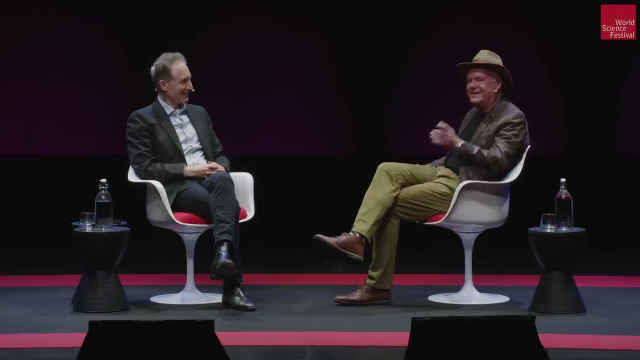 sites, And it was right next to the valley I'd been in for 17 years, unsuccessfully. It bugged me a little bit. Yeah, Yeah, I had that reaction too. A tragedy had occurred a couple of weeks before which I haven't told you about. 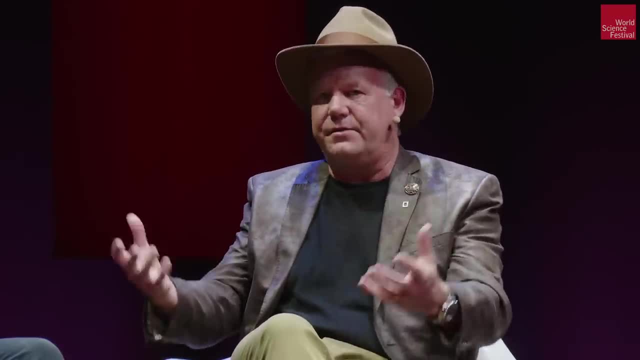 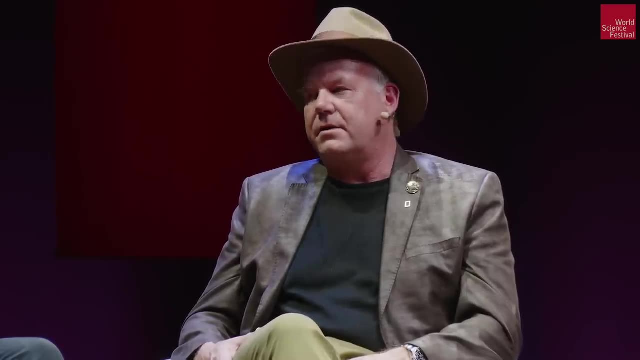 And that is that, the young man that was going to take over. we'd selected to bring in this new technology and stuff. he lived in the UK and was killed in a motorcycle accident, And we had already hired all the young postdocs, bought the equipment and stuff. 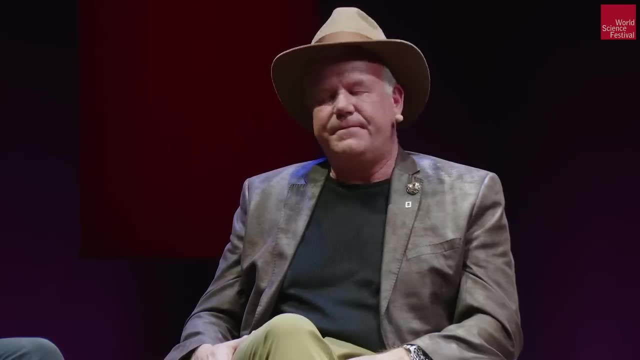 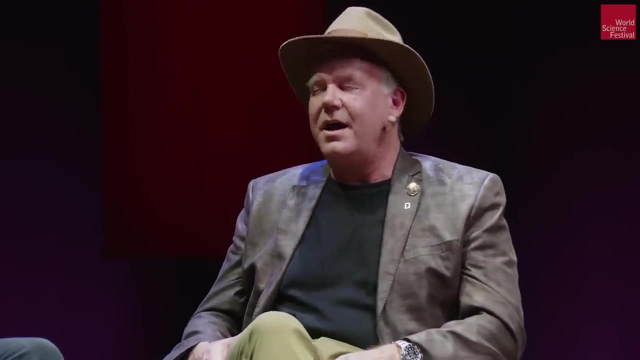 And so one of them. So a couple of days later came into my office Job Kivy and he was a postdoc and he said: would I be his supervisor, And don't call me heartless. I said no. 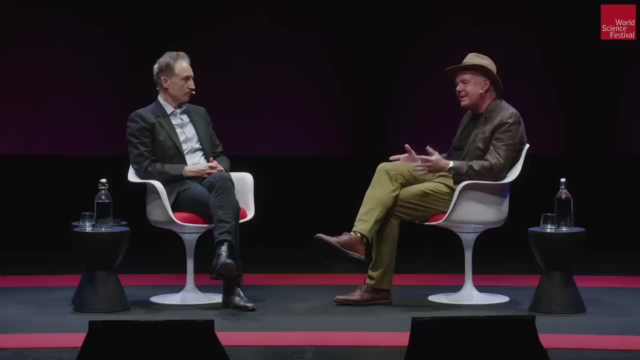 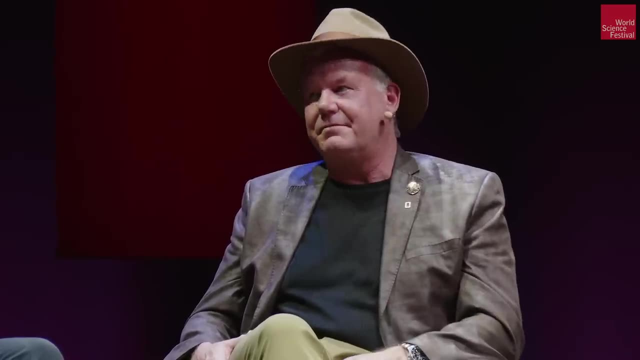 You know, you're a lab guy, I'm a field guy. And then I thought about it and I said: but you know, I've just found this site, I've just found this cluster of trees and it's bugging the heck out of me why I missed. 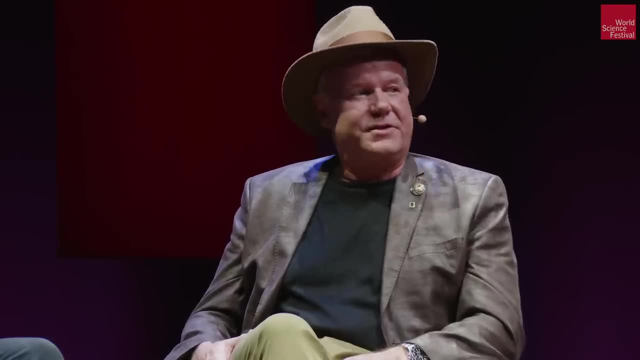 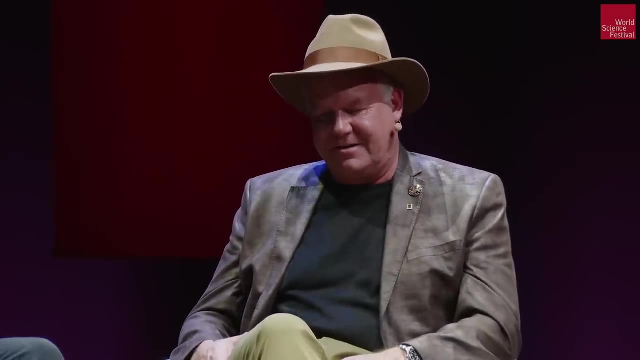 this. I'm going to take another look at it with me. Maybe I'll teach you to be a fossil finder. And so off we went. August 15, 2008,. Job myself, my then nine-year-old son Matthew, my dog Tao. we arrived there. 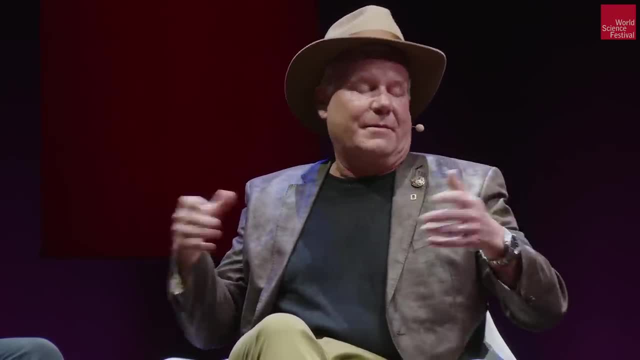 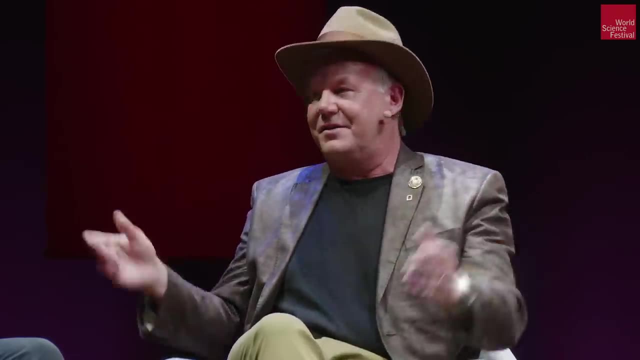 in that beautiful wilderness area And I take them up, I tell them how we found it. you know a much shorter version of what I just told. you Walk up to the site and I say, okay, there's this little hole in the ground, go find fossils. 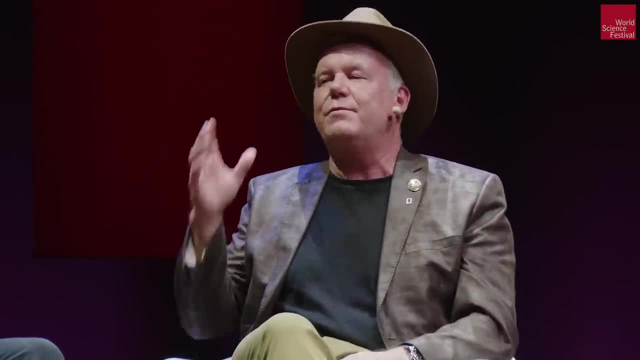 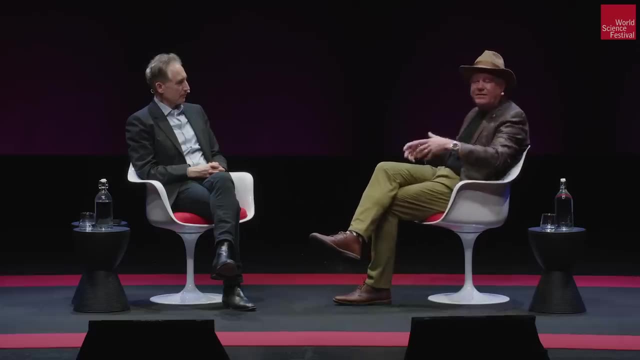 If you find one, call me, I'll identify it. let's see what this site has to offer. And with that, Tao and Matthew are gone. You know they raced off and you know they're leopards and giraffes and stuff and I think. 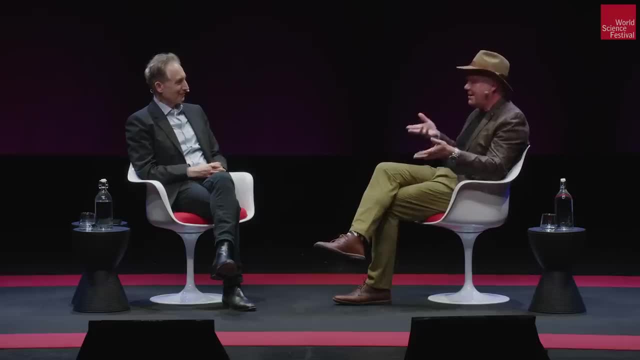 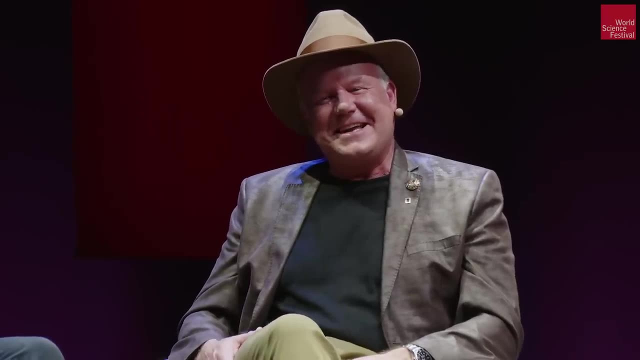 they're going to chase those and they'll see them at lunchtime, And so I'm standing there. that's not funny what they were doing, you know, and I'm standing there telling Job. you know the miners had found it, but they didn't put much blast. 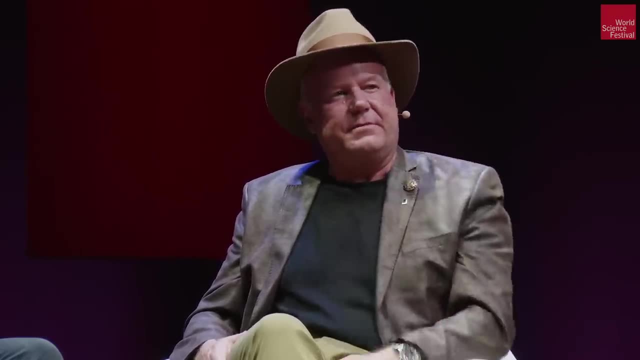 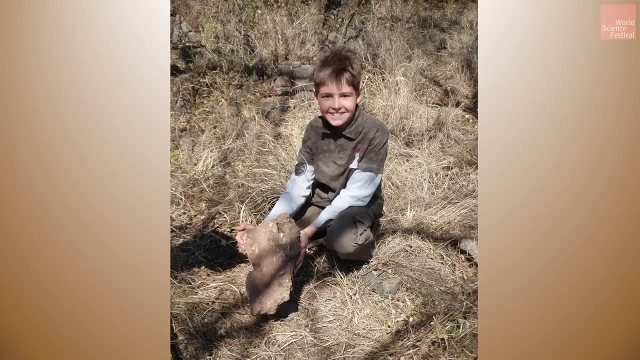 And Matthew goes off and he says: dad, I found a fossil. He calls me, 15 years off, and I start walking towards him. That's actually what I saw: This picture taken at the moment showing this little clump of rock. 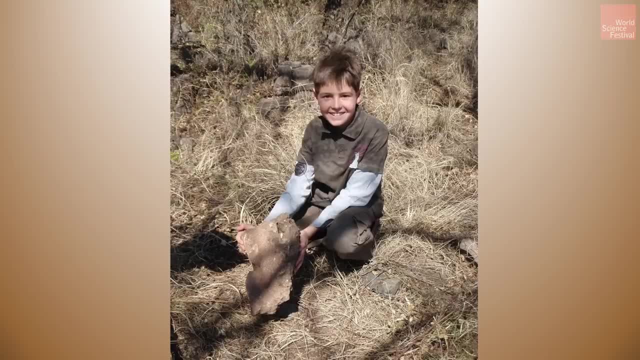 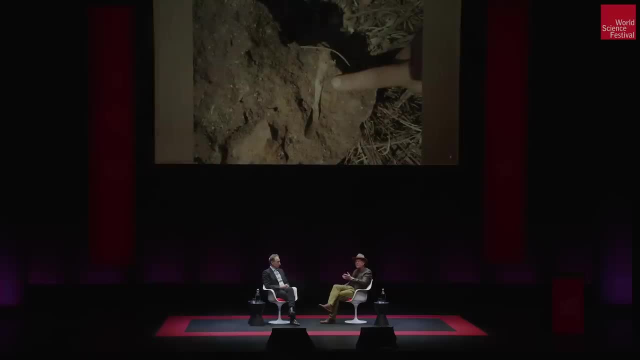 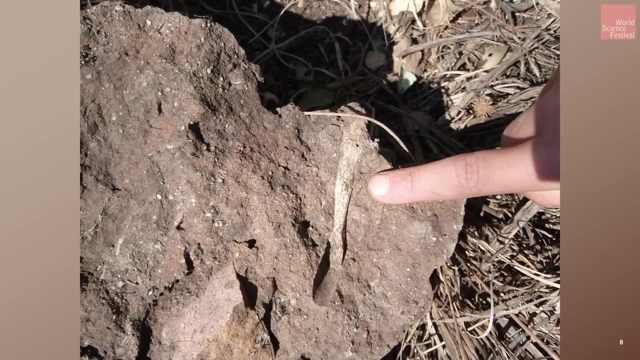 And five meters away, I knew his and my life were about to change forever, because inside of that rock I could see something that would look innocuous to you, that I heard the audience go wow. I went wow because that was a hominid clavicle. 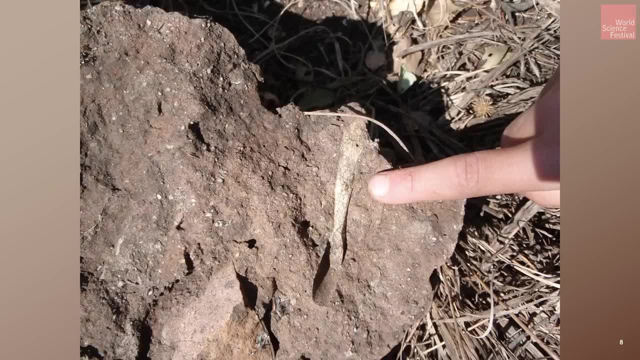 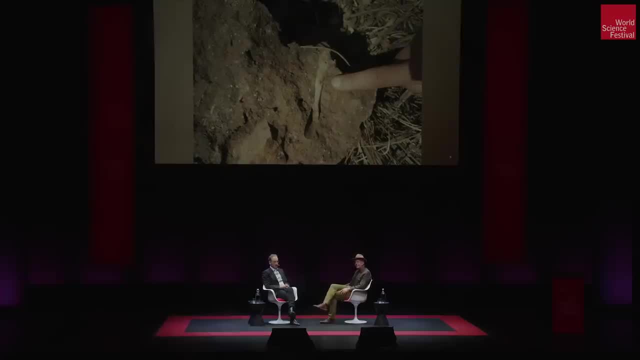 And at that moment in history I was probably one of the world's only experts on hominid clavicles. I'd done my PhD on that bone. All six or seven of them had been found to date from that time. 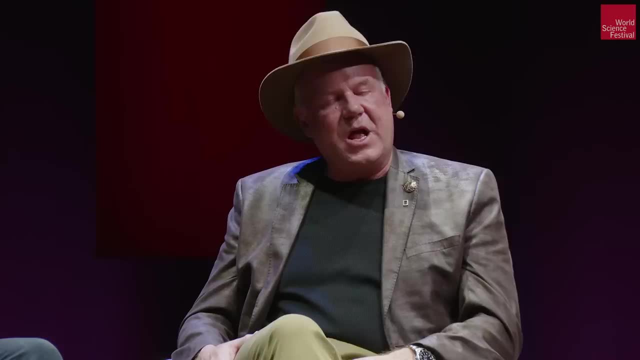 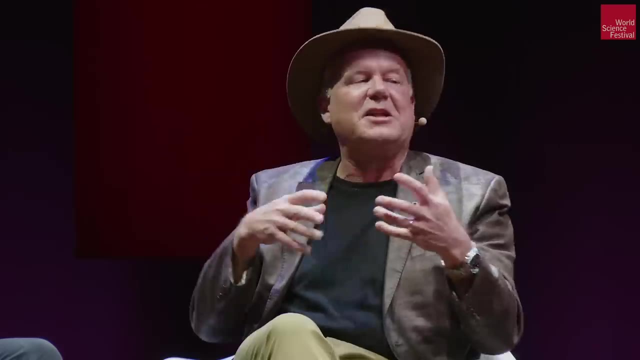 I knew it exactly. it was sigmoid shape, Matthew said. I cursed I don't believe that. I turned that rock over and on the back of it was part of a mandible and the rest of a skeleton coming out of that block. 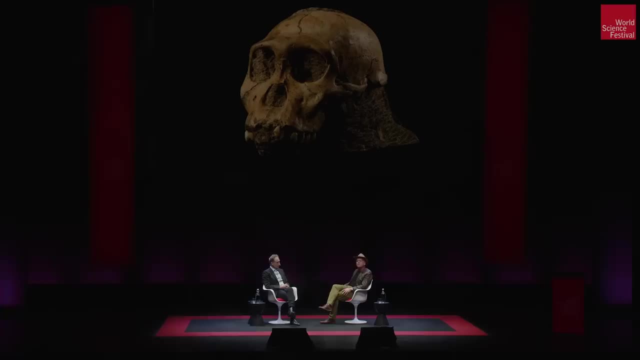 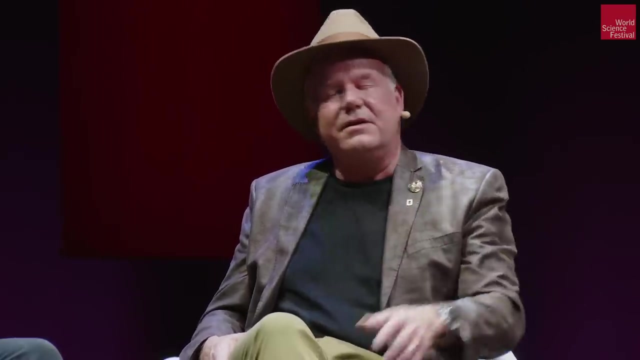 Matthew found a partial skeleton of a hominid, one of the rarest things in all of history. There were literally probably seven or so: Lucy, Turkana, boy, Ones you would hear of, I don't know, I don't know. 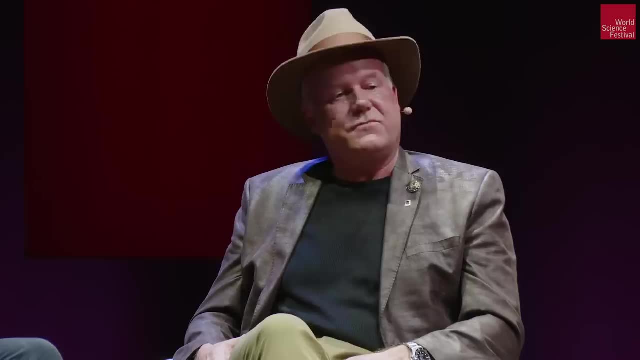 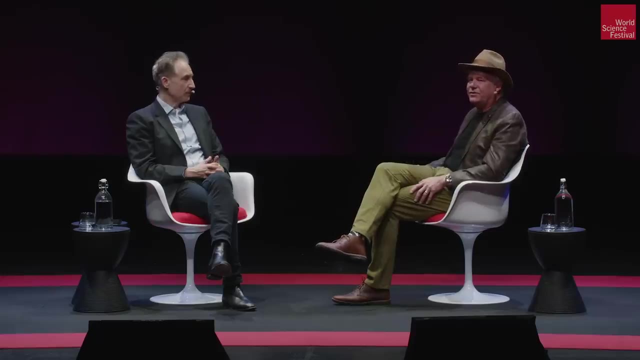 And that was it. And he just found one, And that was, And just lying on the surface, Lying on surface, No idea why, In that rock, And that would lead to the discovery of a new species that you'll see. I mean beautiful. 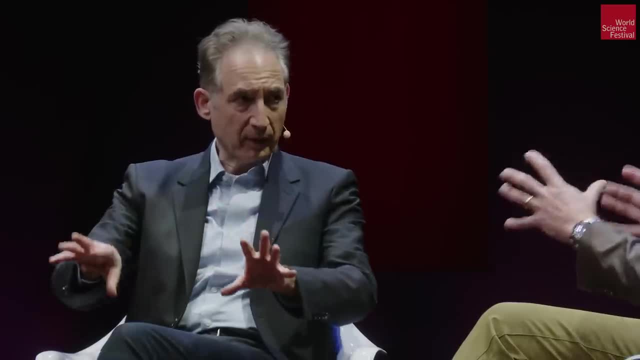 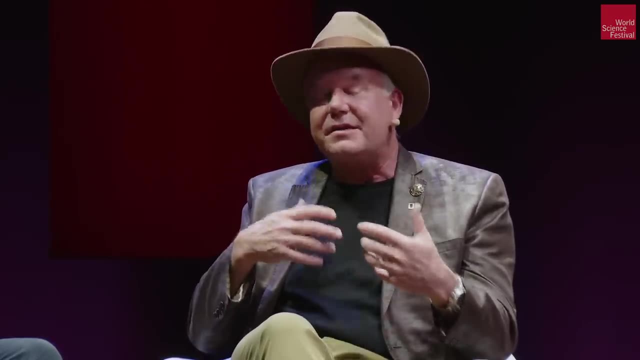 skulls, things like that, All in the area right around there, That's right In the rock. they have to be prepared out. You know, skulls are just beautifully complete from an Australopithecus sediba, we would eventually call it. 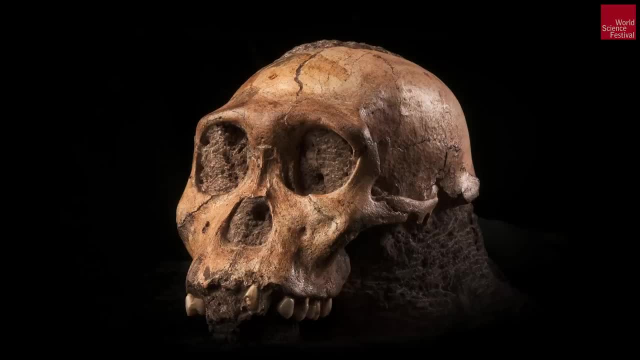 Two million year old hominid things like this. We had never seen things like that in the fossil record And as we would prepare these blocks out, by the way, that takes about 22,000 person hours to get to that state. 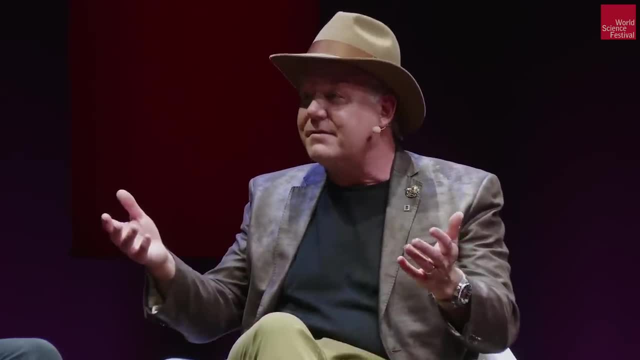 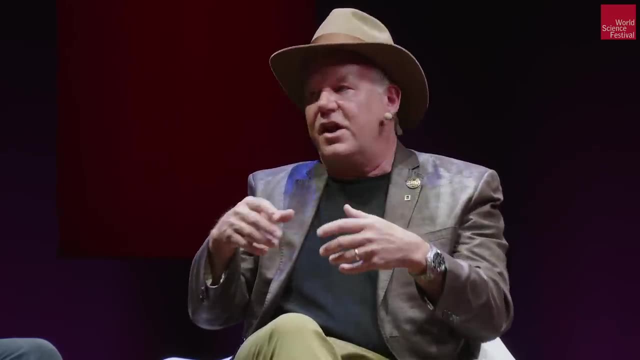 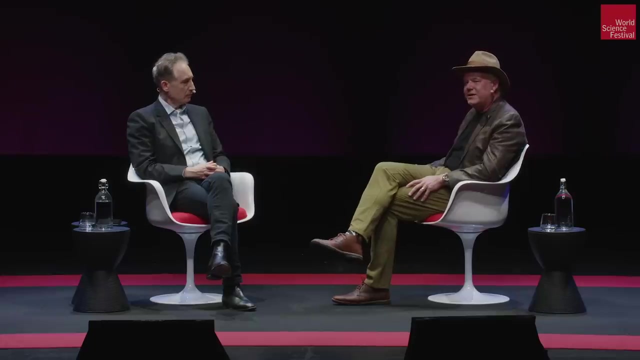 From its concrete like things. we would eventually find skeletons. First time in history, two skeletons had been found together at the same deposit And suddenly my life changed. Yeah, You know, I went from the guy- The guy who was making a career off two teeth- to this one of the richest fossil sites ever. 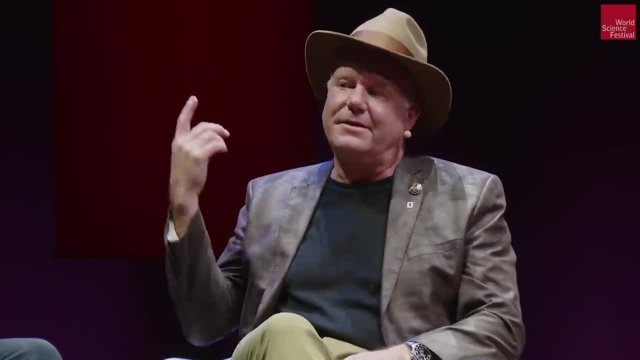 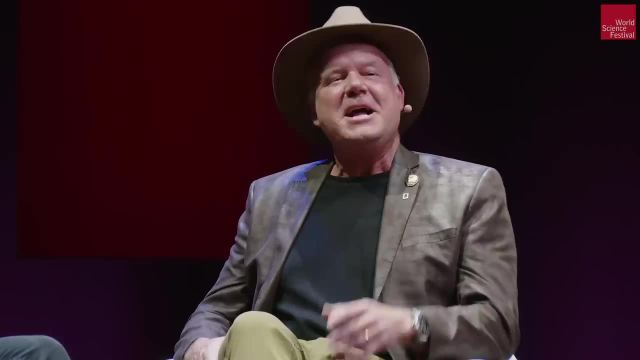 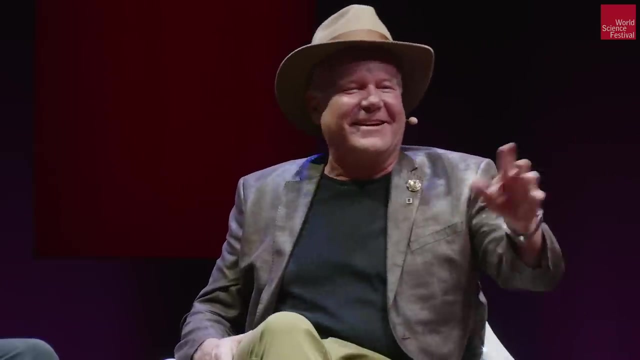 discovered in Africa. We named a new species, Australopithecus sediba, got on the cover of science. Well done You ever been on the cover of science? Not yet, Not yet Three times. That's for you know, people, that I stay at, you know being on science or nature for. 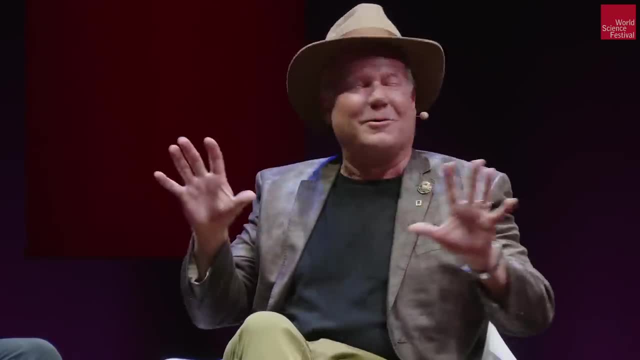 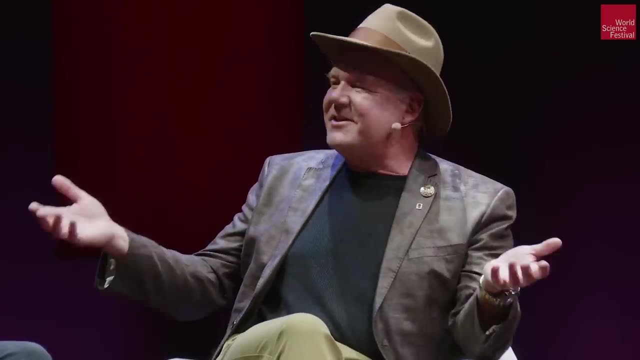 us, our fossils, not us. It's like for a rock star, You know, on the cover of Rolling Stone magazine. Well, I have done that. Oh yeah, Well, Congratulations. And you know, I was living the dream. 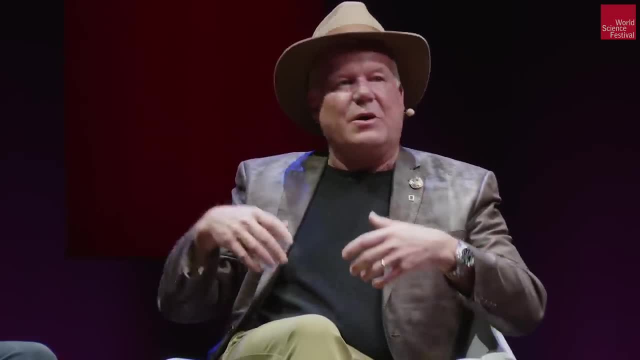 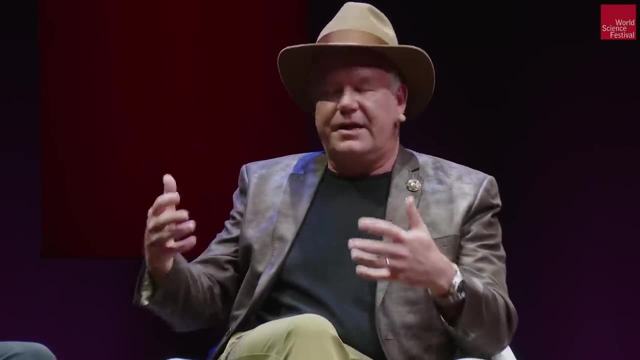 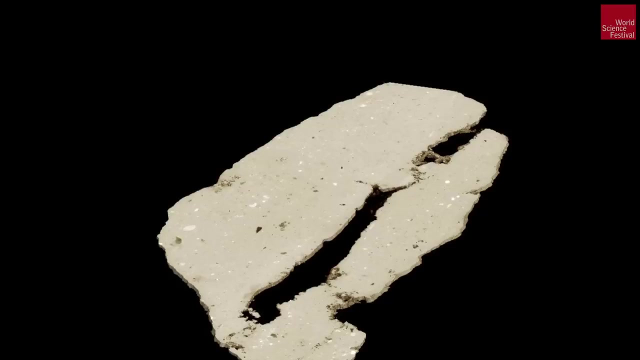 My project grew from one scientist to 40, to a hundred, a hundred plus, in a matter of months and then a year, Paper after paper in the highest journals. I was applying technology. I mean we had the coolest stuff. We were taking synchrotron, highest energy light sources in the world and we were turning 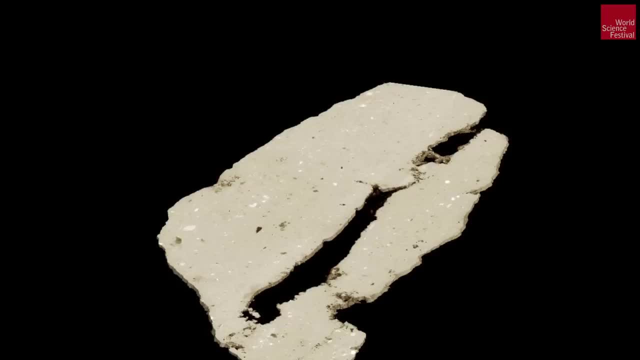 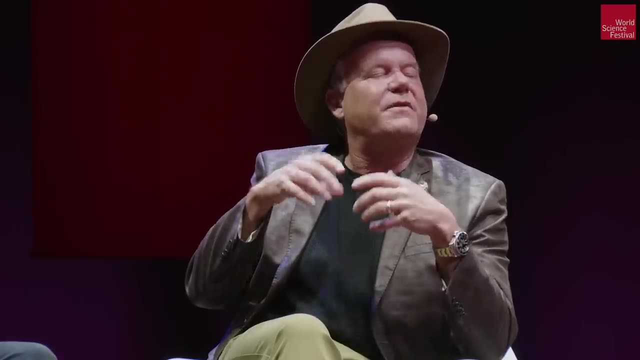 them into these mobile objects. We were doing, we were able to create and reconstruct these just amazing things by using technology. It was the perfect time, the perfect moment to make discoveries. You know, computers had come along. You could image stuff. 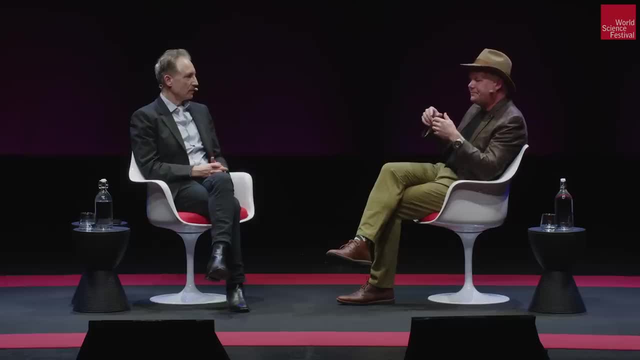 I got to apply open access models to it And I got to bring in early career scientists and other people which was just, believe it or not, anathema to our future, And open access was rare. Yeah, Not only in science in general. 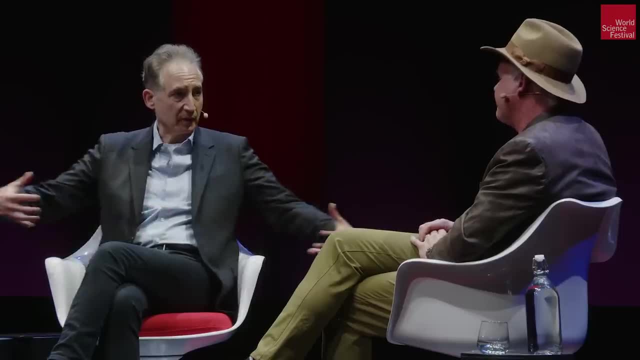 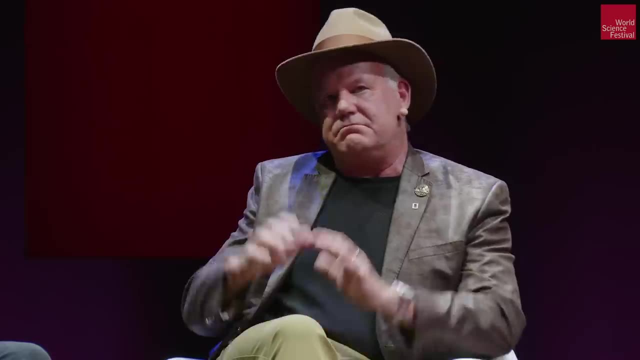 Yeah, Not only in science in general but in your field in particular, which was fairly hold on to your results. Well, it was a field of scarcity. you know you didn't find these things and that was it. And you know, time went by two, three, four years. 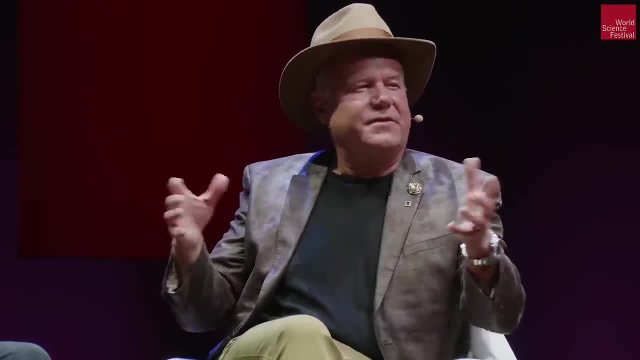 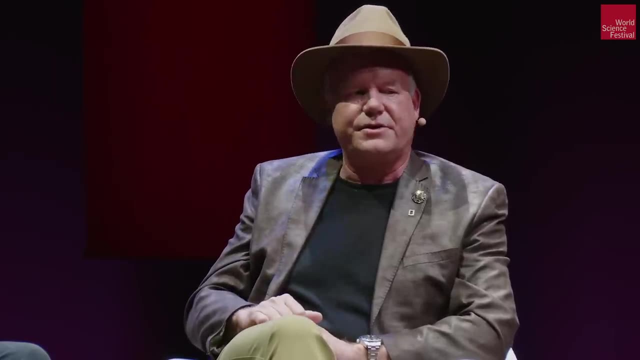 And then we started building this laboratory because we found things like organics over in Malapa- which, by the name of the site, I named Malapa, or my home in the Sotho language- And I started building this laboratory and suddenly got locked out of the site and realized 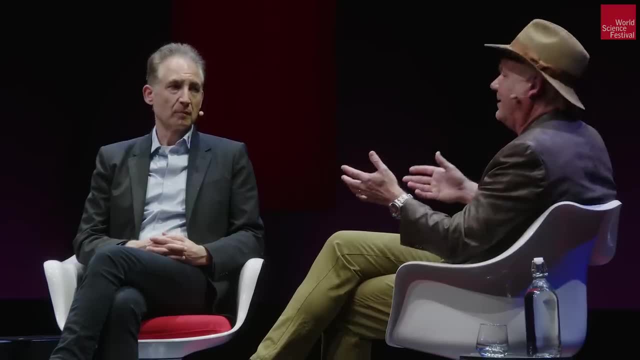 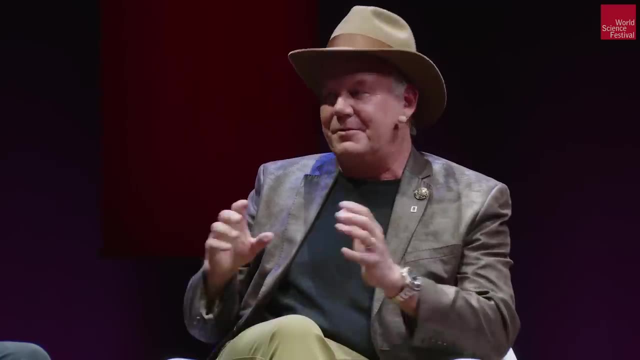 I hadn't been exploring and I hadn't- I hadn't bought that lottery ticket. you know, and contrary to what you say, you know, in my field exploration is the buying of the lottery ticket. If you're not exploring, you're not going to make the discoveries. 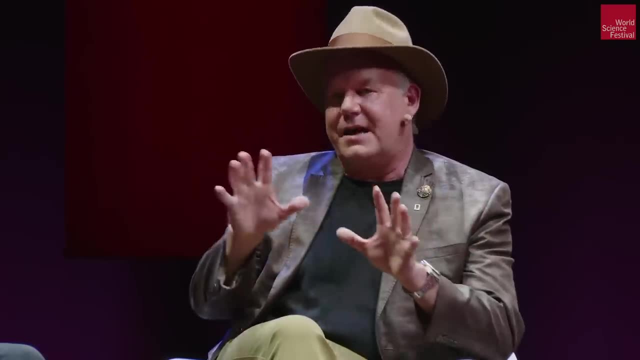 And it was, and so I was thinking: well, you know, what am I going to do while I'm locked out of this site? I got this big team ready and that, and I remember that map that I'd created back in 2008.. 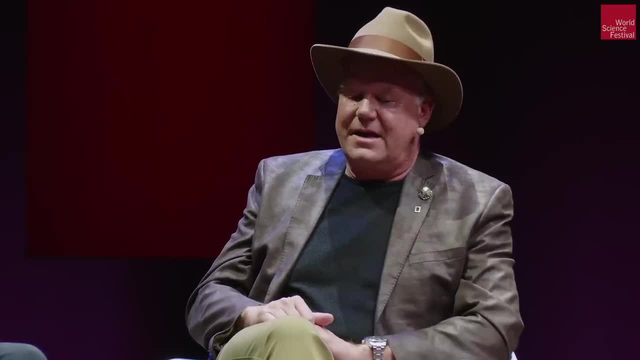 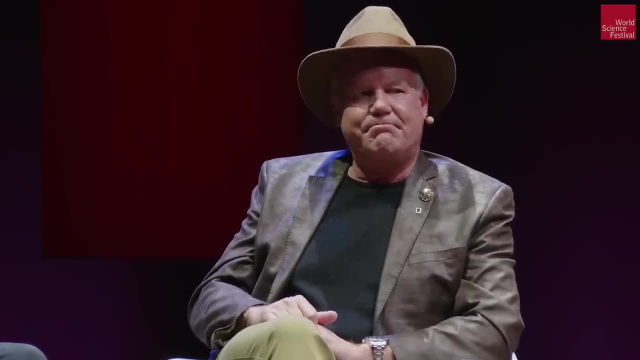 We're now all the way up in 2013.. Yeah, Yeah. And at that moment, a former student of mine, Pedro Boshoff, walks through the door. He's bankrupt, barefoot, in tears. He'd lost everything. 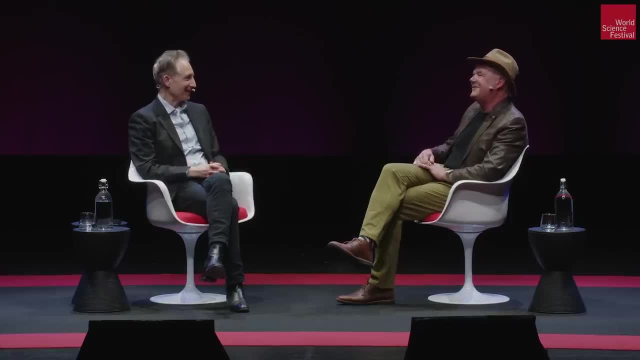 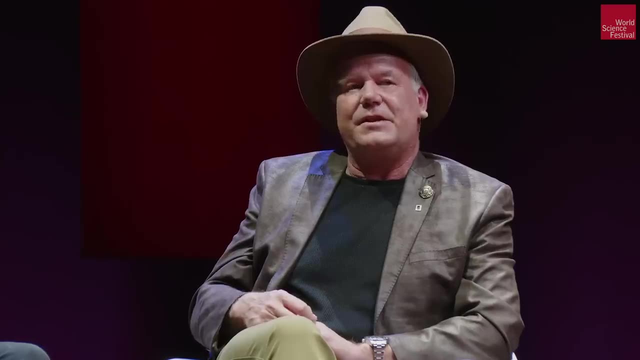 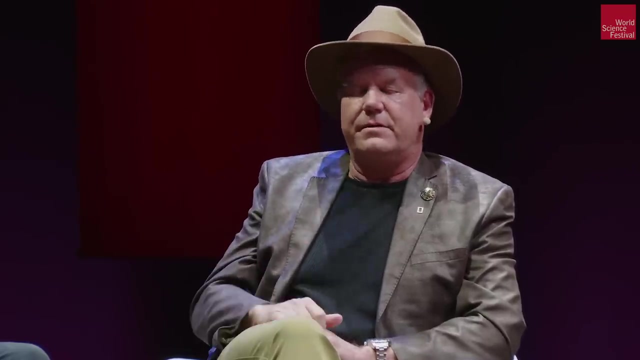 Playing the lottery Well kind of, he went diamond mining in West Africa, but that's as close to that as you you can get. And the coincidence of that was I was beginning to think about what I could do with that map I'd created of you know now eight or 900 localities. 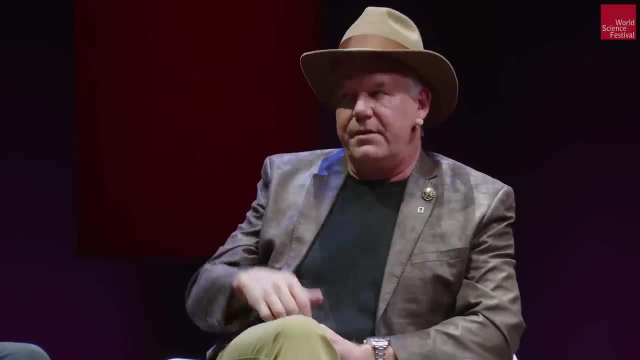 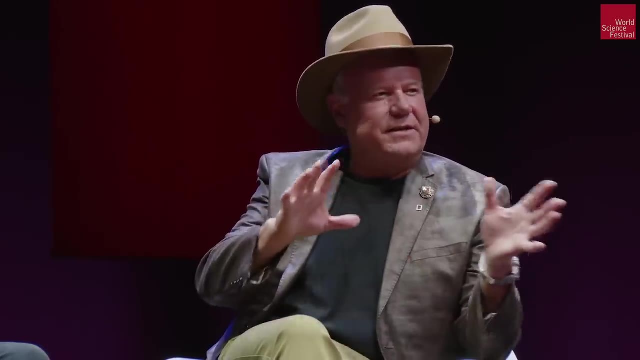 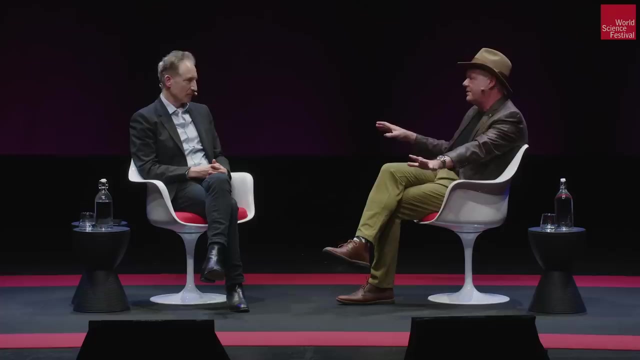 Um, that I'd stopped doing the moment Matt said, dad, I found a fossil. And I was thinking, you know, because one of the interesting things is they're not just on the surface. Every one of those points is potentially a doorway into the underworld, into these spaces. 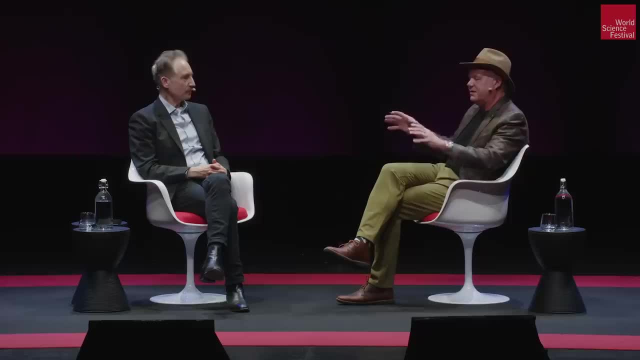 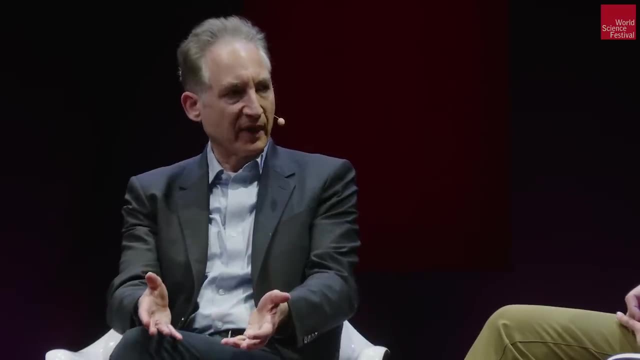 beneath the ground, these labyrinths of cave spaces that cut through that area, hundreds of kilometers of them, but no one explored them at the time. The general sense was: there wasn't, There wasn't going to be a fine to be made underground. underground because the idea 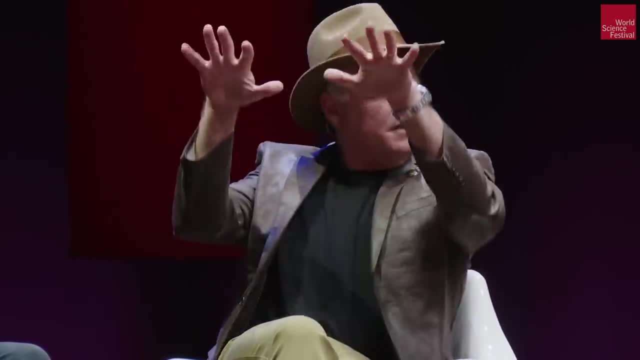 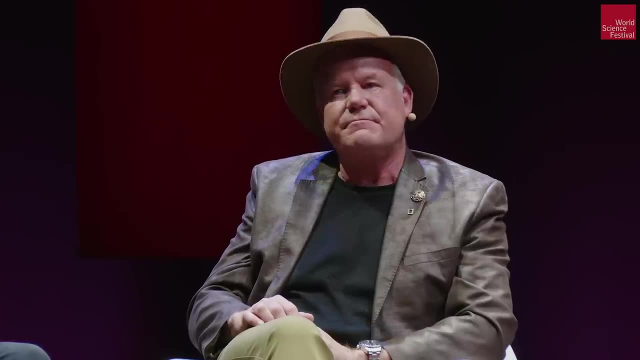 was that the the older caves were on the surface because the grounds eroding away, So the older stuff's on the surface and the caves underground are actually the newer caves, And so the coincidence of all of that, and the serendipity of all of that, was that Pedro 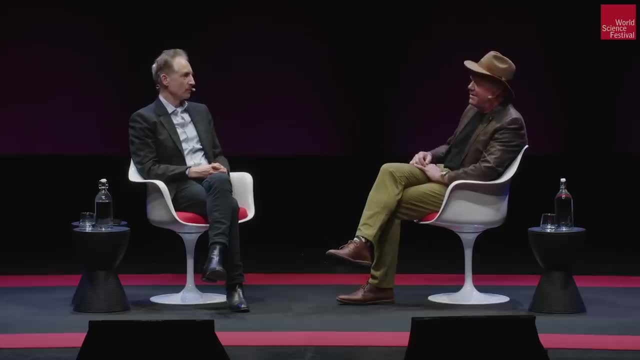 was my caving buddy back in the nineties, And so I said: okay, you know, let's go, look at these, Let's use my map and go underground. What I want you to do is to actually, you know, use these sites to, to, to go to the 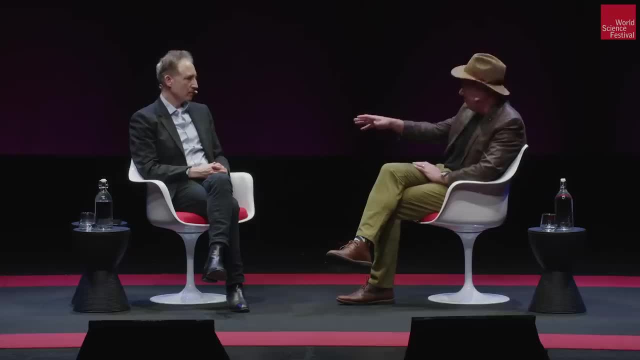 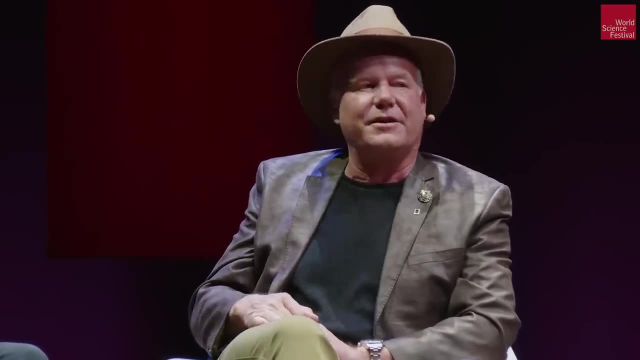 places we think we know best. first because I'd learned a little bit from Gladysville. you know things in your own backyard might be the places, And so off he went. he came back very quickly. he said he wasn't physiologically appropriate. 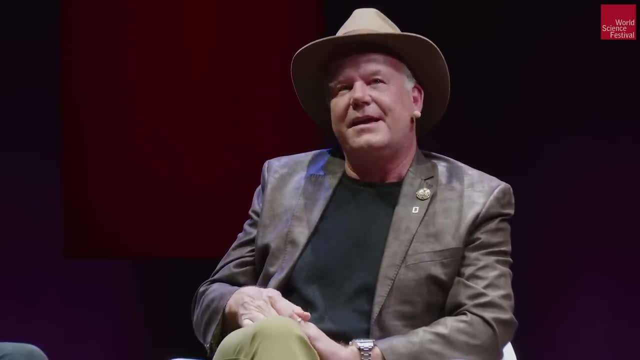 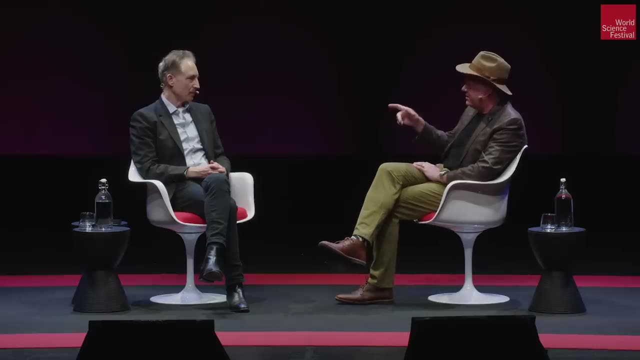 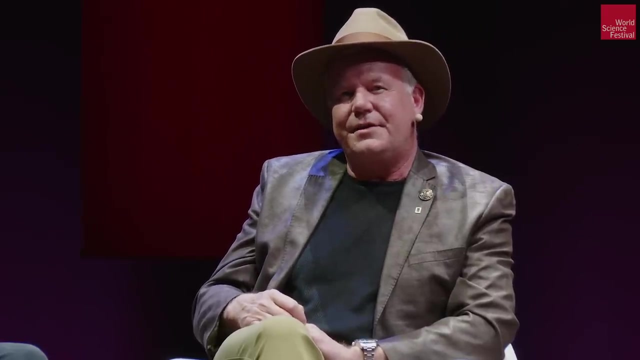 to get into many of the caves. he was too fat, And so we very reluctantly- or I very reluctantly- enlisted with him two amateur cavers, Steve Tucker and Rick Hunter, who were physiologically appropriate for getting into these sites And out they went, and they did a very natural thing. 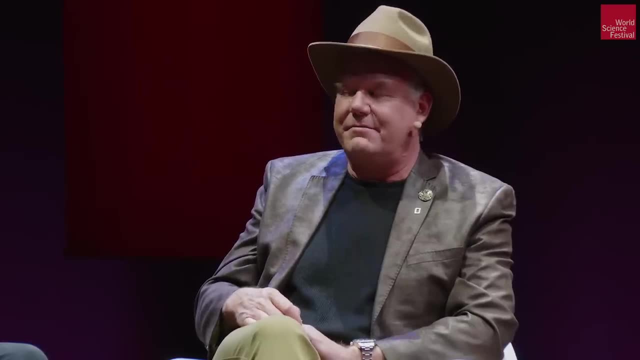 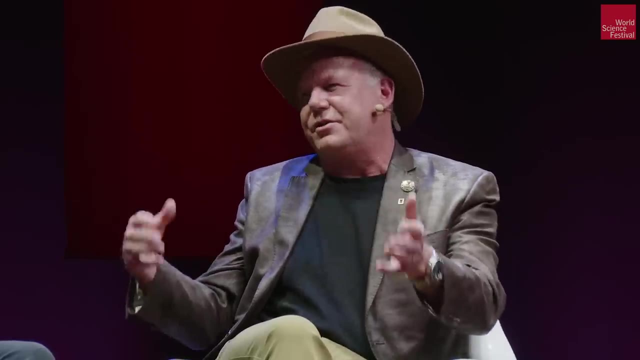 They took my map, all very excited about it, and went to every cave that they didn't know about first, And so they had explored some of these caves. Oh, lots of them had been explored by amateurs and stuff like that. you know, the bigger 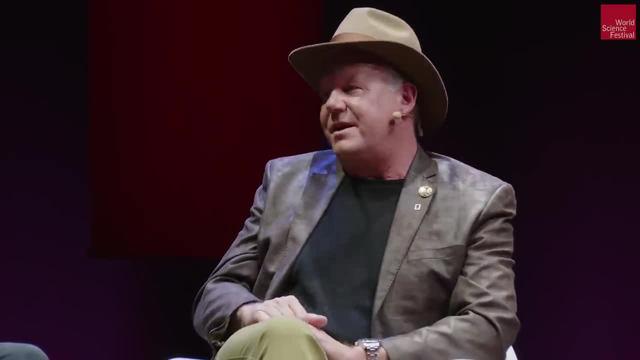 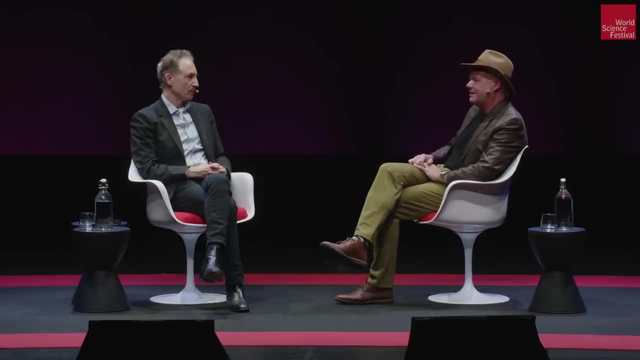 ones and stuff. So they went for all the the new things. it's human nature, And so I was getting reports. We're now moving, Imagine sort of June, July, August of 2013,. they weren't finding much. you know little. 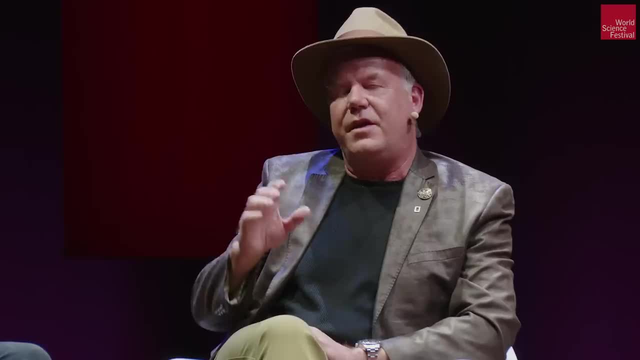 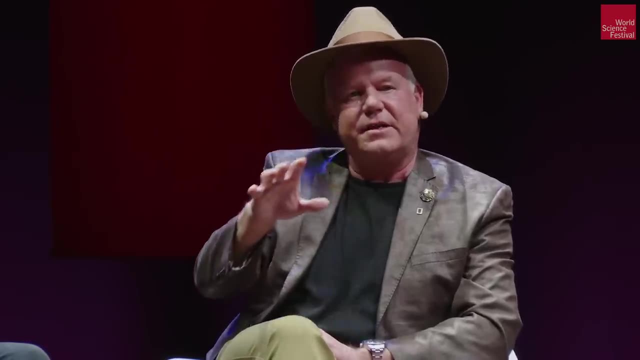 bits and pieces, but nothing really exciting. Then, at the last bit, they went to a cave called the Rising Star Cave, which is a very well-known cave. It's right to paint the picture of this. there are a series of very famous caves, caves. 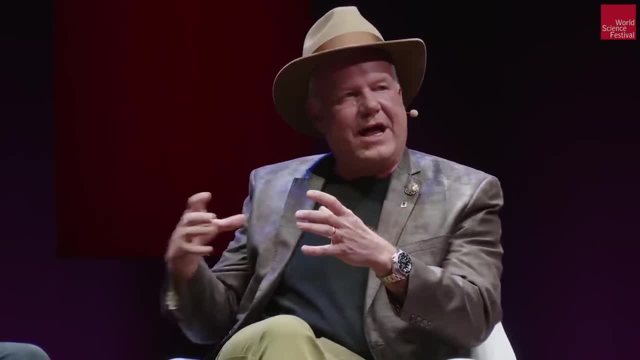 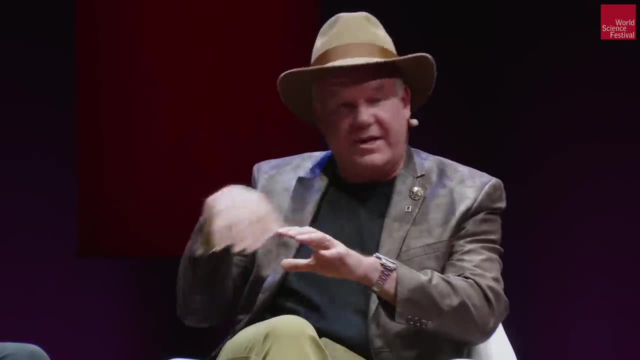 like Sterkfontein and Swartkrans, which all appear in one valley. That was the historical place of discovery. 90% of the fossil discoveries of ancient human relatives had occurred at three sites that are within a kilometer of each other. 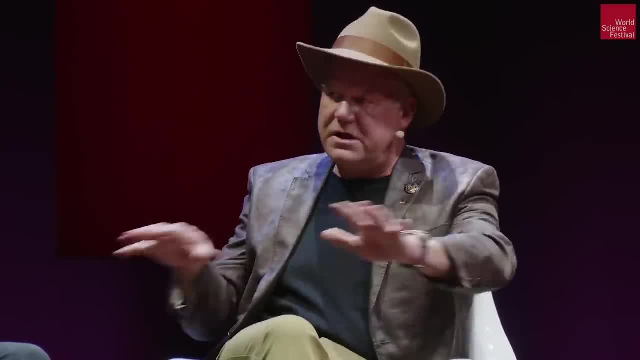 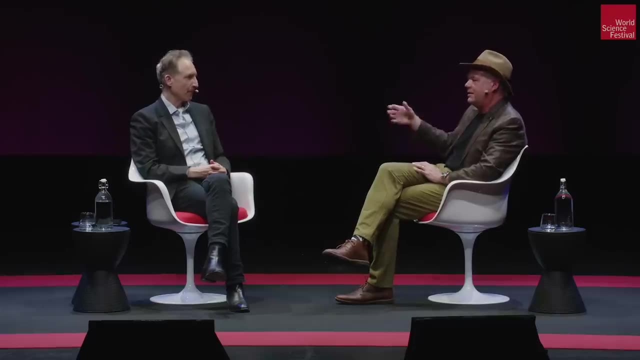 The Rising Star Cave is a kilometer from that, right in the middle of this thing, And so everyone's been in it. It's used for training of cavers. I've been in it in the nineties. you know there's nothing there, but they were dutifully. 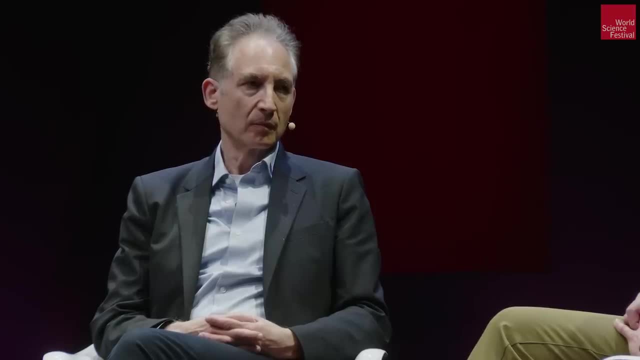 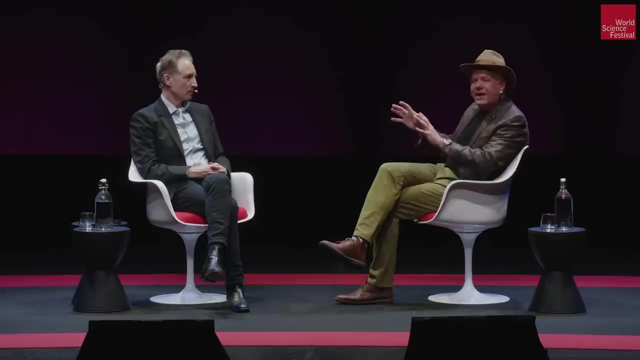 going through everything, And they went in this one night, September 13th, and went through the cave four and a half hours, reached an area called Dragon's Back. This is this area. Imagine it's like 120 meters back into a cave system. 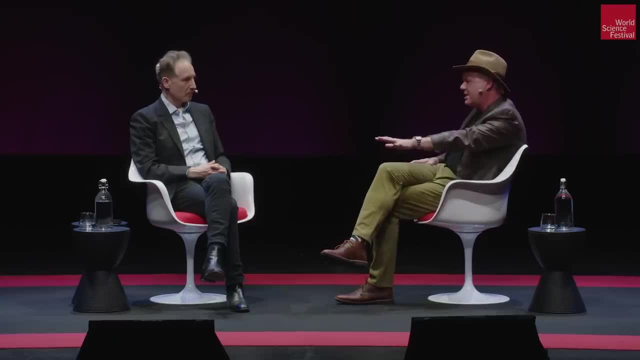 Third of the cave. four and a half hours reached an area called Dragon's Back. This is this area. Imagine it's like 120 meters back into a cave system, 30 meters underground, And they crawled up this Dragon's Back, which is a rock collapse to the top of it. 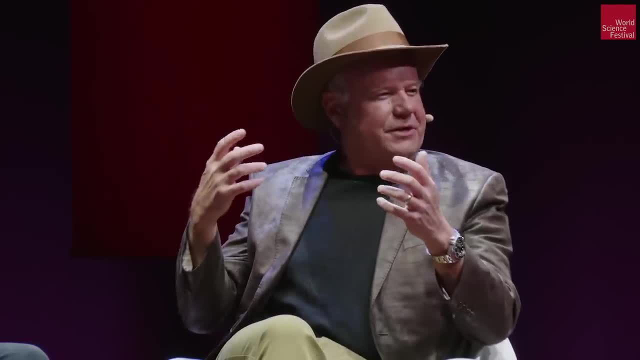 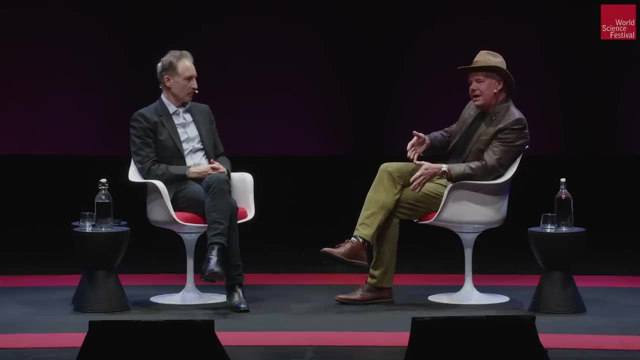 And at the very top of it Steve was trying to take a picture, get a picture of himself, And he slid into this little slot and his legs went down a hole And he told Rick: it goes, And in cavers that means like it doesn't stop. 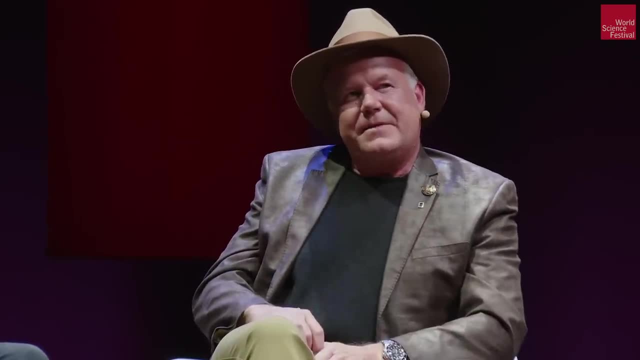 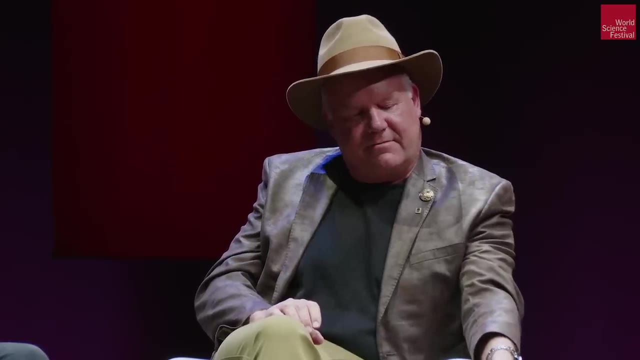 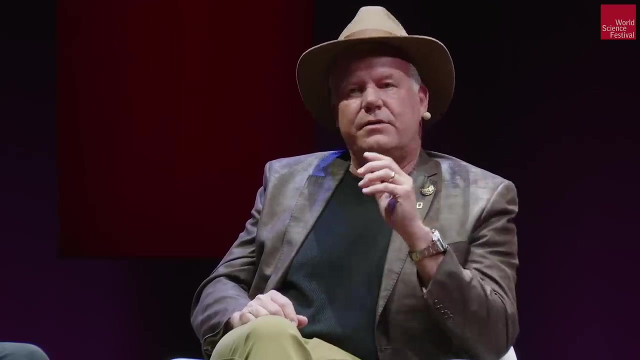 That's a big word, I know And, being young and skinny and insane- Down he went, Not knowing if it opened up into a big thing and he dies or whatever if he could get out, And it goes 12 meters down into a chamber. 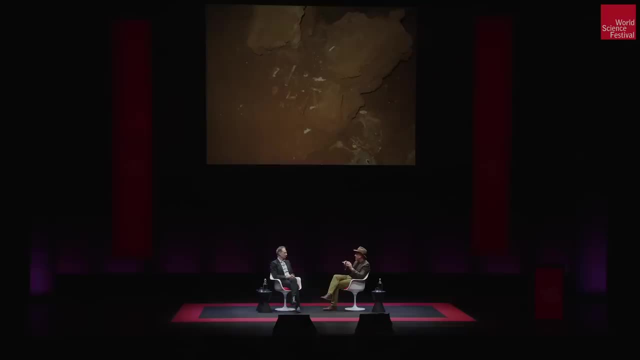 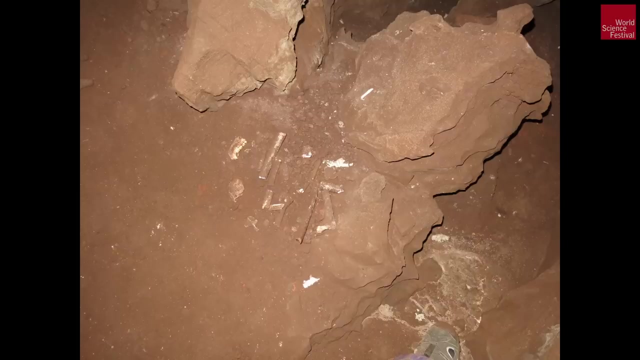 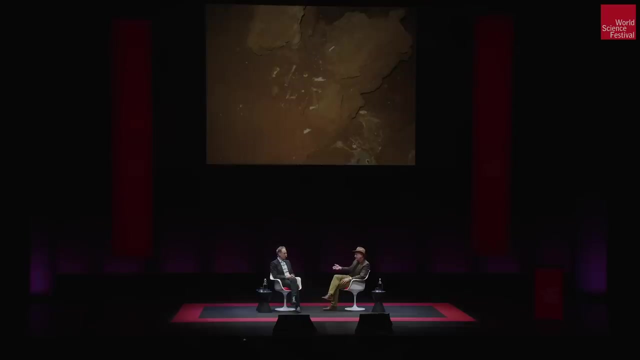 And inside that chamber they saw some bones on the ground, Little white specks like those. They didn't know what they were, but they took pictures of them. That picture And they went out. took them forever to get out And the next couple of days I'm sitting at home 9 o'clock at night. 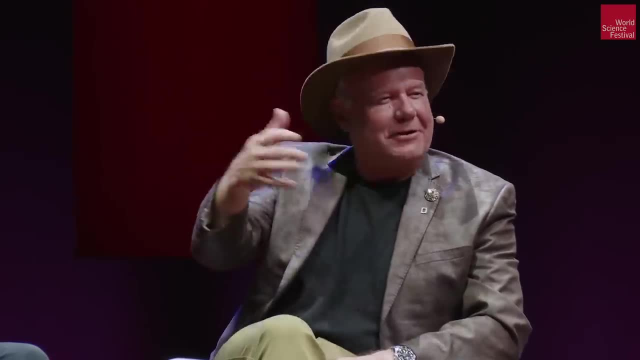 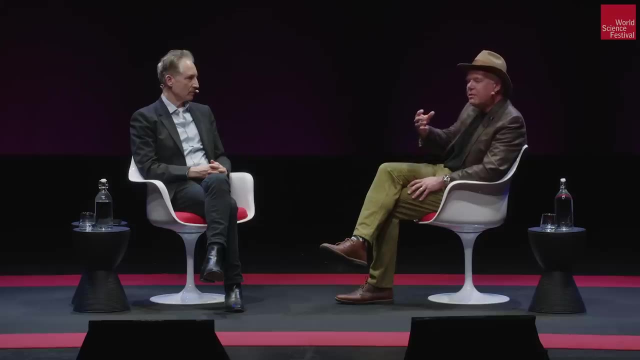 And my intercom. this is Johannesburg, so we have gates and everything long distance to your house. My intercom goes 9 o'clock at night. I answer it and there's Pedro on the other side. he says: you're going to want to let? 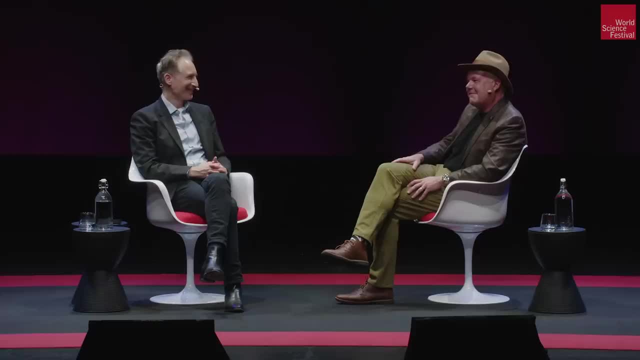 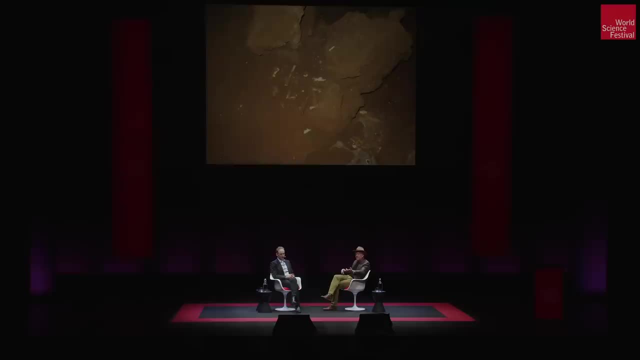 us in Creepy like that, And I almost didn't. Then I did, And Steve and Pedro come in. They opened their laptop, They showed me this picture And they showed me the next picture. Ah, There, I got one. 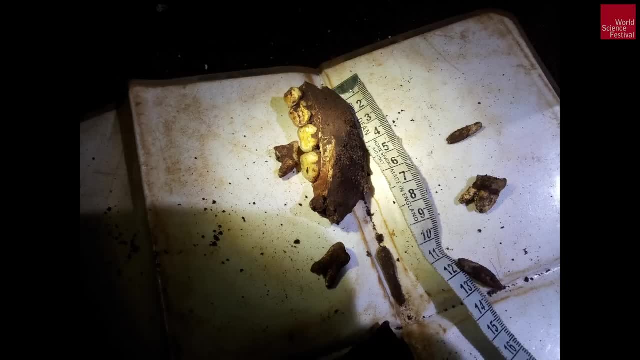 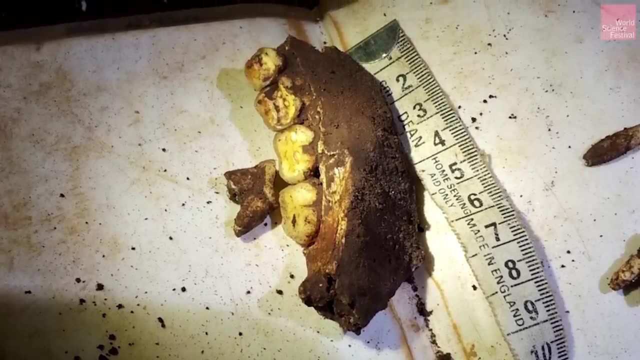 There I got one That is a hominid mandible, And immediately I realized that that's not just any hominid. I could tell by the audience reaction. They too realized that that is a primitive hominid, because the tooth morphology extends. 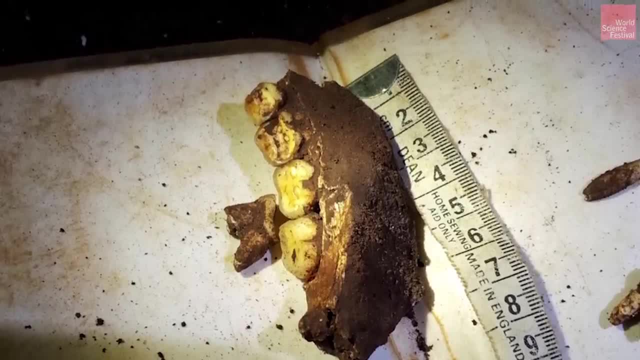 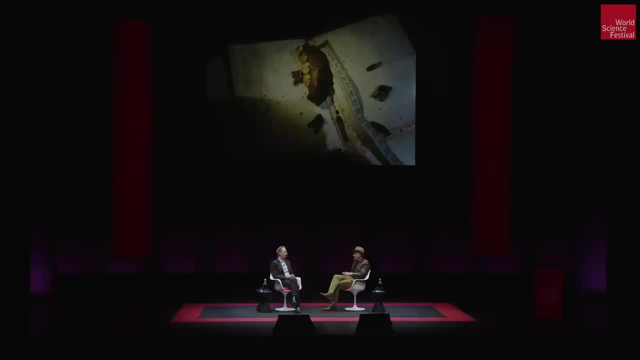 to a larger and larger molar row, which I could tell at least 80% of you knew instantly, And I thought, oh my goodness, no human being. I guarantee you had ever seen an image like that anywhere on the planet. 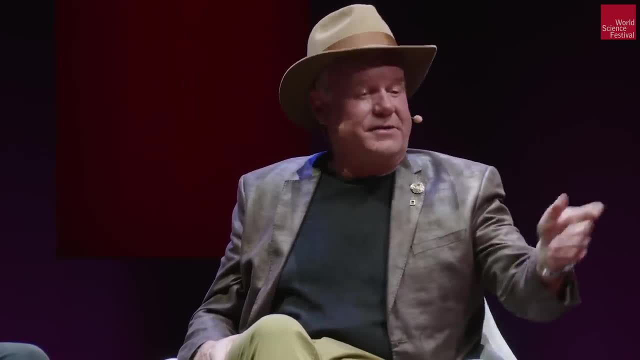 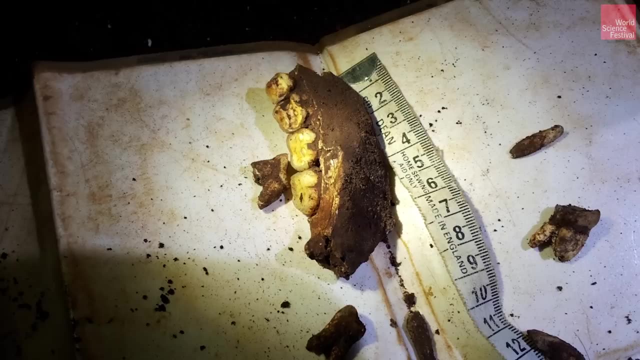 That's a great picture. Like I said, 22,000 hours to get that skull out. This is laying on the floor, And every picture they showed me had another one, and another one, and another one, And they described the situation it was in. 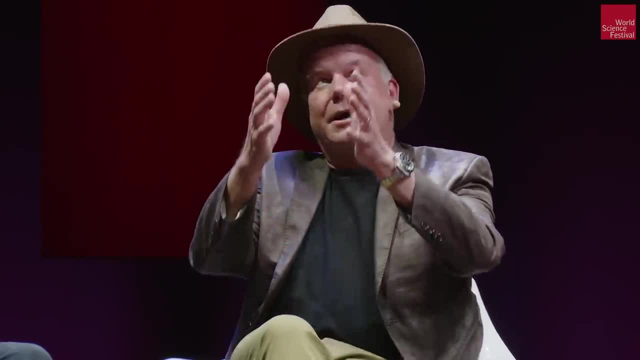 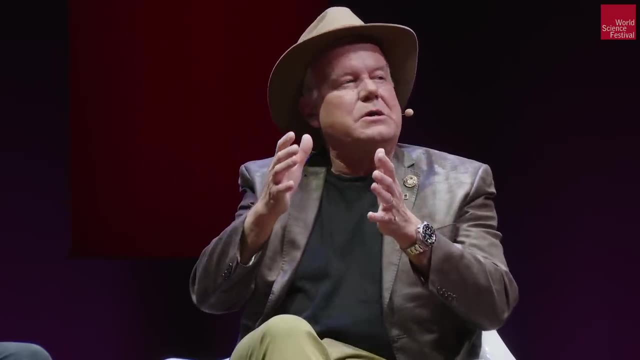 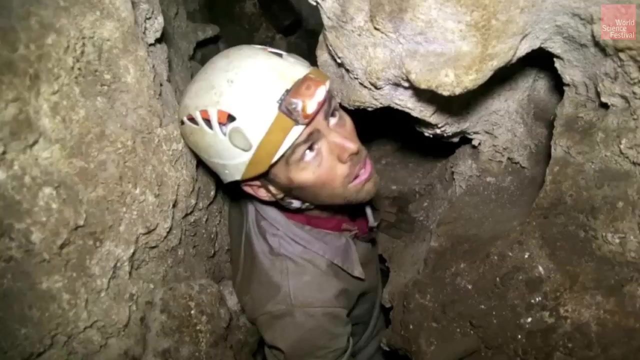 This 130 meters back up this climb and down this shaft that they happily fed. The chute-like thing they described was 19 and a half centimeters is its widest, 17 centimeters is its narrowest, With all these terrible moments in it and these guys, you know, these guys are the size. 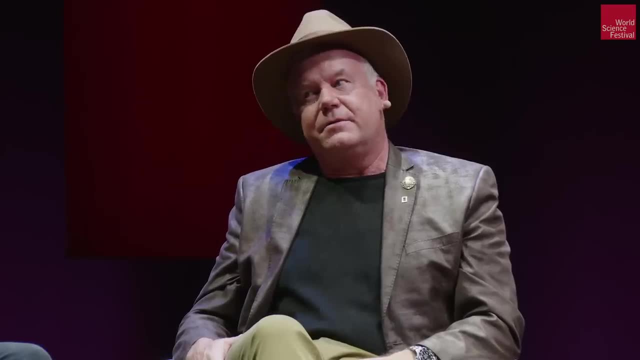 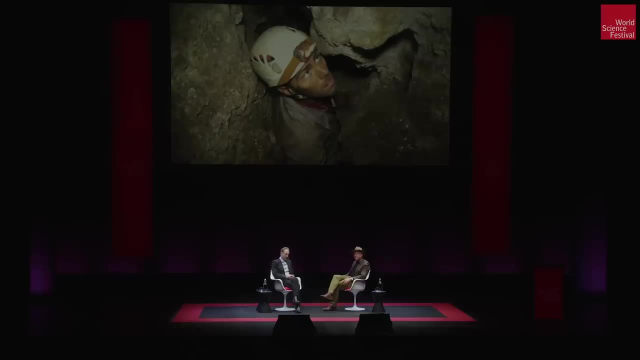 of paper And I was like I will never do this. That's it. That's the entrance, That's the wide part. Look at his helmet, folks, to get an idea of that. You want to see how really bad it is. 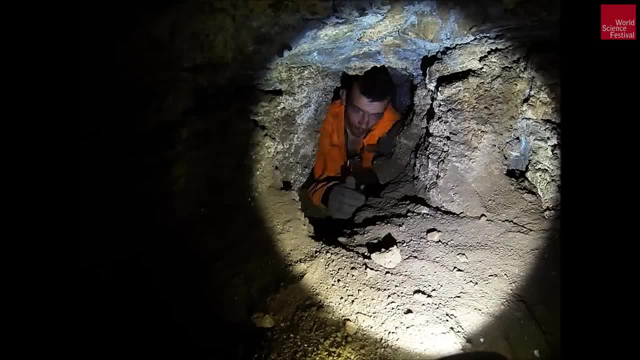 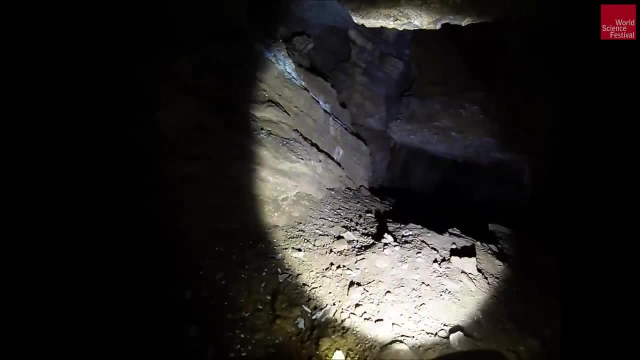 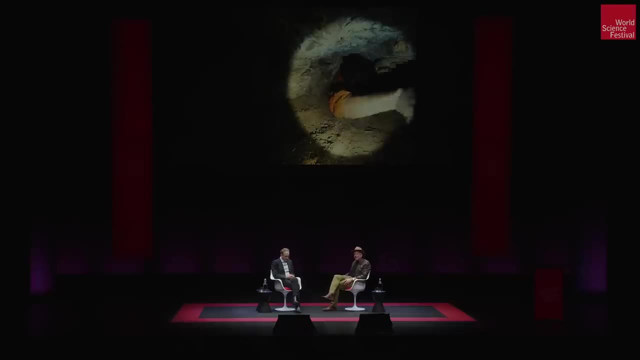 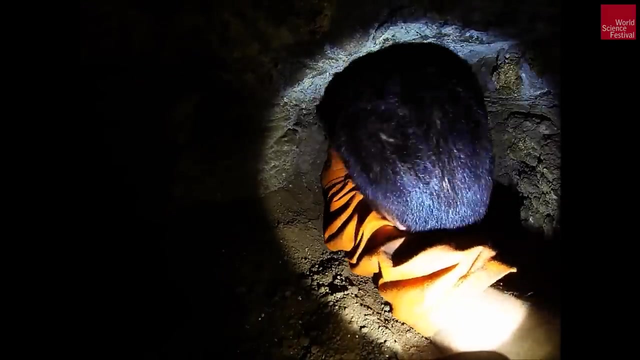 This. Yeah, Here we go. This is what it looks like. This is the easy part, folks. This is what we call Superman's Crawl, And this is where you have to, Superman, because you know the flying position. You extend your arm out and you go. oh, come on, we all, I get through this. 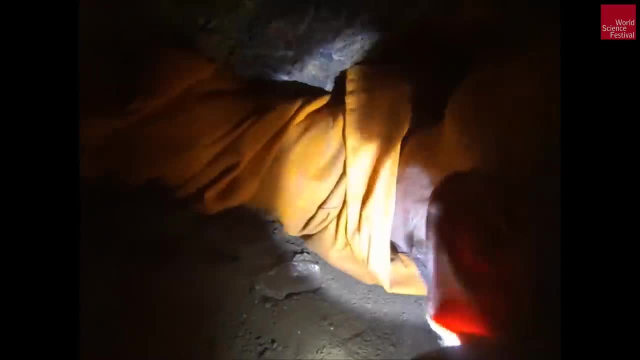 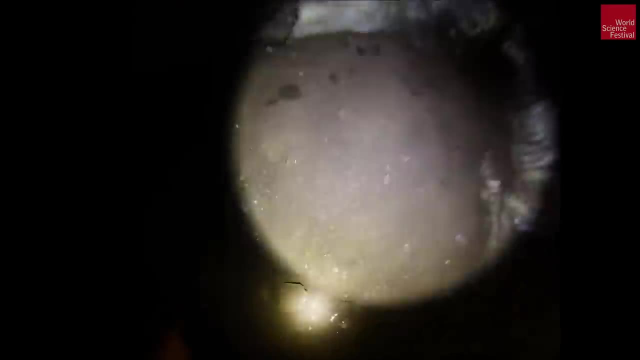 That's not terrible. You go through this. You climb Dragon's Back. You then get to the hard part, the chute area That you go. it's not that bad folks, It really isn't. Even in this dark I can see the claustrophobes like all going. you know, looking down at. 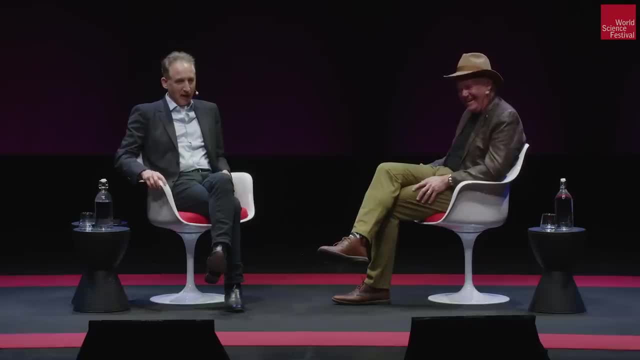 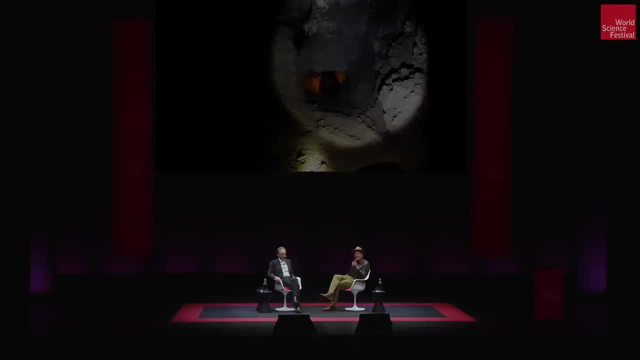 the ground. Well, you're making me anxious. right now I need a sedative for an MRI. You want to be anxious? Let's look at what it's like, if we can, of what it's like to come through the chute. 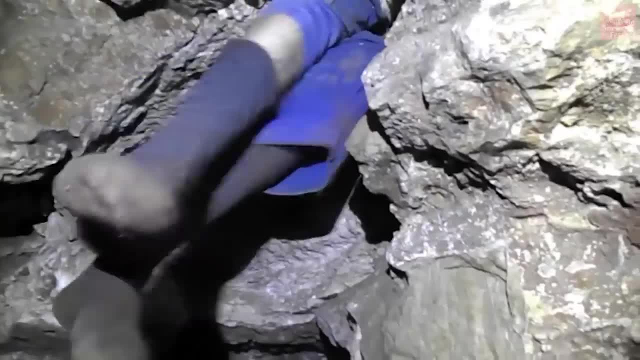 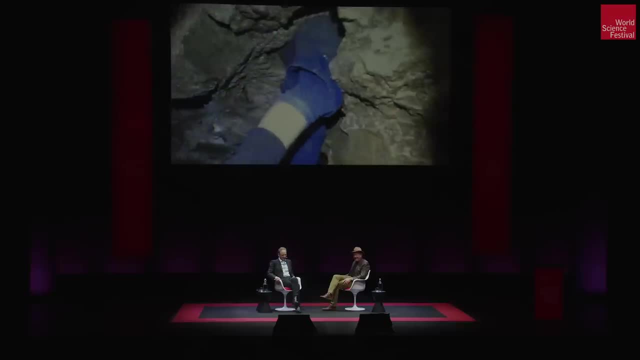 I think the next video does that. This makes me anxious too. by the way, I did that once I was a baby. I think You came out feet first. That explains a lot, Maybe. yeah, right, So is that now at the end of the journey? 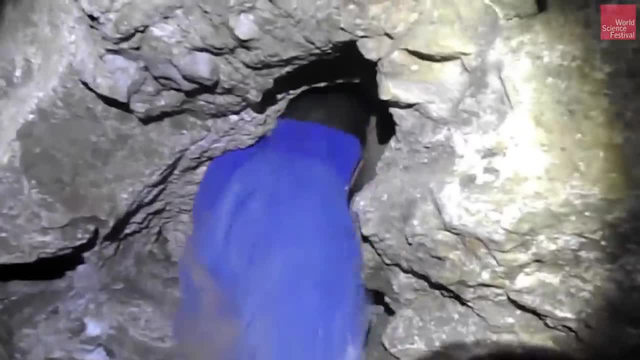 That's in the first chamber. You're in these spaces, in these very narrow spaces, and that's what we had to do. So you've got to remember. I'm seeing this, I go through there and I'm wondering how we're going to do this. By the way, in order to test, I'd hired these amateurs to see whether it was real, because, you know, I'm trusting the entire reputation of my team. If I put together an amateur, I'm going to be able to do it. 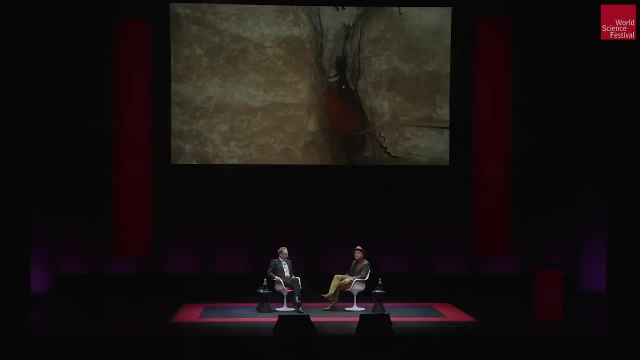 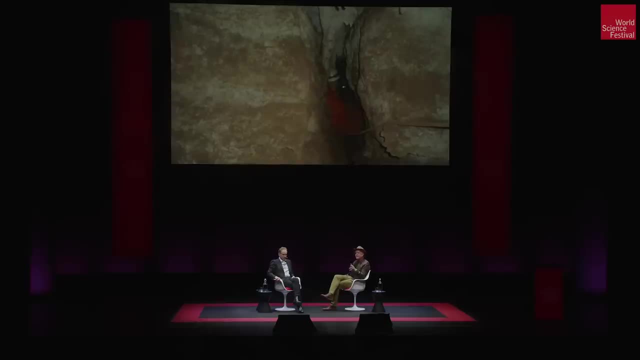 Pedro and Steve left. I'm all full of this. oh my goodness, this is a gigantic discovery. They're lying on the floor. 2 am in the morning. I called the head of missions at National Geographic Society, Terry Garcia. 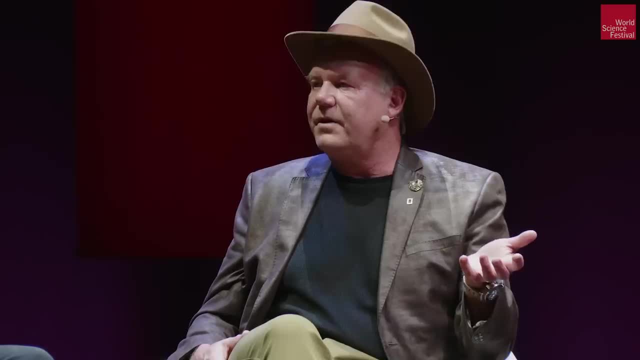 2 am in my time. I'm like: oh my God, What is this? I'm like, oh my God, Oh my God, Oh my God. I'm like, oh my God. I'm like, oh my God. 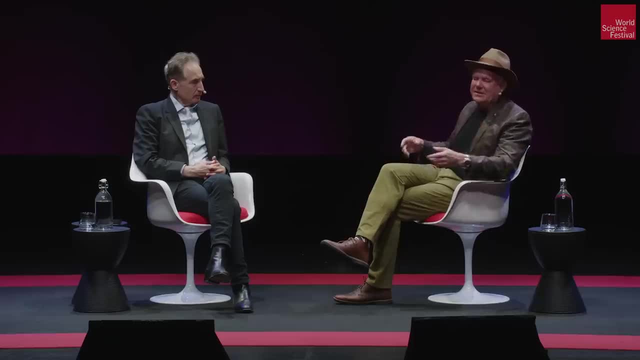 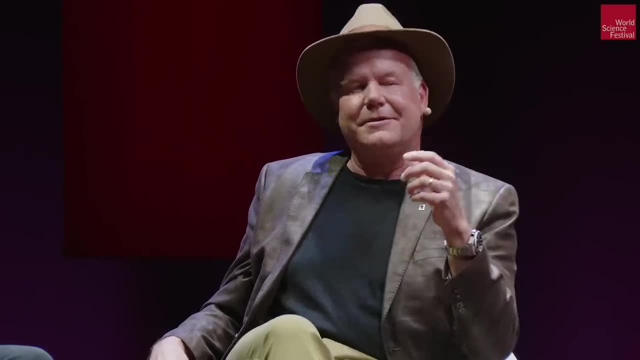 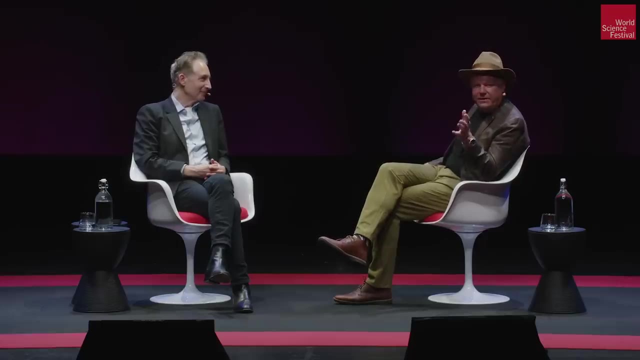 Terry Garcia, 2 am my time. It was like earlier in the US And even though I had caller ID, he answered the phone And I showed it. I said: are you near a computer? I showed him those. 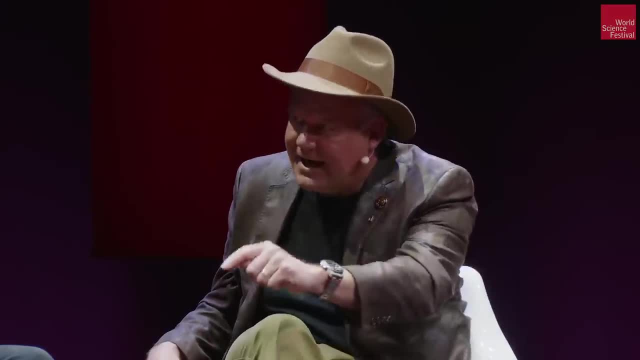 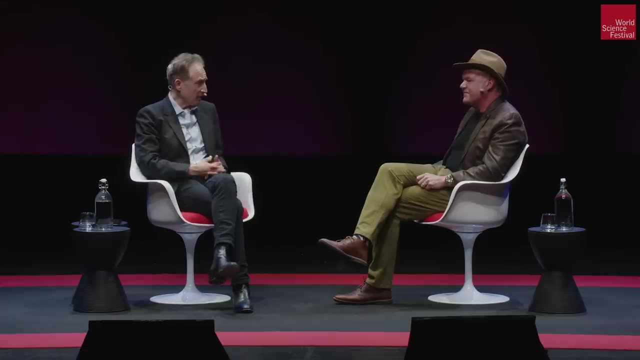 pictures And I said: if you are ever going to believe in me, believe in me right now. That's explorer, speak, for I need money And they had funded you in the past. Yeah, Okay, And he paused for a little bit And he said: okay, Lee, do what you need to do. 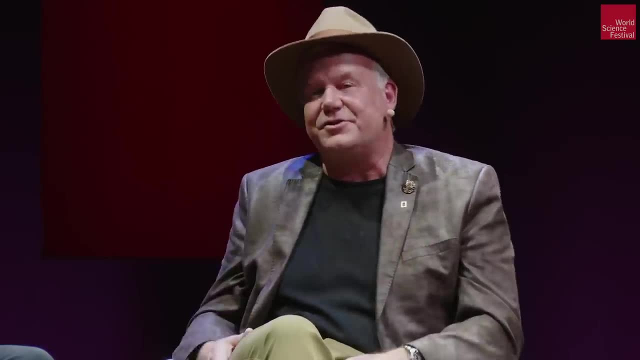 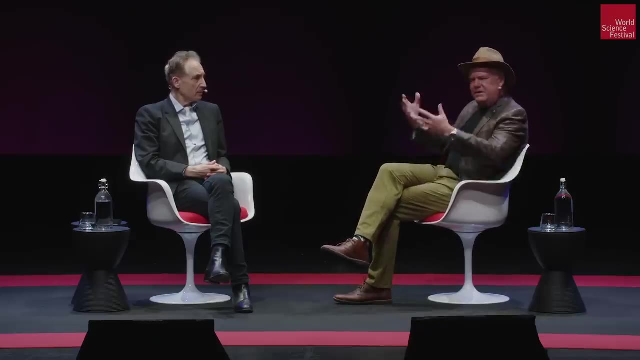 That's funder speak for. okay, spend some, but don't do too much on that. I hung up the phone and I got cold feet Because I'm just risking. I have this incredible. I mean I'm living the dream of science. I have this incredible team, one of the biggest teams. 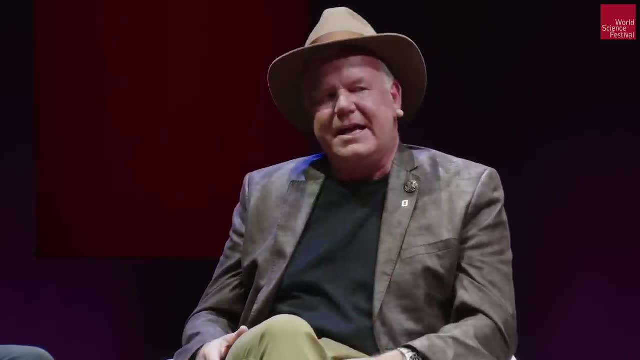 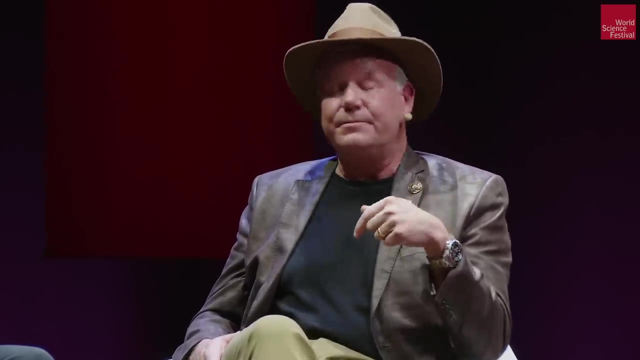 ever assembled for this, all these prestige papers and all that, And I've just risked the entire reputation onto amateurs In this sort of situation, a place I will never go. But you saw the photo right. Was that You ever seen Photoshop? 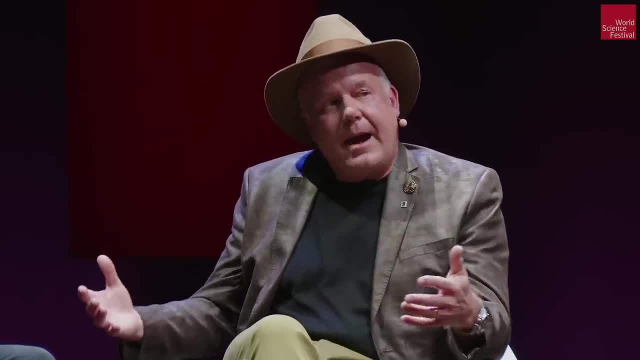 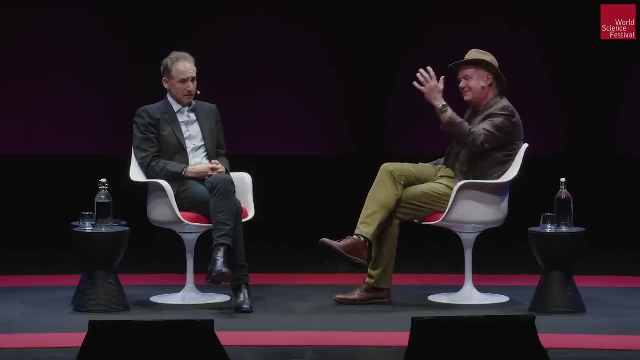 No, seriously, Yeah, You're worried. that could wow. People do funny things, Huh. Oh, come on. Someone just faked a shark picture and it was a plastic model You saw that from. I mean, it'll do anything. I've seen Bigfoot too, So how was I going to test this? So I knew 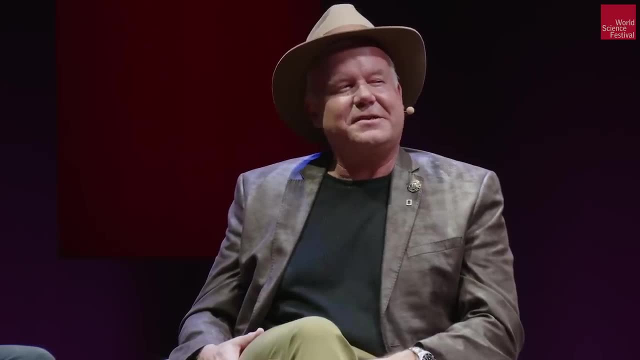 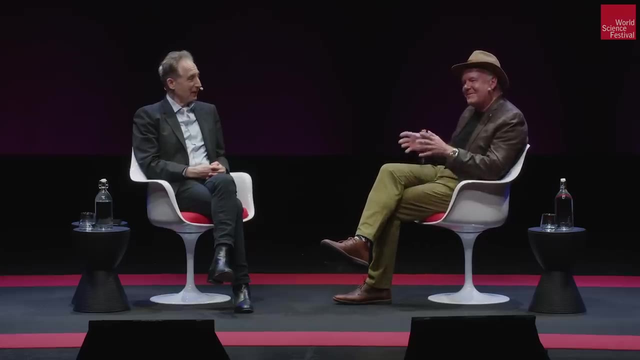 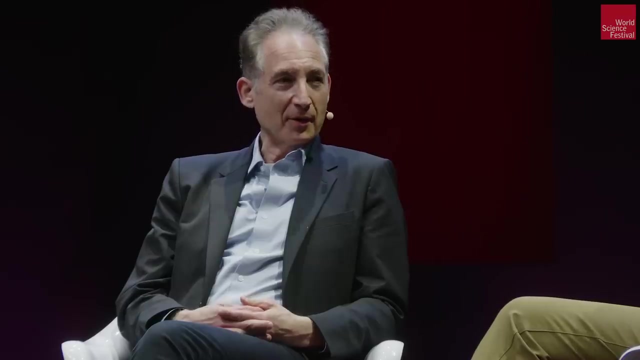 someone I trusted that could fit in there, My then 15 year old very skinny, Very skinny son Matthew. So I taught him how to use a scientific camera and scale, Sent him through, went through with him, sent him down. Was dad at all concerned about this? 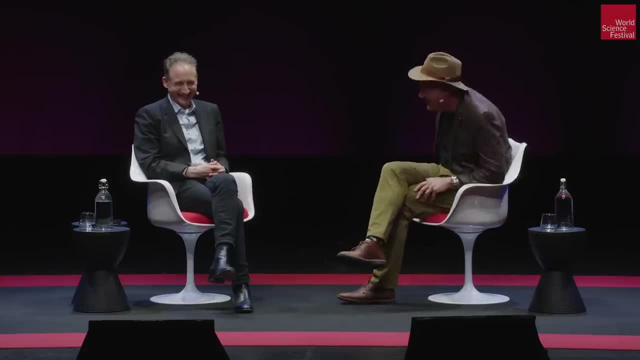 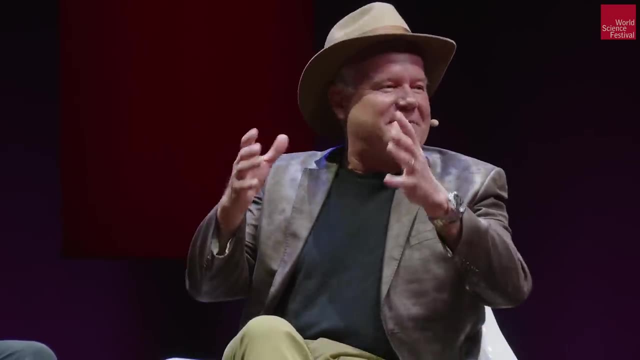 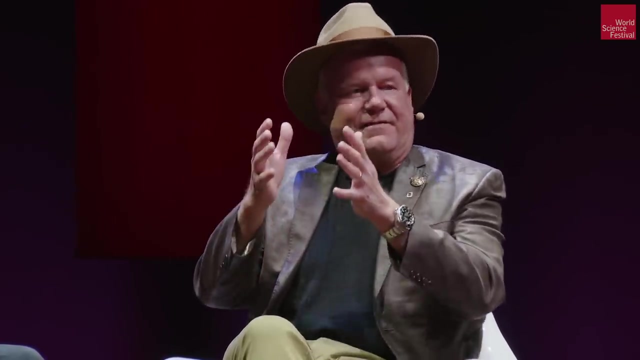 Did he damage the camera? Oh man, His mother didn't know, So their, I am seen in the dark. He's down 30 minutes. He comes back up, Has a camera, camera. and you know, as his head emerges from this death defying thing, because I'm going for father, 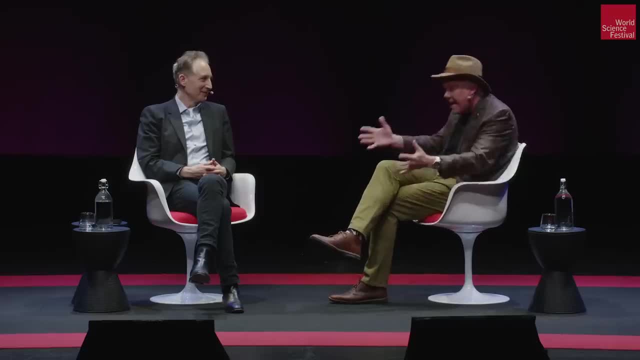 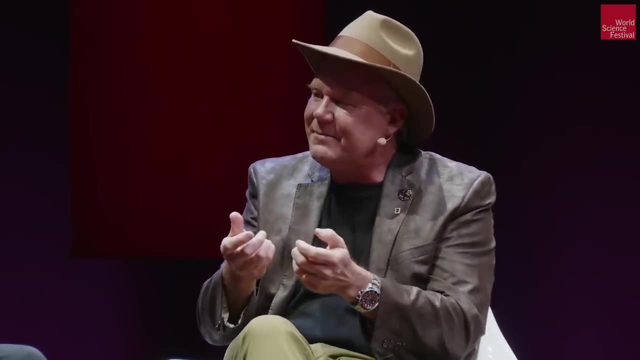 of the year. you can all tell there I didn't go. you know, are you? okay, I went and and he goes. he turns around. he said, dad, it was so beautiful, my hands were shaking for three minutes before I could take a picture. and he shows me the back of that and there they are. it's real, so I go out that. 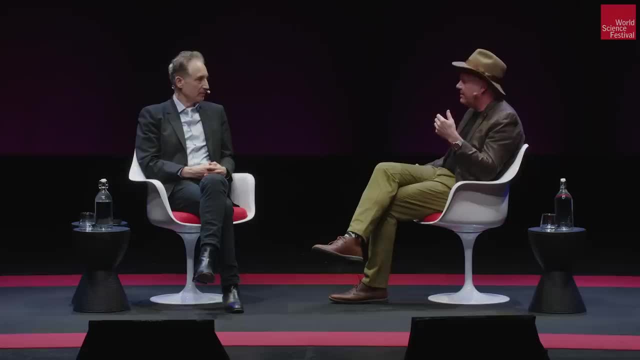 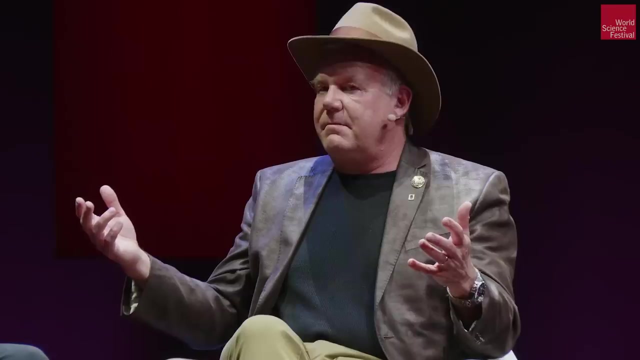 night after coming out of that terrible thing and I'm like: how am I going to do this? I need people. I need people who can climb, they're skinny, who have degrees and PhDs and can excavate precious material. how am I going to find that? and now, of course, the amateur community knows about this. 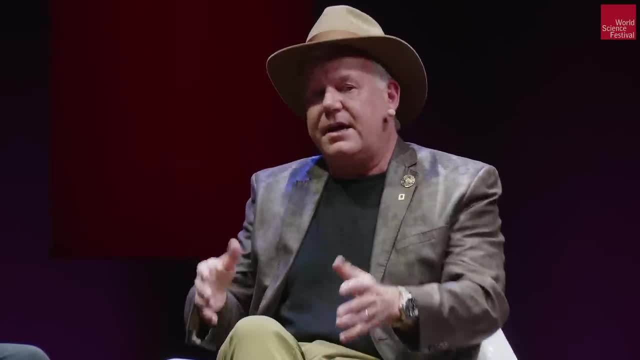 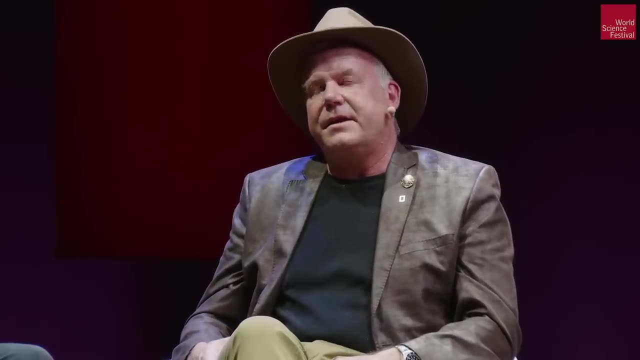 right, you're worried, I'm worried. yeah, they're just lying there. I mean you can't close this off. I mean it's a. it's not even on my land. you know it's on someone's land, yeah. and so I'm thinking: how do you do this? and so I guess I did what anyone would do. 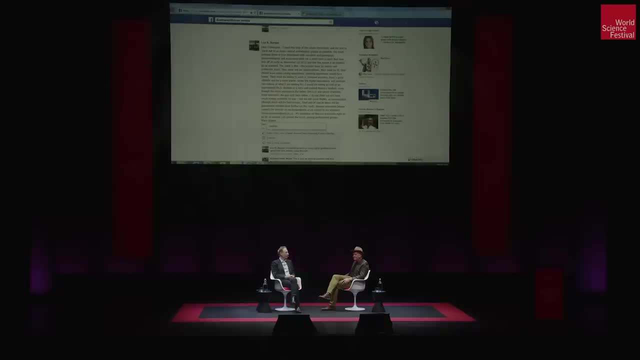 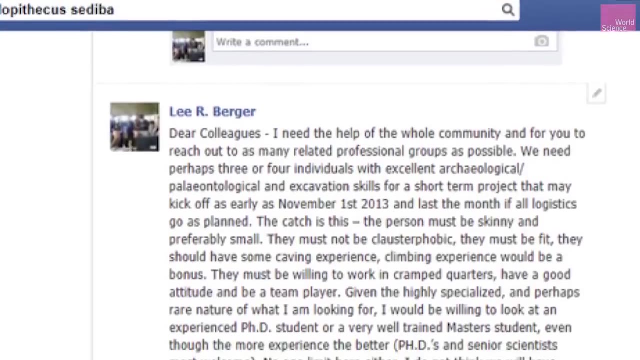 you. I put a Facebook ad out. you don't have to read that. it says: I need skinny scientists that are willing to drop everything and come for an expedition. they have to have a PhD or equivalent or be studying for one. they have to have excavation experience, climate experience. 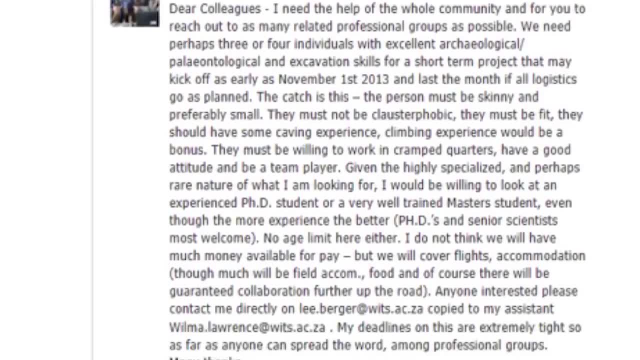 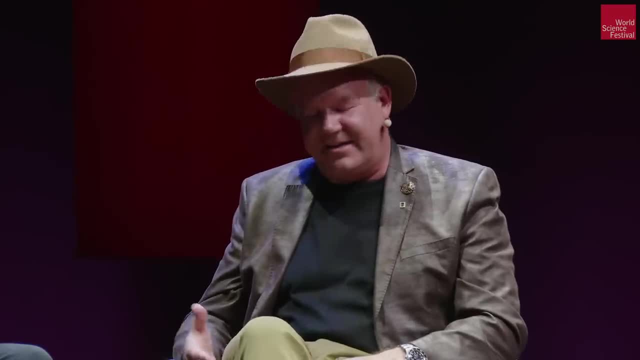 caving experience, not claustrophobic. work well in teams, are willing to work for free and I'm not going to tell you what you're going to do and you're going to risk your life. and I sent that out and I thought you know there are three or four people in the world. 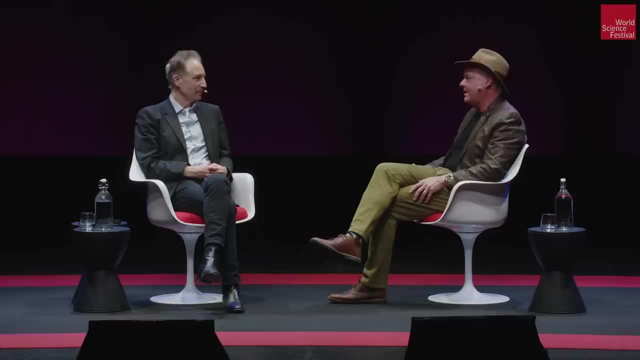 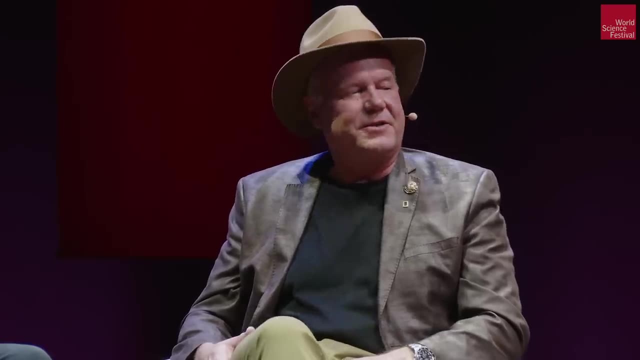 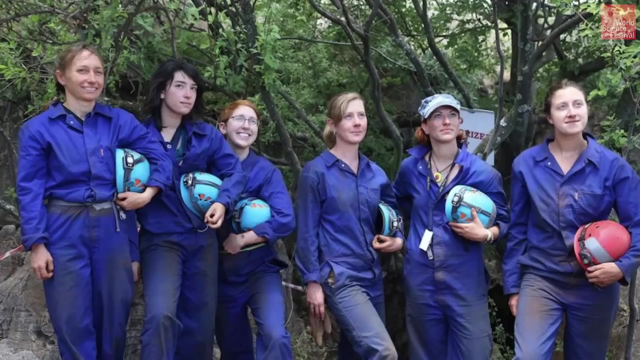 my, my, my. I got 57 qualified applicants, of which I selected six of them who were the most qualified, who just happened to be young women, and they were extraordinary, and we launched what was called the rising star expedition, after the cave itself, to get these things. I designed this whole system, this. 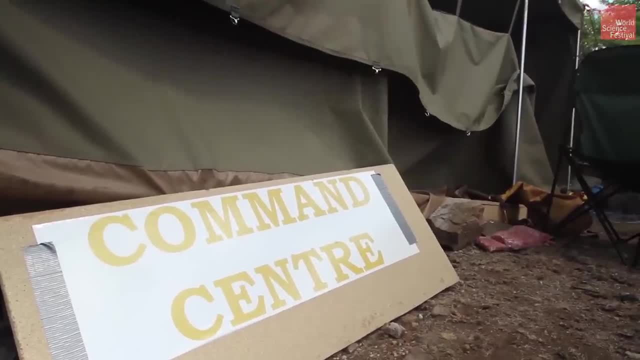 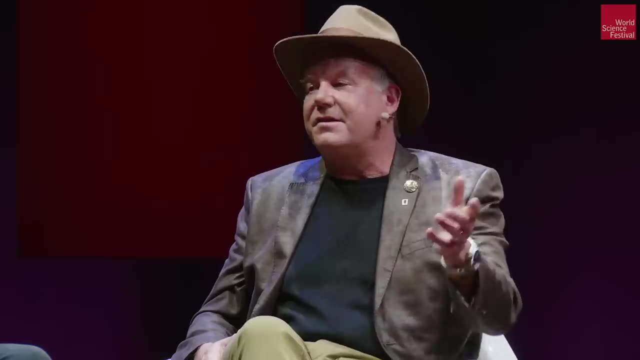 NASA like system, you know, with a command center and three and a half kilometers of cables, with security cameras and all that. and I was like, oh my god, I'm going to do this, I'm going to do this, doing it, And we started this expedition And I also decided, by the way, to live stream it to 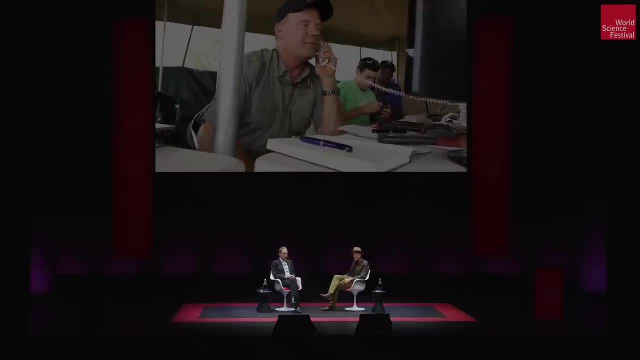 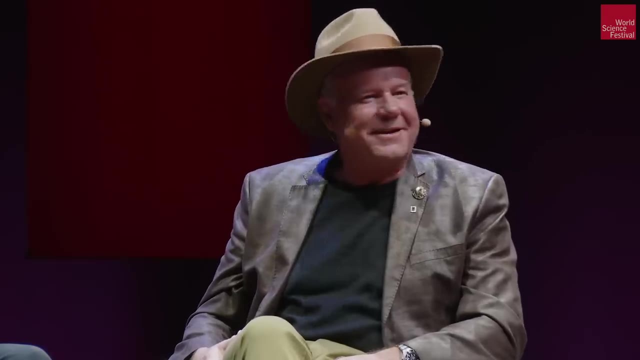 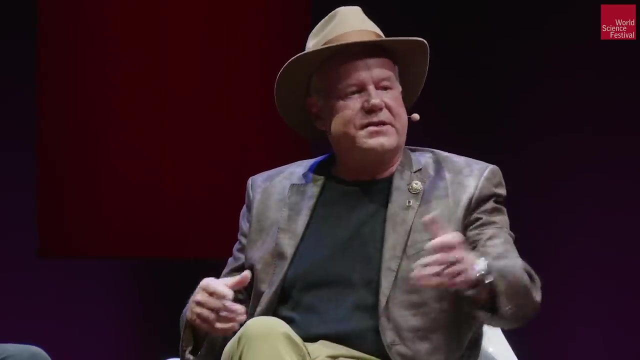 the whole world. I had a million followers by the end of this expedition Day two. we knew I was wrong. It wasn't a hominid skeleton. It was more than one hominid skeleton. We had three right femurs By the end of the week. we had brought up from underground in these extreme circumstances. 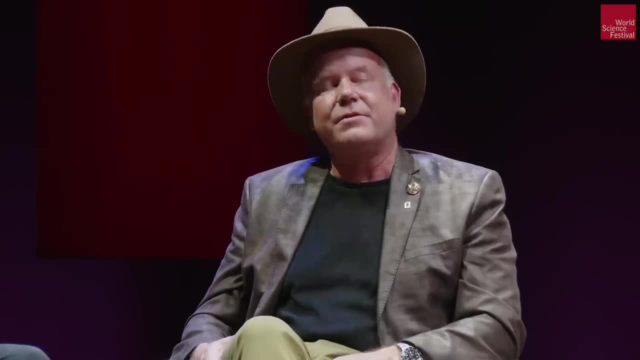 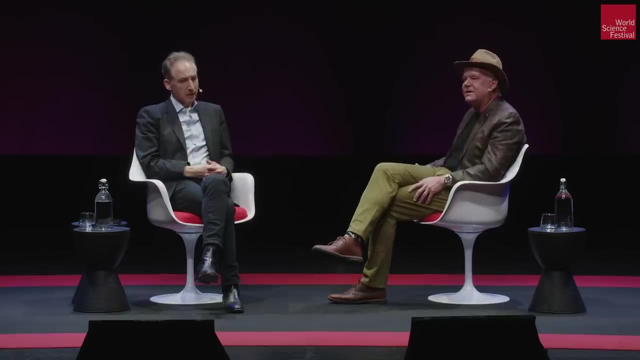 more hominid fossils that had been found at the richest site in the world to that date- Sturkfontein Caves, which was a kilometer away One week. It'd taken 90 years to get that Sturkfontein By the end of an expedition at three and a half weeks we discovered the richest. 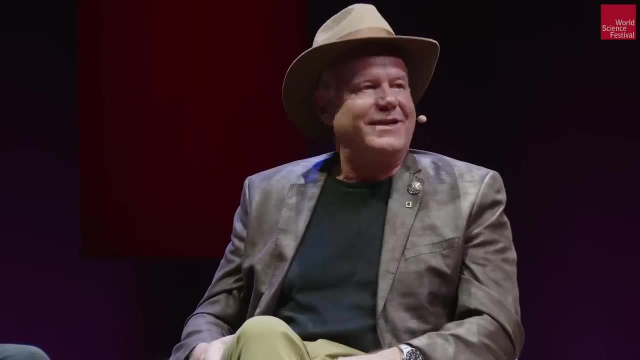 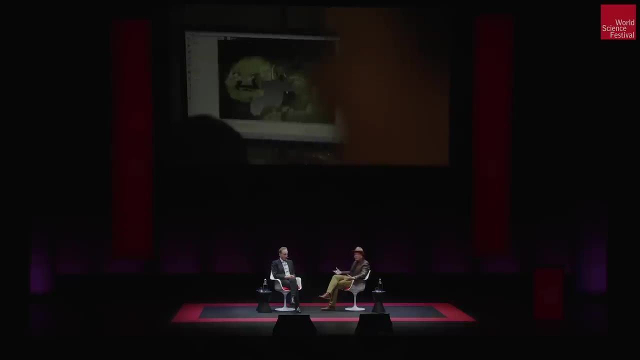 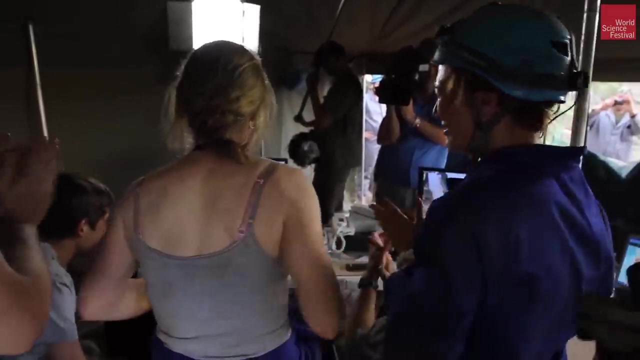 series of hominid discoveries in all of history. In the middle of it we were just. everyone knew this was like. it was like a moon moment. You know you can see the emotion, I think, on the faces. We were just in awe of this moment that we were in. that discovery was happening. 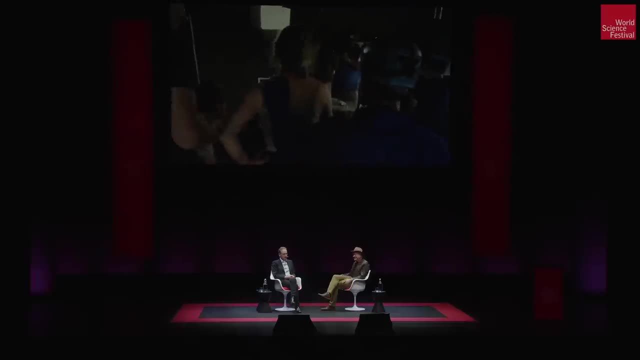 And you know this was like scientific nirvana. You know it's, and you'll see the kind of conditions they were working in. you know, deep underground, This is what they were doing in these spaces. They were incredible, They were heroic. I one time, during an interview in that period, 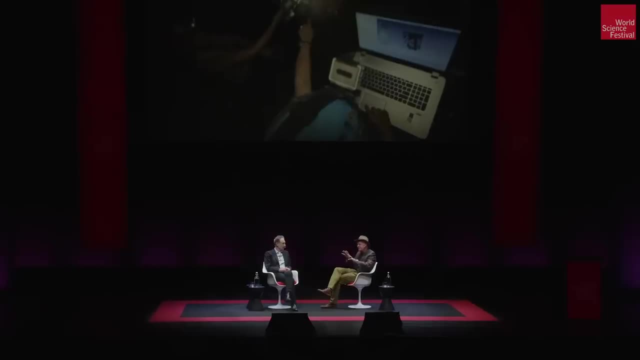 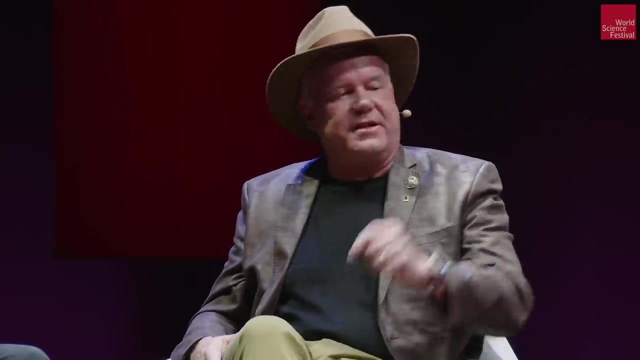 I said: you know, I'm looking at these, I'm seeing them on these images. They're like astronauts. They're so remote from us when this happens. They're like underground astronauts. Boy, I wish I'd never said that, Because I hate. 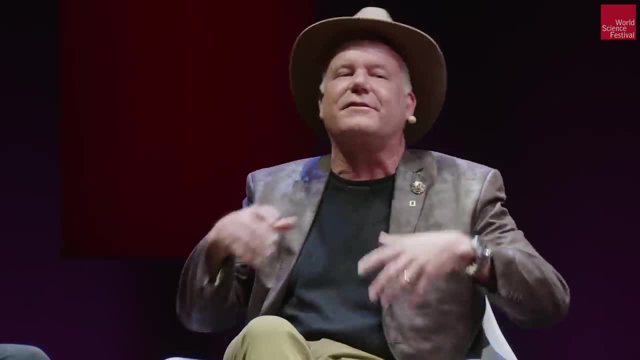 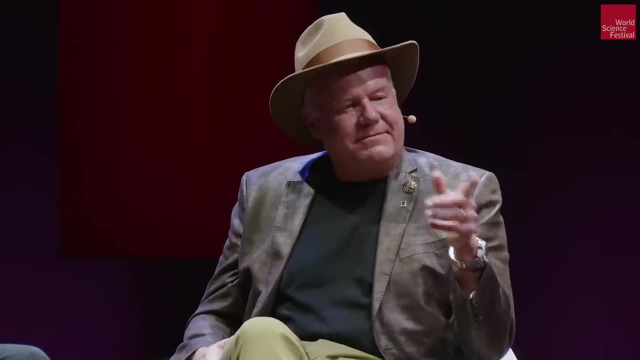 I hate to say it, but I hate to say it, but I hate to say it, but I hate to say it. And I said it and it caught on, And then I got in trouble for it, But it stuck And, and you know, 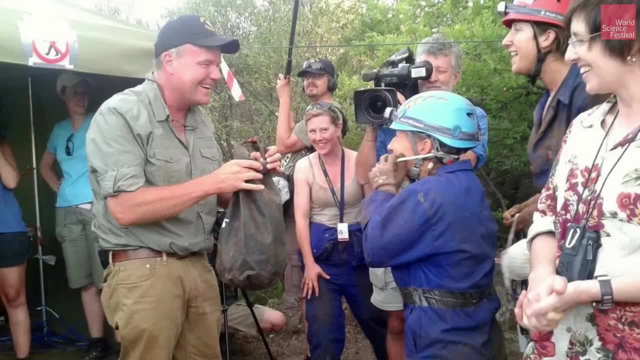 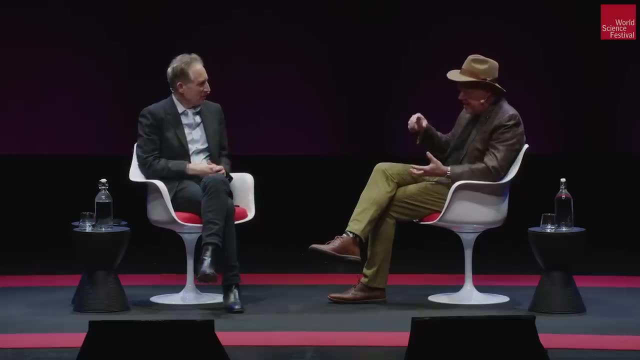 you can see how big they are. by the way, Look at Becca here. This is the kind of size of people that get into these spaces And how do they carry the bones out? In little tiny bags inside of this. really, we had this hugely complex development that I'd done of Tupperware. 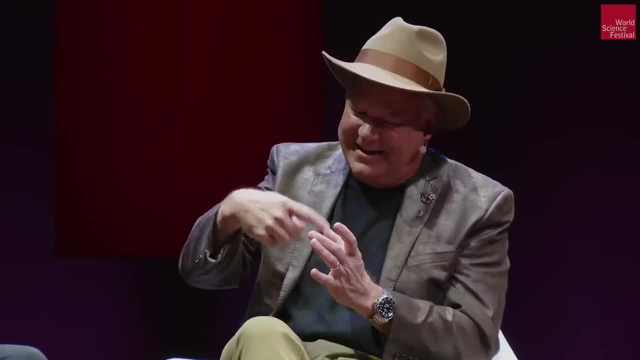 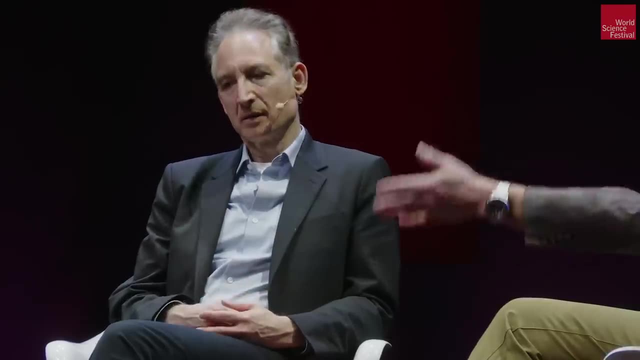 You closed and put the thing in in foil and then in toilet paper, inside of Tupperware, inside a waterproof bag and hand carried out in a sort of chain We would go. the lab suddenly got busy and scientists started flying in from all over the world. I think you can see a picture of 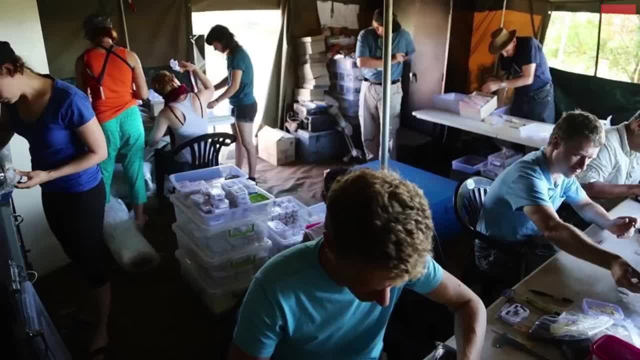 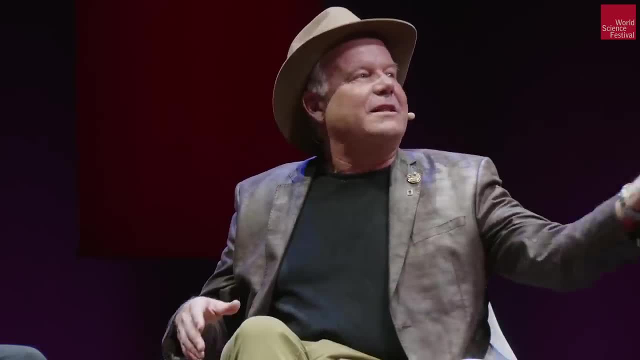 the lab that we, we, we constructed. coming up there We would work all day. People were, all these scientists were arriving. It was so cool, It was live science happening in the middle of the world. We were working late into the night. I mean, you know, you, you, there's some images. 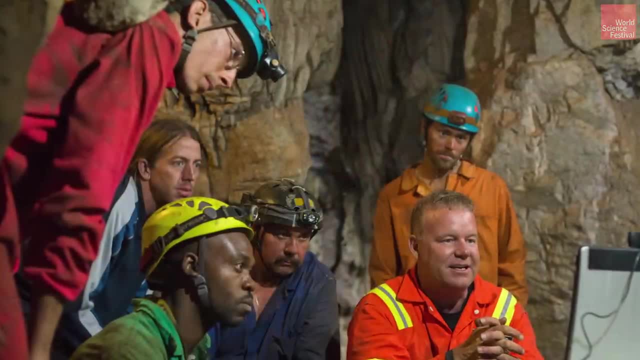 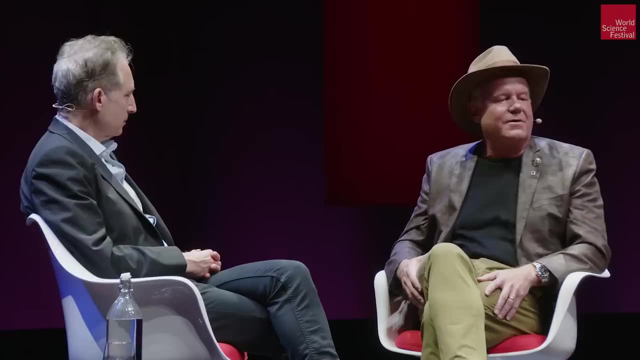 I think of us in at night, in there, And you know, all this time we're watching these images of them on the screen, going back and forth, back and forth, And we're working for hours and hours and hours, And it was unbelievable. These are the kind of images we saw. I mean, this is, this is. 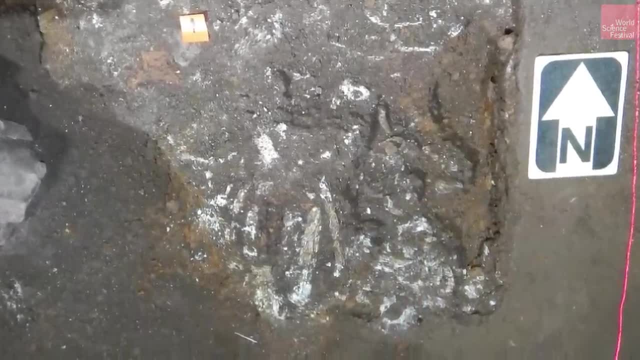 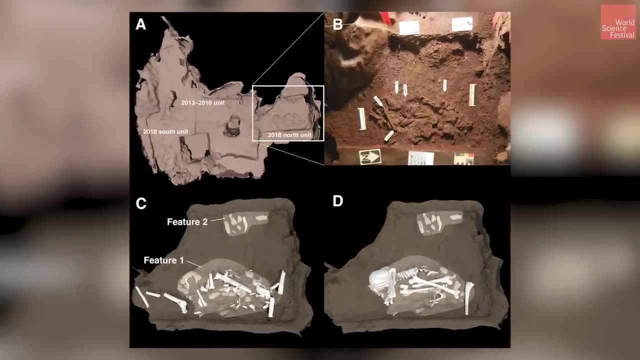 incredible These you see these images of. that's the kind of thing that you're watching. I would spend the next seven years staring at images like this, this place. I just want the audience to know that I am an equal opportunity. 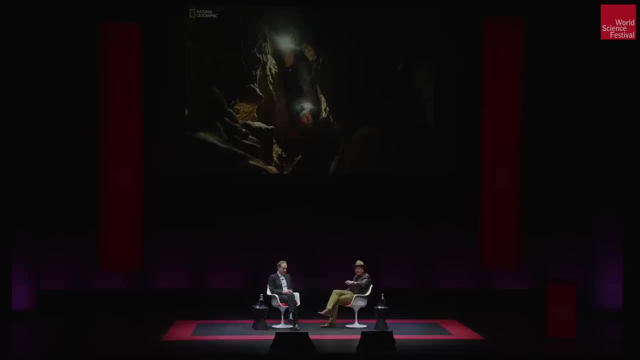 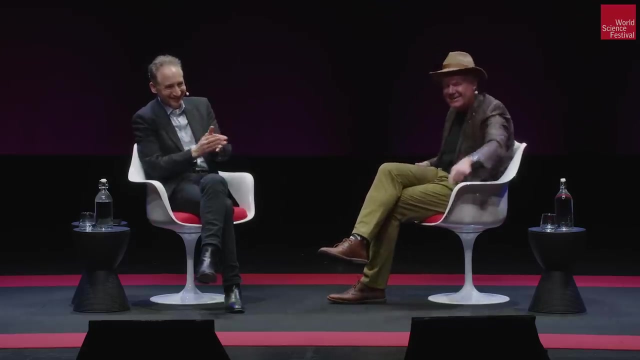 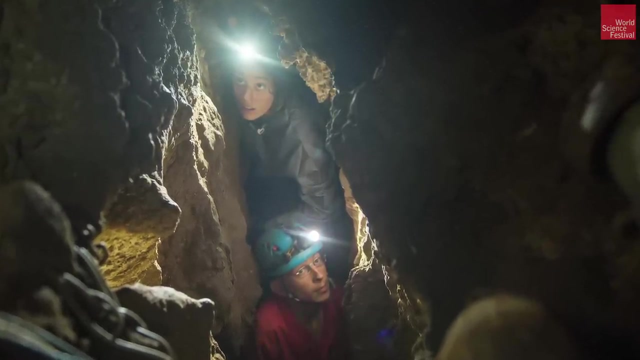 child abuser. That's my daughter, Megan, who's in the audience today. Somewhere here She's University of Queensland vet school. right here, That's a position called shoot troll. She's up at the top there And her job was to go up and down the chute. I used her to test the 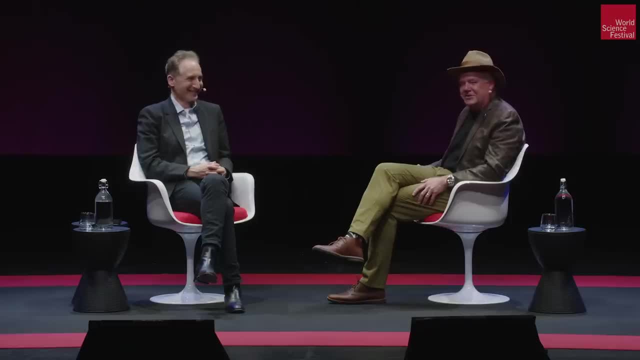 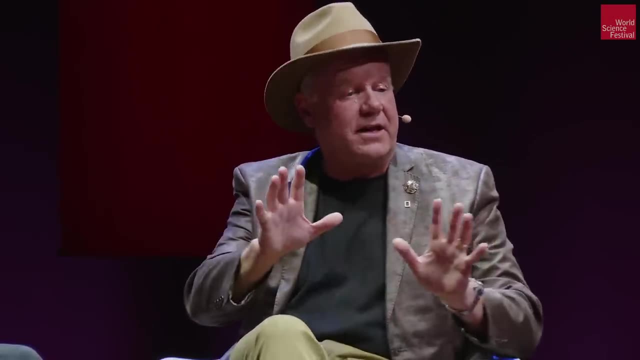 safety equipment before I sent the aspirin. I didn't tell her mother that either. Look, I'm sending other people's children in. I need to be able to risk my own And I'm serious about that. I was taking other people's kids into the extreme spaces Into that expedition. it was. 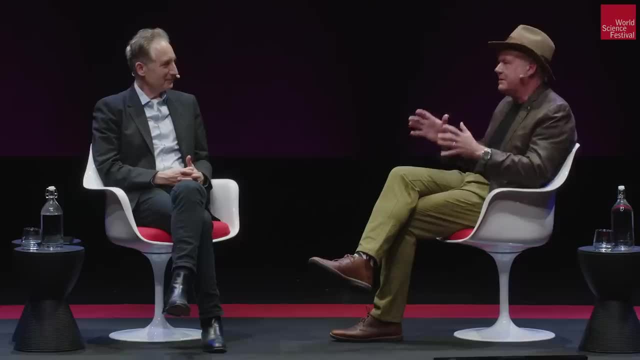 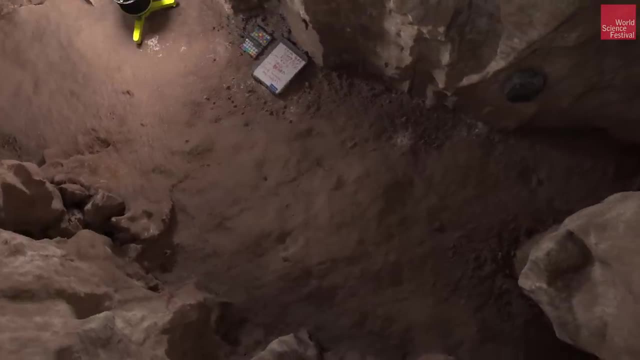 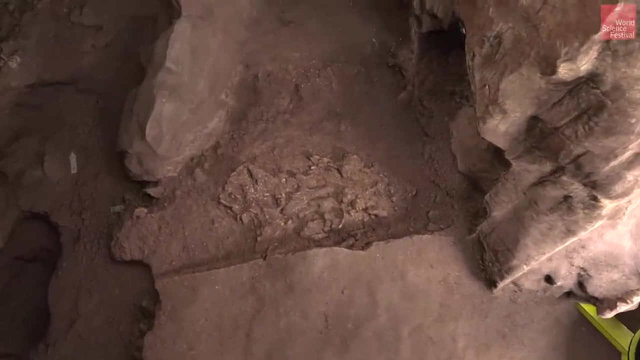 extraordinary, And you know from this little chamber, deep underground, a tiny space that's sort of 10 meters long by five meters wide, we discovered over 1,500 individual fossils from a one meter by 50 centimeter excavation- The richest single. put that in perspective, folks. 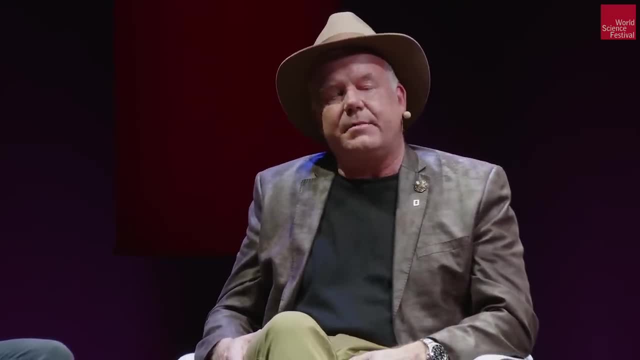 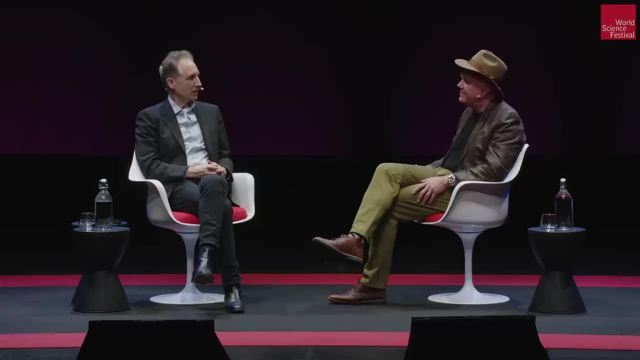 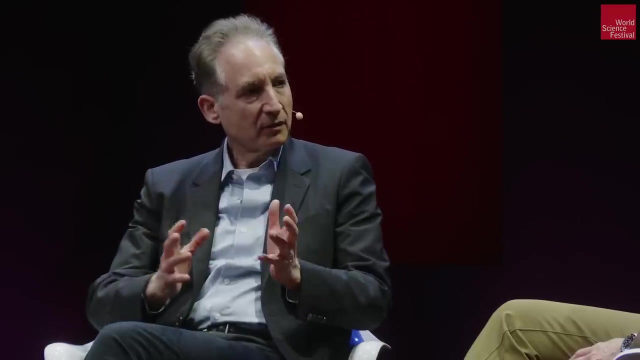 to that point in history In sub-equatorial Africa there'd probably been 1,100 individual fossils found, About 80% isolated teeth Three weeks- And there was clearly more of them in there- And could you tell how many individuals were? 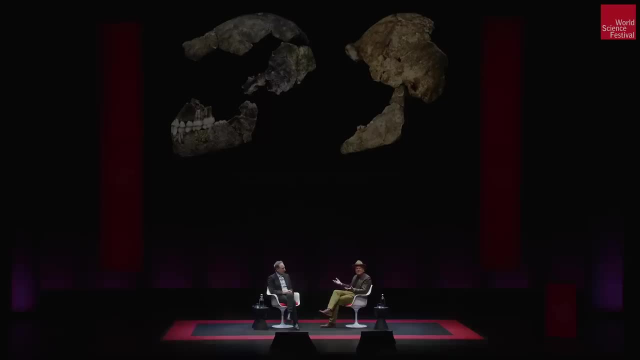 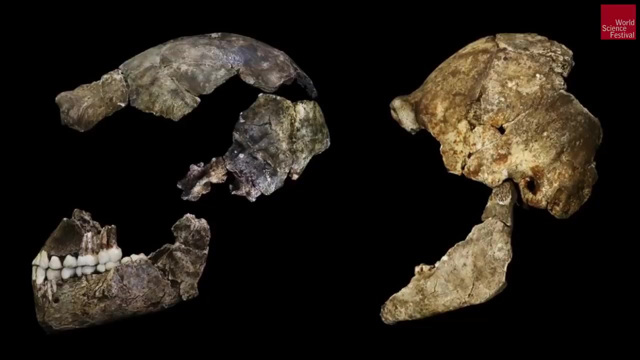 After we started looking at these fossils. you know we had skulls, We had actual skulls And skulls are rare. You know we had that one from there. We had skulls like this, you know, and we had slightly bigger ones and little ones. It was clear they were really weird And we had a lot of 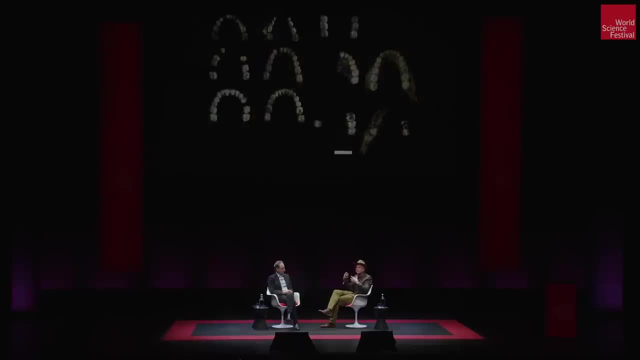 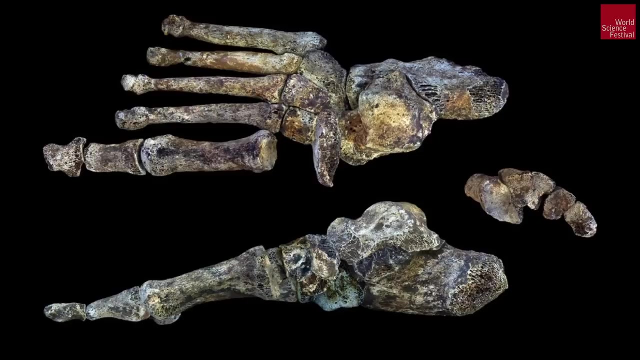 weird from it. We had dentition, We had, you know, dozens and dozens of teeth, We had foot bones. that were just completely things like this. You know you should go off for this, Because paleontologists around the world went holy cow. These are not the kind of things we see in the 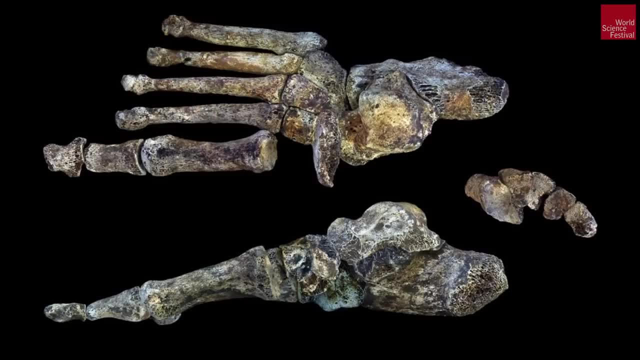 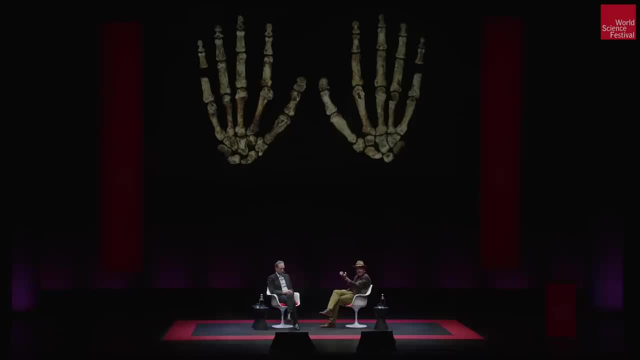 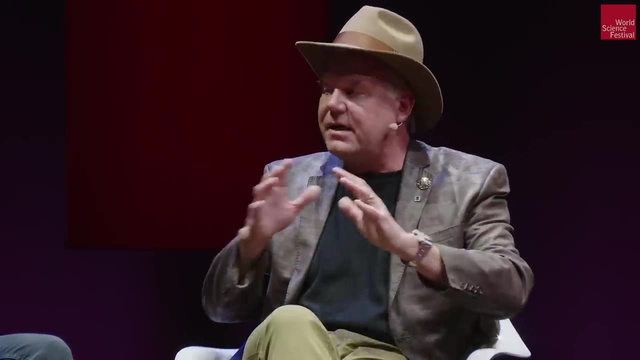 fossil record, You know the primitive hominin fossil record. We had hands that were actually sitting, articulated, Just like that one, Just like that. It was unbelievable and stupidly odd. We knew that as we were looking at it. You were looking at a. 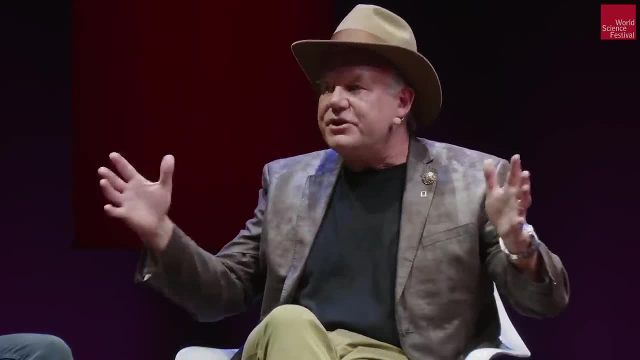 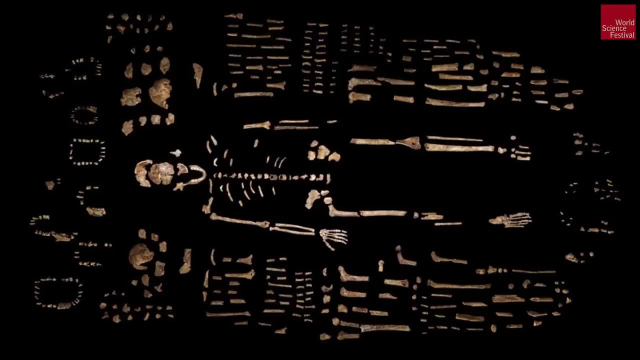 thing that was different. At the end of it we had this just assemblage. You could lay out just dozens and dozens and dozens and dozens: 1,500 fossils for 15 plus individuals. It was unbelievable. And then I got to play science. 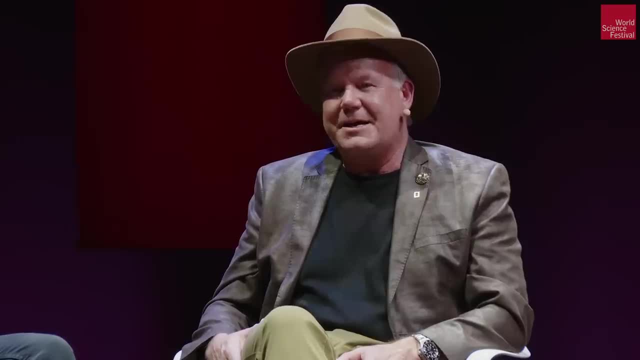 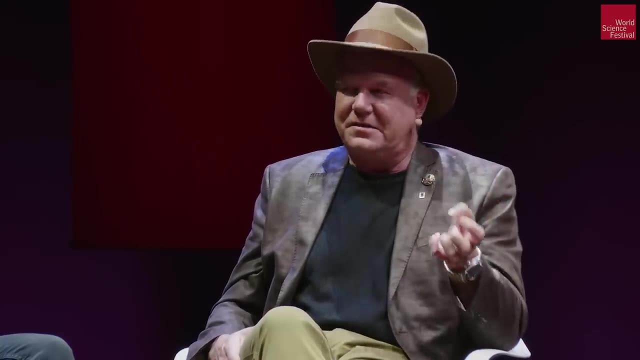 In terms of interpreting what the heck this is Absolutely, And I got to play science in a way that was really, really nasty. I said: you know, there was a thing in our field about you had to have experience to study ancient hominin fossils, And there was even someone who said that if you haven't studied one, 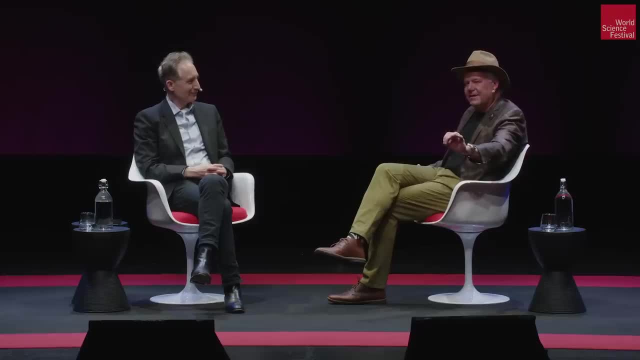 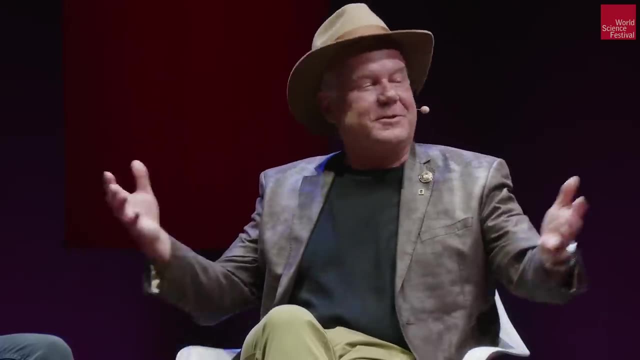 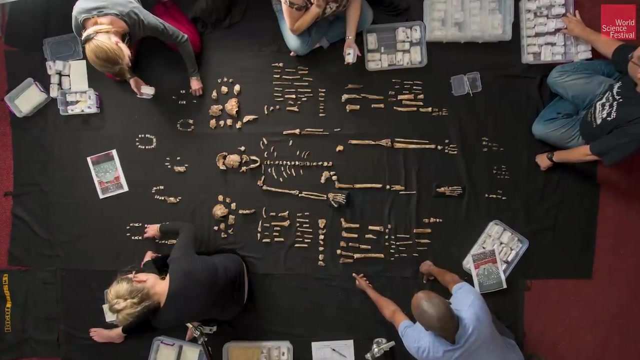 before you shouldn't be allowed to study another one. That's the shaker kind of mentality of of of you know science, where eventually you all die out and everyone just looks at the things, I guess, And so I I picked particularly young people from across, the very best and brightest. 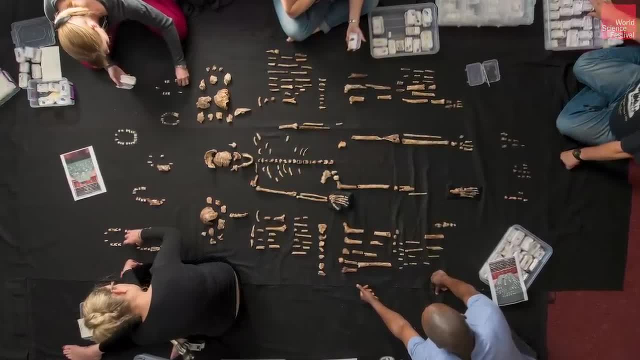 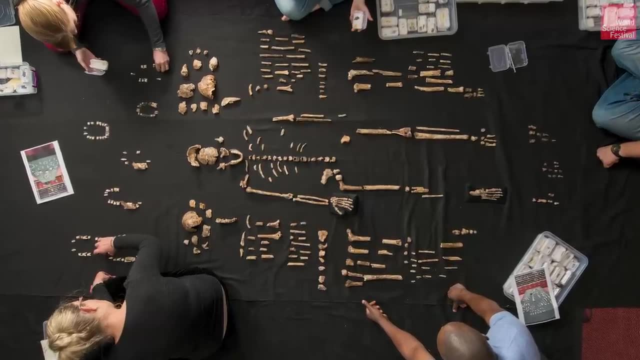 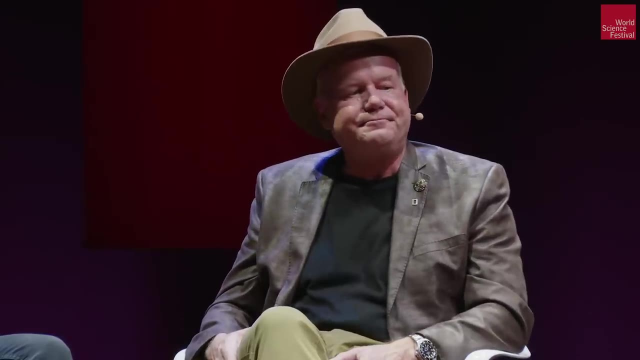 hugely diverse and brought them together as a gigantic team to study these, And we had the time of our lives. The only rule was they had to. they had to release all of their data sets to the team. So we shared data and made it open access across the field. And then we named a new species. 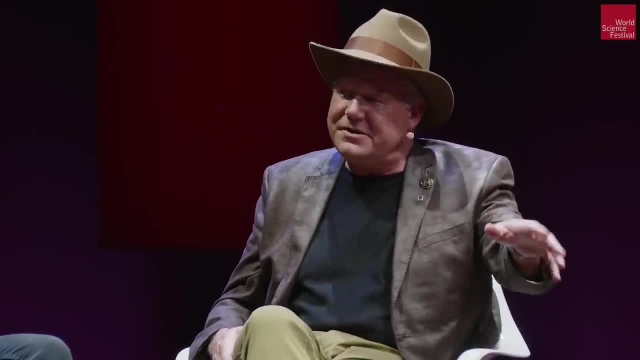 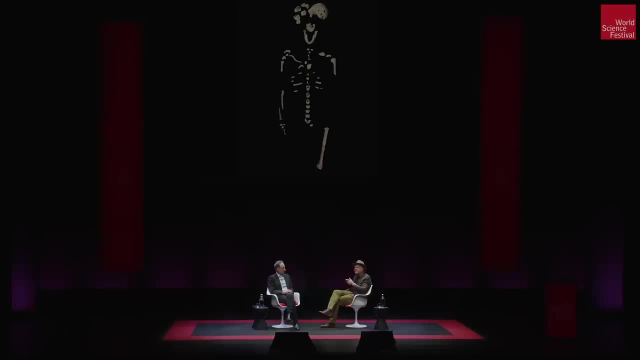 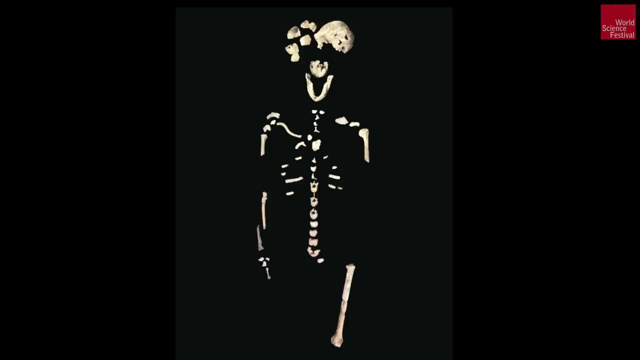 and started finding more of them, not just in that chamber but in other chambers nearby. We found a skeleton from a chamber 100 meters away that was in an alcove up on the wall. A beautiful thing, Maybe one of the bigger. 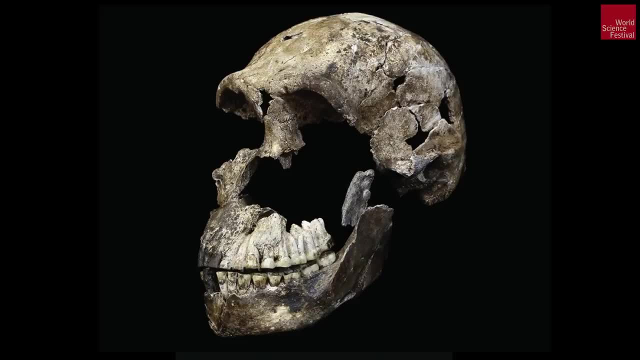 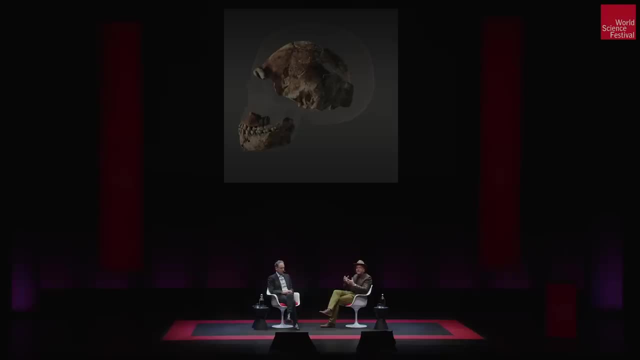 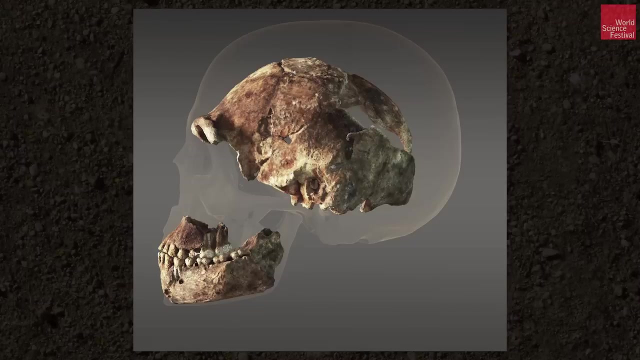 individuals. we found It had a beautiful skull. I mean, just almost the complete thing that you could look at. You can actually see this face and this tiny brain hominid, a hominid that had a brain about a third the size of a human. It was clearly primitive. There's one. you can see it. 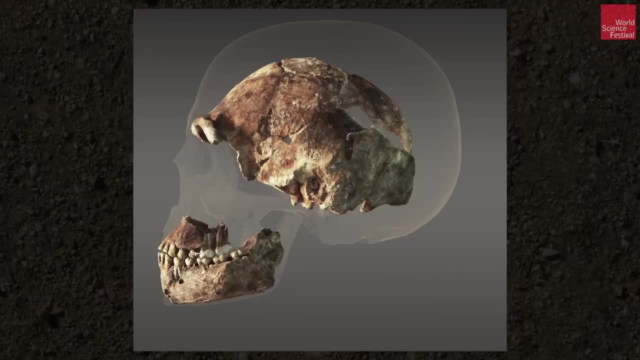 They had. they had this kind of rounded cranium, kind of like a, like a human, but they had these brow ridges that you can see there. They had a flattened face that was prognathic, That is, the nose stuck out. The teeth were small but primitive, like I saw in 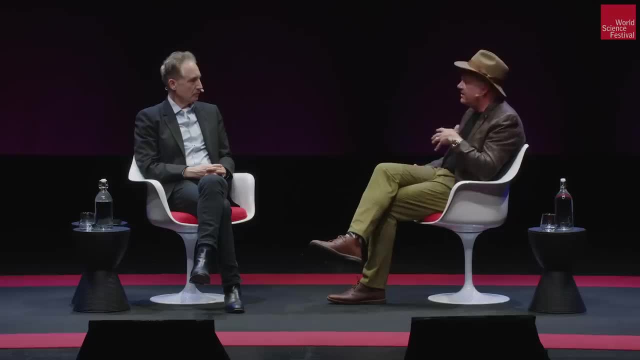 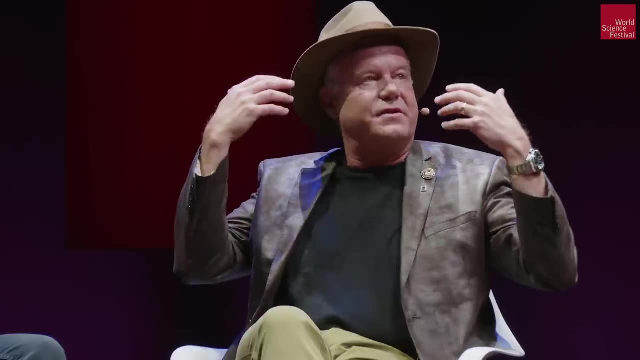 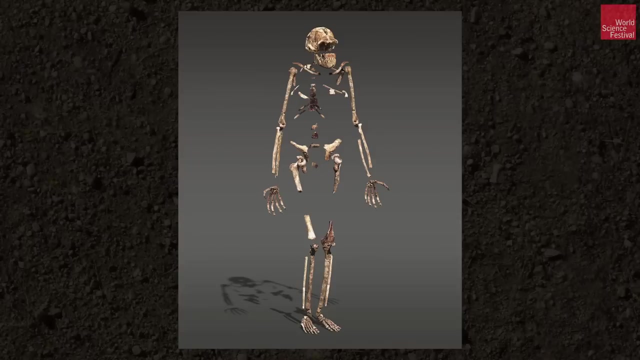 that first mandible, But that's where most studies in our field would have ended. But we had these bodies, everything from neonates to the elderly, And so we could begin to construct the whole anatomy, And what we saw was this bizarre mosaic creature. You know it had. it had shoulders like 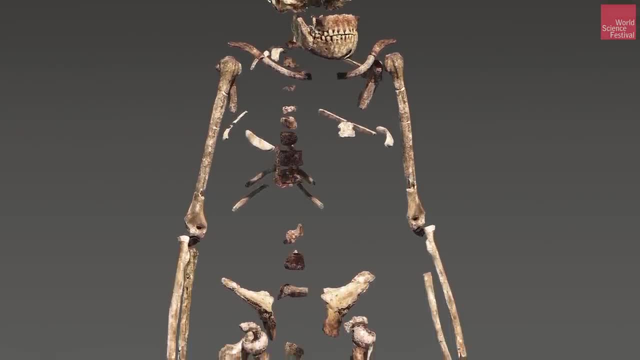 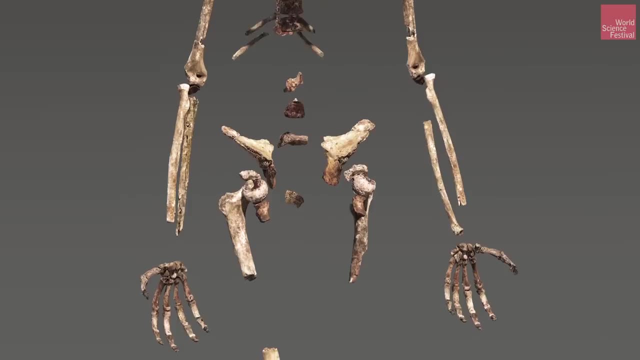 an ape. It had a spine like a mini Neanderthal, a pelvis like a hominid that was three or four million years old, like Lucy's pelvis, But then, as you move down the limbs towards the feet and the hands, they became more. 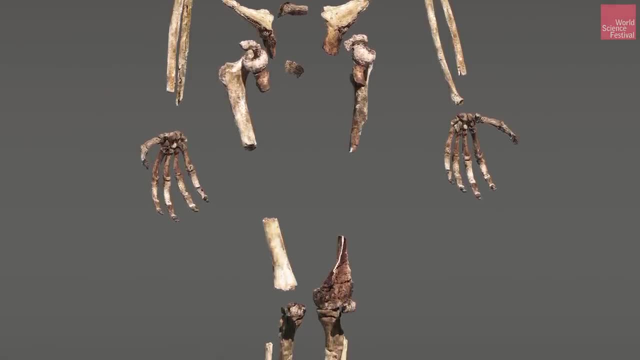 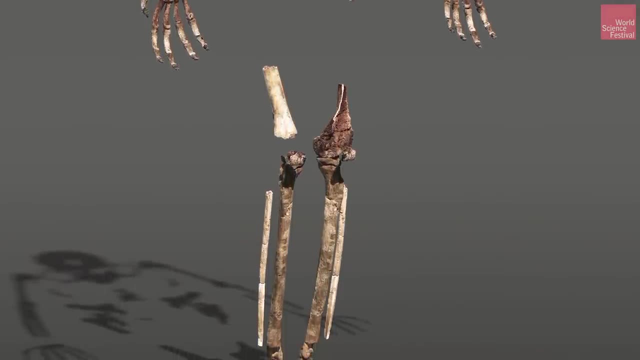 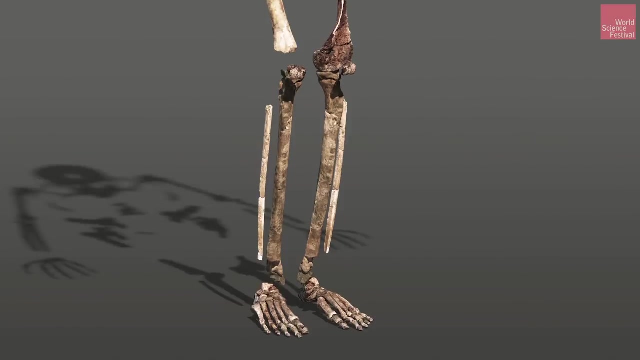 and more advanced, until you reach these hands, that while they were curved, they were almost superhuman-like, with really long thumbs And the feet. as you got to them, the long, skinny legs, and they became almost human-like, except for having slightly curved toes. It was like this mishmash. 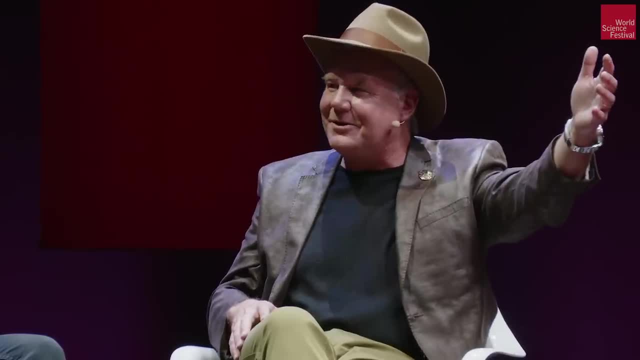 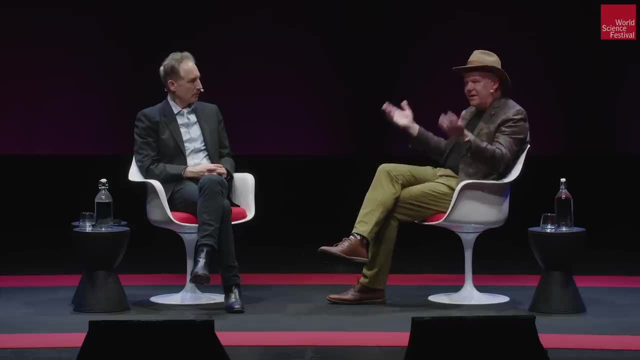 of everything, Every species that we'd found, from like three million years old to say a million years old. We would put it all together and we could look at this creature. You could actually see its physical body effectively and reconstruct it and compare it to other hominids, And so you got this visual. 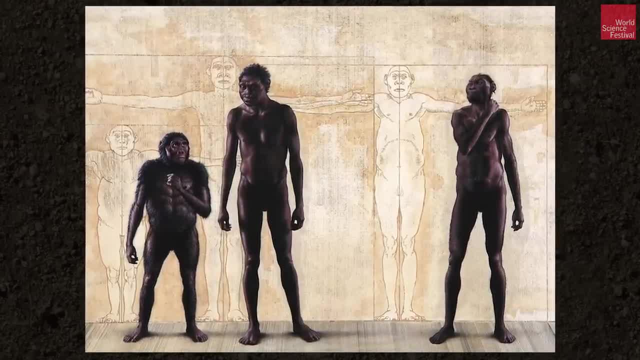 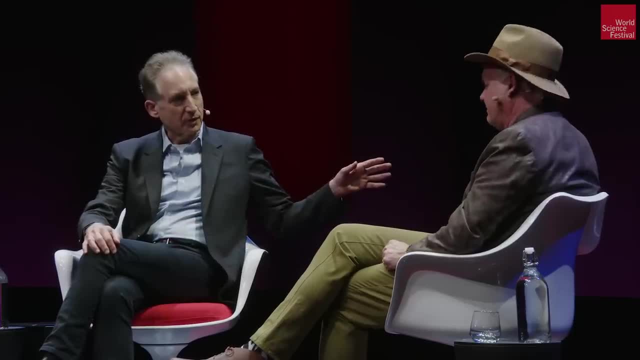 reconstruction of a of of this living creature standing next to all these other hominids. Now, if you just say: had the feet, you would have reconstructed it. You'd have a different looking creature. We would have said human, Huh. 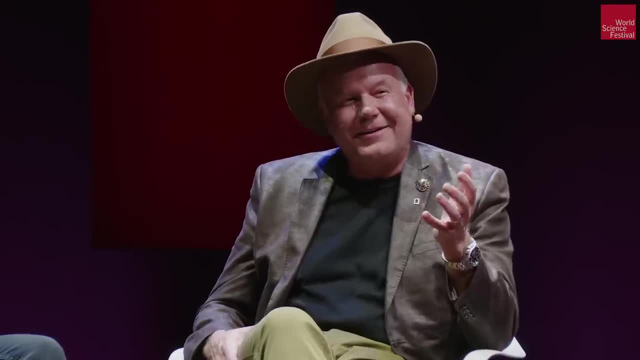 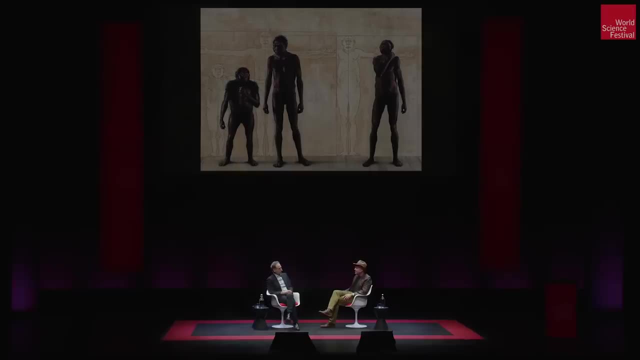 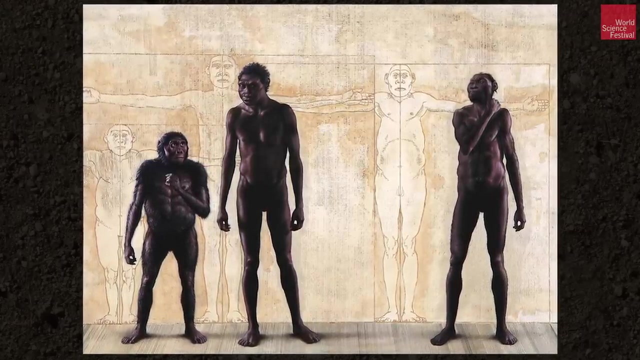 If it had hands, we would have said: funny human with a long thumb. If we'd had the teeth, we would have said: maybe it's a mini robust australopithecine or primitive australopithecine. If we'd had the face, we would have said: oh, that's, that's an australopithecine. If we had the 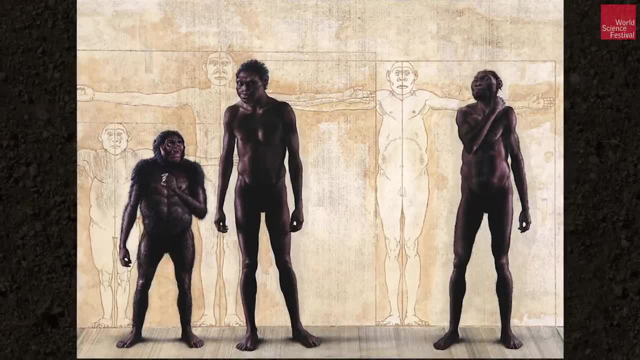 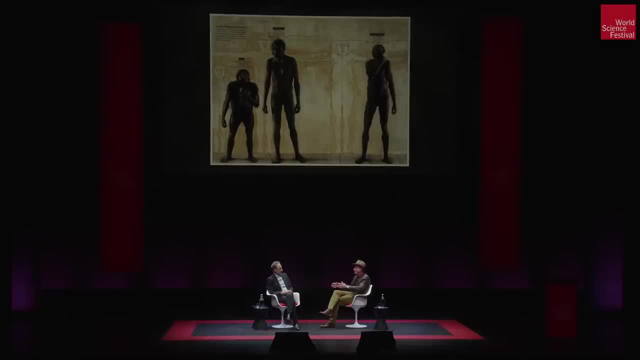 head cranium, we would have said homo habilis, Maybe a bit of homo erectus thrown in there. If we had the spine, we would have said funky Neanderthal. But there are no Neanderthals in Africa. So if we had the shoulders, I might've said gibbon. 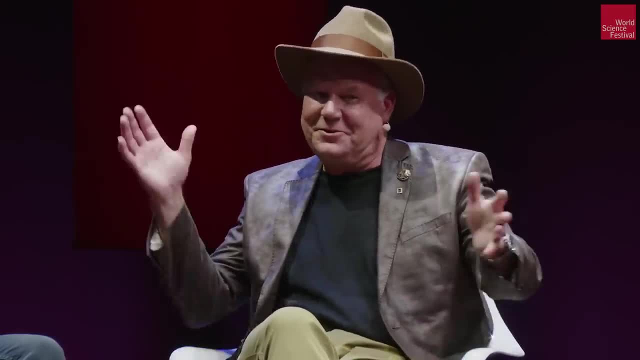 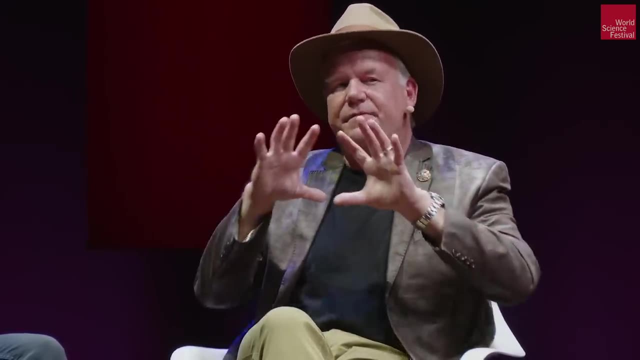 And so we did what scientists do time and again: we named a new species, homo naledi. We put it in the genus homo because of that head And because we felt the overall grade adaptation was to bipedalism and living on the ground. 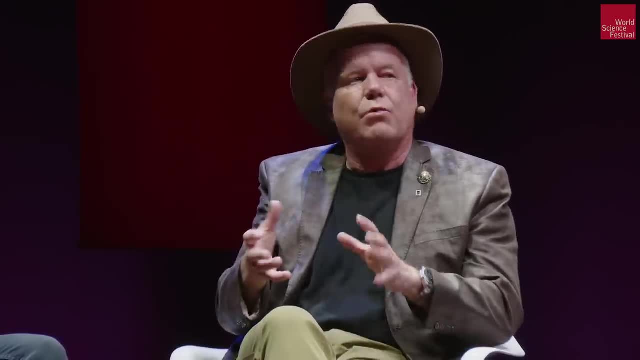 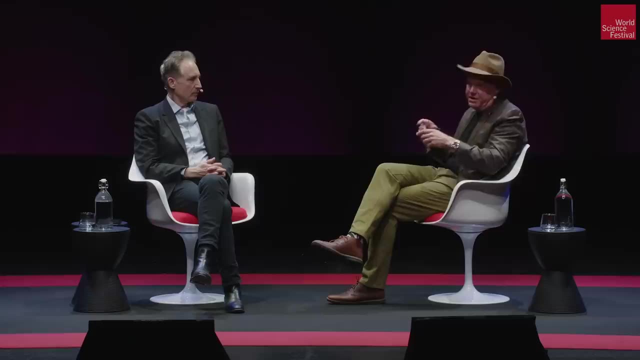 that this was in our ilk, More so than australopithecine, but we debated it a long time. It hovered there on the edge of both sides. depending on what part you looked at, You know we could build it. This is when John Gurchi's great reconstructions 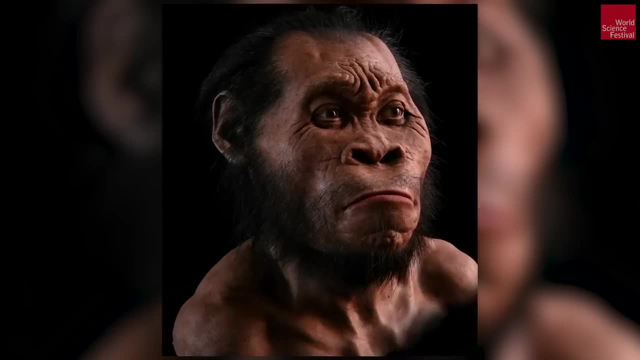 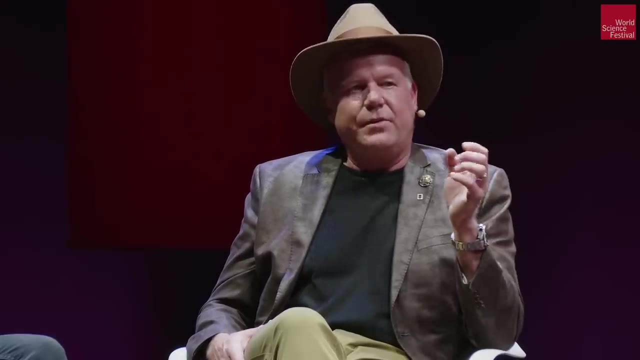 We could build this whole image of this guy And that was so exciting because maybe people in the audience- I bet some of them- realize that we didn't get to do this with certainty before this moment. Almost every other discovery you've ever heard about in this. field is built from scraps, and often built from scraps that we are not a hundred percent sure about. And there are other things that we are not a hundred percent sure about And we just have to turn it around, because it just sort of becomes that way. 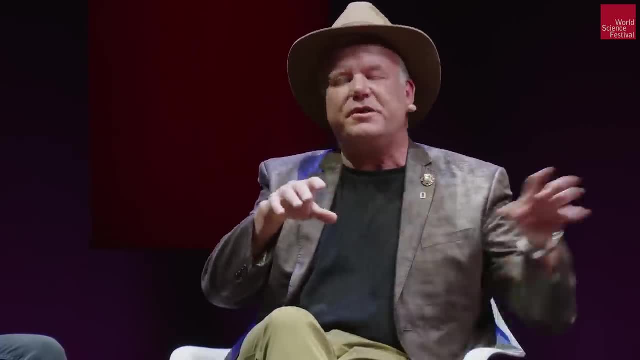 And if you look at the found in the field, there's a lot about this And so it's not clear, but I'm trying to get a little bit more into this. often built from scraps that we are not a hundred percent sure belong to the. 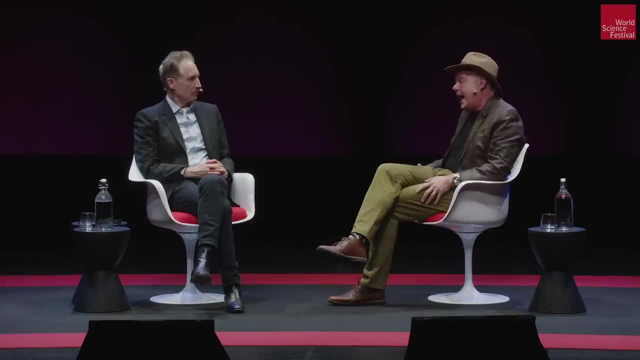 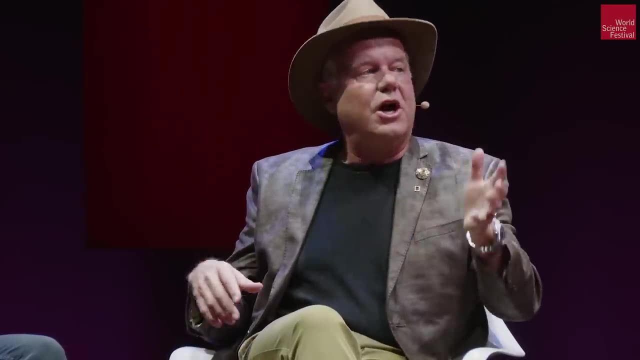 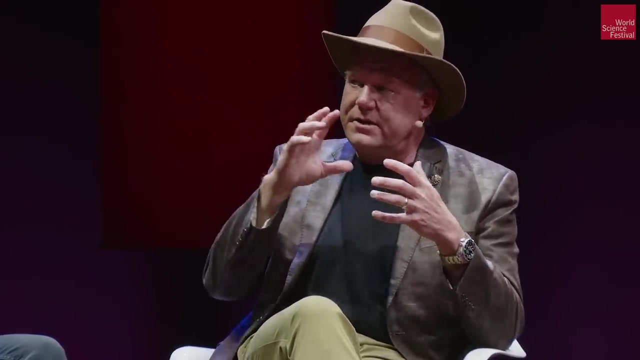 same thing, and with the exception of- perhaps, I'd argue, Neanderthals. we just don't have a highly diverse record of young and old, and so the ability to build an image of one of these, and then lots of them at different age groups, and the ability to understand them was was truly unknown at that time, I mean you. 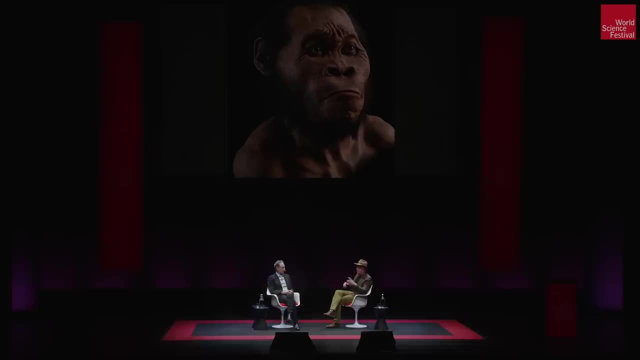 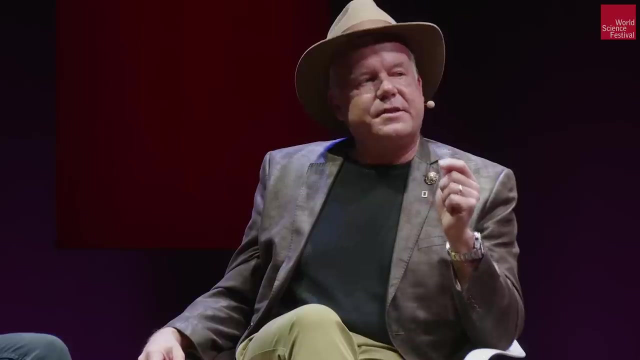 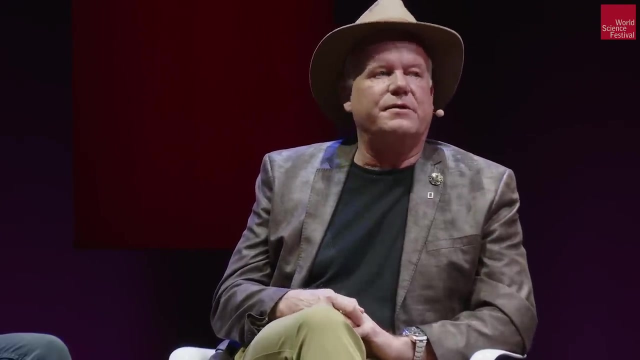 know Australopithecus sediva and Malapa had been extraordinary, but it wasn't. this, this was that on steroids and we were sitting there with this knowledge that something weird was going on. and here's what that weird thing was. by the end, the first week as we were sitting there in this command center, you imagine 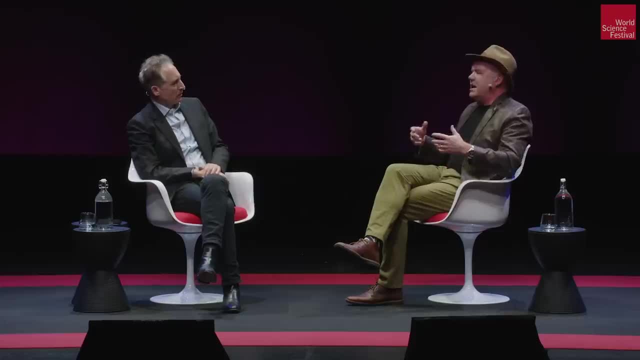 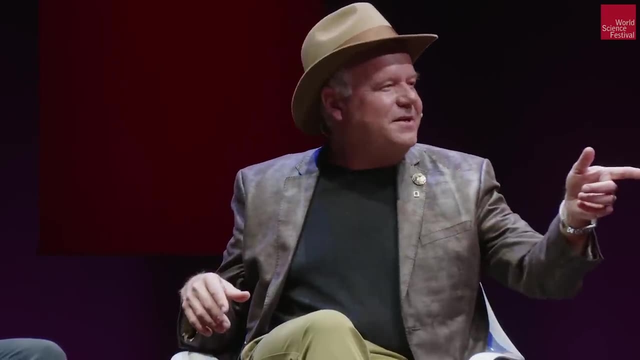 everyone and you saw the emotion on everyone's face, which is like I had to buy. there was a joke going around during the expedition of: you know, we're gonna need a bigger vault. you know, remember that scene in Jaws where the shark comes on he goes: we're gonna need a bigger boat. we. 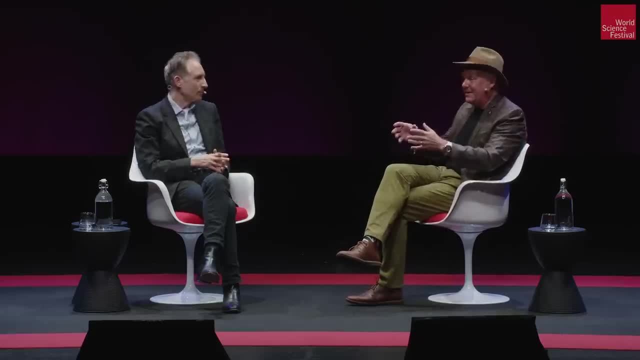 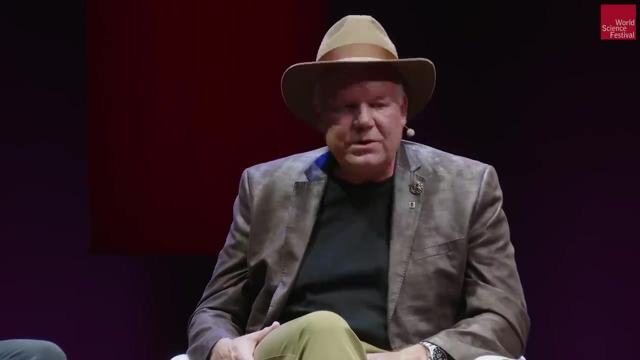 need a bigger safe, because we'd brought these safes out to keep the, you know the five pieces. we were certain we were gonna find we had 400 by the end of the thing, and but what I didn't kind of highlight was we had only hominids only. 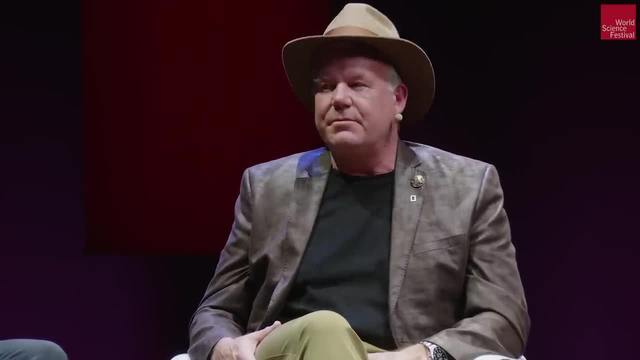 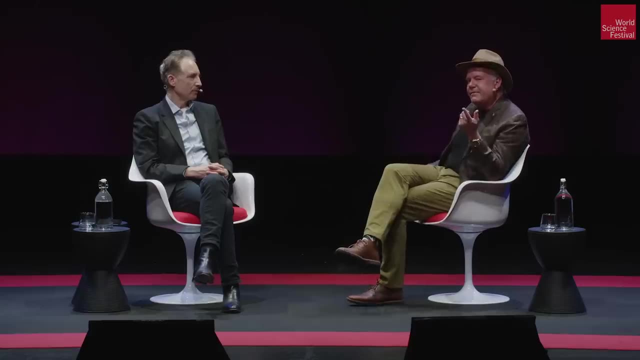 hominids. from those deep chambers. nothing else was coming out, just these fossil human relatives. I remember very poignantly at the end of the first week. you know this is all happened to us. at the end of the day he's filthy underground astronauts come out. one of marina had brought out the last bit. I 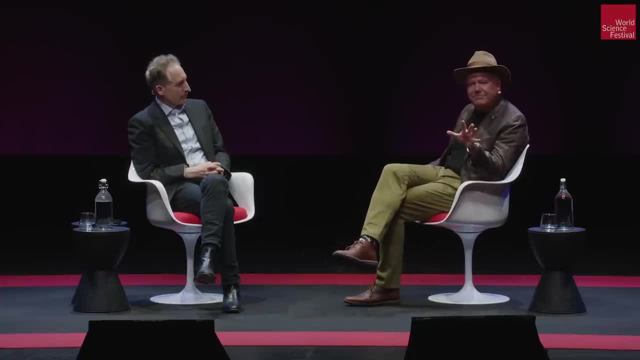 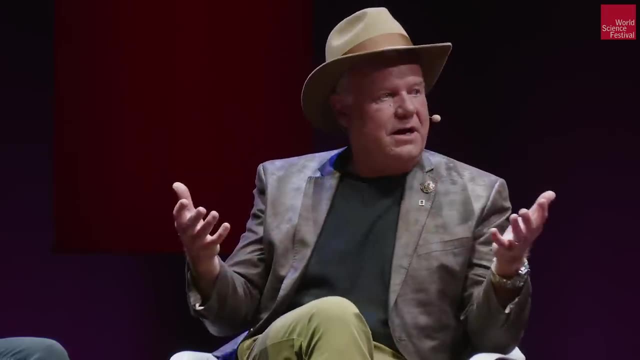 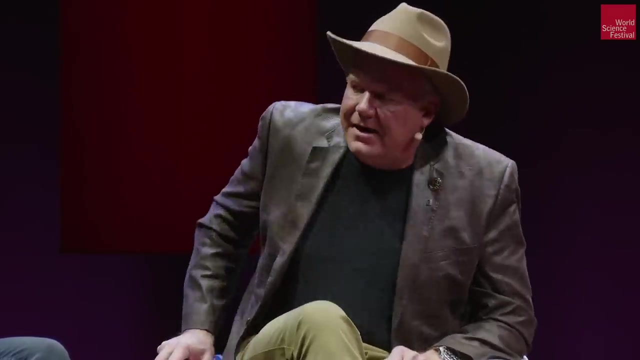 look at it and it's all hominid. I said: are you guys cheating? are you actually picking up only the you know and leaving the you know the animals behind? and they went. nope, we're taking them as they come and over beers that night with a couple of scientists. I remember this really powerful. 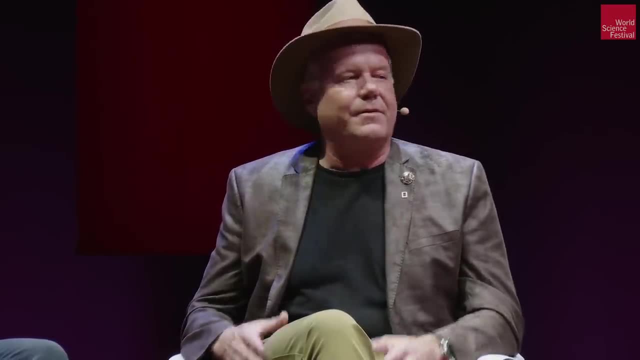 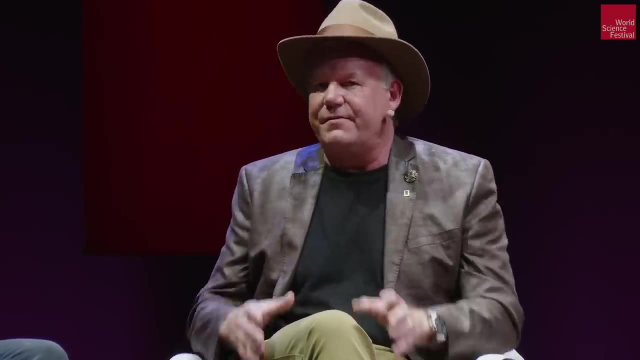 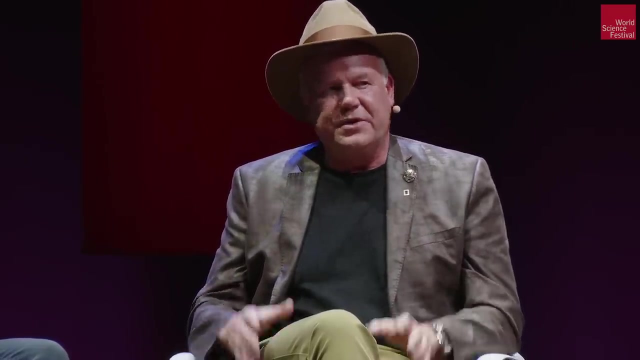 moment that was occurring, because you know all of a lot of us had trained in lots of things. I was a geologist, an archaeologist, and part of being an archaeologist you train is sort of forensic anthropology, and one of the things you learn as a forensic anthropologist when you're 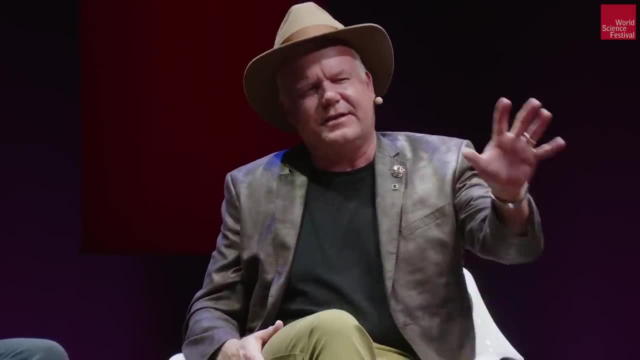 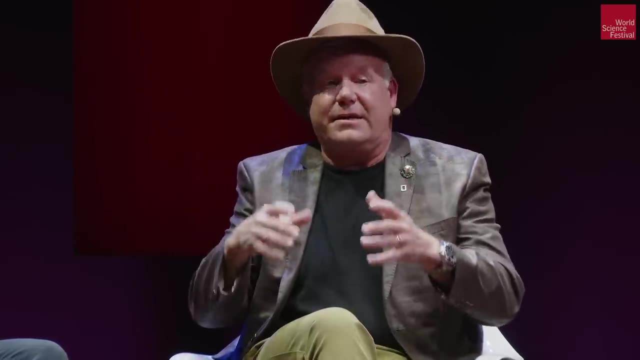 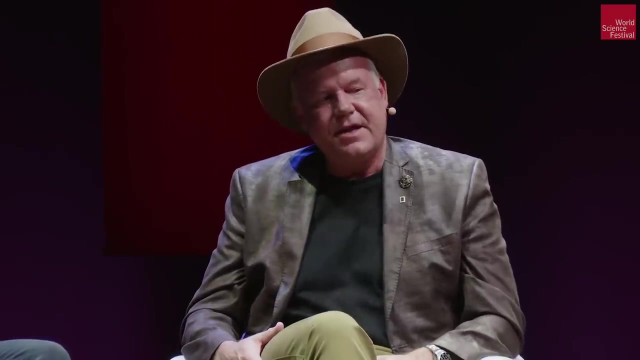 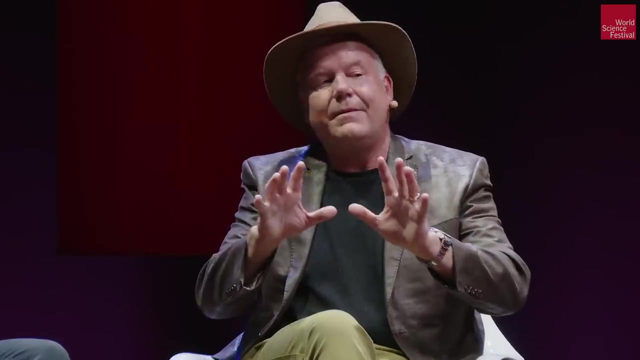 studying natural occurrences. whether they're collected by carnivores or catastrophe, they're always mixed. you get animals and everything and in fact in the hominid record it's like 99.9% animals, 0.1% hominids. we had never seen a situation that was all hominids. well, we. 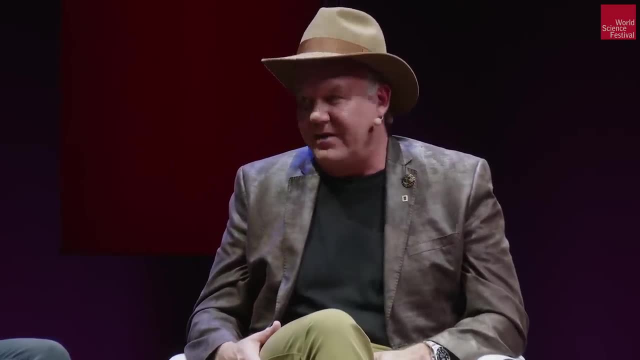 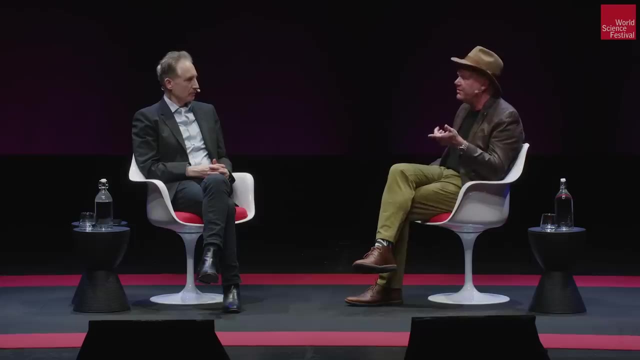 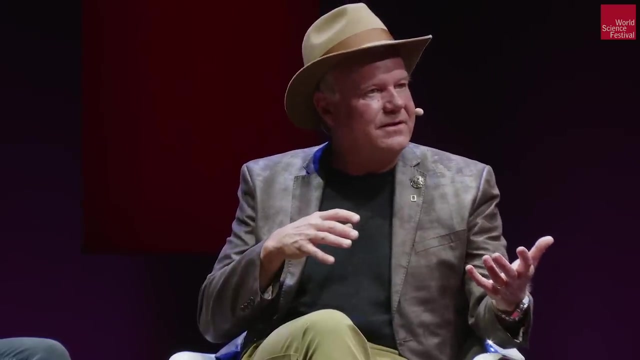 actually had, but not in the ancient fossil record. we see it all the time in human assemblages. the reason we see it all the time in human assemblages? because humans sort themselves after death from the natural world and we have places that we put ourselves. 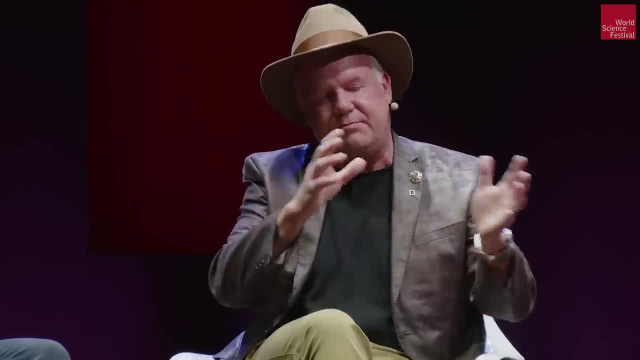 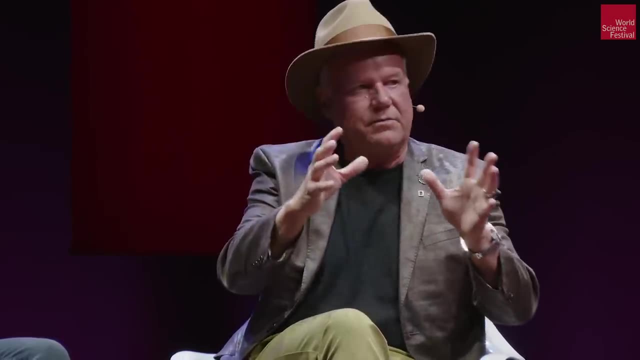 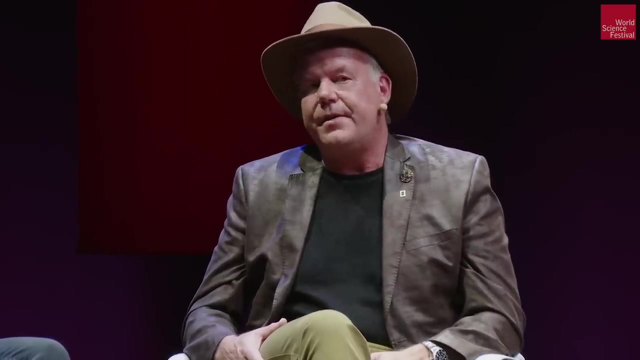 mostly separate. you know, sometimes we put our dead poodles with us, or if you're a pharaoh, you're dead cats and falcons, but mostly we put ourselves with each other or alone, and so it was becoming pretty clear, even like week two, that there must be another explanation. 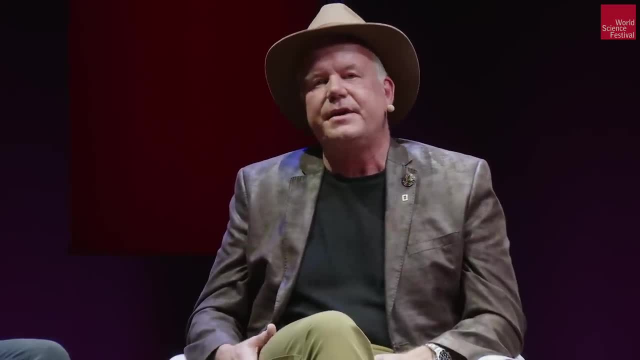 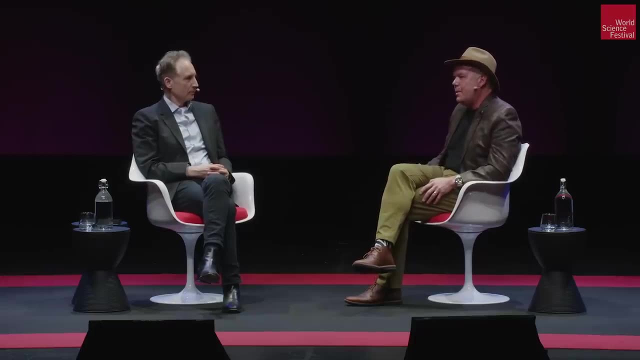 and so when we publish the book, we're going to be able to see that there's a lot of this new species, the homonid- that we published this new species, hominid leti, in 2015 in the journal e-life. don't remember that we said something incredibly controversial. we said: 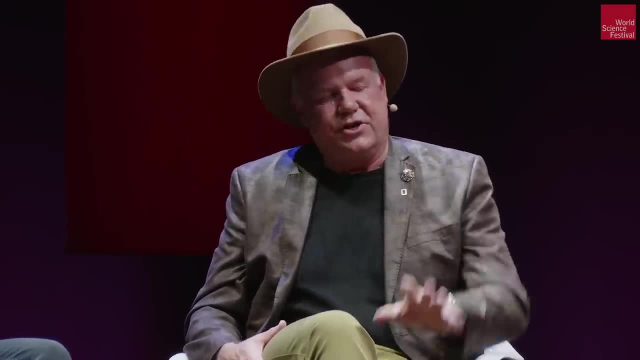 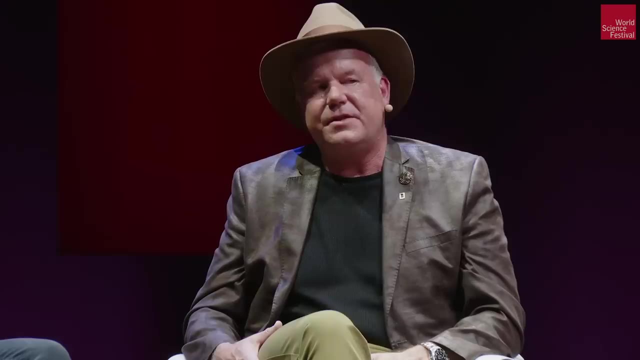 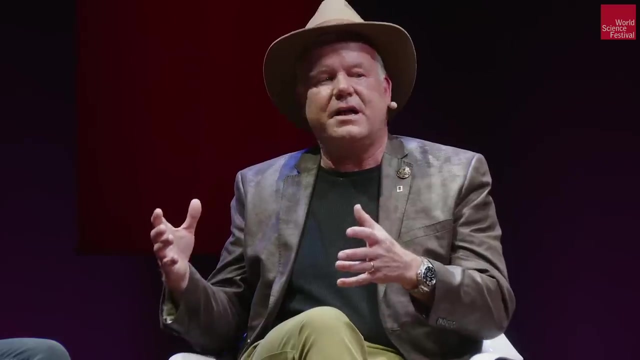 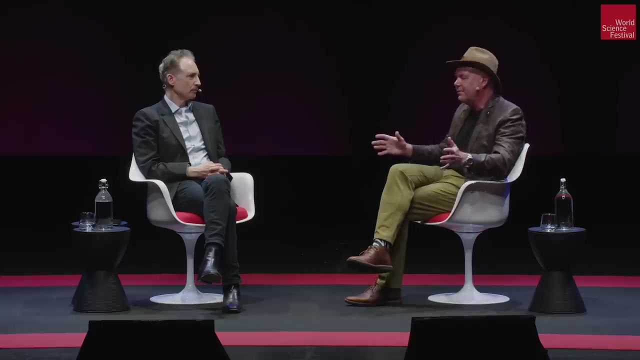 that the only possible reason that there could be only hominids in this deep, dark, remote chamber is that they put themselves there. they must have gone through some kind of tile, sort of ritualized behavior of carrying their dead into these spaces. and I'll tell you before. 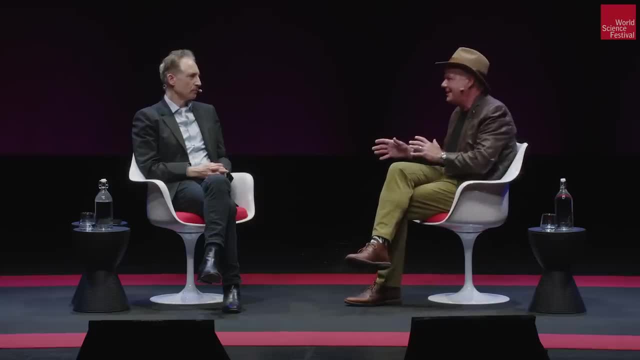 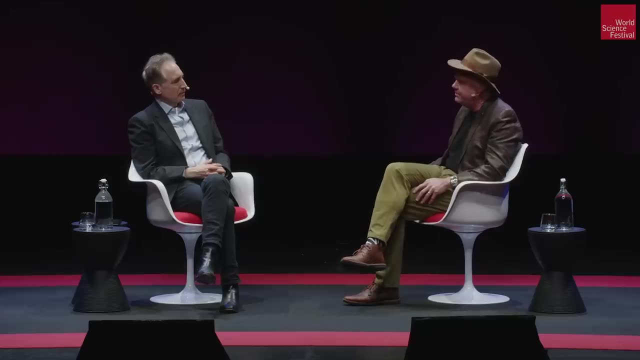 it's in your mind. no, the spaces haven't changed that much. No other entrances, No other entrances. They're going into this extraordinary space the way we do and they're taking their dead in there and they're disposing of them. 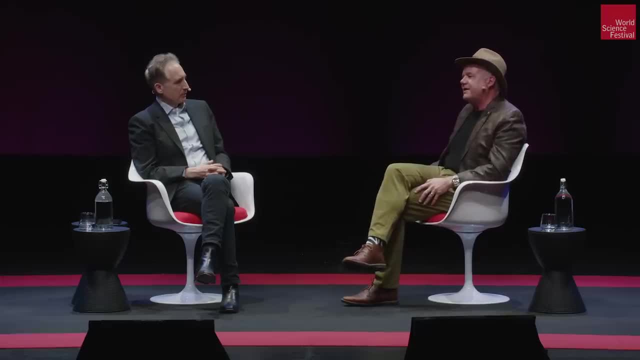 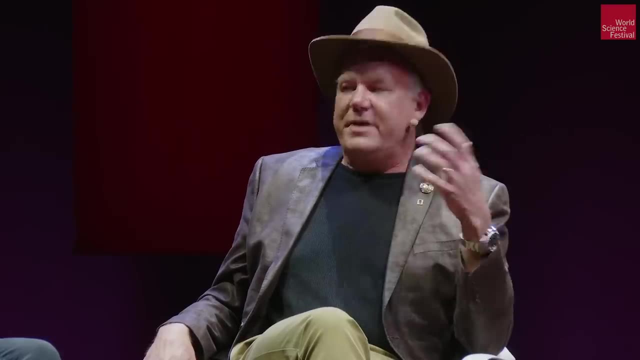 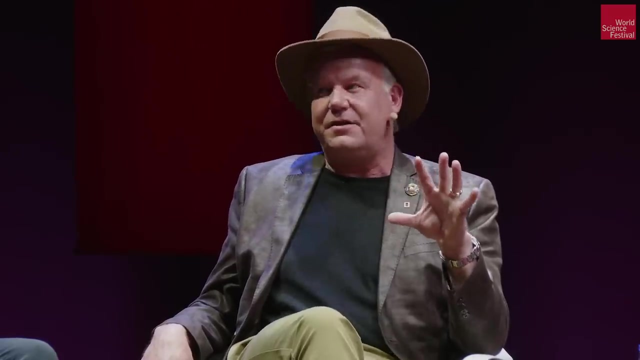 in a ritualized manner. I want to be careful there, because ritual means different things to different people. I was very careful of saying ritual means repeated, because while the world accepted our new species very readily, because we had so much to say, that a tiny-brained hominid 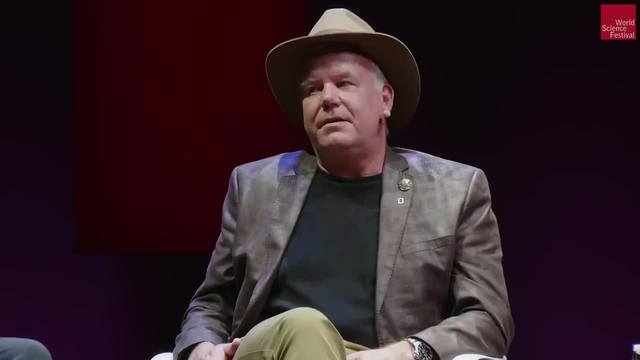 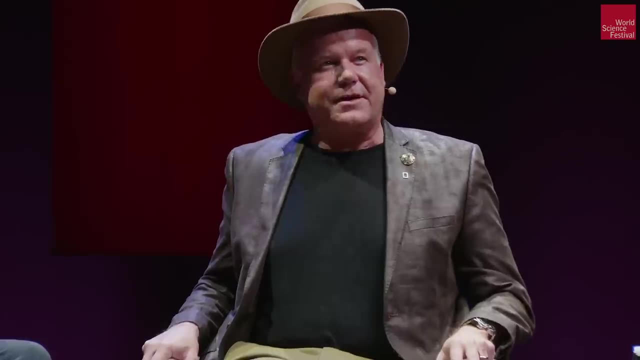 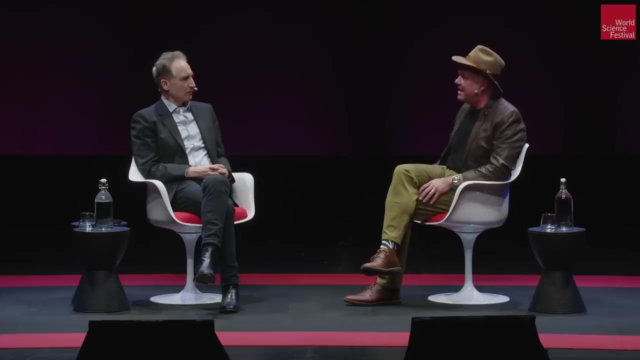 was actually disposing of its dead in a ritualized manner in a place like this. that was received and so you ever heard the saying of. you know it floated like a lead balloon. That was kind of how the reception was, because those type of mortuary 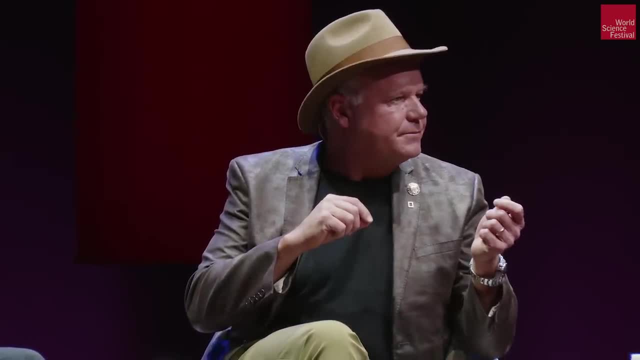 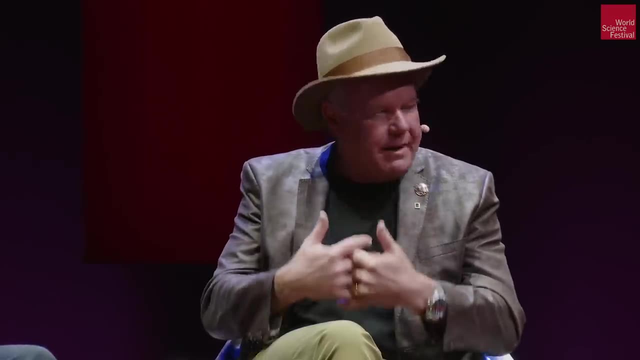 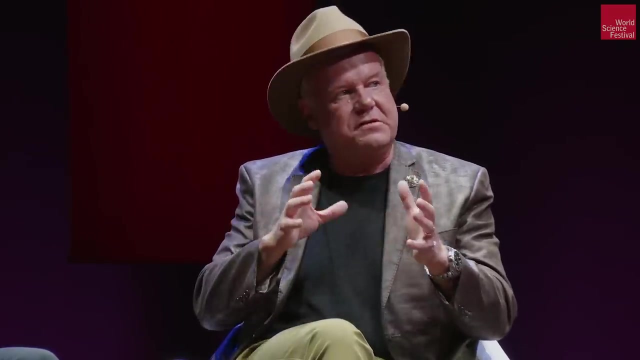 behaviors are related to a big brain. We claim it as ours. It is a human thing, It's done by humans, It's done because our big brain and the way we are, and it only happened 60, 70,000 years ago. 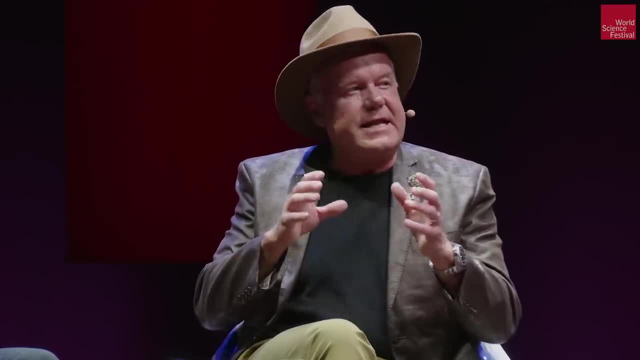 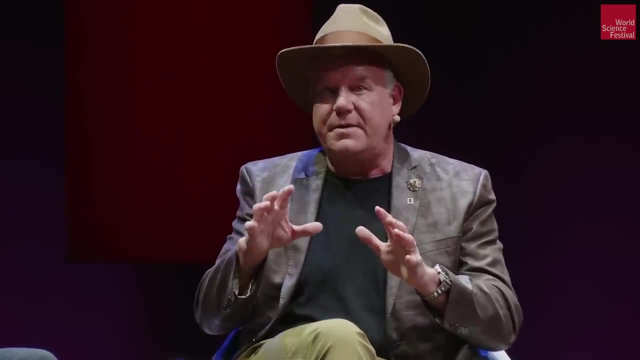 In our lineage maybe a little earlier, and even the cases where people say it may have occurred in the other large brain thing, Neanderthals, the few cases where they think there may be burial that took decades of fighting to even be remotely thing. 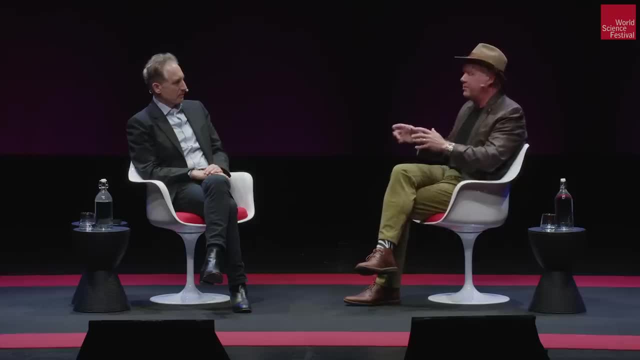 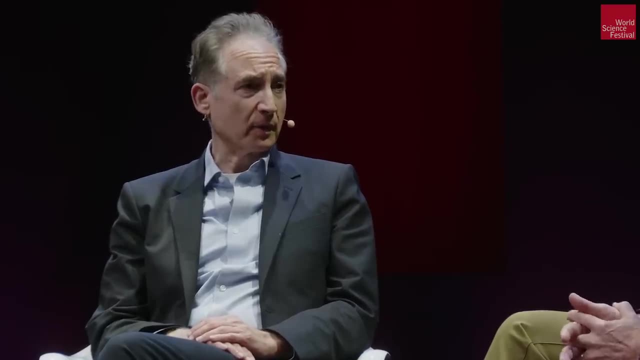 We were stepping into the definition of human. By the way, did you know? there's no definition of human, Brian. If you ask me, I'd be hard-pressed to give you a definition. so I can well imagine. So is Webster's. 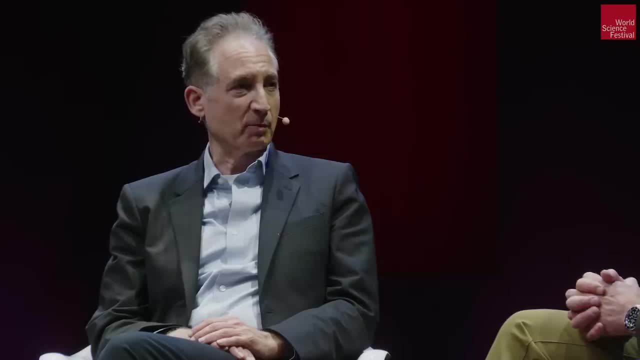 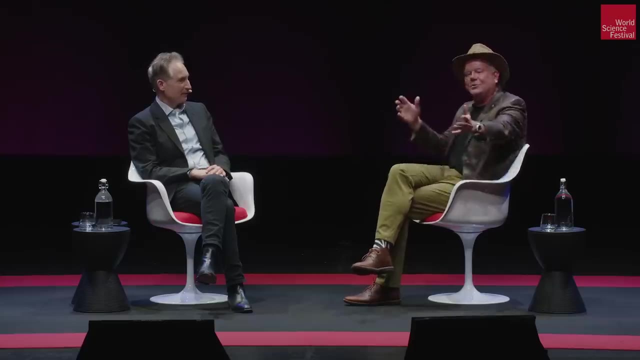 dictionary and every other science. It probably is kind of circular. right, It's like humans are people who are kind of like humans, or something like that. He's not joking. Look it up. Google the definition of a human. It'll say having the. 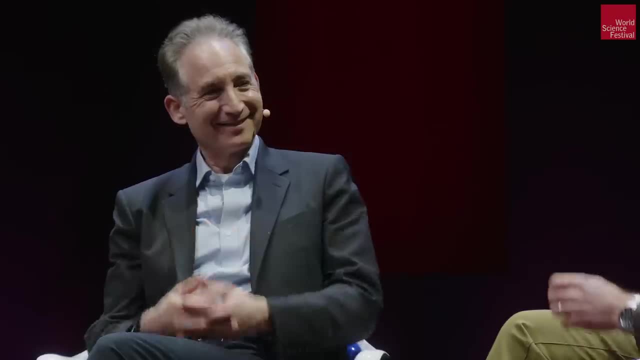 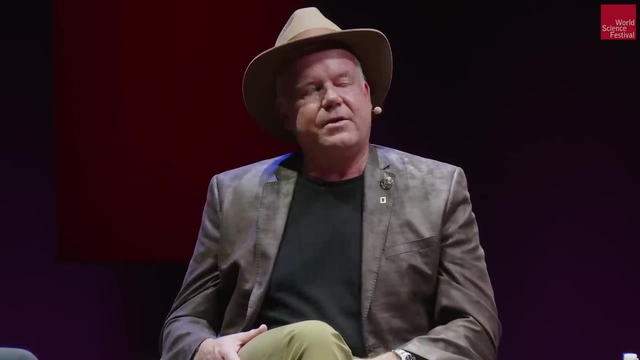 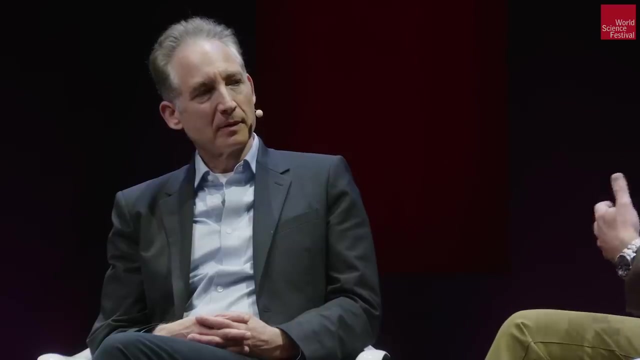 characteristic of people or a person. If you look up Homo sapiens, it'll say having the characteristic of a human. You know why? Because we don't have an out group. Everything's like us, that does like us, and we see ourselves as totally human. 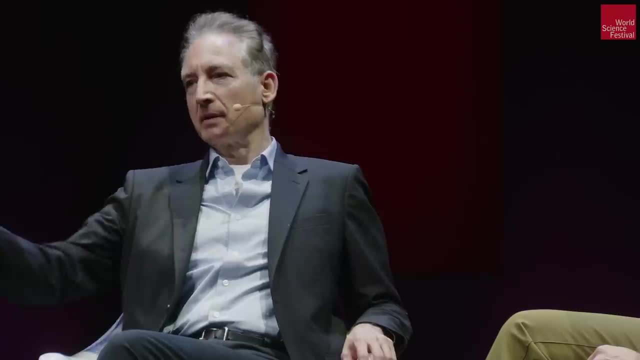 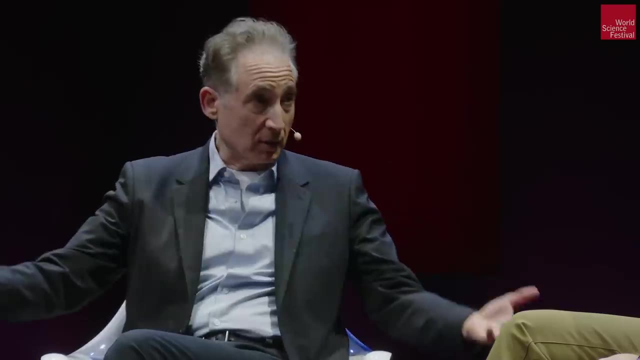 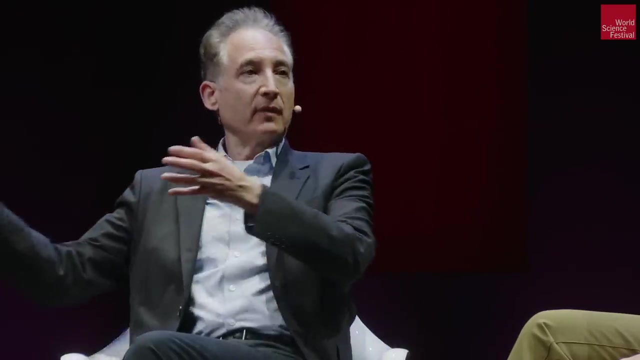 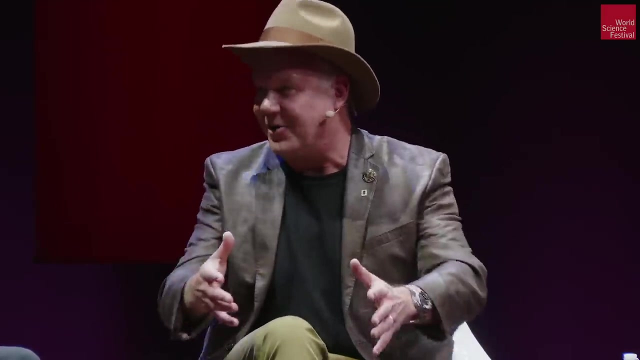 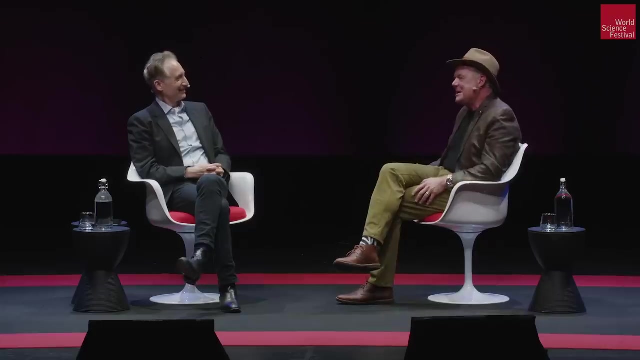 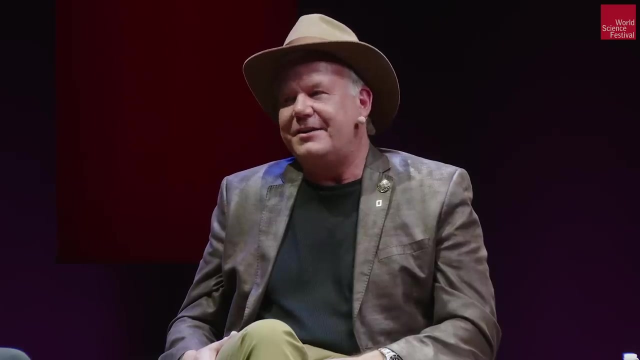 We're just like the conceptual. I actually got in the cave, but I'll tell you that That's for later. The answer is that we threw one of the largest scientific teams in history at this problem. We did not say it lightly And we eventually, like Sherlock Holmes, had worked our way through. 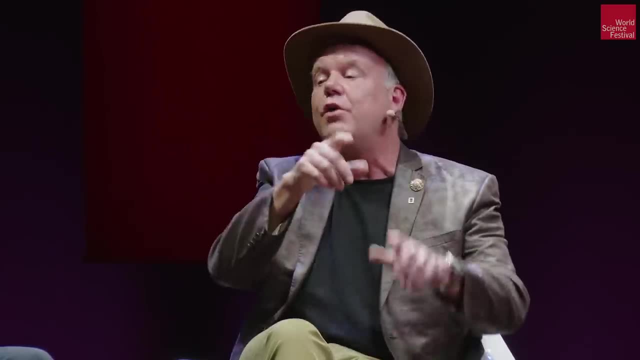 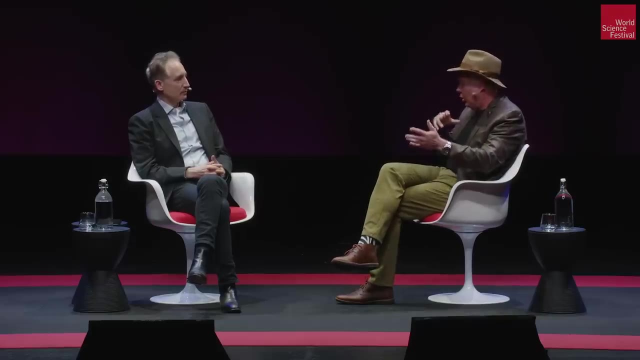 We could prove they weren't washed in there. We could prove that they had come in over time. Some were earlier, some were later, Some were earlier, some were later, Some were earlier, some were later. They had come in whole. we could see that as bodies. 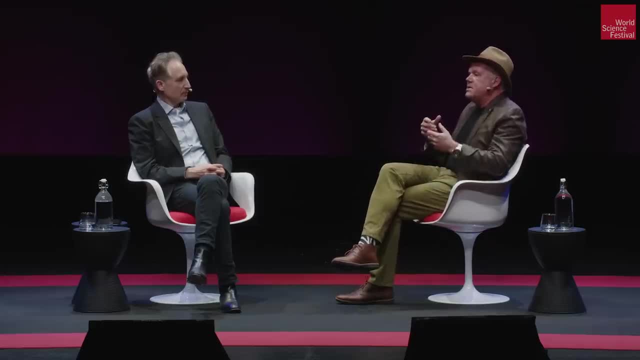 They were violating gravity and all that They had. it wasn't a catastrophic event, It wasn't some movement of water. There were no evidence of carnivores or scavenging or any marks on their bodies. And eventually, after that and lots of other evidence, 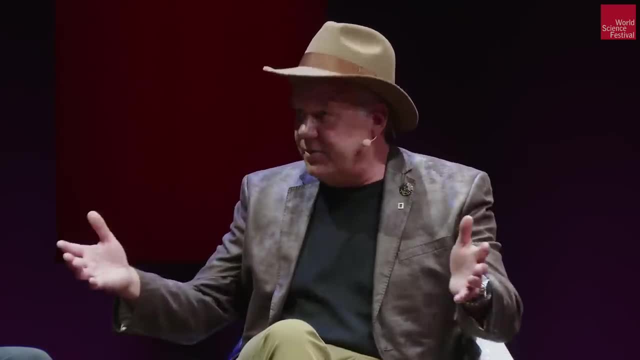 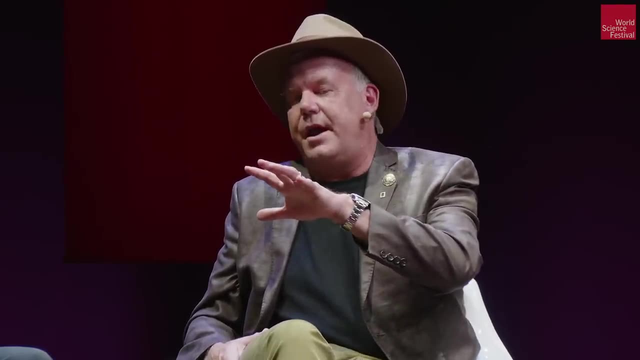 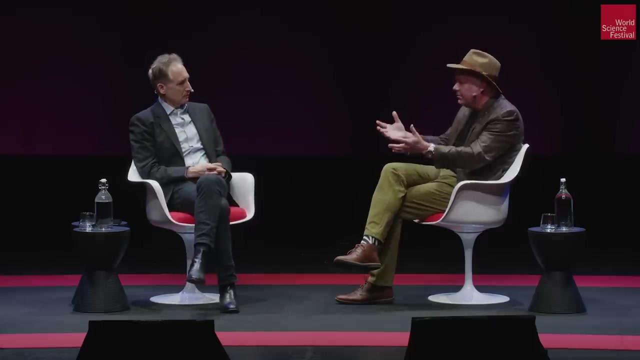 we had eliminated all the probable and we were left with the improbable: That we had discovered the first time in history that a non-human species, and something that clearly is outside of our grade, that was practicing some sort of deliberate mortuary. 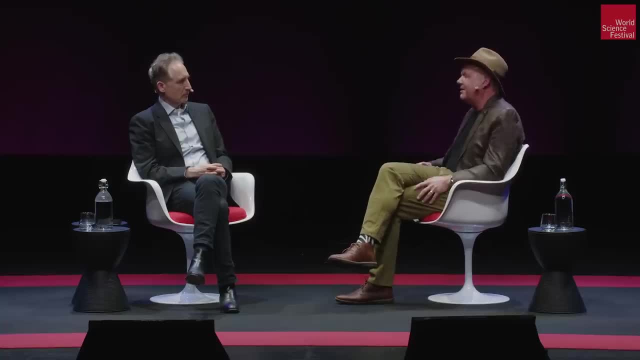 That remains controversial. I'm hoping not for long, But it remains controversial today. And what really made it tough was, with this tiny brain hominid that by then people were had rapidly began telling us We didn't have a date for it. 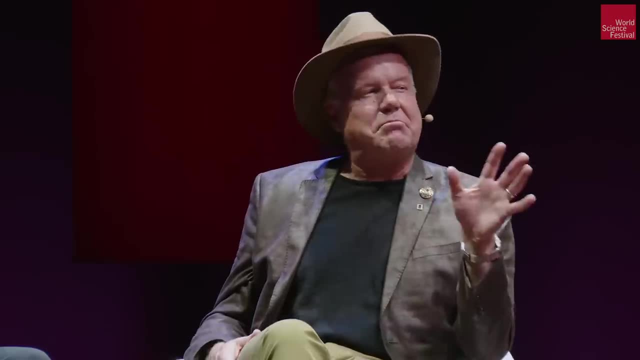 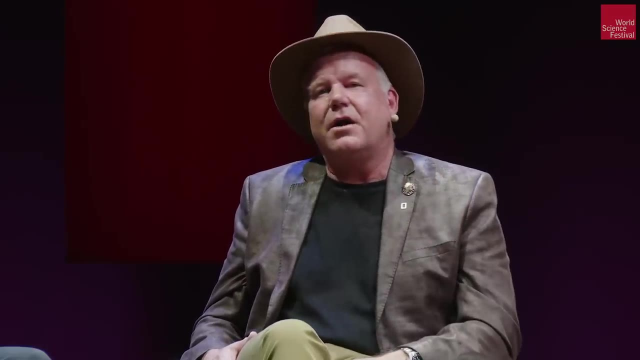 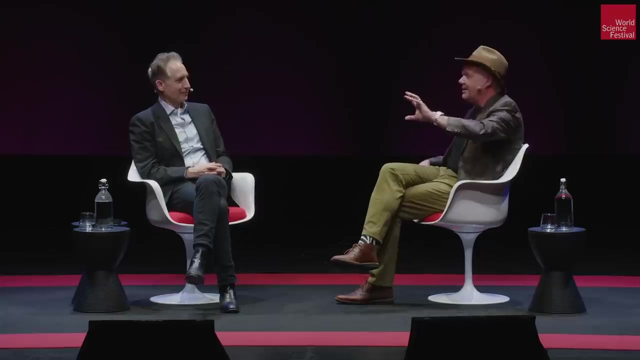 We couldn't tell you how old it was. Now that's a problem in paleoanthropology, Because everyone thinks dates- wrongly, by the way- are super important for saying where something fits, Because everyone thinks evolution works like a Biblical story of you know. 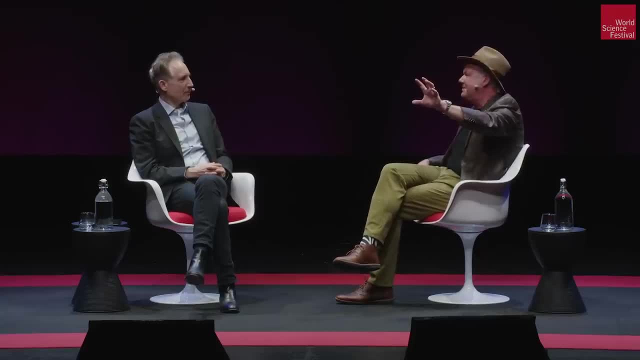 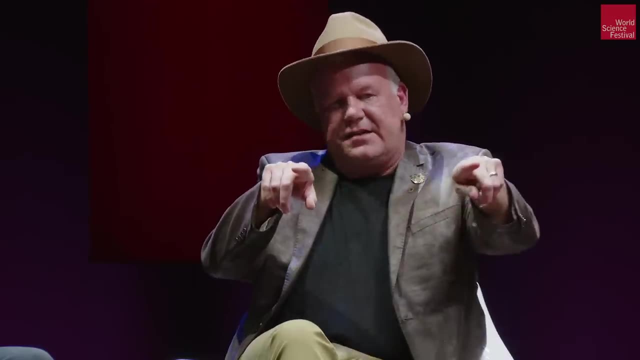 you know, afarensis begets homo habilis, begets homo erectus. but it doesn't happen that way. Species can arise as a fission or breakout, and the others can continue quite happily. That's why we can see coelacanths today. 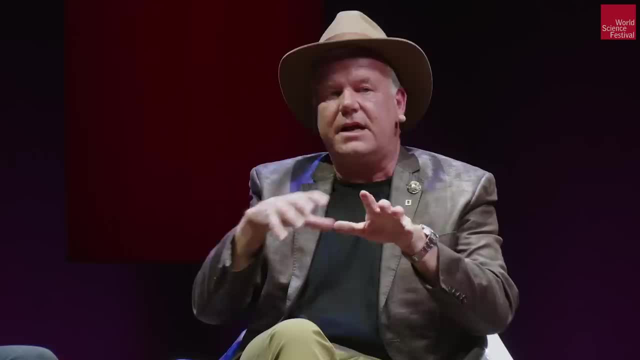 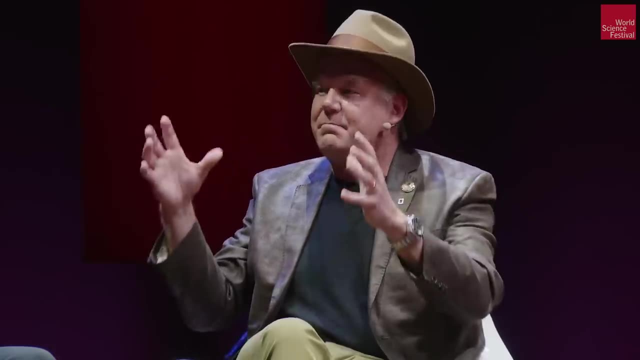 You know, Sure, They just keep on going, They keep on going, And so it's much more complex. But humans have always seen themselves as so exceptional that we have this sort of image that once the next better mousetrap evolves, nothing can. 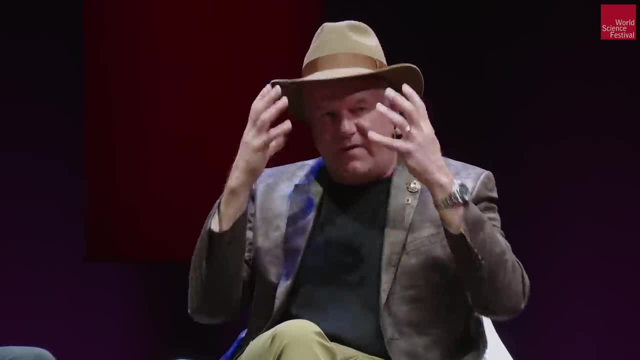 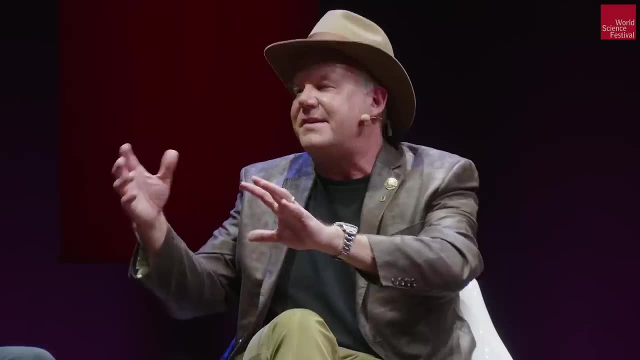 So we had scientists that were saying that the morphology of Naledi was showing that it was really probably just some kind of primitive homo erectus. When they say that, they mean two million, 2.2,, 2.3 million years old. 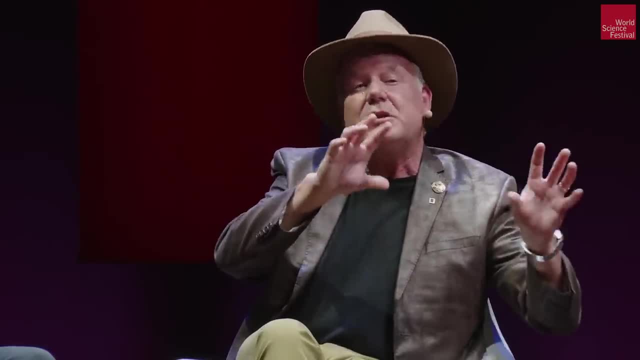 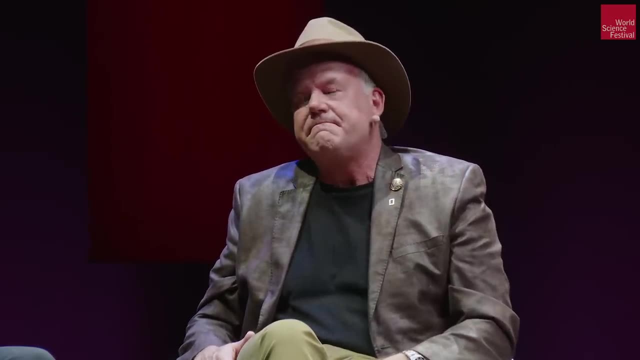 Or it's another species of primitive homo, or it's even a late australopithecine, but all of them were, you know, a million and a half, two and a half million years old. You could look at its anatomy. 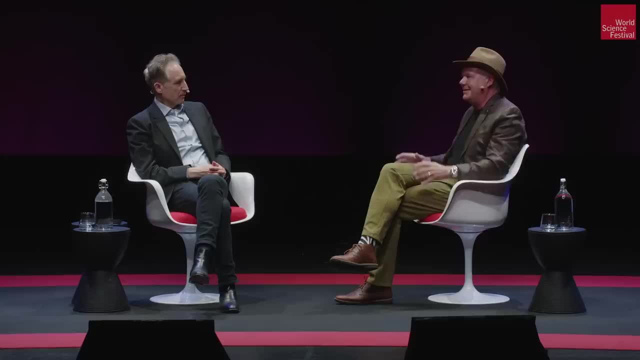 But we threw the kitchen sink at getting a date Because no one had ever. You've got to remember, you've got to be sympathetic with us. No one had ever found a whole bunch of hominids lying on the floor in a dirt cave and then immediately beneath the floor. 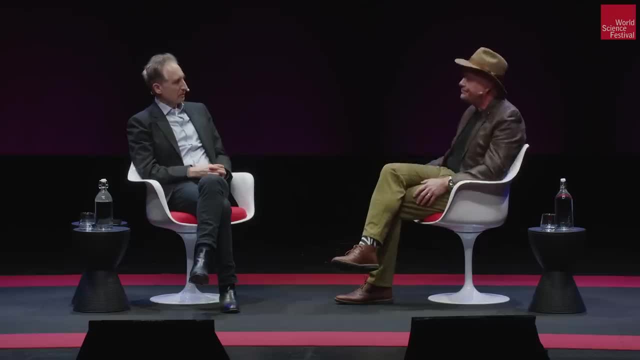 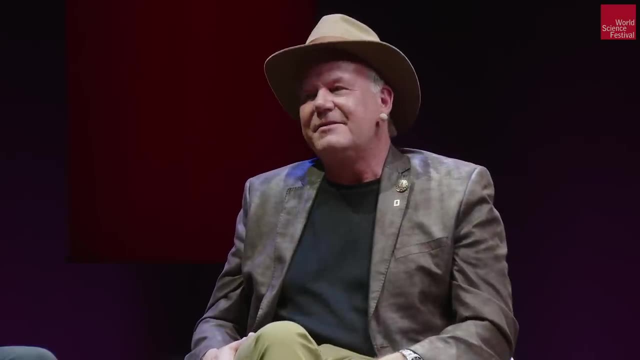 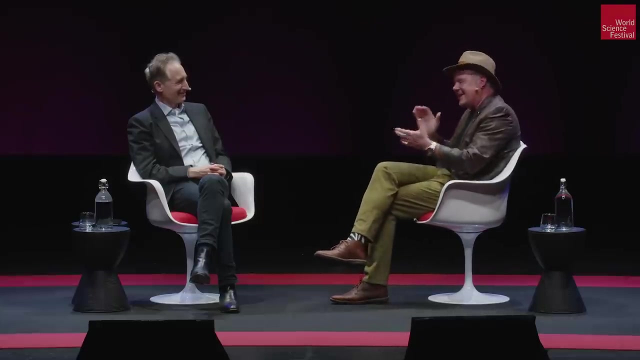 We didn't have technology. We invented it With, by the way, quite a lot of Australian researchers, Some from Griffith University here and others with your great facilities here, And we broke through the day. Yes, indeed, that does deserve a round of applause. 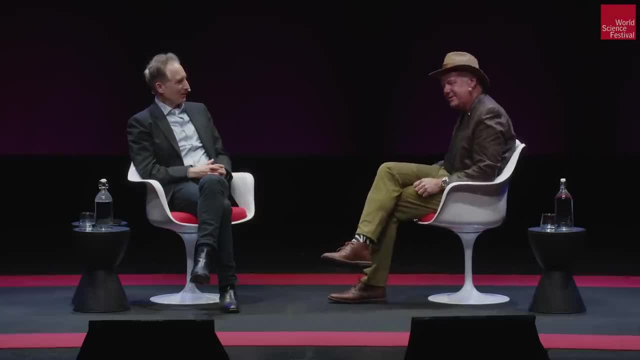 Thank you, Australian Research Committee and Australian government. And do it again. And we broke through. We invented new ways, We refined new ways, We refined new ways to come to these answers And then we announced how old they were And the answer is: 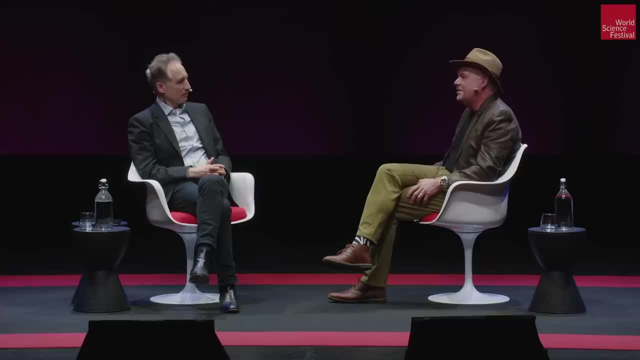 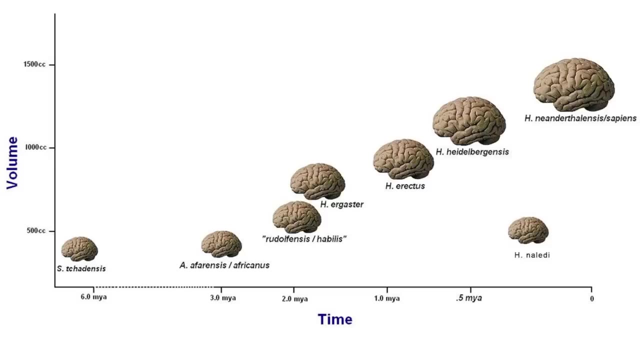 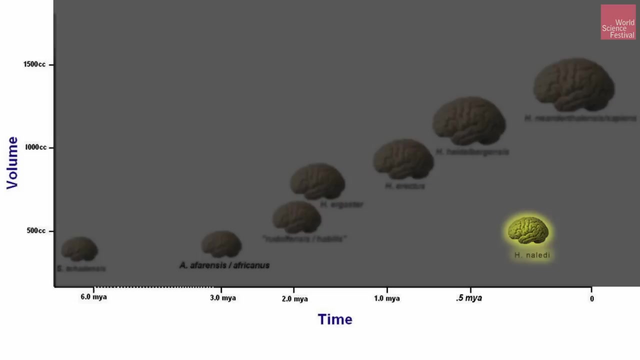 Young, Incredibly young, So young that it was unbelievable. In fact, there you see their tiny little brain at 230,000 to 330,000 years ago, More than a million and a half plus years of what they should have been by their looks. 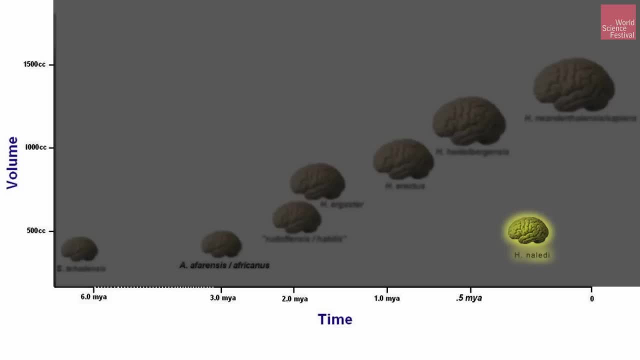 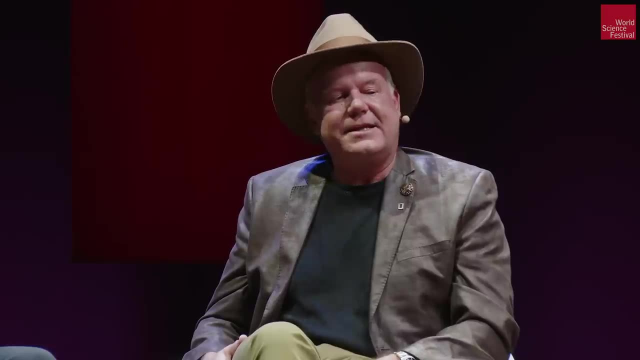 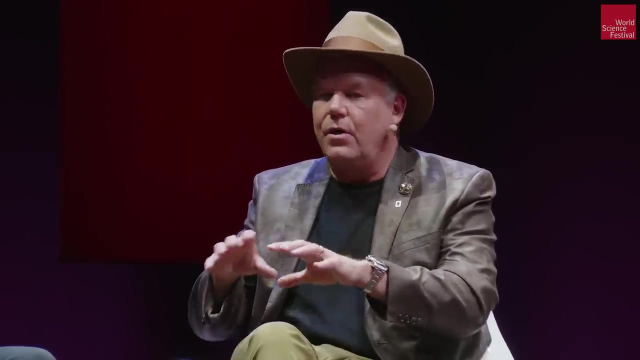 Right in the middle of Africa, At the time when only Homo sapiens should have been there. At the exact moment when we thought that modern human mind was arising from all the archaeology that was appearing, We were seeing the development of more complex archaeology. 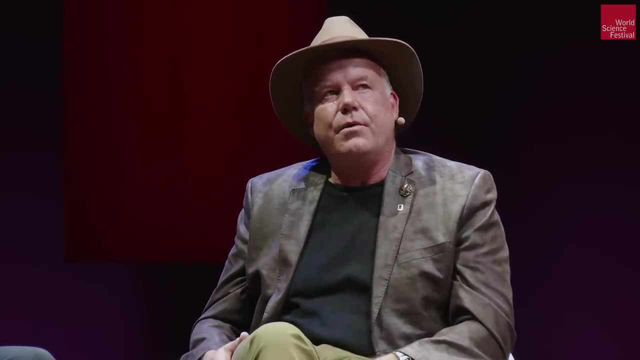 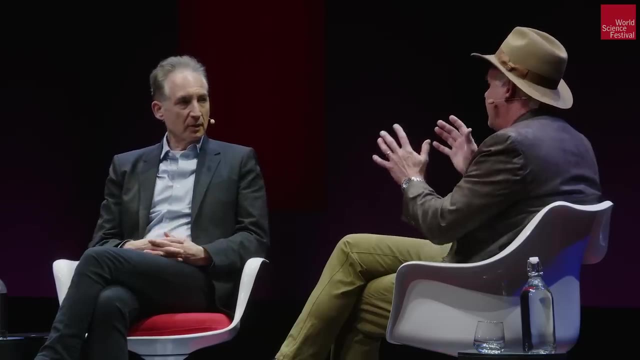 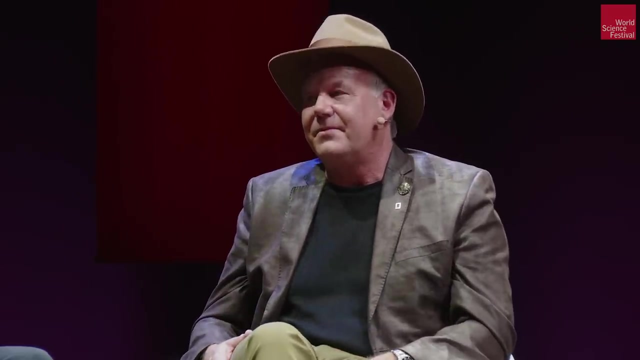 coming along And that that blew everyone away. And how confident are you of those dates? I am confident that some of them are that old, Which is all you need really to make the point. Yes, yes, My hesitancy in your answer. 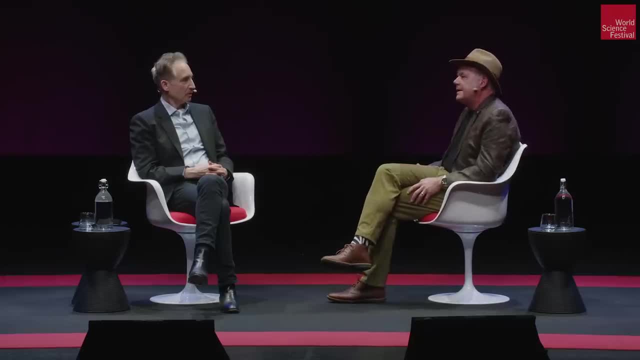 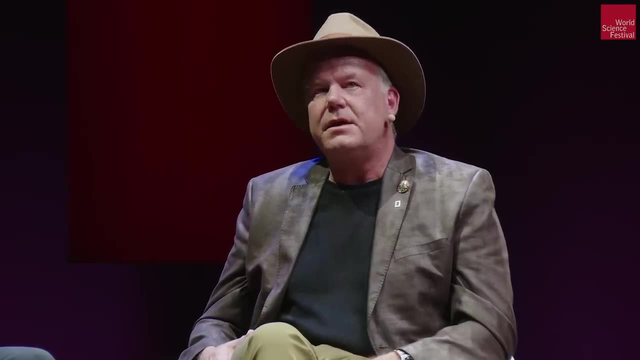 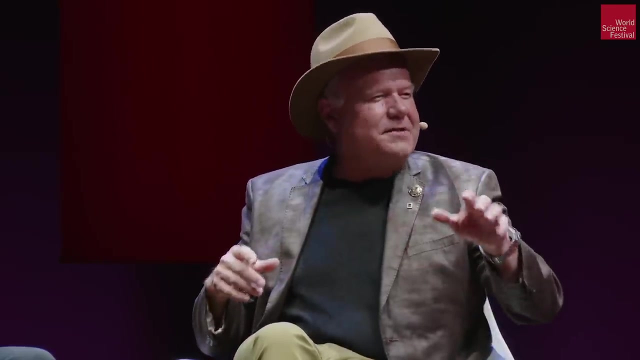 is that we've obviously been continuing the research And I suspect that things are going to change. I think that we have encountered something extraordinary: The idea that if a small-brained primitive hominid- And, by the way, that doesn't 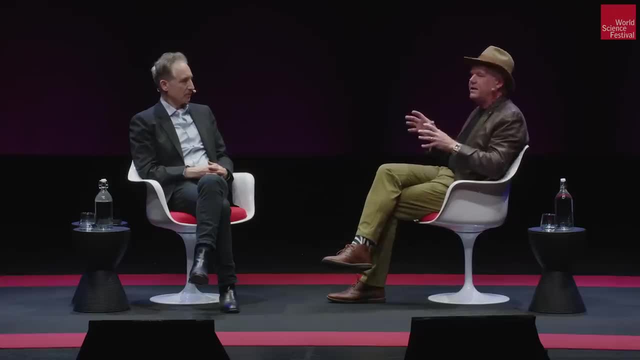 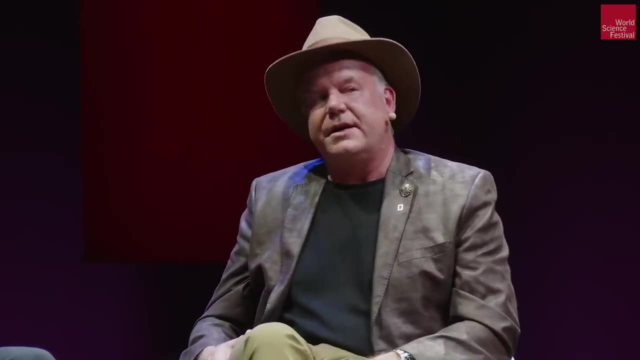 It doesn't mean our colleagues are wrong, that Homo naledi doesn't exist at a million, a million and a half, two million years. You remember the coelacanth example that I gave? What it means is these groups of them. 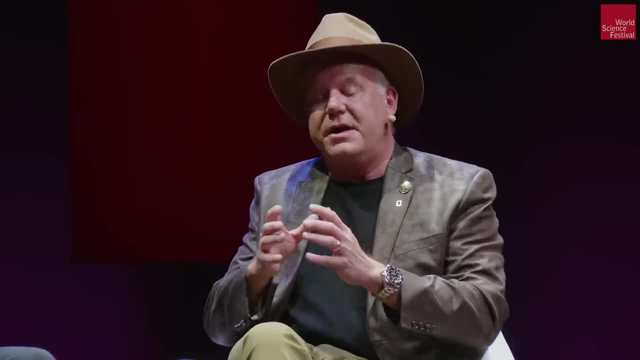 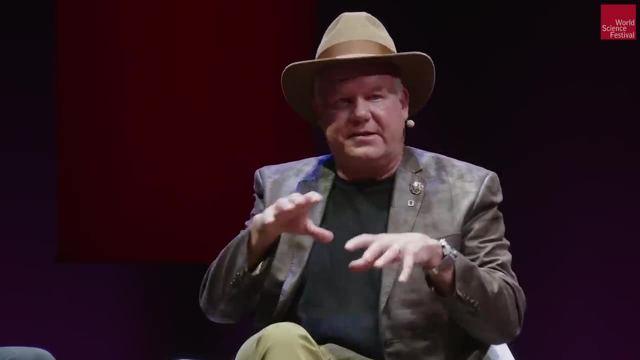 at least some of them aren't that age Right, But it means they existed back then. It also means they could come forward in time. We're not witnessing an extinction event, So I think there's going to be big news in the future. 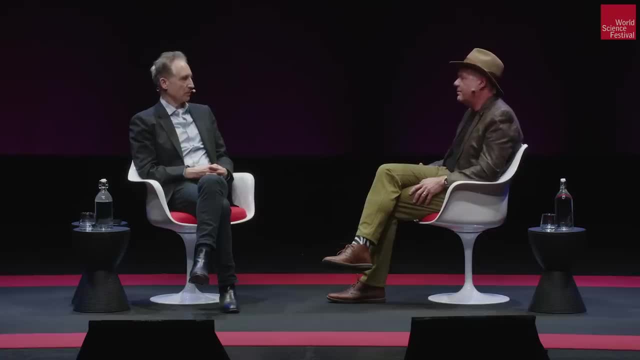 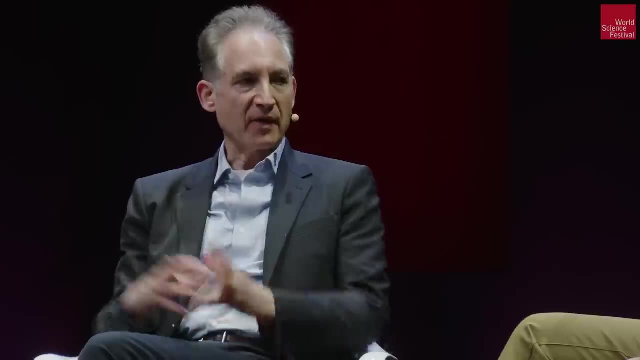 about the range, the time range, And you know, just because you happen to be talking to someone who kind of maybe knows that there are going to be alterations in that. And this is one cave area. right, You have many other places, sites to. 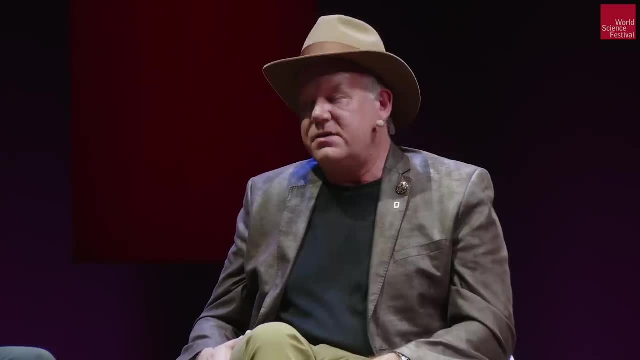 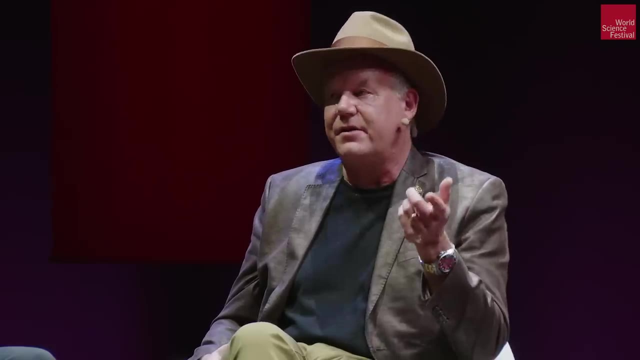 Sites. potentially We have yet to find definitively Homo naledi elsewhere. But I would caution you if you go back to that brief anatomy lesson I was talking about, it'd be hard to see something like this if you didn't have the whole picture. 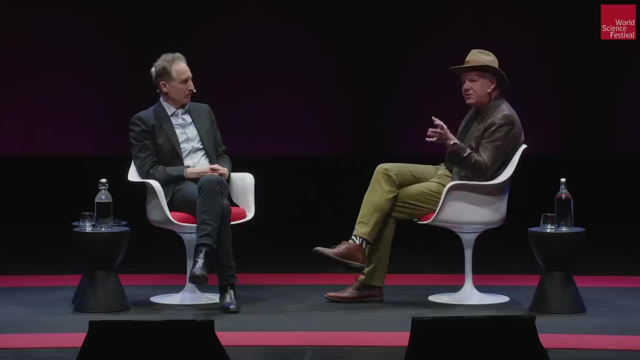 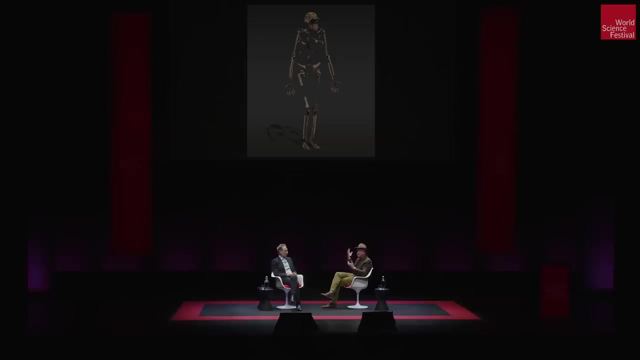 And it would be easy to take bits and pieces and mix it into other things that we had and not see the whole, particularly in a record that has been as sparse as we have. when you look at this mosaic anatomy, We are on the edge of just incredible things, Brian. 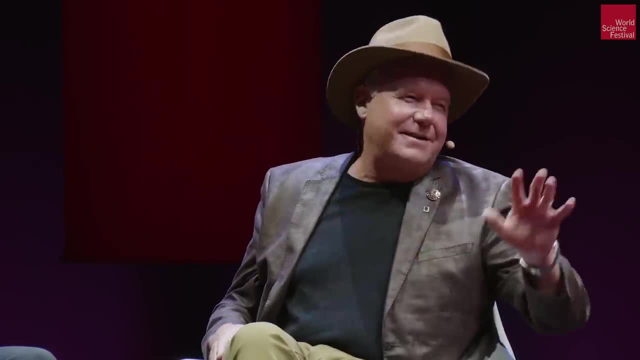 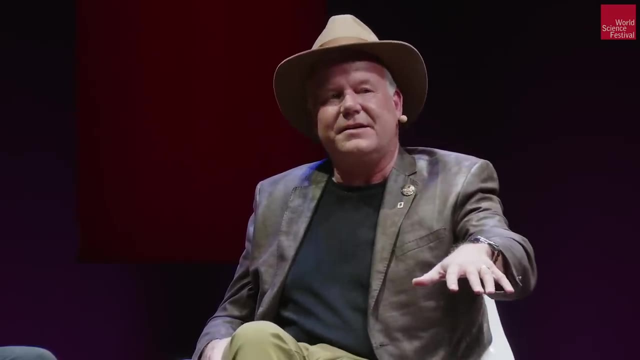 I mean it is. We've been at this. By the way, I didn't stop exploring. We have made other discoveries in other places. I learned my lesson from Gladys Vale and learned my lesson from Sediba. I learned my lesson from this. 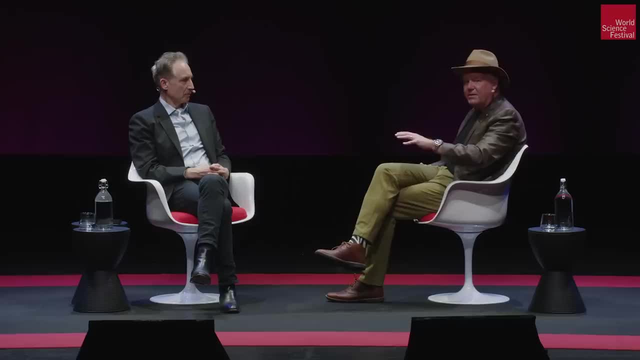 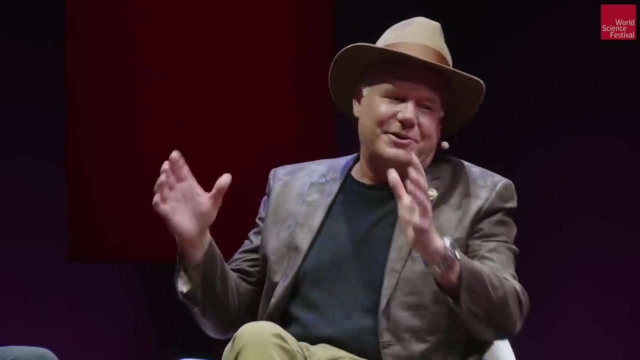 I didn't stop exploring. During COVID, we discovered, 250 meters away from this site, an entirely another giant site full of hominid fossils, but not these fossils, Something different. And that was really cool too, because COVID was great for us. 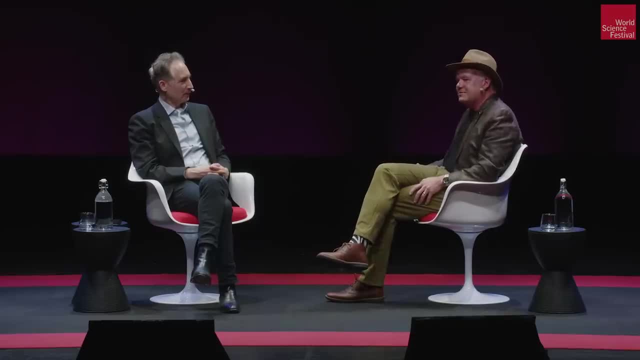 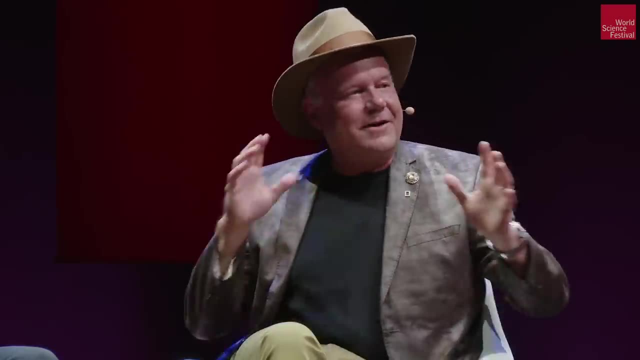 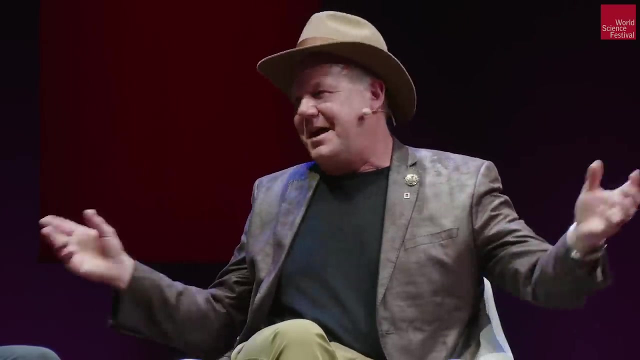 Don't hate It knocked me off my pedestal of success. It took me out of this rut of you know. here I was. I built this gigantic organization that was based on scientists. We make a discovery. Scientists fly in from all over the world. 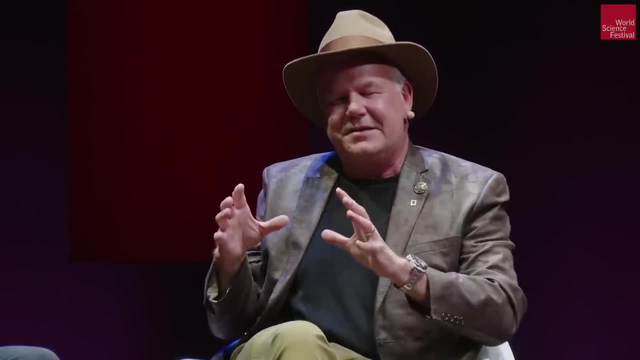 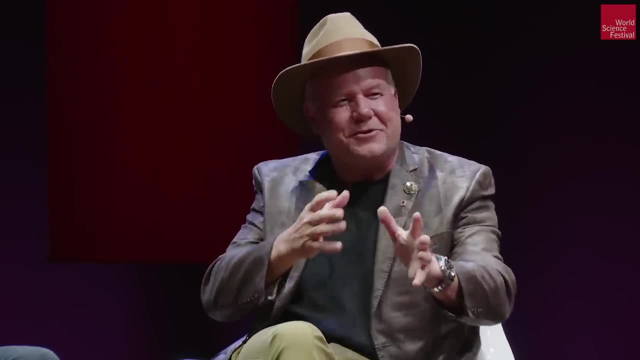 They work with it. They mentor all my young scientists in Africa. We get the papers out, We describe them Off, we go. My teams are working in confined, humid spaces underground where, if they get stuck, we have to send in other people to rescue them. 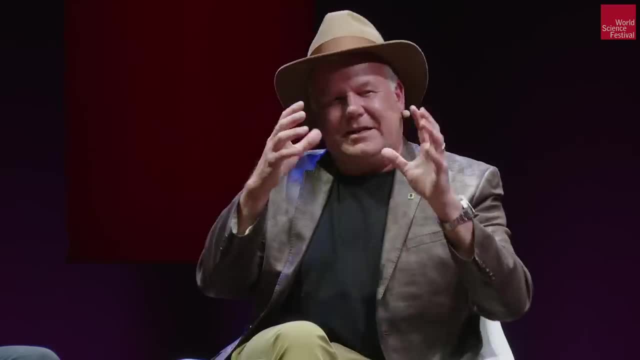 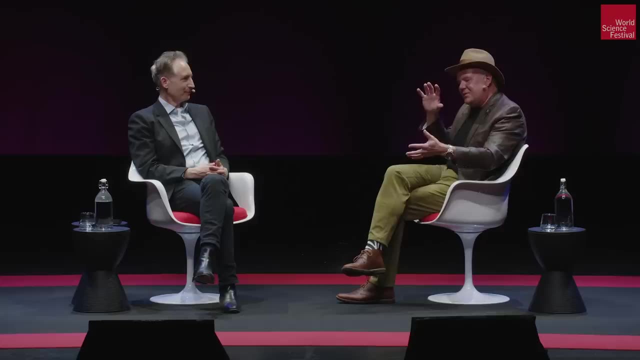 And we're all working in. you know, even our preparation was in these rooms together that are likely probably poorly ventilated. but don't say that, And you know. and then a pandemic comes along And I went from hero to zero in minutes. 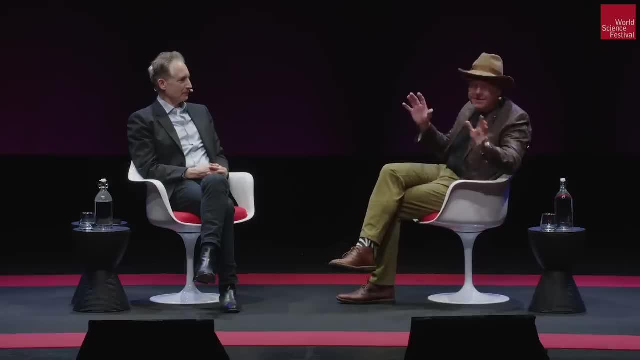 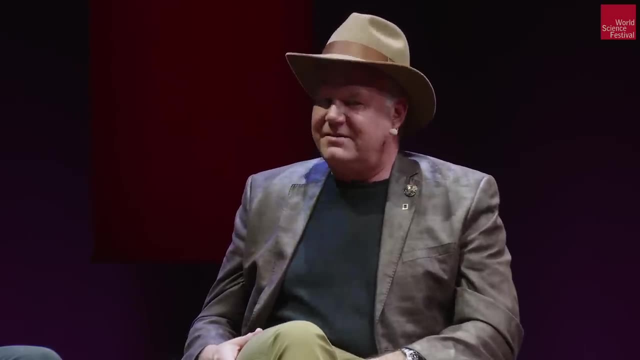 You know, South Africa did not have an easy lockdown. I know you didn't too, but ours was worse than yours, And so I had to start over, And it made me redesign it, And I had to figure out how to excavate a site. 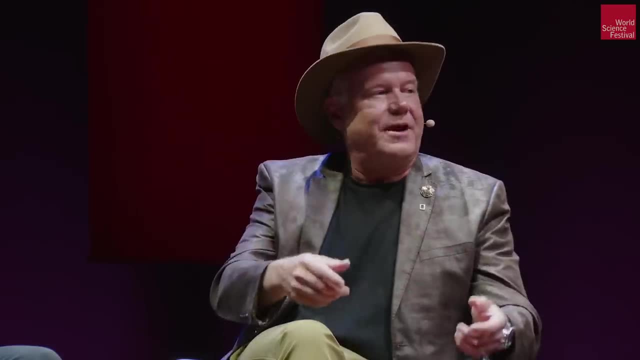 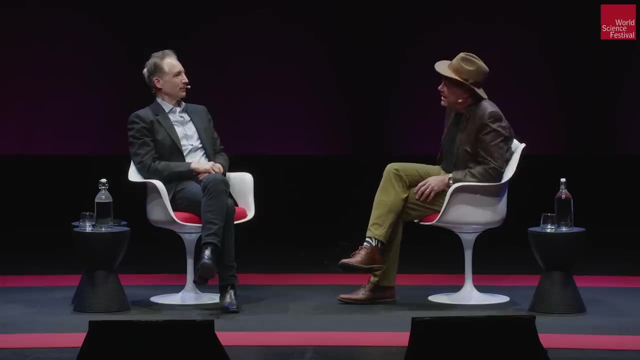 And so I did And I reinvented. I couldn't work underground, So I took the underground and brought it above ground. Watch the YouTube videos. It's really funny And and it also made me realize that I'd made a mistake with. 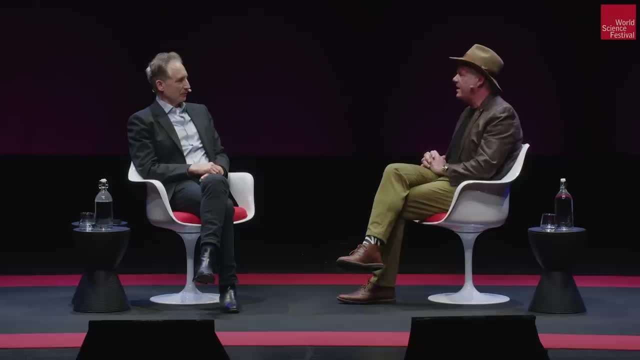 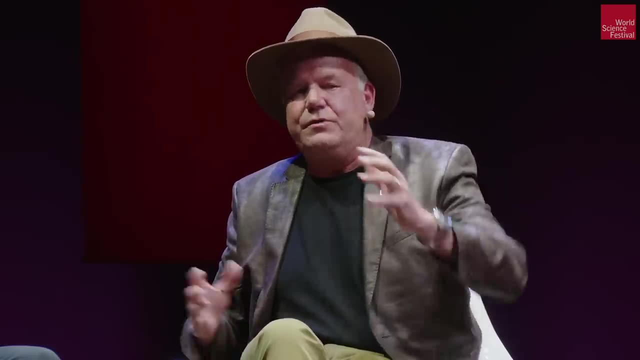 with my idea that bringing in the best and brightest scientist all the time was a way of mentoring. The young African scientists were coming up. What it also was doing was they could do it better and faster, So it was a form of mentoring, but it also meant there was always someone right above you. 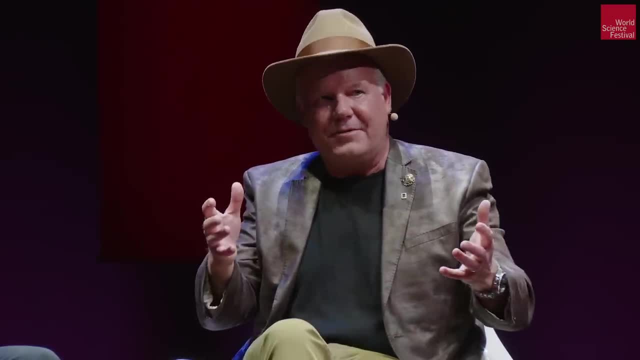 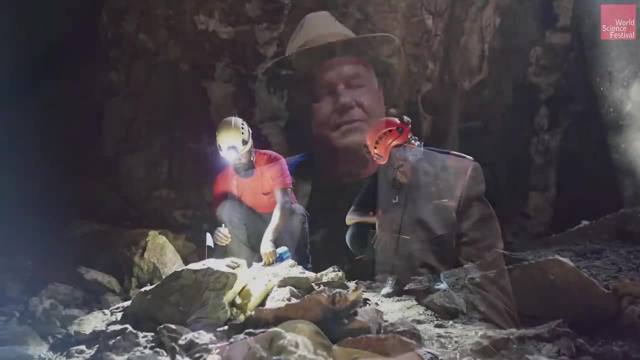 that you couldn't be through. So I'm standing here with this discovery that we made in the middle of COVID. We brought the cave up and there they were, you know, these new type hominids, And I had all these young people around me. 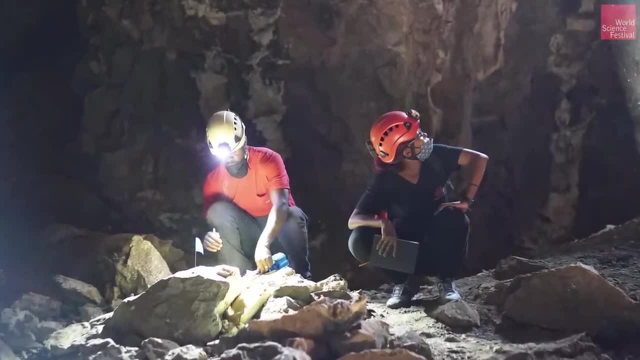 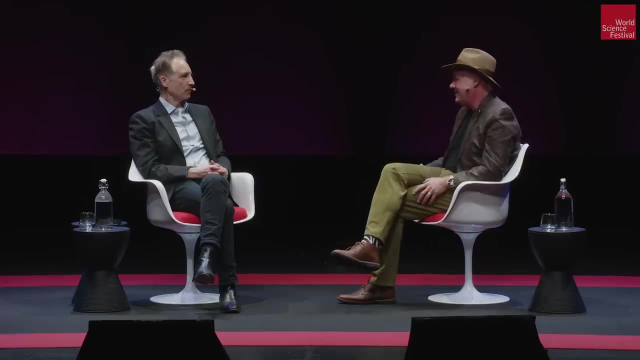 And I said: you know what I haven't done is I haven't given them the leadership on this. So I did, And you know how what they did? they did great, You know. they just turned on the afterburners. 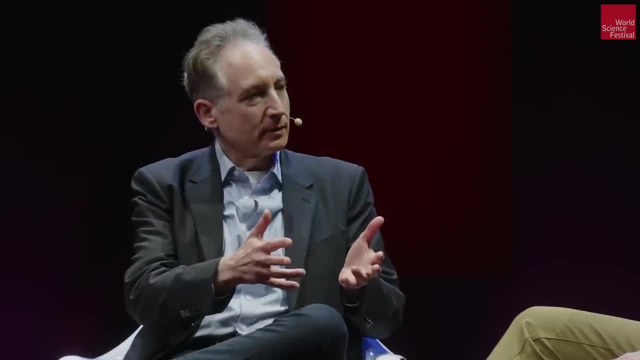 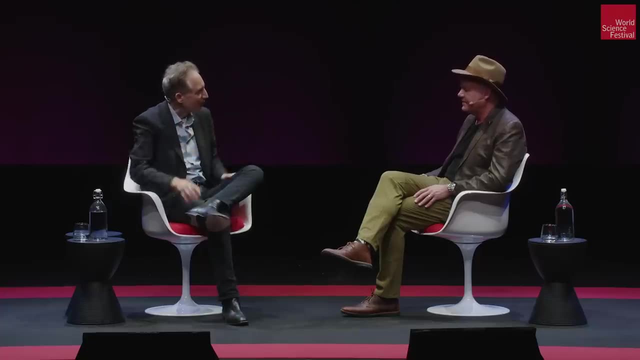 All right. So you're watching all these wonderful discoveries taking place, but you're close, but one step removed, watching it in a, in a television monitor, a computer screen. You must've wanted to go down right To be part of it. 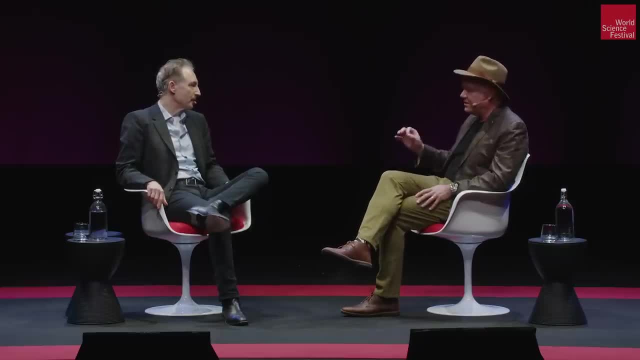 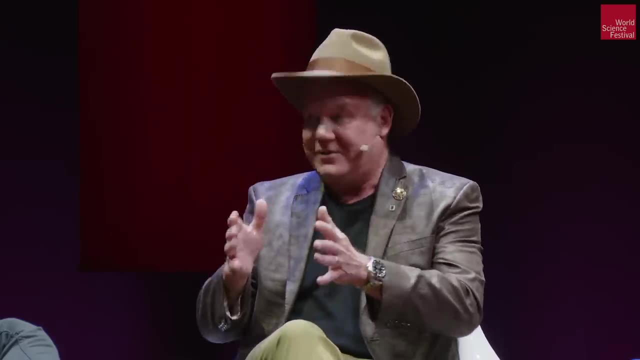 You know I used to cover up the that desire. you know, from the moment that Steven Pedro showed me those images and describe the situation, And when I crawled up there and sent Matthew down and was staring down into that void, I knew I'd never fit into this space. 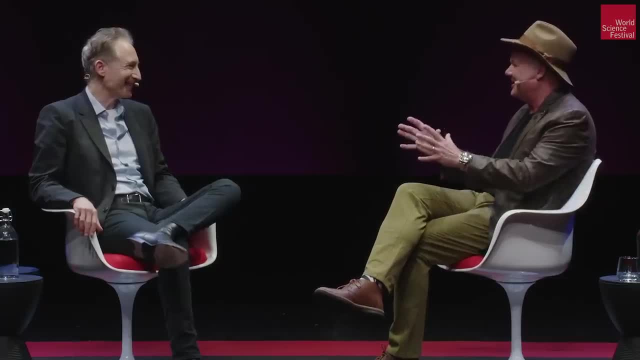 I used to. I used to joke that you know, my ego was too large to actually fit into that, that that shoot area And a lot of that was a way of covering up that. I just couldn't do it, You know. 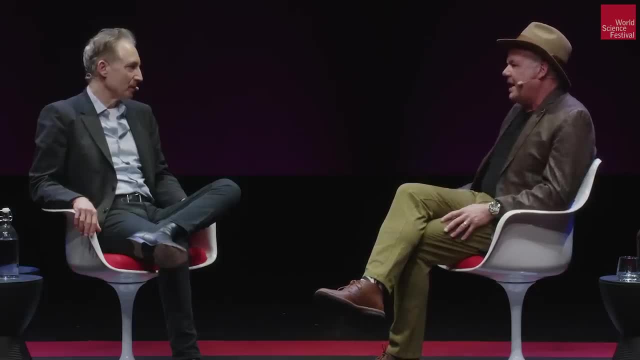 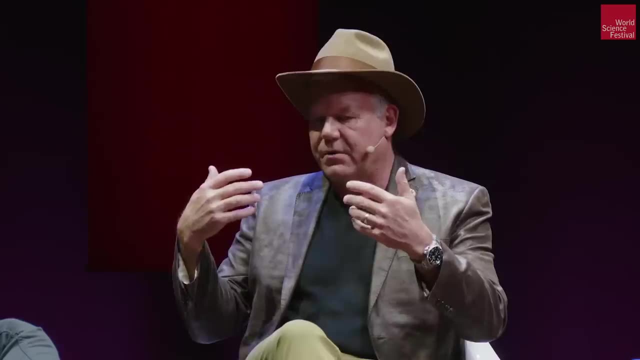 with people that were going in or fit. they're smaller than me And and things began to change as over the years, I was watching this and you know I'm watching it through these video screens. I'm remote from it. 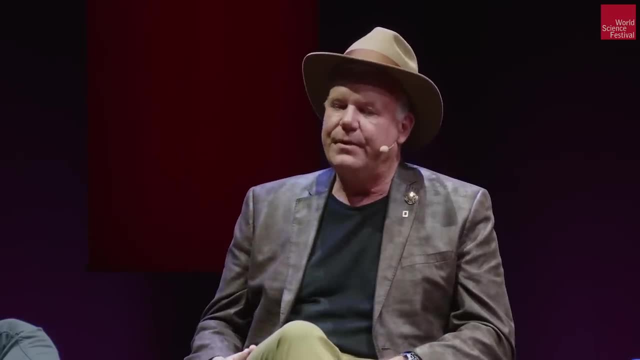 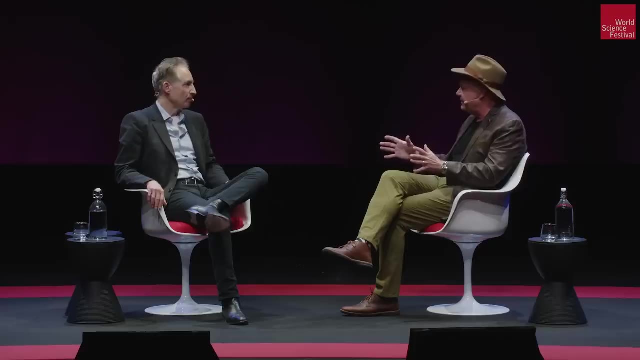 but just before COVID we made a discovery, And that discovery was sort of shocking, I think, to all of us. I was in the command center. uh Kanoe Moliopane, one of my mentees, was sitting next to me and we were watching the underground astronauts excavating. 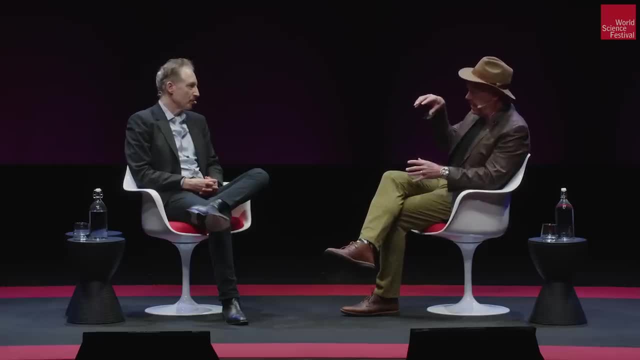 And they had moved the camera that day So it sat up above them, behind them, over their shoulder. It normally sat on the side So I could be monitoring where their hands were saying: Oh you know, hold on, That looks like a mandible. 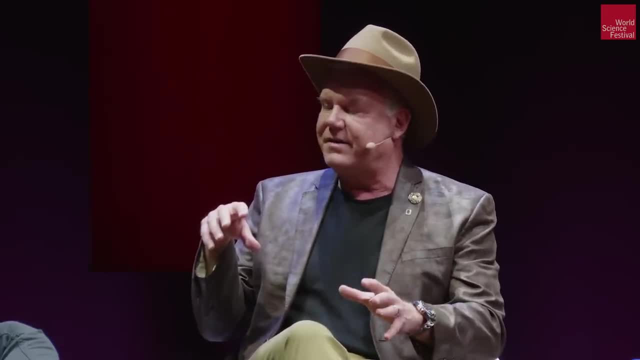 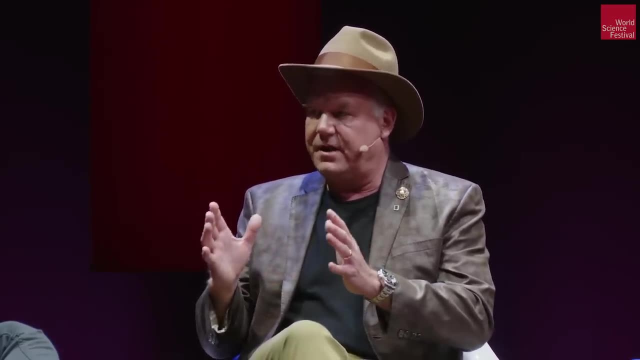 This looks like stop or, and they moved it because it was in the way of the excavation And it was an infrared camera. And a weird thing happened because, as they would shift, occasionally they would block the light that was adjacent to them, that we were shining on it, and it would shift infrared. 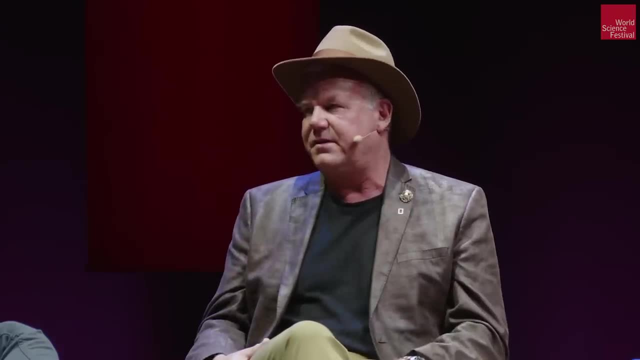 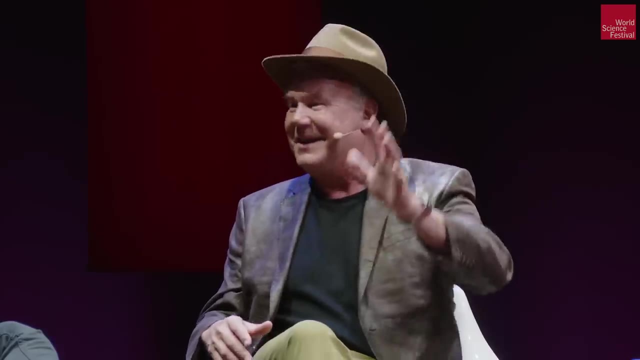 And in a moment I was sitting there staring at this excavation. You gotta remember that's happening for days and days and days of the tedium. You know you're like a NASA watching a space flight occur where you can never touch it Right. 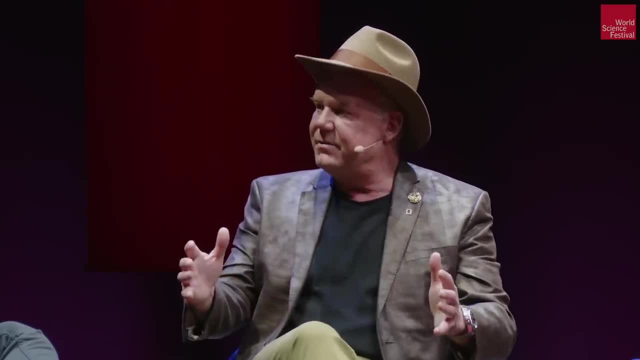 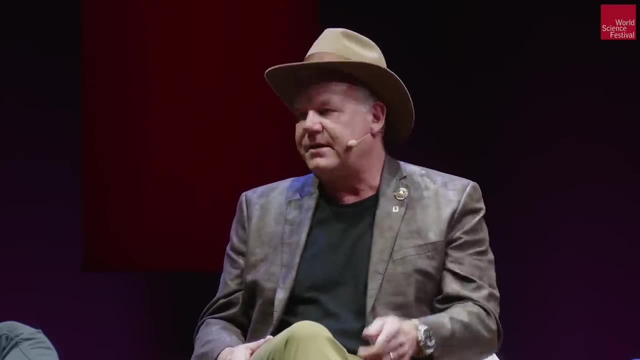 And I saw this shift and I realized that there was an edge to what they were digging. I could see a physical feature And I turned to Kenny and I said: you know, you see that. And she looked at it and I said: 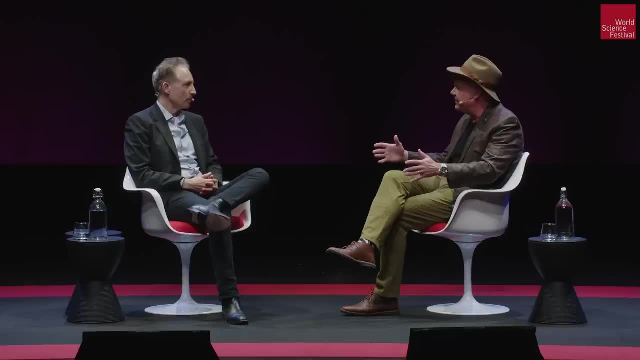 this is a line, This is a feature, And I suddenly realized something that had maybe been sitting in the back of my mind and some of our scientists through this remarkable thing where we're looking at this assemblage, the world's largest assemblage of hominids coming from these tiny areas. 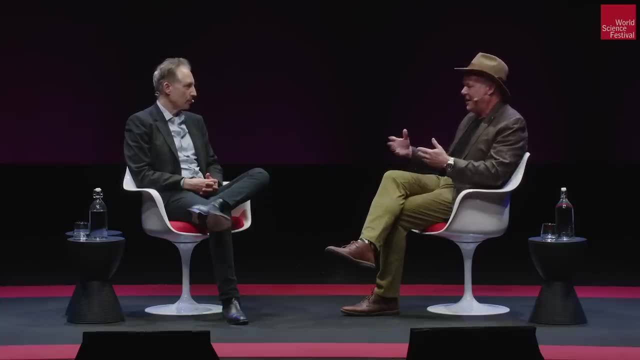 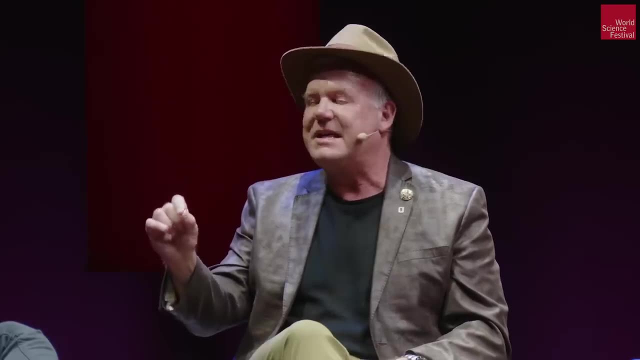 We'd always been terrified to say the words burial. I've been, as you know, I've been super careful over the years to say ritual disposal of the dead, because we're dealing with a hominid with a brain slightly larger than chimpanzee burial graves. 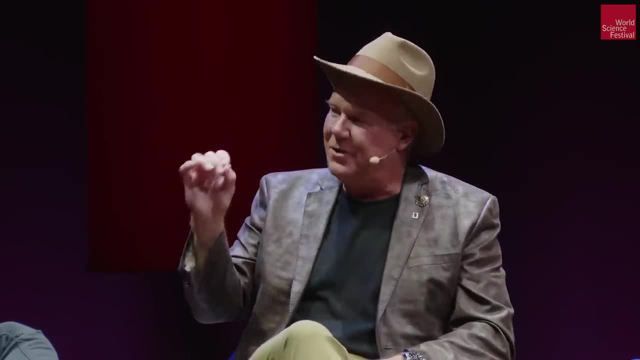 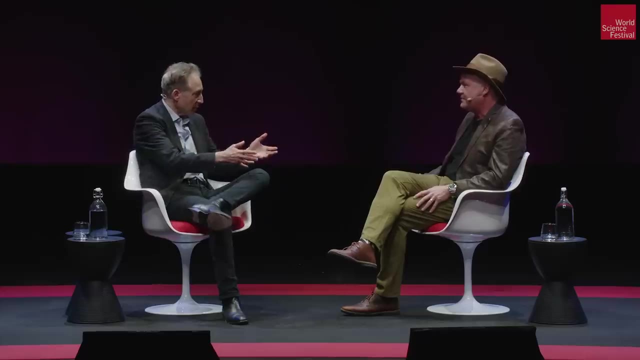 That's a human thing. In fact, if you had to talk about something, it almost defines a big brain, human behavior, That's the thing. You know. that's one of the things, And the earliest known ones to that point were like 100,000 years at most. 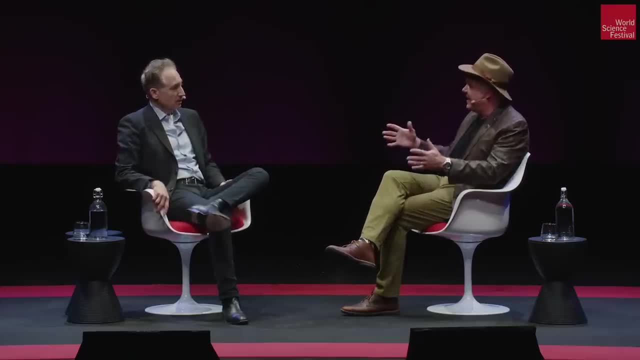 Not even 78,000 to 85,000.. You know it's young, Yeah, sure, And Neanderthal is younger than that and controversial. And I'm staring at it and I realized this is a hole in the ground. 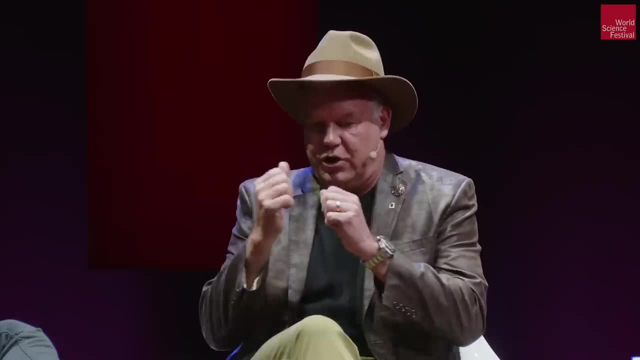 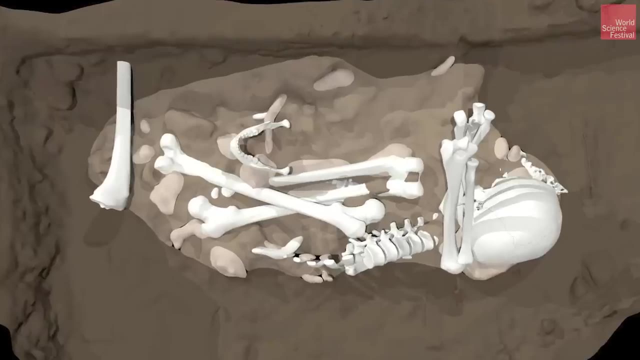 They've been digging a hole in the ground with a curled up body in it, One body in a fetal position, And suddenly I could see it from a trick of the light And I told them to stop. Oh boy, they were not happy. 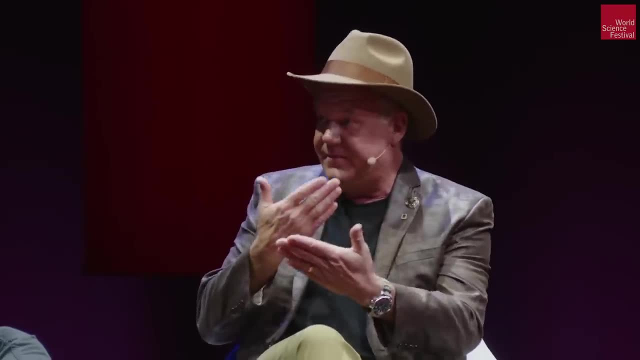 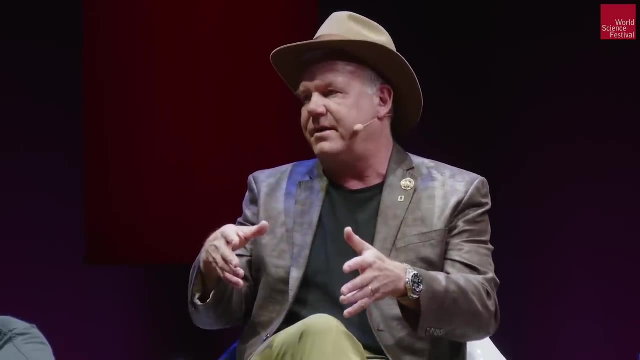 I will tell you that They were, you know, because they're right. here They are, And this is a terrible place. You know you're risking your life every time you go in. Well, we do the science, We do the excavations. 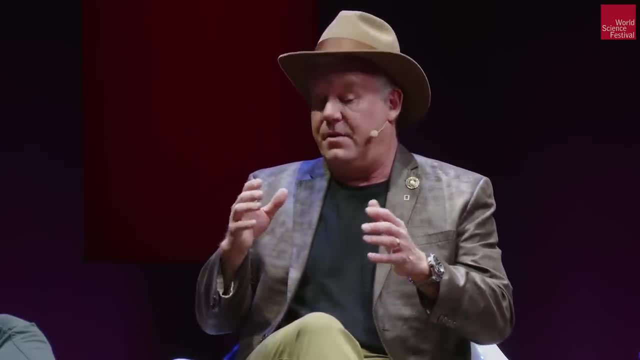 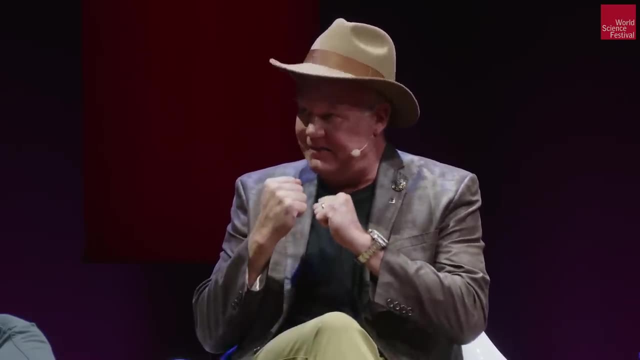 We would find out it was a burial. It was a grave I'm going to let. he went in and dug holes, put whole bodies in them in a flex position, like a fetal position. You can actually see the remnants of the whole. 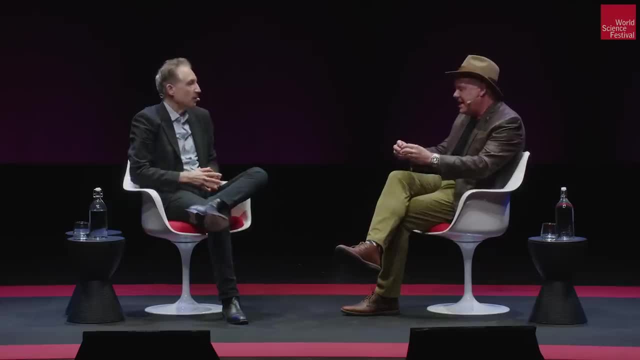 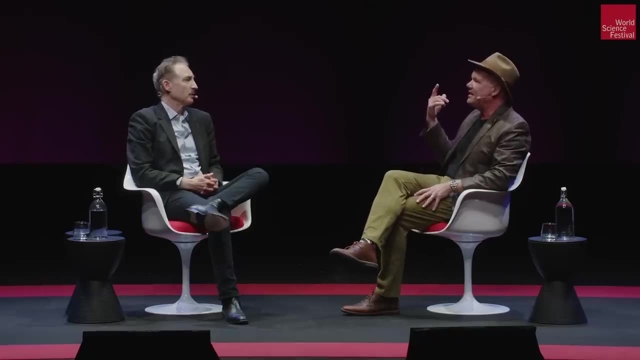 And you can see the remnants of the whole. They dug even to where the dirt clods are tossed out of it. Then they put those back on, Wow, And you suddenly find out That's a hole. So you know, they dug some about about all the mysteries. 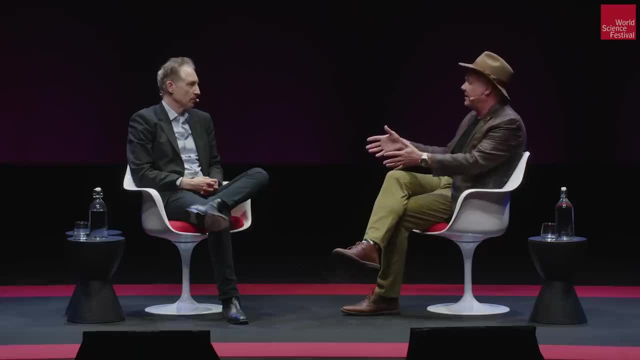 why we were getting this dense bodies. The first excavation we- uh, we worked in back in 2013,. you know where we recovered that incredible assemblage of home and parts from one meter by 50 centimeters. You know why it was four or five overlapping graves, like a medieval symmetry, where they dug through. 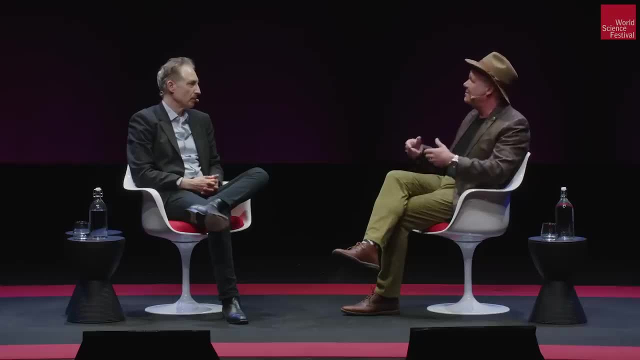 Didn't know. the body was there. Toss them together and put them back. explain why there were vertical bones, because the bodies had been sitting up and had collapsed on themselves. The material we saw on the surface was stuff that had dribbled out as the mound of 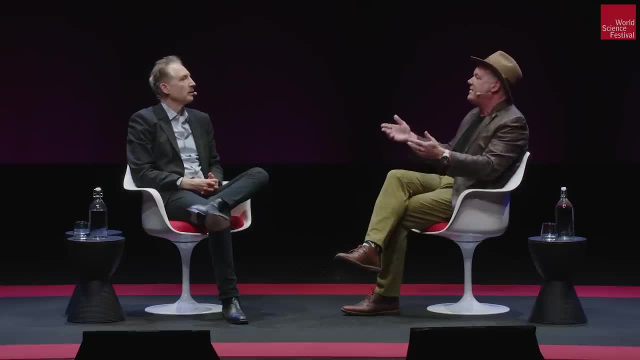 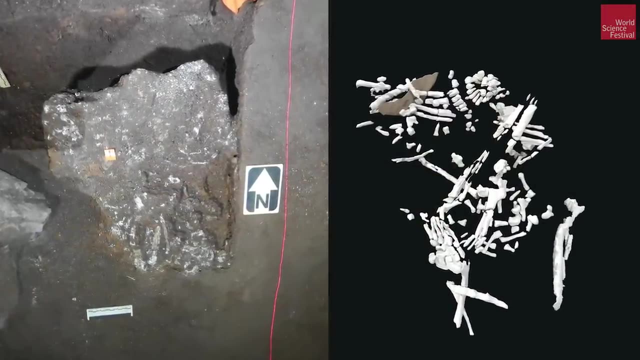 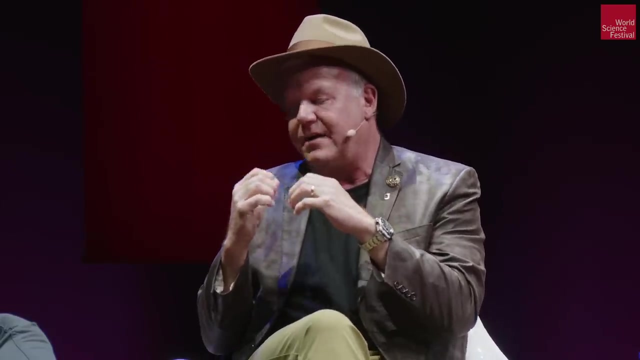 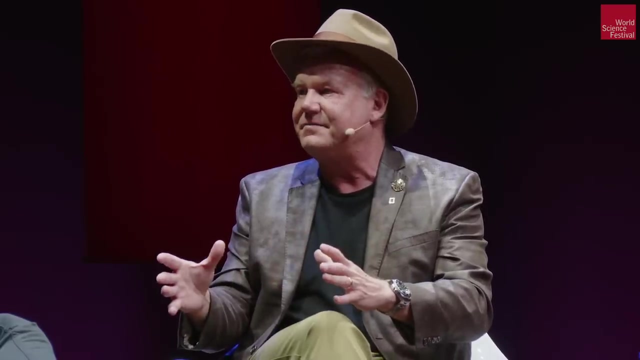 dirt settled below the bodies. Then we found the same thing in the hill antechamber. We found children, four of them in one hole, one little 13-ish year old body curled up, the whole body, two faces- just the faces of children- and a fetus in one hole in a slope. 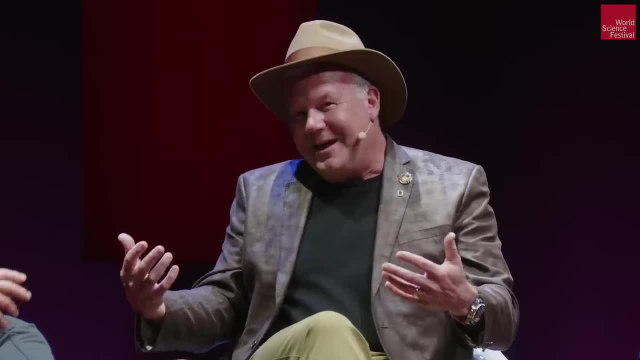 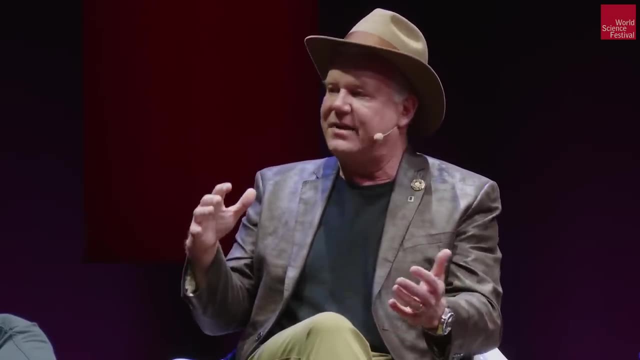 And nothing else, no grave goods or anything. Well, funny, you should ask, because when we scanned this we actually took it out in a plaster jacket hole, which was no mean feat. You've heard the description of this thing: It had to fit through. 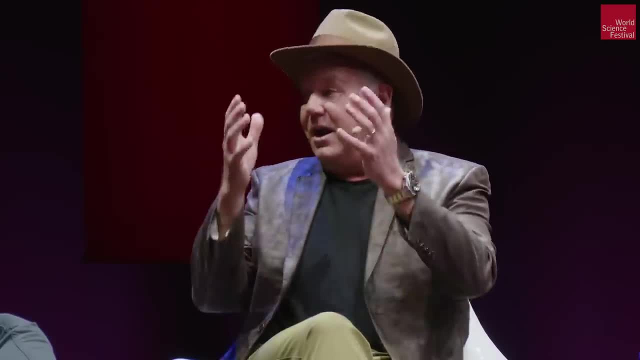 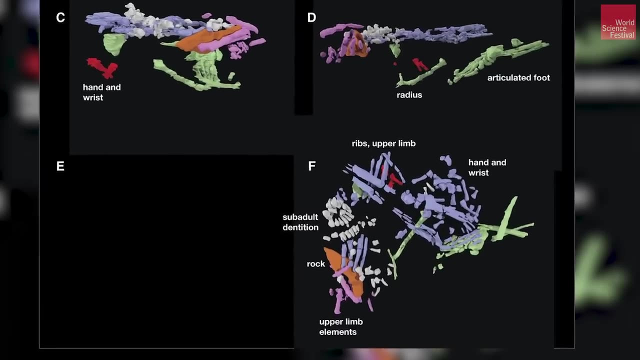 17 feet 17 and a half centimeters, So we had to get this thing up. It weighed probably 70 kilos. You can imagine getting up that 12 meters. When we scanned it with a CT scan, there was one rock in this. 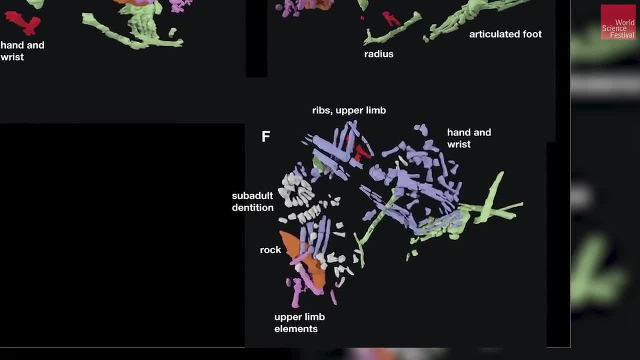 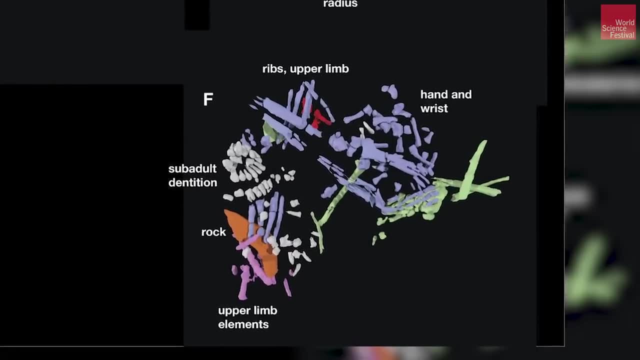 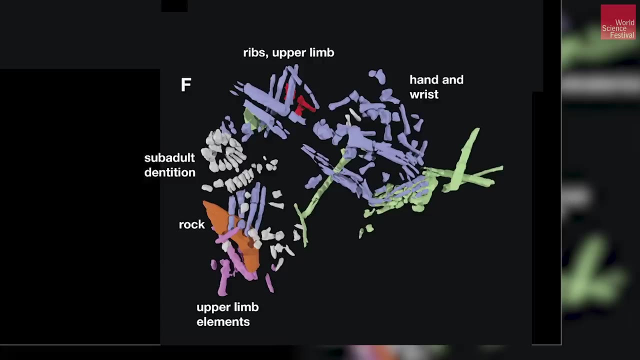 whole thing. You can see the base of the grave, You can see where they dug into it And that rock is sitting in the hand of the child, that's curled into a fetal position And it's shaped like a tool. Now, no human being has ever touched that to this moment. 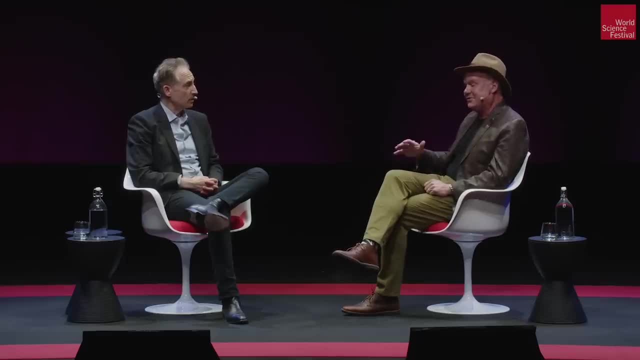 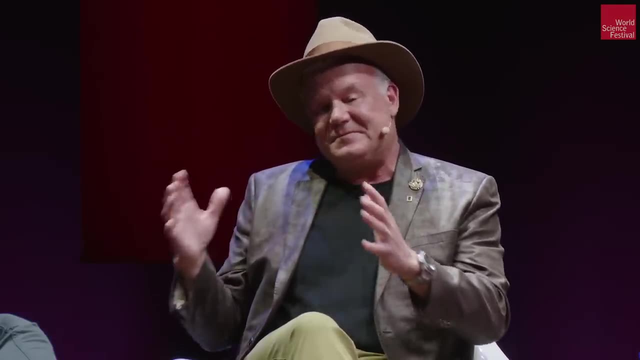 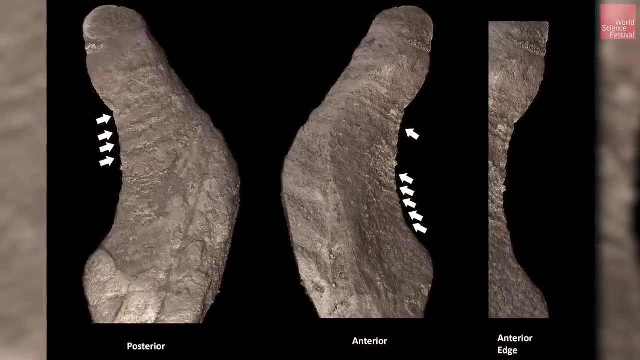 It's still in that plaster jacket. Oh is it. We've synchrotroned it. We have it at 30 microns And this paper we just published is: we've been very cautious that calling it a tool-shaped rock, But I'm not much of a betting guy. 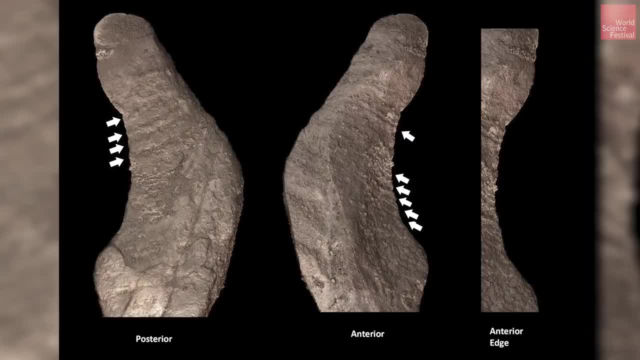 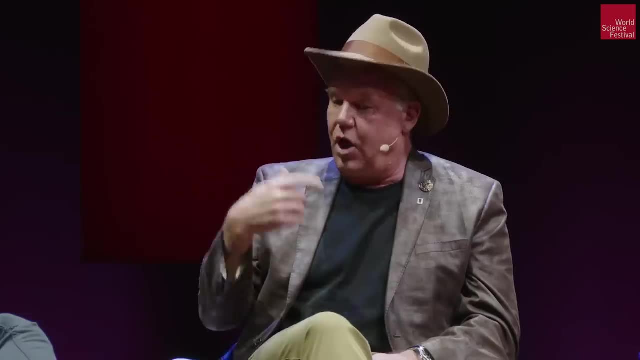 I'm a scientist, But I'll tell you it shouldn't be there. There's no other rocks like that And it's shaped exactly like the first tool with art on it from Blombos Cave at 78,000 years, done by Homo sapiens. 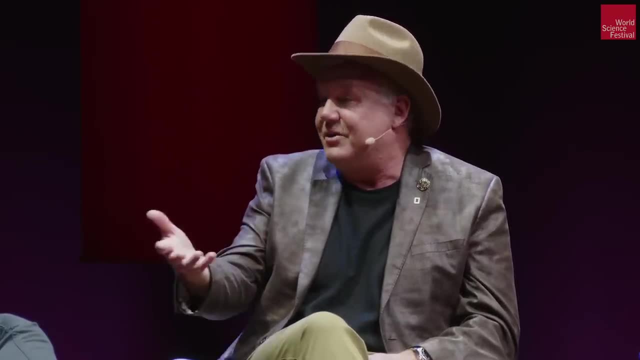 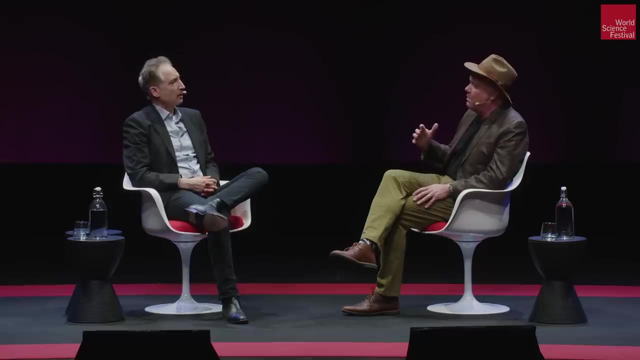 Shaped, identical. It looks like a kind of engraving tool, And is it? but it's in the child's hand, Literally sitting in the child's hand, Is it or isn't it? It's probably going to be argued for the next either hundred years. 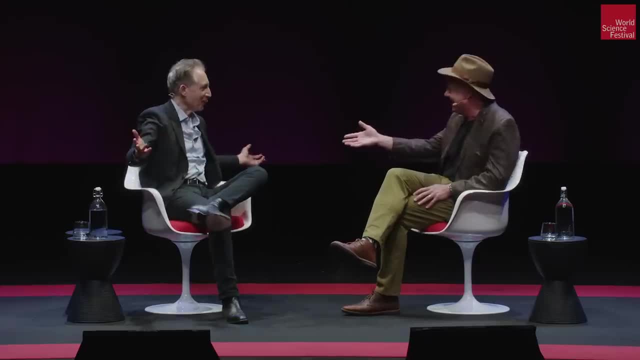 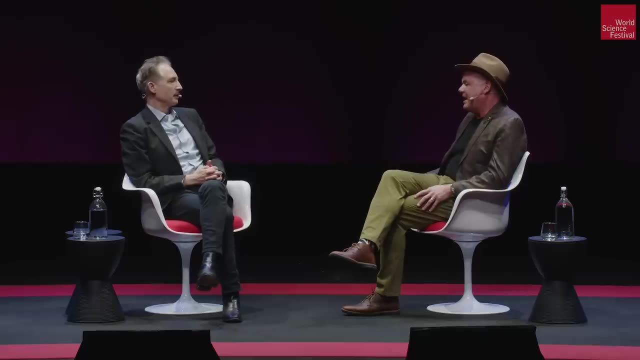 or the next few months until we find it. The other ones right, Yeah, Right. But so you started this with getting down there At the beginning of last year. I'm turning 57 that year, you know, 2022.. 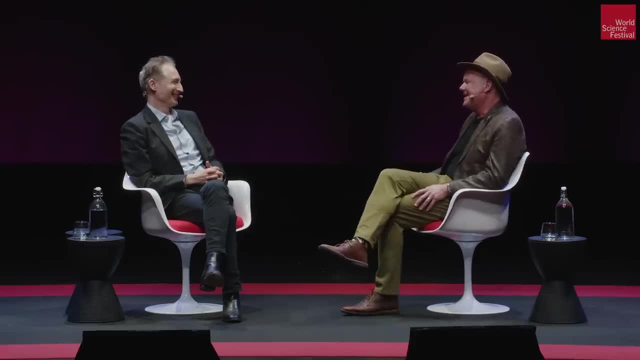 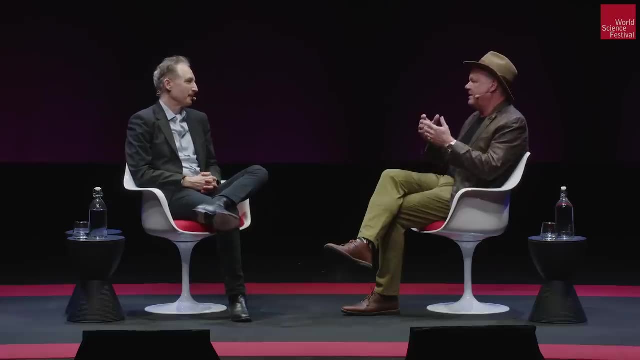 Spring chicken? Yeah, Not so much, Not for caving. And I was staring at these papers that we were preparing And this is a big deal. I think this is the biggest discovery. I think this is the biggest discovery. I think this is the biggest discovery. 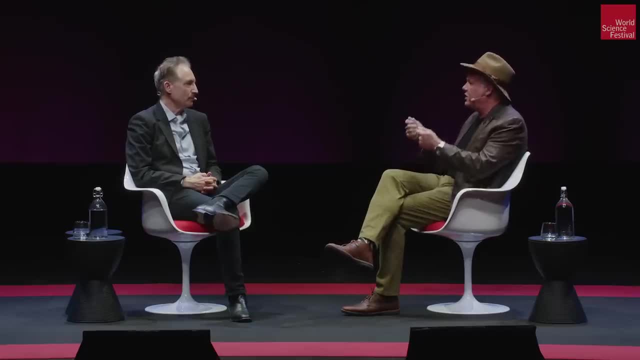 I will make them my entire career. I mean, we're about to describe a non-human species that buries its dead potentially hundreds of thousands of years before humans invent that. That's a big deal, Yeah, And I think it is the biggest deal As we're writing this paper. 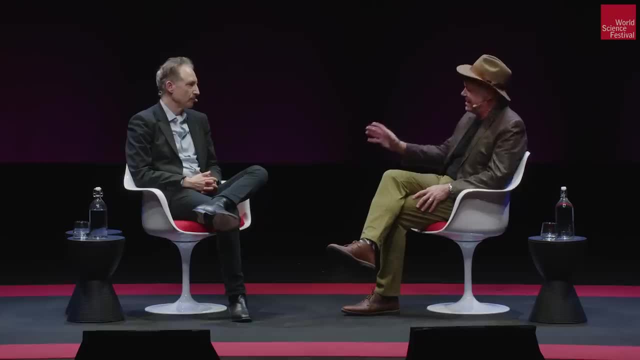 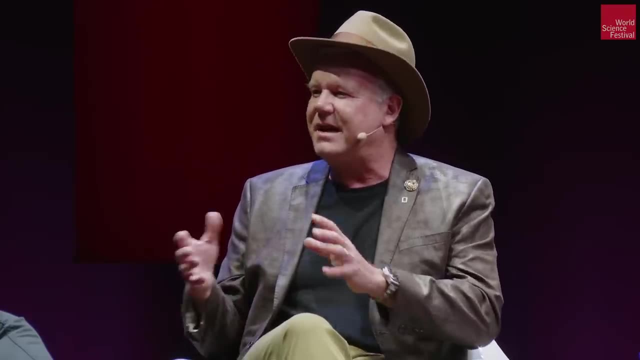 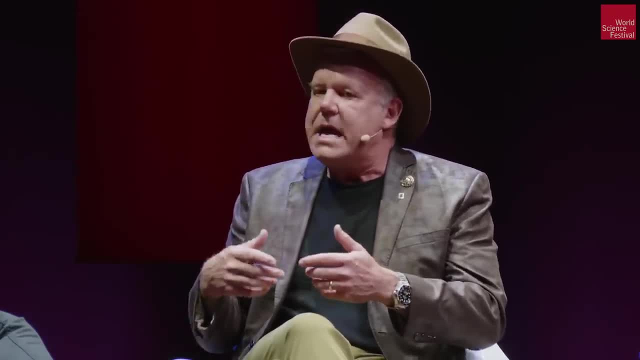 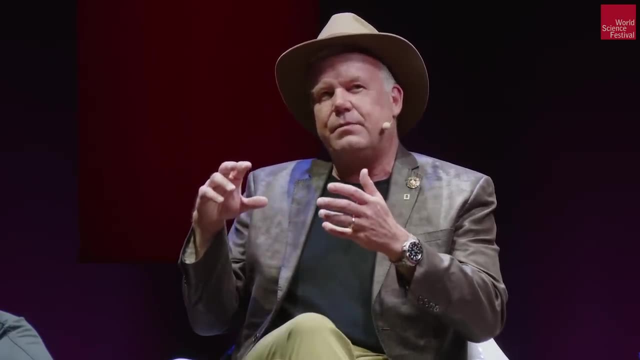 flow or movement of material, maybe water's involved, And yet all the geology, all the thin sections say that's not true. There were. there were problems with the way that that we were describing the relationship between the two burial chambers, the hill chamber and the. 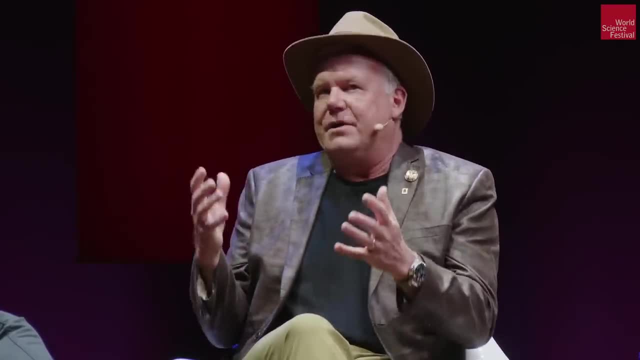 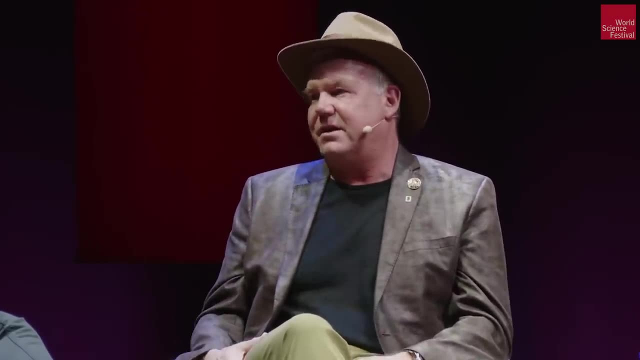 Dinaledi chamber And and there were a bunch of little sort of minor things. But I'm sitting here thinking I cannot put out this gigantic discovery that is literally going to affect archaeology and paleoanthropology forever if we don't have everything. 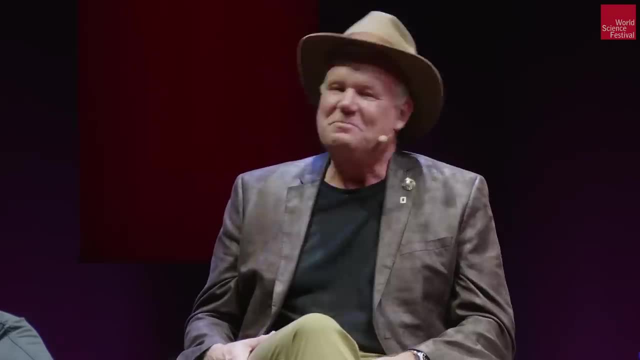 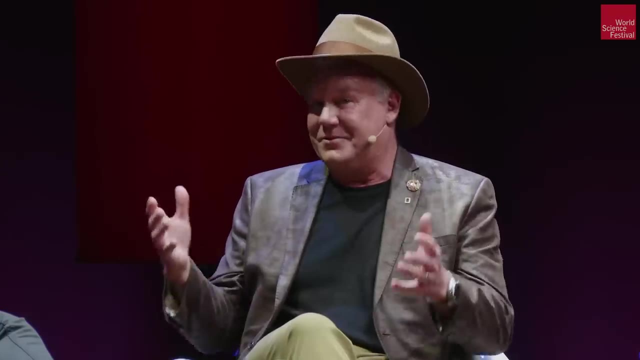 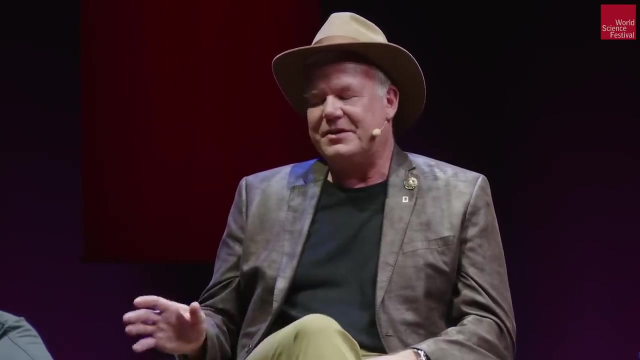 And so I started looking at myself. I had, of course, like everyone, put a little bit of COVID kilos on, And and I've always been a big guy and I'm tall, And so in February I was- I realized that we were going to have expeditions in the middle of the year into this area. I wanted to 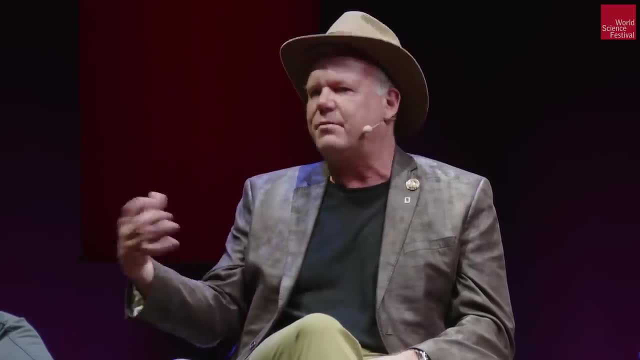 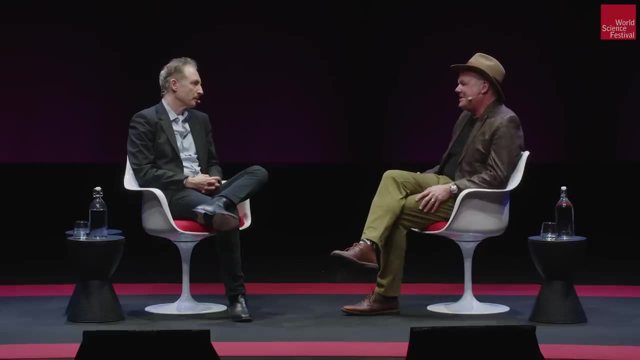 excavate in the chamber adjacent to the burial chambers- Dragon's Back, where we kid up and get ready to climb And go down. You've seen those images just now, And so I started losing weight. My wife and daughter really liked saying: oh, 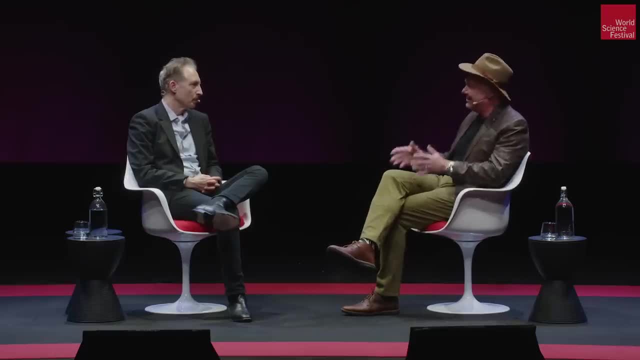 you got COVID kilos So I just was quiet, I didn't tell anyone. I started losing weight By just eating less. Eating less eating high protein, smaller portions, starting to work out a lot, and lost twenty five kilos. 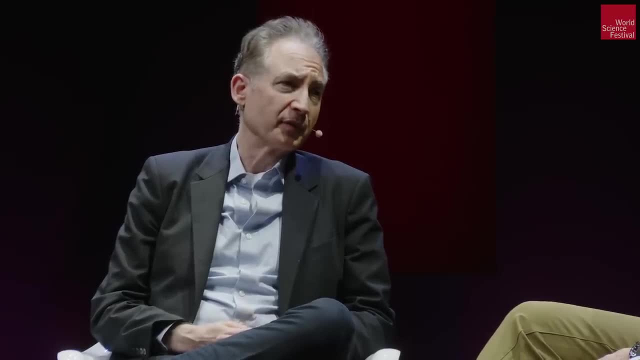 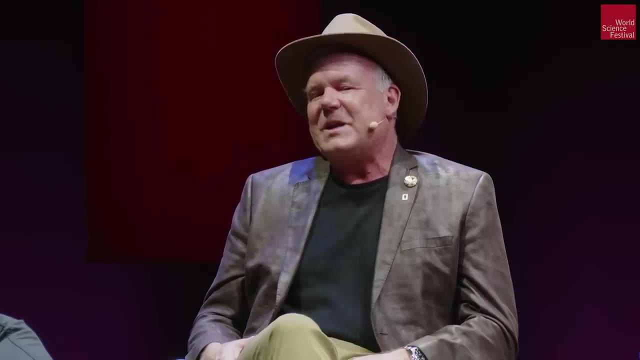 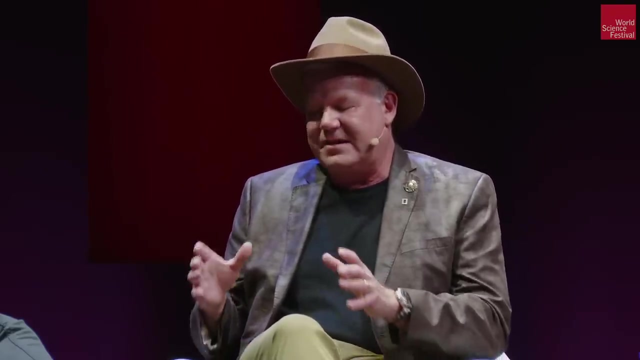 Twenty five. Twenty five kilos, So a chunk of weight, Fifty odd pounds. I'm back to 32 pounds. I've been that since I was in the the Navy And coming up on the expedition in July. we started the day we started the expedition. 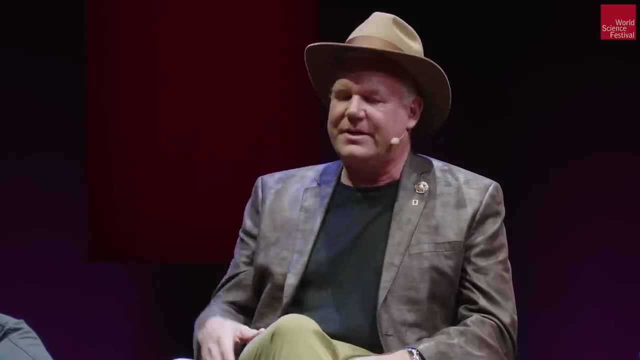 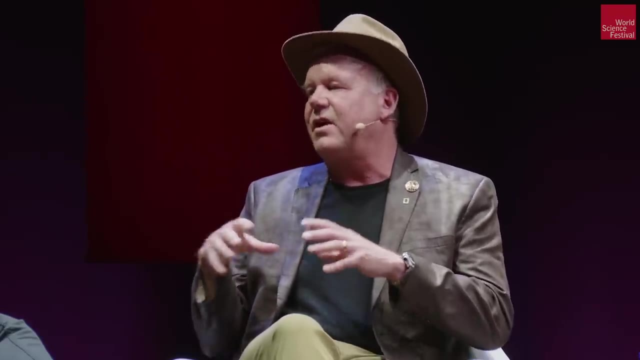 Ken Elway was going to be leading the team excavating in the Dragon's Back chamber. I climbed up- we had a documentary crew filming us at the time- and I climbed up Dragon's Back with. some colleagues had flown out for this work from the US and I got to the top. Then at the 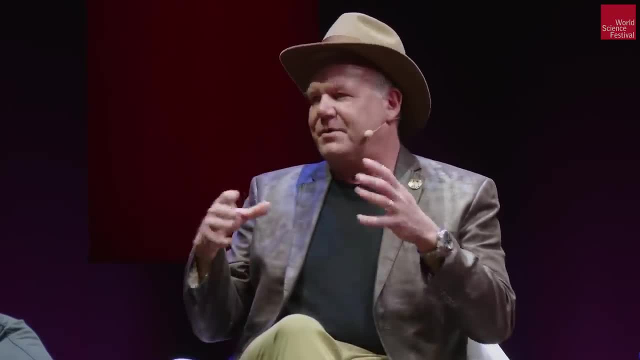 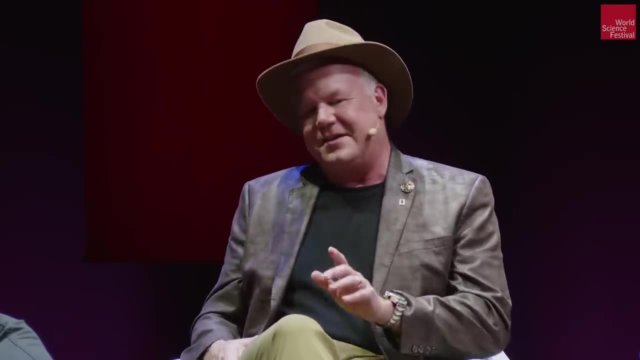 back of Dragon's Back where the chute is. I took them up there, showed them that They'd never seen it. They go down as they hook harnesses and go down this really this hard climb, And I stayed and I slid back into that space and it did something I'd never done before. I slid into this. 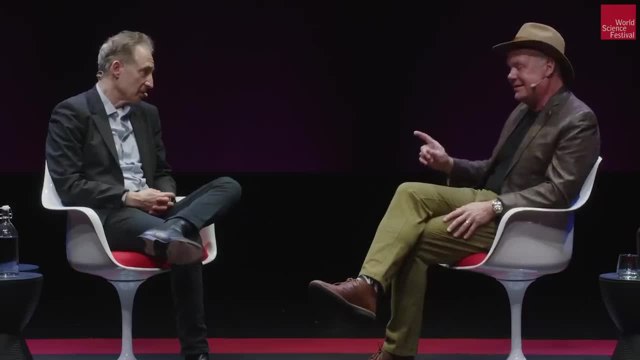 chute, Thinking you were going to go down. No, not right there, Not right there, Not right there. You would. it's too. you do not go down alone. Yeah, I don't think you just freelance, But I slid. 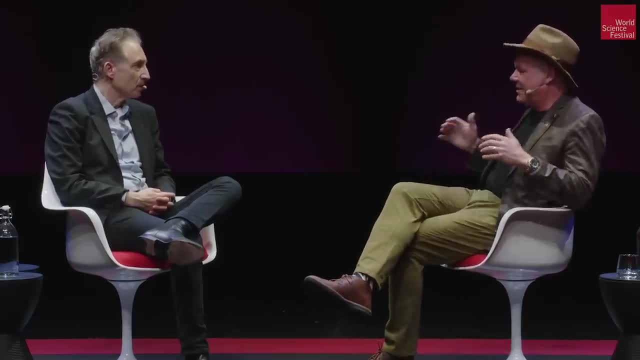 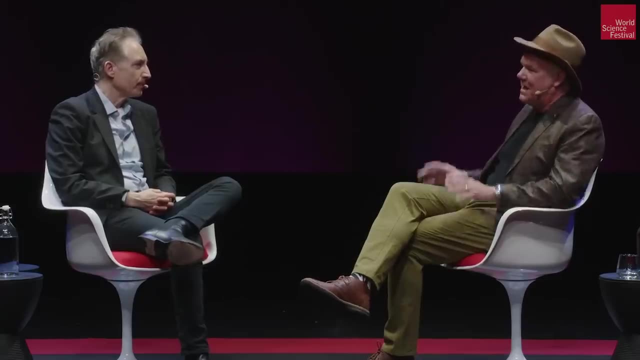 into it and dropped myself in, got my pelvis back and waist and then stared down into the abyss. So I can make this. I came out, had the days in briefing and said I'm going to make this attempt tomorrow. You should have seen. 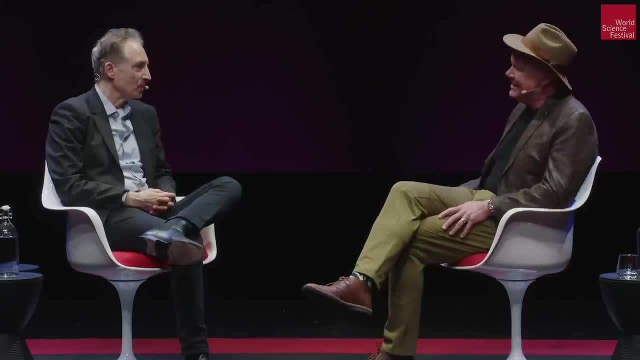 the faces of my explorers. they were not uh, thrilled, I think, But they, some of them- were like you can do this, and others were like, yeah, you could see the, And so the next morning Did you have caving experience? I've been for, you know, for decades. Okay, You know I. 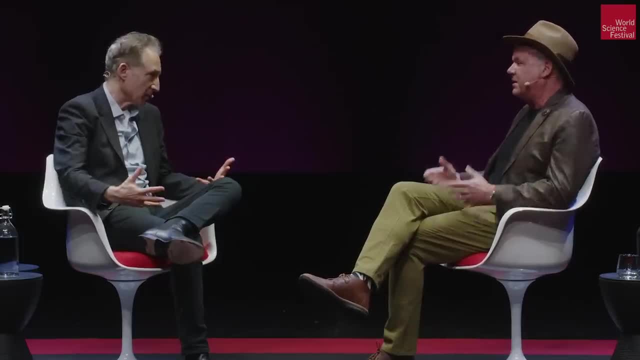 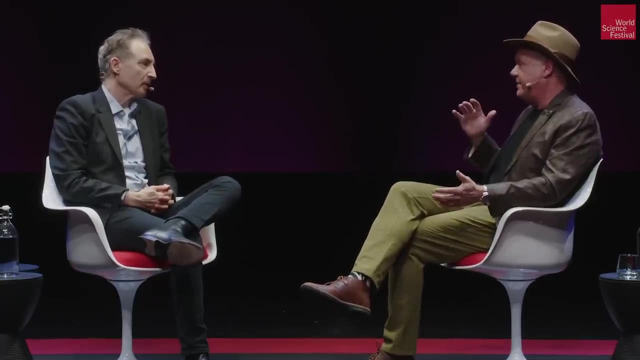 So it wasn't a matter of the technical. It's not experience. It's not technical, it's where my body can fit, And I would be by far the largest person that's gone in, both in physical dimensions and height. Only 47 humans had ever been in that space. 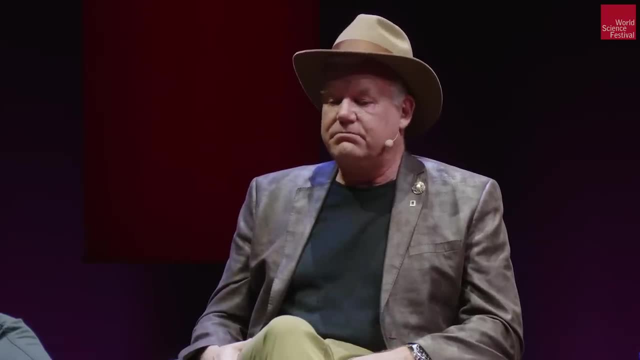 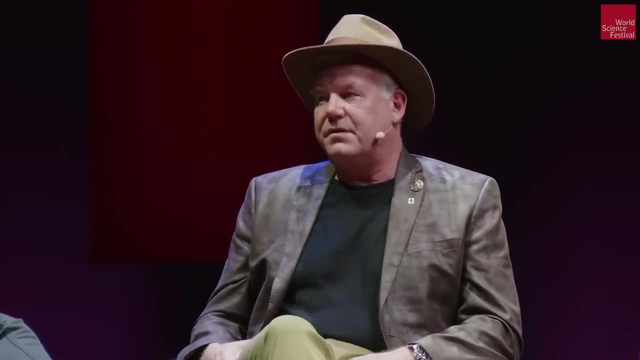 And because of the danger and the difficulty. And so the next morning I made the attempt and got in, And from the moment I got in I knew this was the hardest thing I'd ever do in my life. I mean, it was terrible. 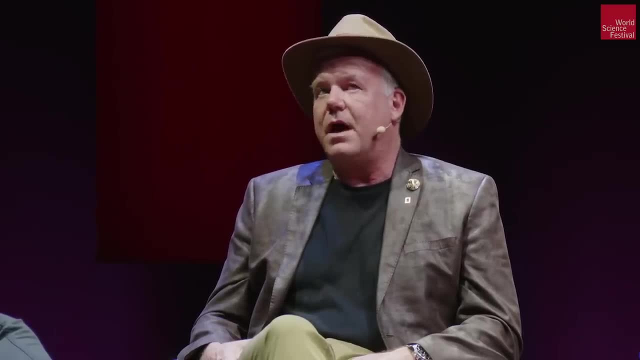 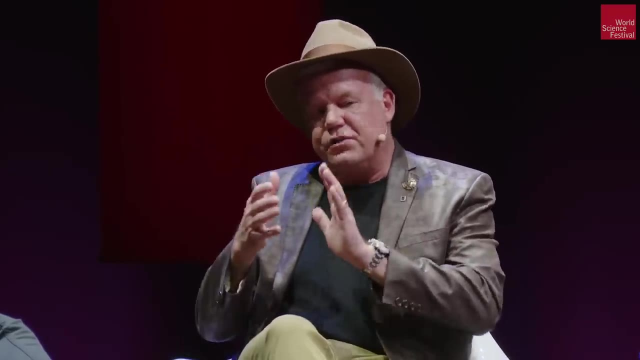 I mean, it's not a shoot- I don't know how we've described it like that- That tells you it's a vertical chimney-like thing. It's not, it's a labyrinth And you're moving actually laterally almost five meters as you move down this. 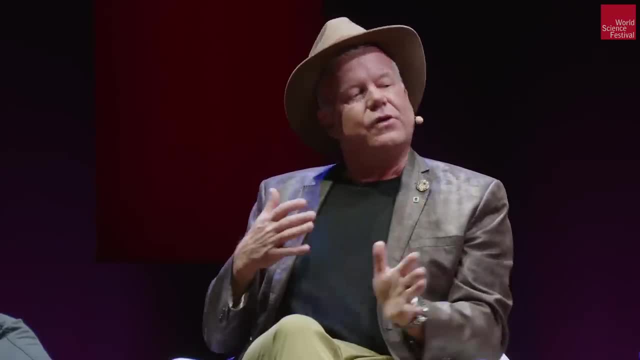 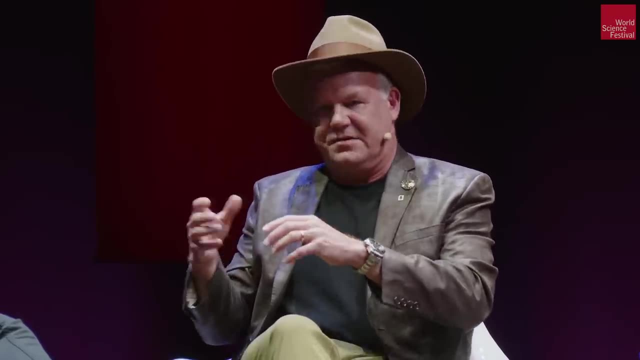 And that's a long way when you're moving through spaces that you can't even turn your head nor see your feet. And that's before you get to the 17 and a half inch squeeze, which is about halfway down, six meters or so down. 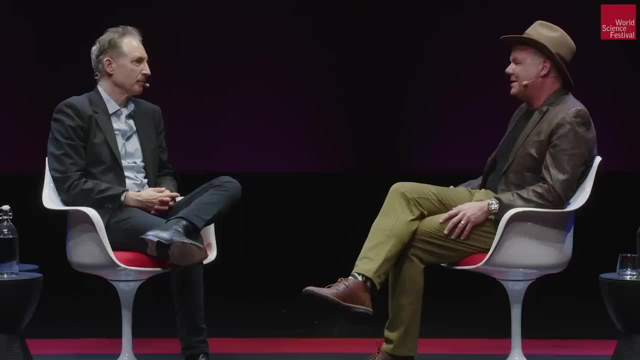 And I got to that and I pushed into it and realized that I had to make a decision Because it's not going down. you got to come up too. Yeah, Going down, you have gravity. And I hit my chest and realized that if I push this next thing, 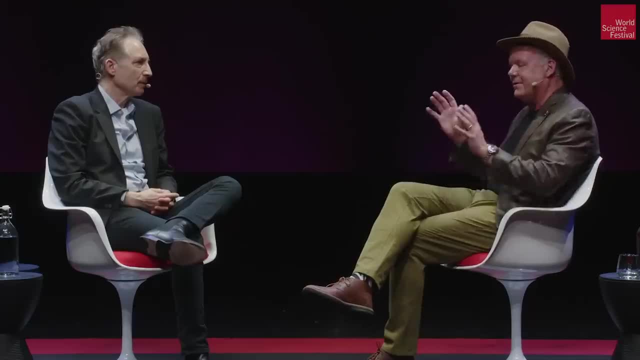 I might not be able to get out of this And we can't I answer all those questions. No, we can't modify it. It's a labyrinth of, of, of, of, chert layers and stuff, And this is gigantic ancient dolomite. 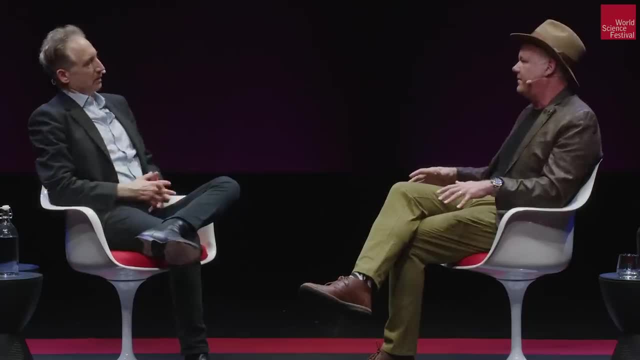 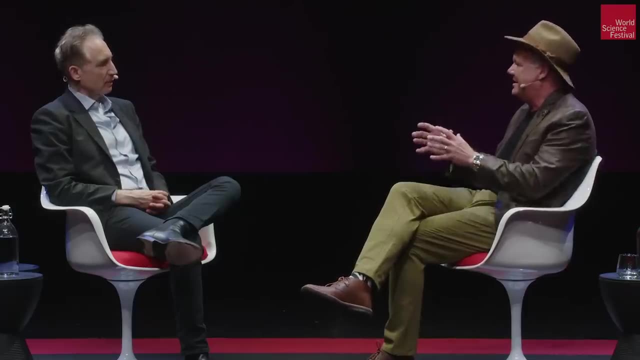 You break the wrong stick on this, that whole thing can come down. Yeah, Not only destroying the fossil situation, but killing you And the process and anyone else near you. it doesn't collapse in little bits, And so I pushed in and went on in. 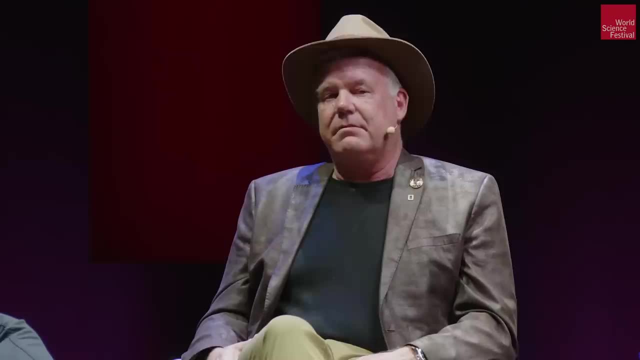 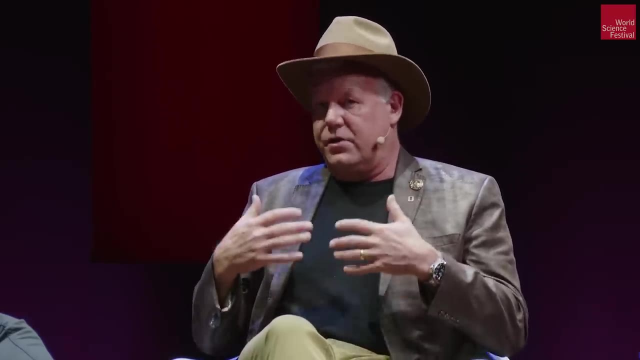 And now that was emotional everything, But I get in finally and it was hard And I'm sitting in the hill antechamber standing there And I was very emotional, You know. you haven't been able to breathe properly, So I'm hyperventilating kind of thing, probably. 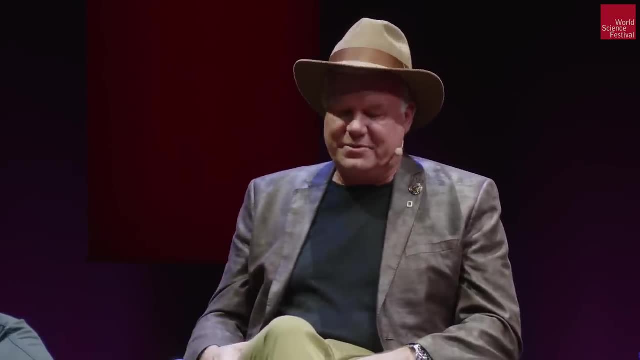 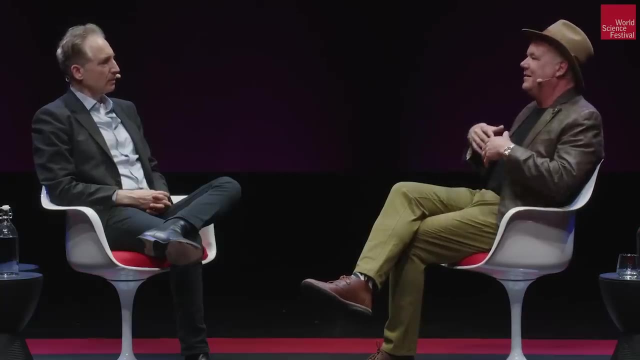 because I didn't think I'd ever be in there And I'd done a funny thing which you'd appreciate. I decided I was not going to take a picture, because I've been watching this place digitally for almost well three quarters of a decade. 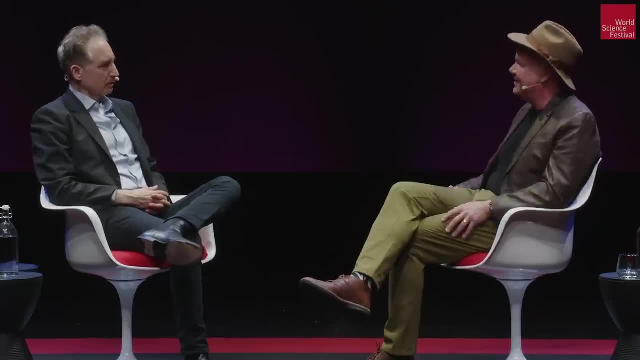 I want to narrate, So I took a narration out and I started talking, describing everything at a measuring device. and talking and describing everything, And I start describing this and I immediately start seeing things we missed, like simple things that don't mean a lot to people right now. 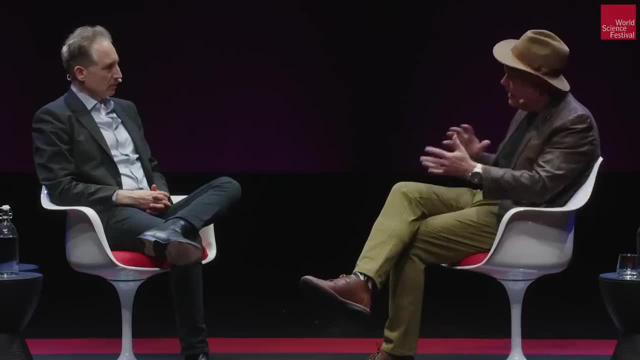 But the dirt wasn't coming out of the chute And we've actually written that. I don't know how we quite missed it, but it's coming out of another passage, So the dirt that's in the chamber is coming from the interior of the cave. 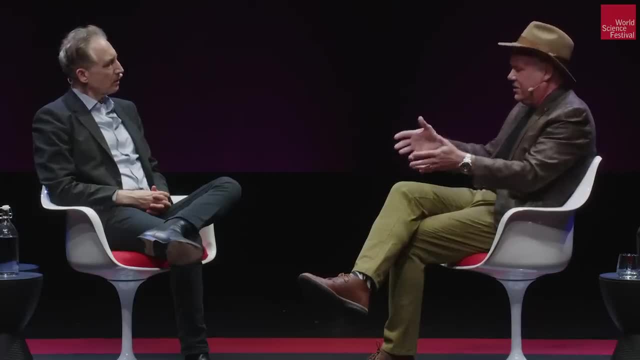 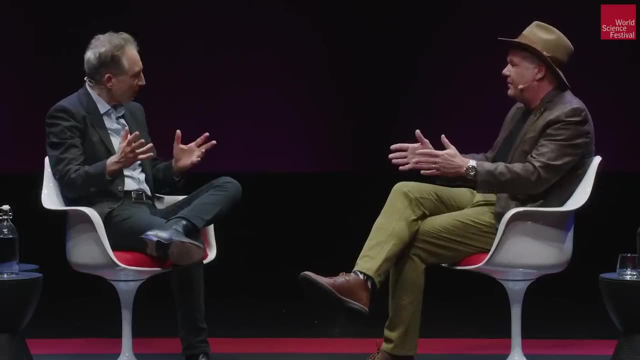 No one was throwing bodies into this, It didn't come. The dirt's not coming from where we're coming in, We're just coming in the way we can fit. I said there's another. Well, there's internal entrances that don't go anywhere. 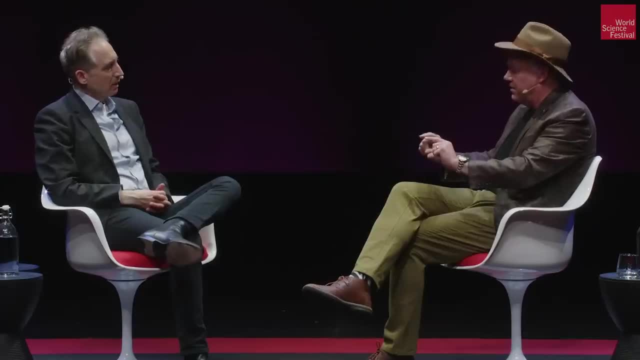 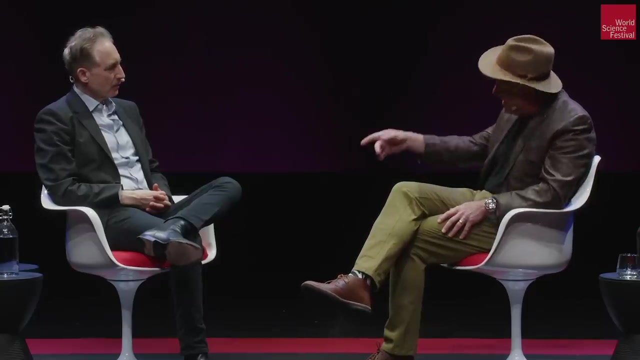 I see, OK. Then I noticed that flow stones on the ground had been broken- but not by us- in the deep past, and moved uphill Plates. Homo naledi had broken them to get to the dirt underneath, to bury the bodies underneath, because flat plates don't move uphill. 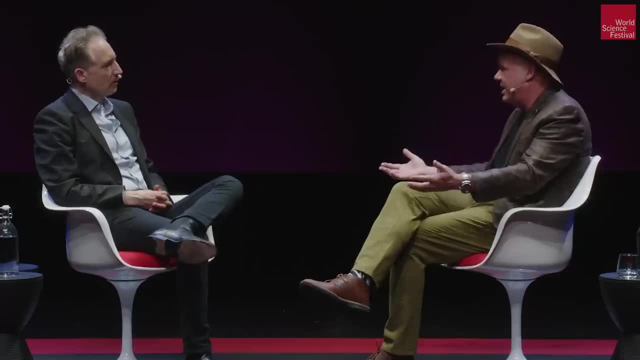 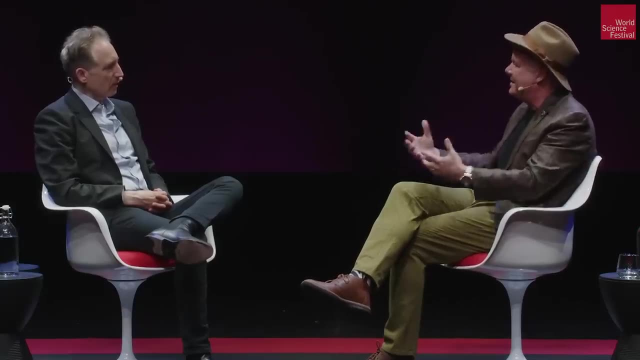 And these are little things that people have been in there, but only like three geologists have ever been in there. People quit noticing these things. You know it's backyard syndrome. You and I have talked about that before- The idea that you quit seeing places you're familiar with. 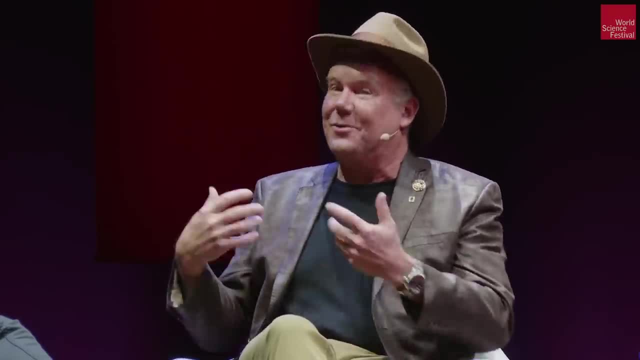 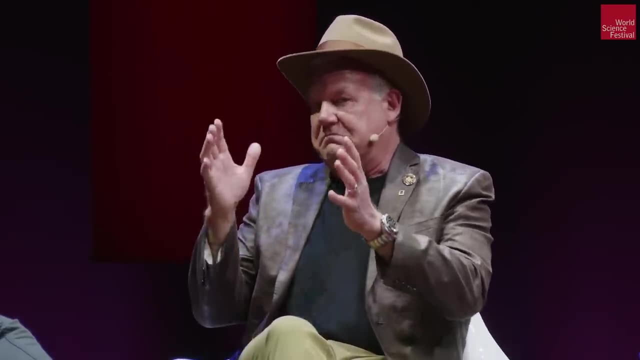 particularly places that are hard to get to. You've almost died getting there and you're worried about getting out, and you're there to do a job. And then I get to the edge of the chamber and there's this passage that leads from the hill burial chamber to the din, a lady chamber. 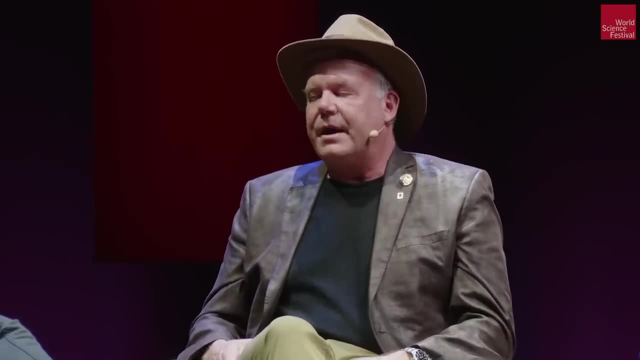 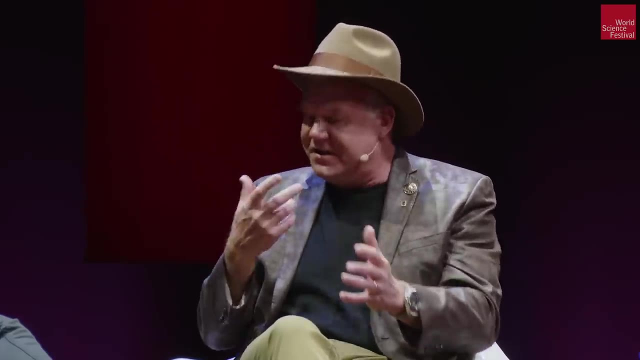 where the big burial places are, And it wasn't like what I imagined, seen on images. When you're there it's totally different. It's a doorway, And I say this. you know, I say it's smaller than I thought. 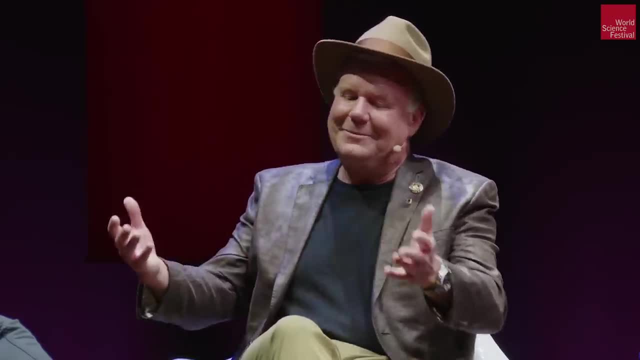 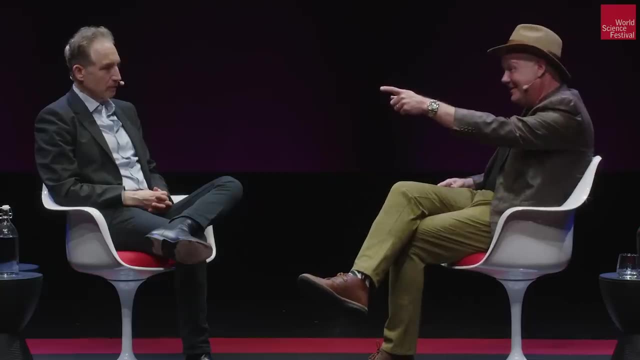 It's? it looks like a doorway And I'm I'm an archeologist. I see doorways. What do you see Above doorways? Well, you see there's a doorway. What's above it? The exit sign. Yeah, 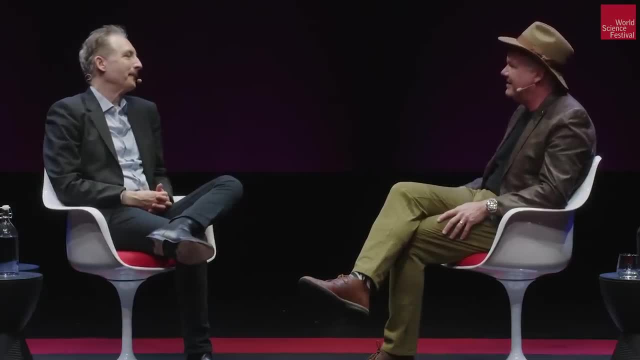 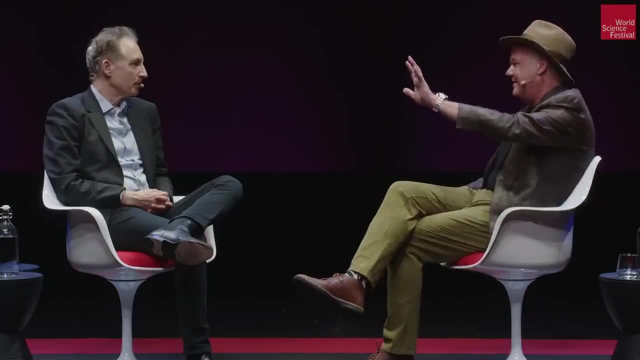 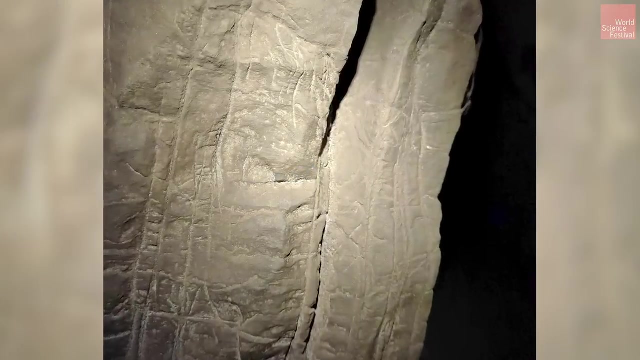 A sign, Yeah, And I looked at it and looked to the left and actually couldn't believe. what I saw there on the left hand side were carvings, engravings, symbols. First thing I saw is a cross, One up right side up, one upside down. 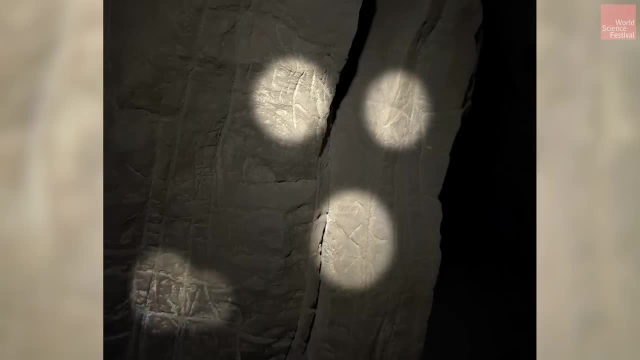 A box, a square, and you saw triangles. I saw a fish shaped image. I mean, I don't know if it is a fish or not, It's a. it's a non geometric image, Ladders. It's incredible, All etched into this 2.9 billion year old rock. 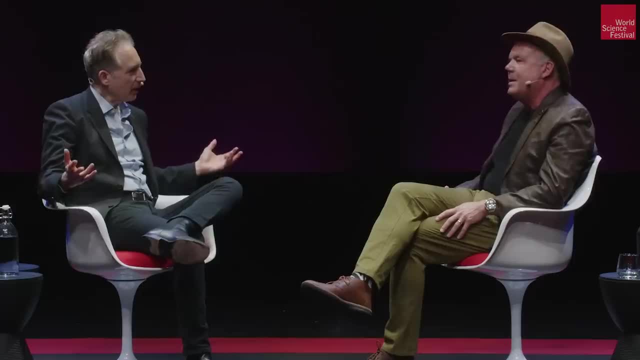 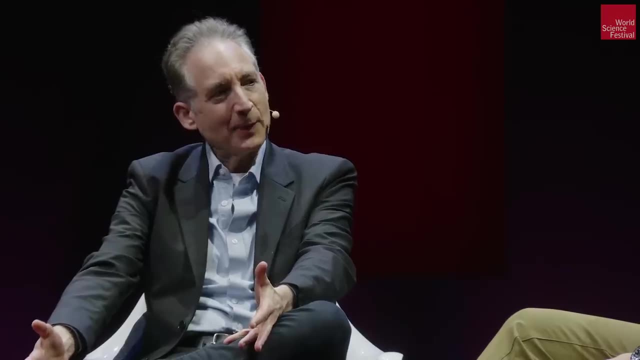 and people had just walked by them. Isn't that insane? I mean, I know I gathered the backer, I get it, But you have trained team The world's great, You know, wouldn't some- I did it- surprise you? 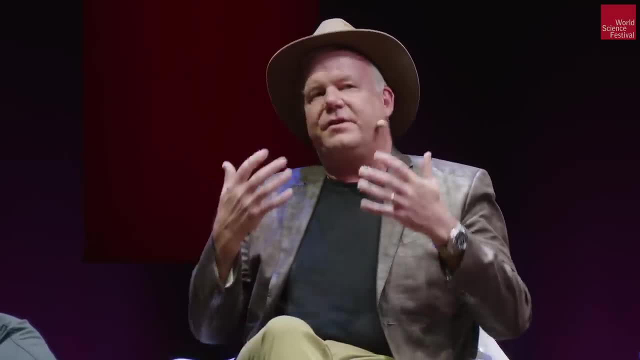 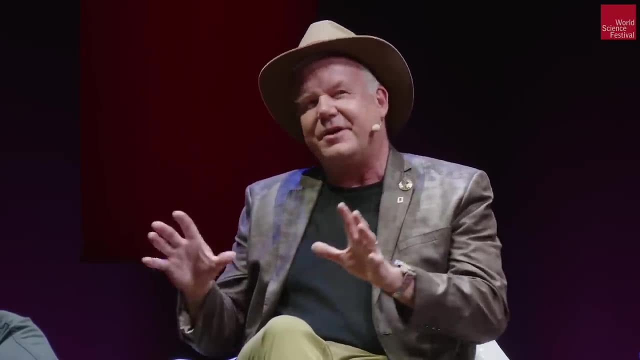 You know I've thought a lot about that, obviously because you know I go to them, I look at them. I almost had a transcendent experience. It's really weird. I'm often embarrassed to even talk about it like this, but 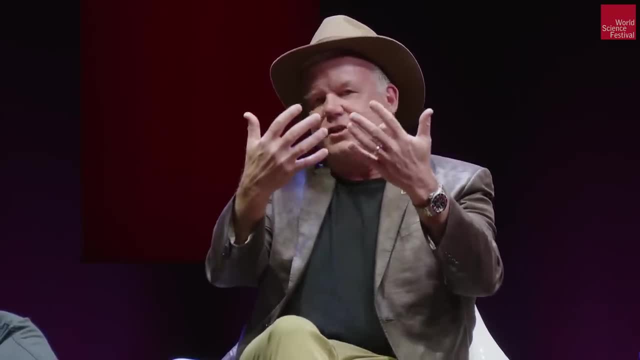 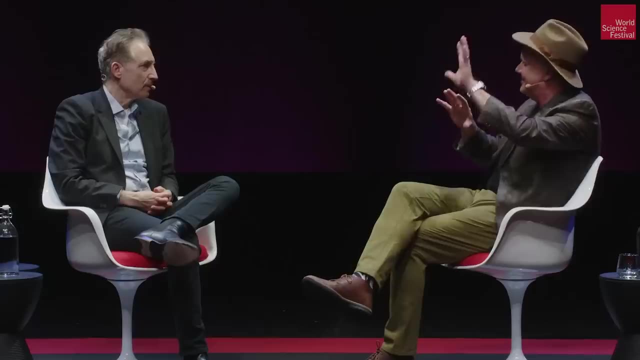 I know why it happens physiologically. But that material, I looked at them and they actually floated off it. When I turned on a black light onto them they floated in space. you know, kind of like Queen's Gambit sort of stuff that you see a beautiful mind. 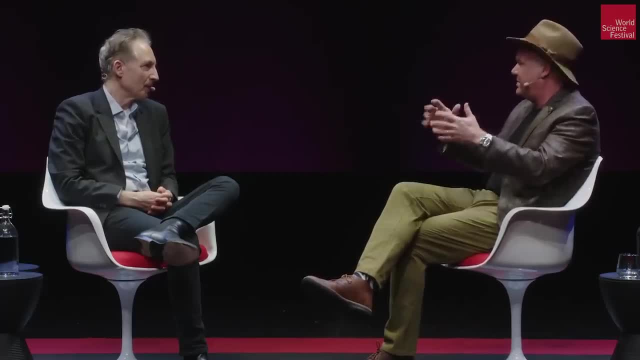 And I know why it happened. It's a light shift phenomena. You would understand that it's what happens when you see car lights at night as they move in the opposite direction. You know why your brain does it, But yeah, it's still very weird, Yeah. 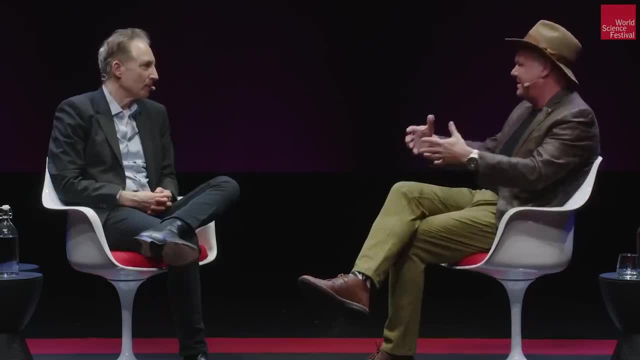 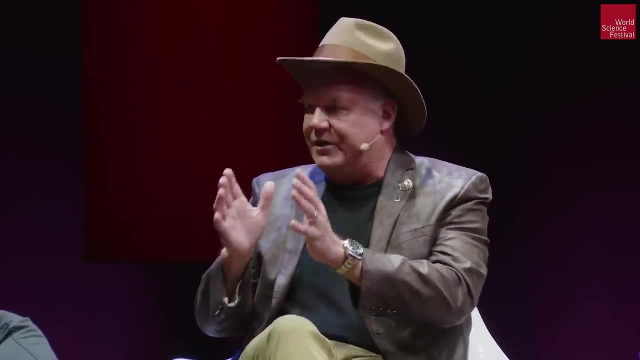 I was probably as close to a trance state as you could probably get, you know, from exhaustion and fear and all that kind of thing. But I think that the Pathfinder syndrome had sort of built in is a dangerous place. The first people in are risking their lives. 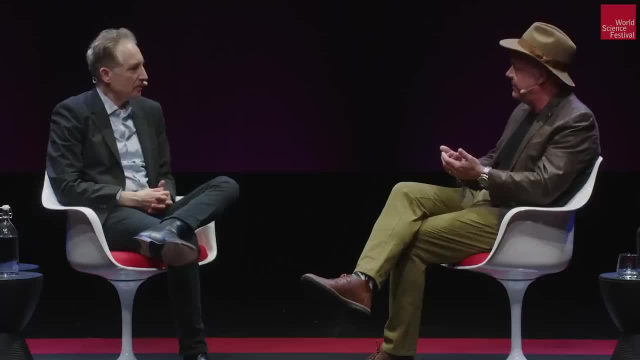 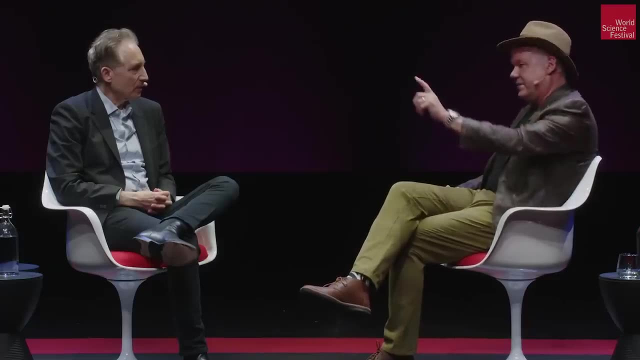 Everyone's preaching: Get back alive. You know, that's the thing. That's why some few people live and you become very mission focused. We were there to dig. Almost always we were digging in those far chambers By the time the third, fourth or fifth person has gone in. 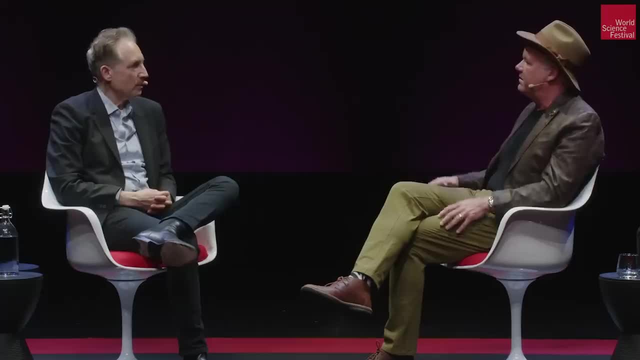 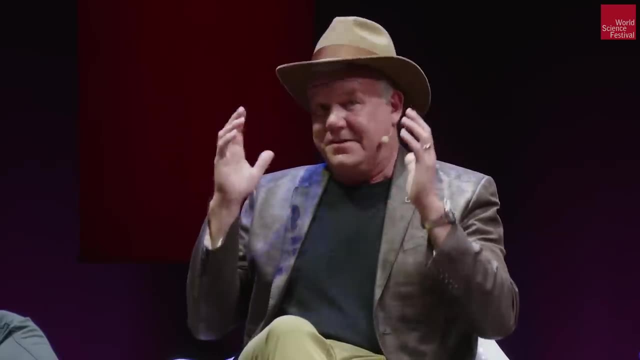 everyone gets the explorer mindset, which is so dangerous. Smart- Just what you said. smart people have been here, that they've seen everything It's here. That's not my job. My job is in there. I think that's what happened. 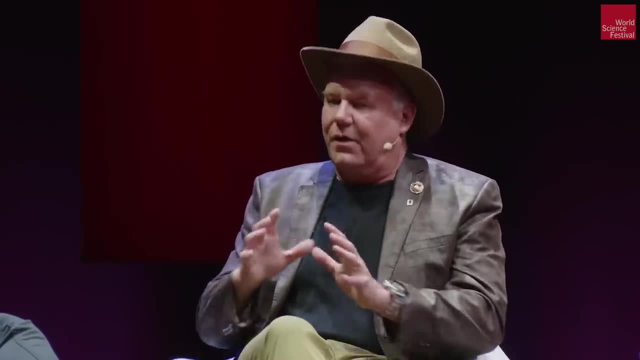 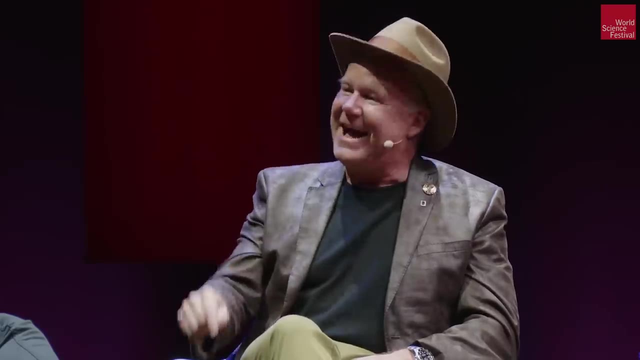 And I'm there with a different mindset. one to solve problems. And two, I know for damn sure I will never be back in this space. This is my shot. This is my first and last time to be in here, Right, Anyway, I describe them. I am blown away. 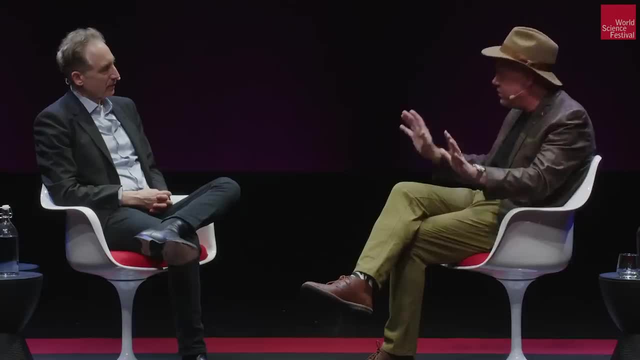 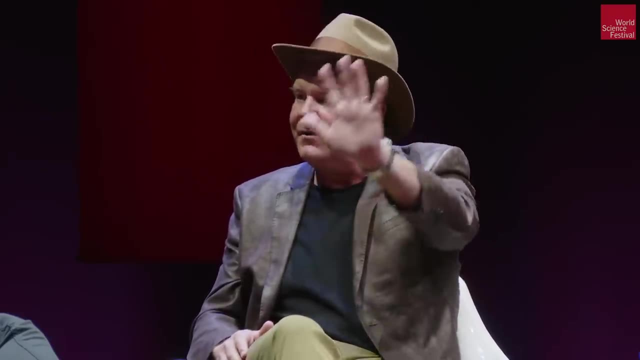 I can't believe it. I'm looking at engravings and I know no humans have been in here other than us. These aren't us, And I could see there were layers. They've actually erased Older images with dirt from the ground and then carve through them again. 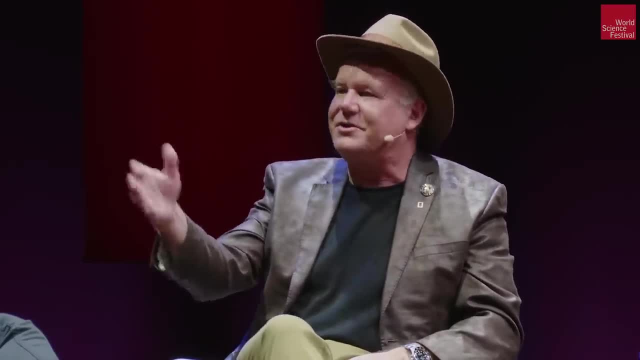 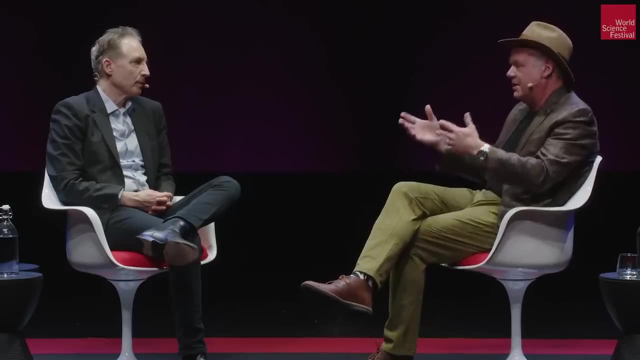 maybe to highlight them. We see that in upper Paleolithic images all the time And these images, I knew, look like the things we see. you know Neanderthals doing We see. well, not so much that, but humans doing. 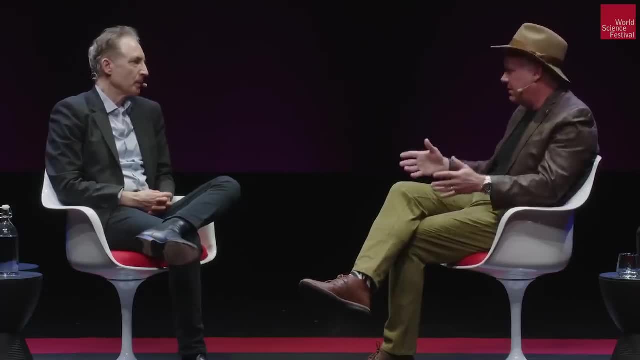 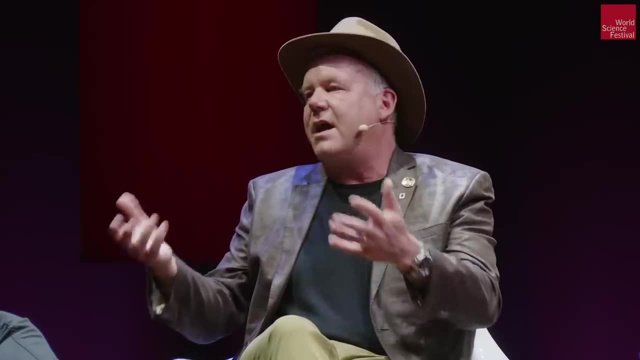 Yeah, You know, the earliest engravings, these geometric forms. It looks like the earliest art. Anyway, I go through, I go through the whole cave over the next three hours or so. I discovered soot on the ceiling that we hadn't seen. you know, our explorers hadn't been looking up. 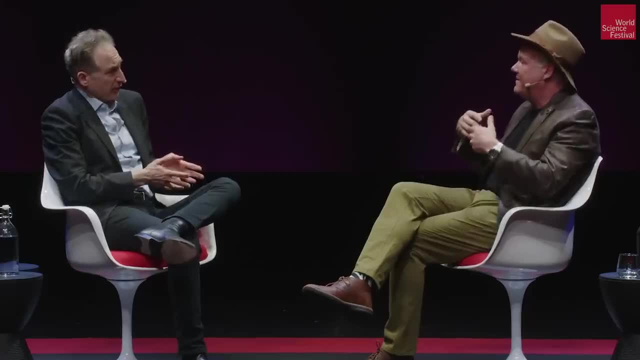 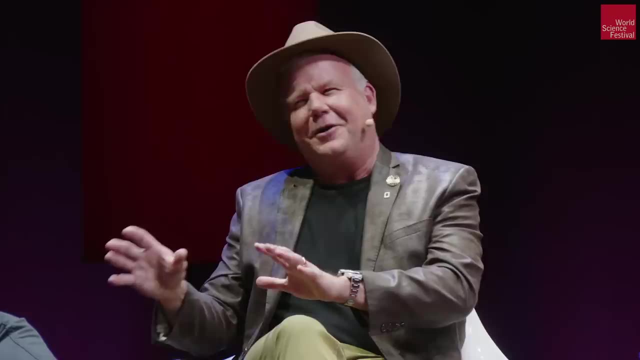 Fire was in there and it was right in front of our eyes Because in earlier accounts, remember, it was saying there's no evidence, No evidence, Fire. And you, yeah, when we, you and I, talked about this. you know fire is hard to see. 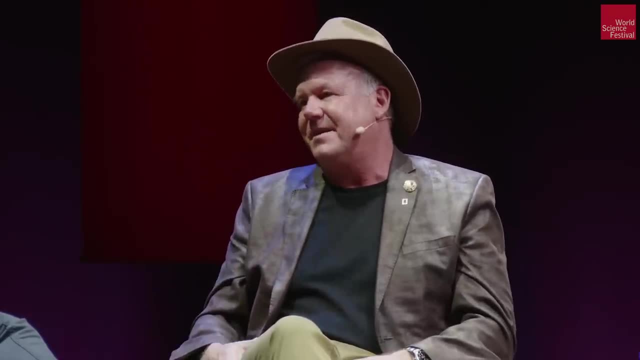 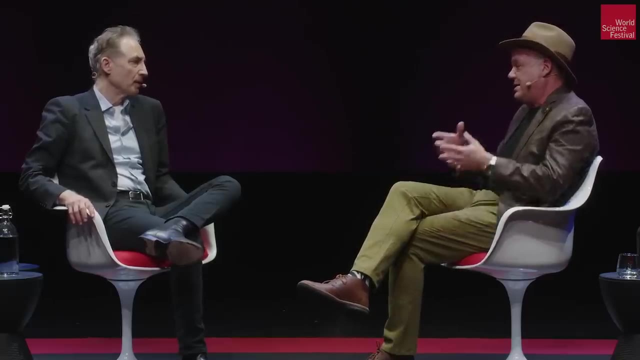 And a couple of we talked ourselves out of the obvious. Scientists are human too. folks, They're human too. Hmm, And you know you, these things happen all the time. There are thousands of scientific discovery stories just like this, aren't there? 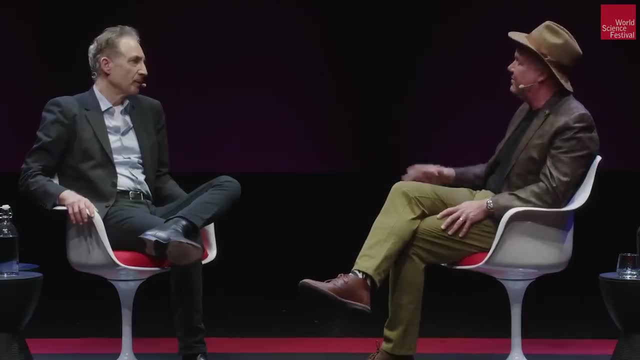 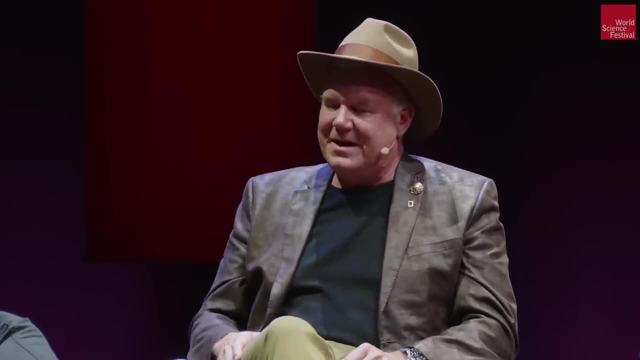 Yeah, Where something, someone suddenly sees something right in front of everyone else, And I finish and I'm coming back down this passage And I decide to do a funny thing. I'm coming out. I'm. all I'm thinking about is: I've got to survive this climb out. 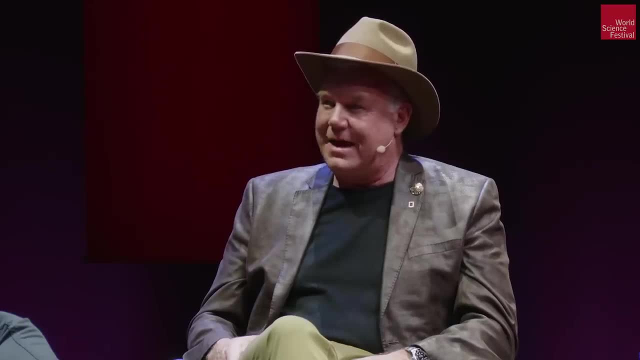 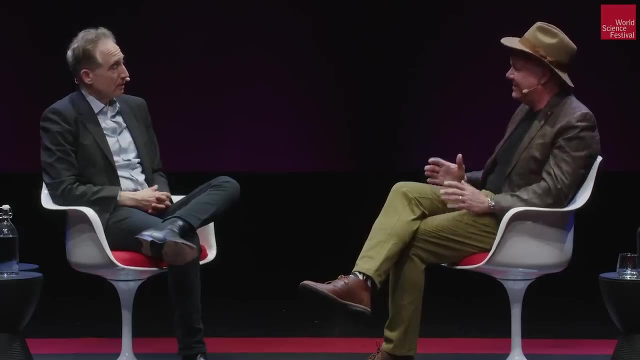 And then I say: you know what? This is my last chance in here. I want to be the height of Naledi, And so I got down on my knees in this passage and started crawling And I got back in Just opposite the back of that. 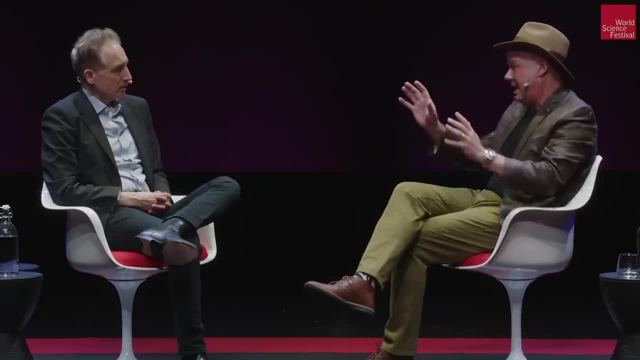 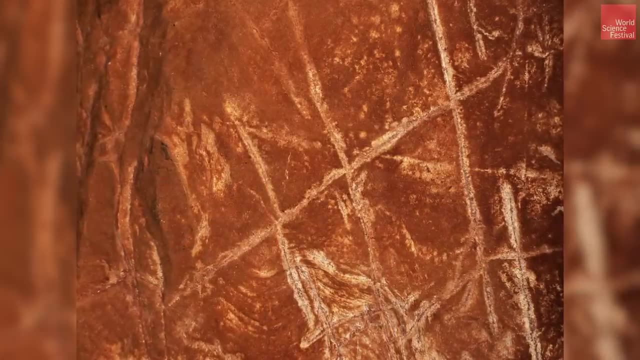 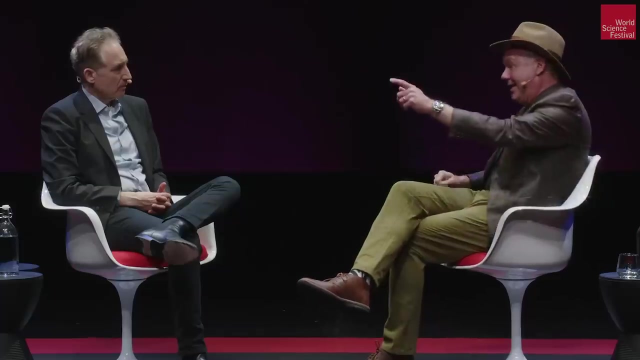 Those images carved on the left hand side of the door, So now it's the right hand side of the passage. I see this gigantic crosshatch type hashtag Crosses- I mean gigantic- right there, As bright as that exit sign. 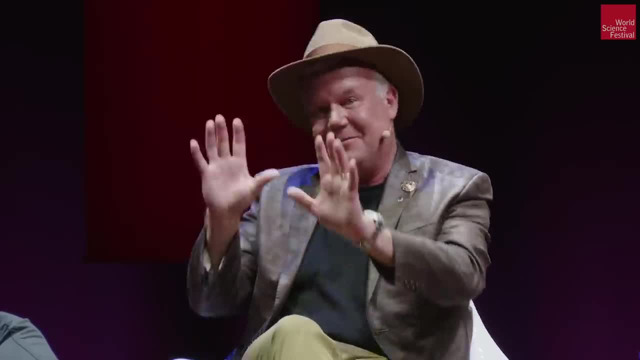 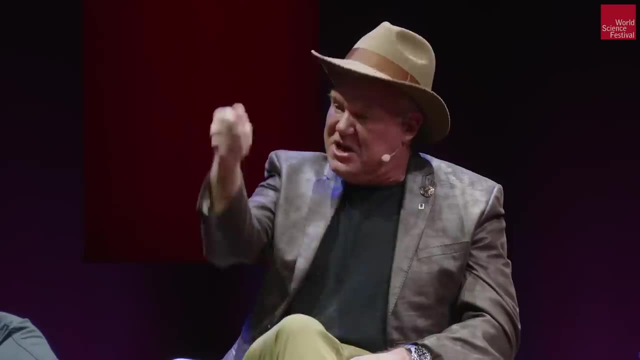 You know, I'd even walk by it on the way in, And there it was, carved deep Into this over an algal stromatolite billions of years old and then done multiple times. Somebody worked hard, hard and multiple, multiple times. 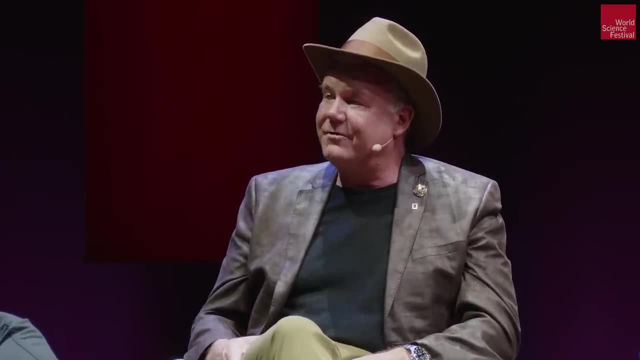 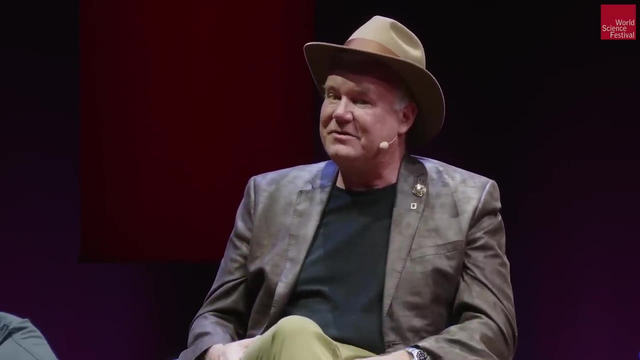 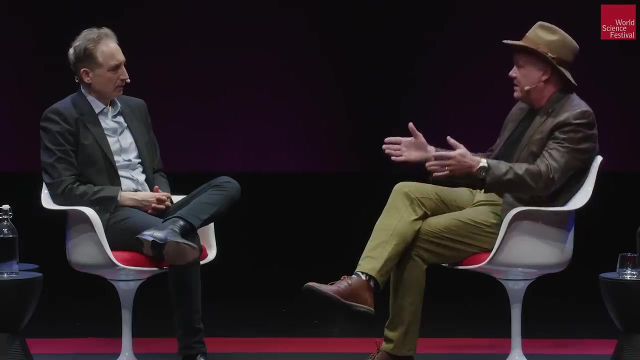 You know, I discovered the earliest symbols ever create. first time, humans have recognized symbols created by a non-human species with a brain slightly larger than a chimpanzee. We've, we've seen. That's something. I mean none of us. As you know, burials are one thing. 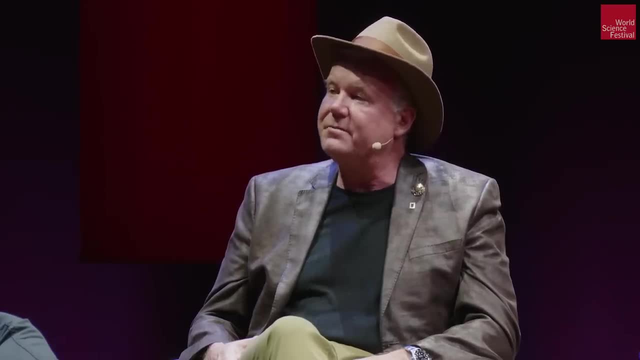 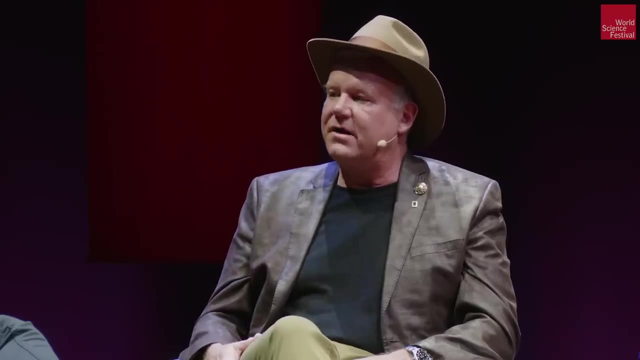 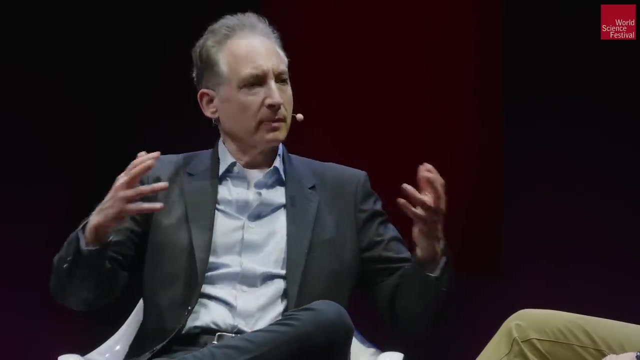 Meaning, making symbols carved into the wall above those burials and in the passages by. We thought that that's us, It's not us And it's hundreds of thousands of years before us. thinks about that Now. one question immediately comes to mind. 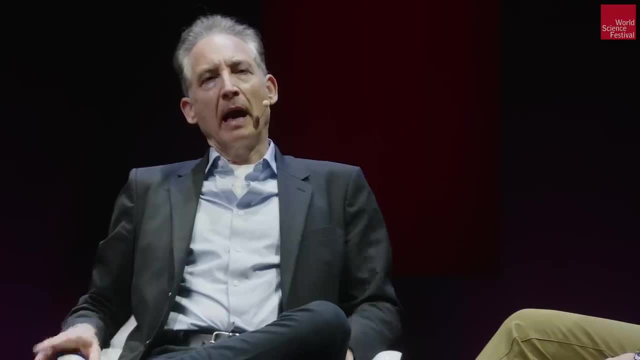 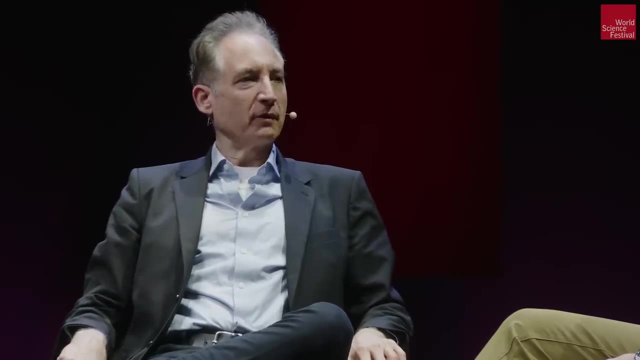 I'm sure it's been thrown at you a thousand times, but at what point do you think You Think you're reading more into it? Like could it just be like the mindless doodles of the unconscious mind? Just you know they're down there and I'm not reading anything to it. 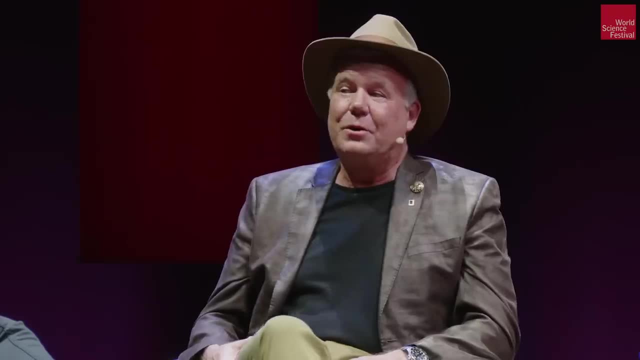 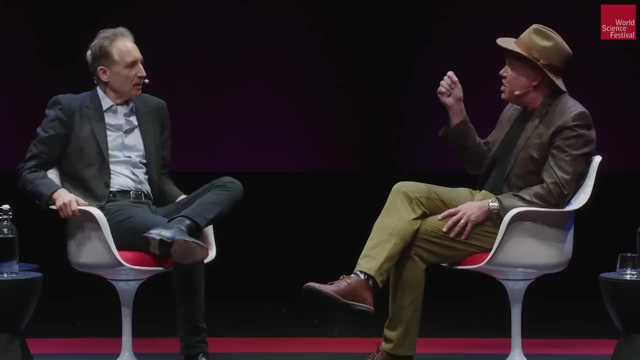 I haven't said the word art. Yeah, I haven't said the word. I said they're meaning making symbols. Even an unconscious doodle is a meaning making symbol. right, Nothing does that. Nothing on the planet that we are aware of has ever done that. 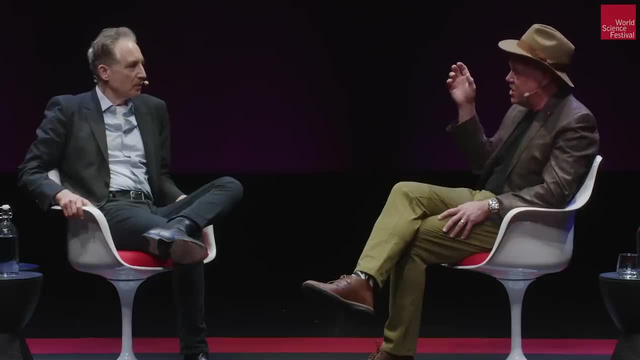 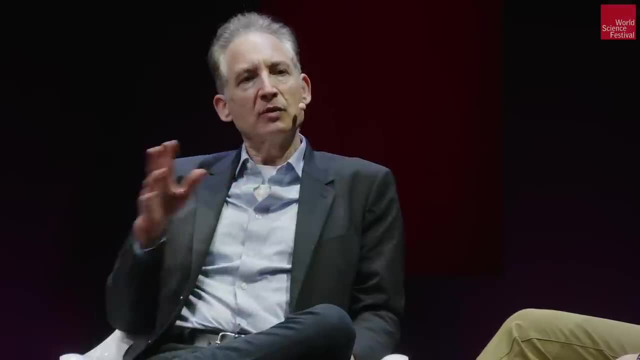 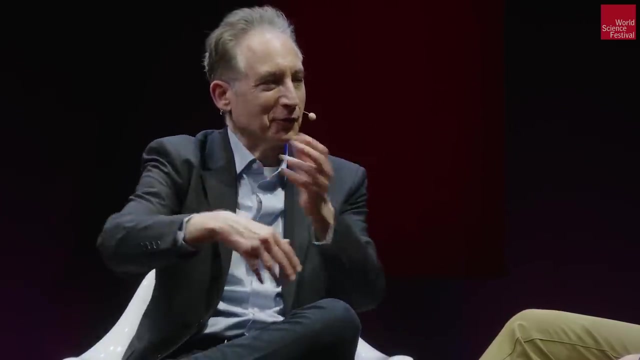 Other than large brained humans And possibly Neanderthals, which are large brain humans? And how do you distinguish it from other things that are, granted, are different, but, like bowerbirds, when they make their, their nest to try to try, where they make an elaborate design, that's a radically different kind. 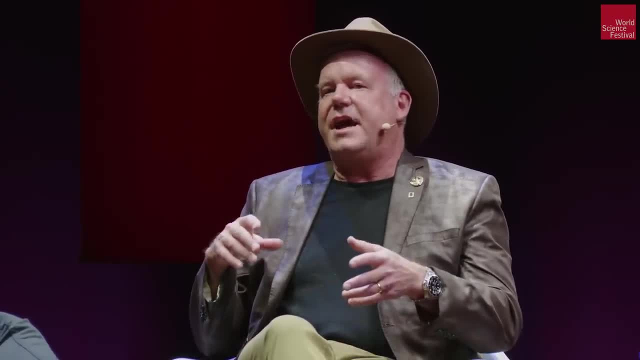 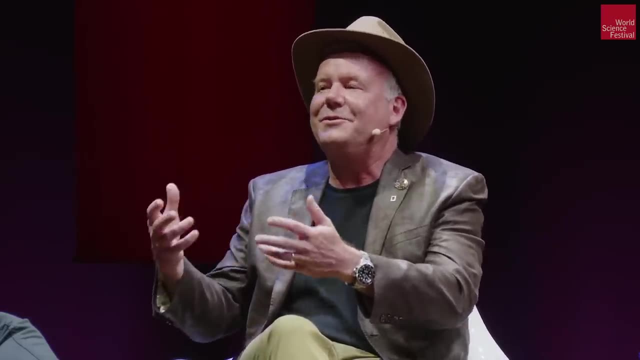 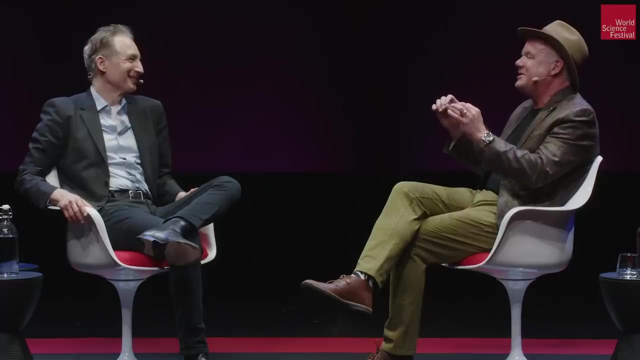 Radically different kind of thing. That's a, that's a sort of it's. I believe that I think I think we may, as humans, be in a moment where we're about to lose our special human, Special nature. The idea of human exceptionalism maybe just died. 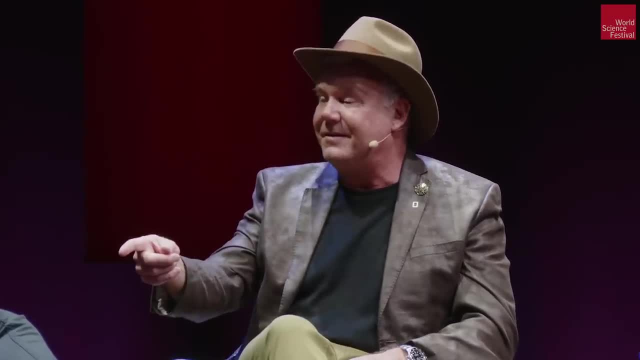 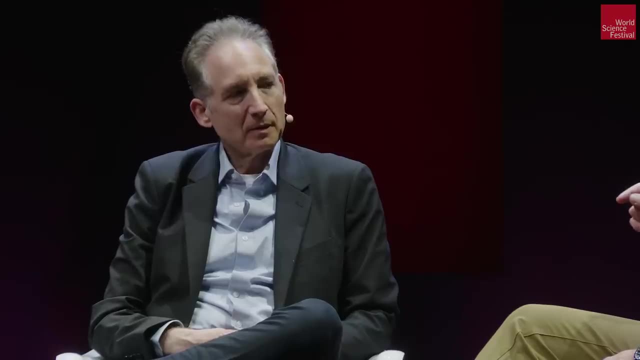 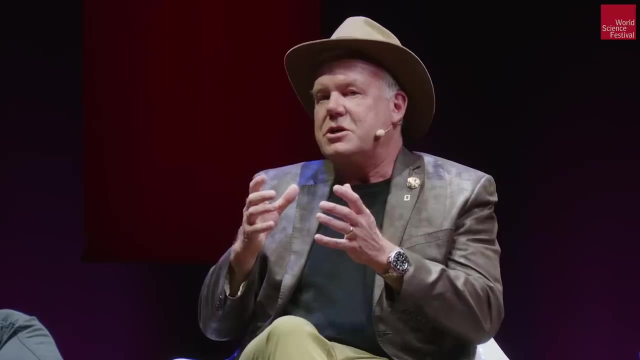 I don't know if that's that different. I know we made it different, But homo naledi just proved to us that another species with a brain that's not our brain, and much smaller but smaller, but incredibly smaller, Yeah, Accomplished effectively the entire cultural package. 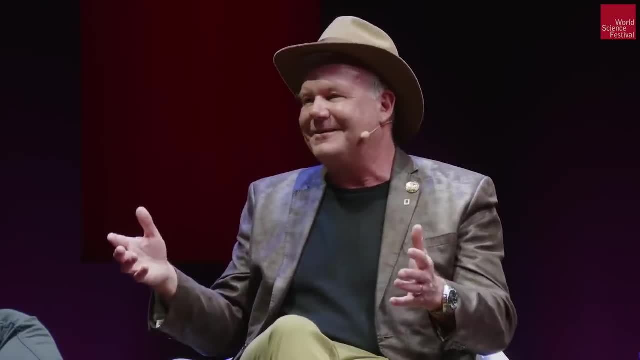 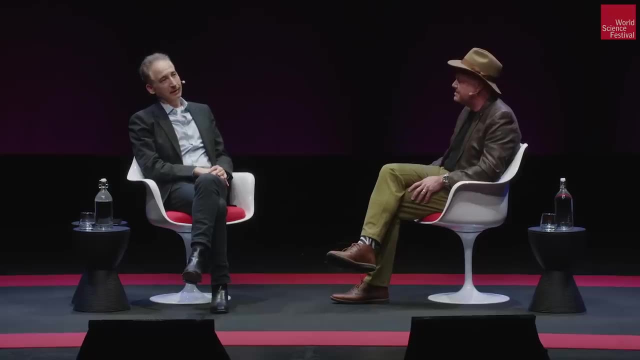 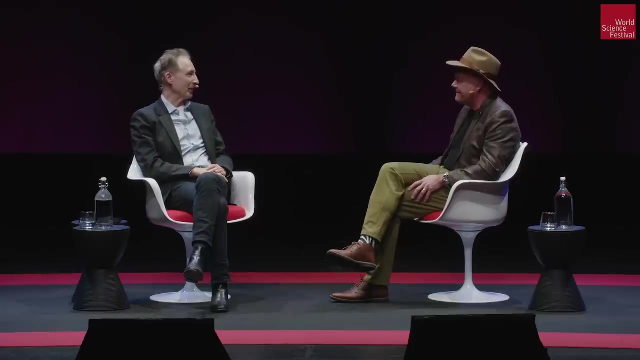 that probably was used moments before the definition of what it means to be human. It's an absolutely remarkable story and it is something that we will all be looking forward to, And you know. thanks enormously for all you're doing to clarify where we all came from. 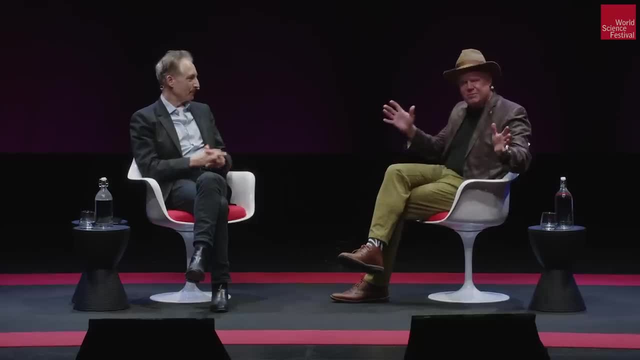 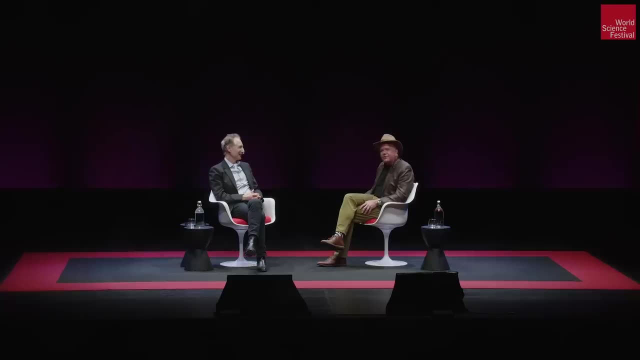 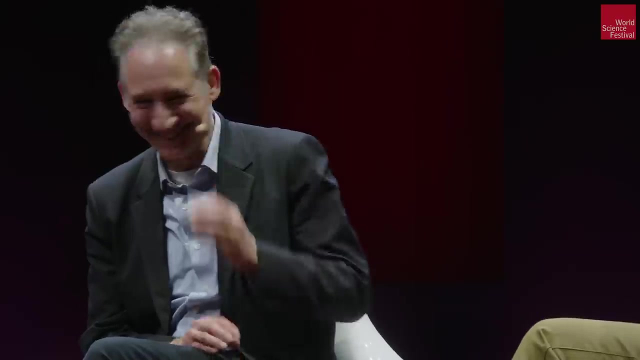 Thanks, Brandon, And thank You guys. By the way, I love Brisbane- Oh my goodness, I'll get in trouble for this on YouTube, but it's like Miami without people. Miami, Miami, Thank you. He said that. 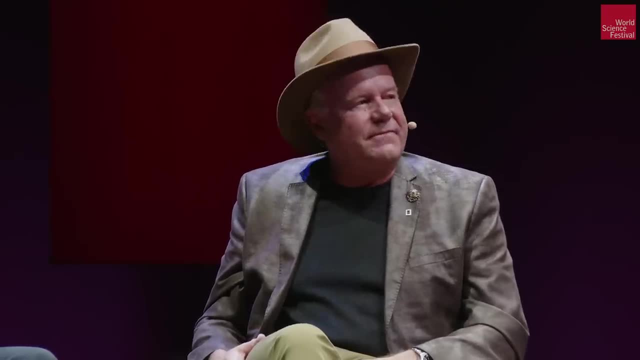 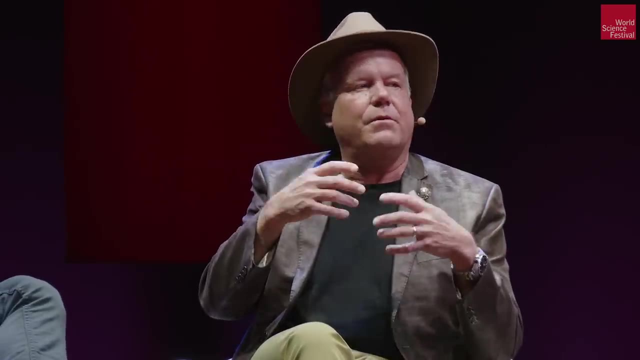 I'm going to say it too. And secondly, I just want to say one thing. I hope what you get from this, because I really want to inspire You know I speak to kids all over the world And part of what the thing is is often they're depressed. 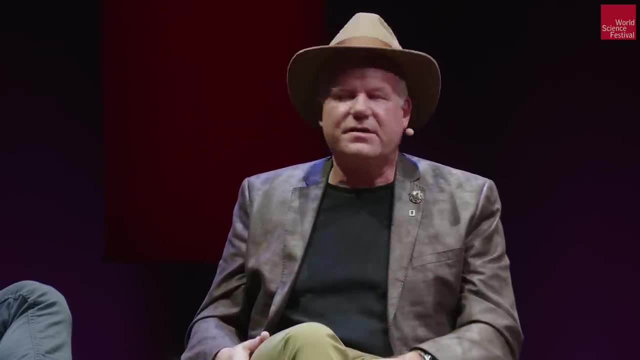 about the idea that they won't be. They don't know how they're going to contribute Young scientists, how they're told that all the great discoveries have been made, that if you're moving in you're just standing on the shoulders of giants. 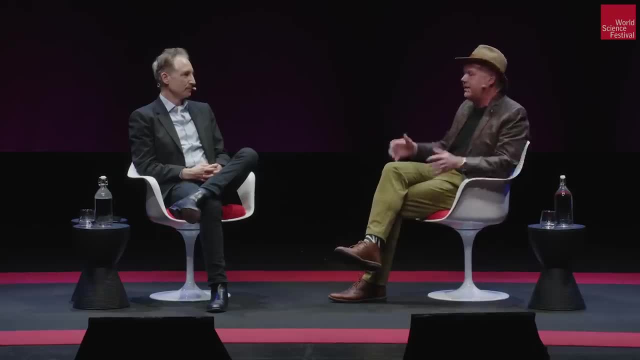 And what I hope. the reason I want to tell my whole story is. I hope you see that that's just not true. We haven't touched discovery. We are at the front edge and I'm a field that thought it was over 20 years.